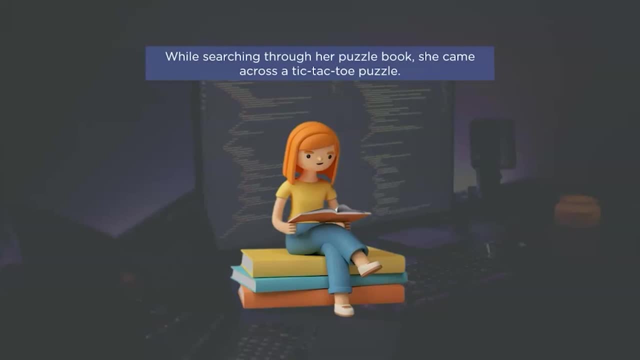 play this puzzle game. This fact captivated her interest, encouraging her to begin playing this tic-tac-toe puzzle game. Rachel began playing this game with her friend Alex, who already knew how to play this game. As a result of her repeated failures, Rachel became frustrated and 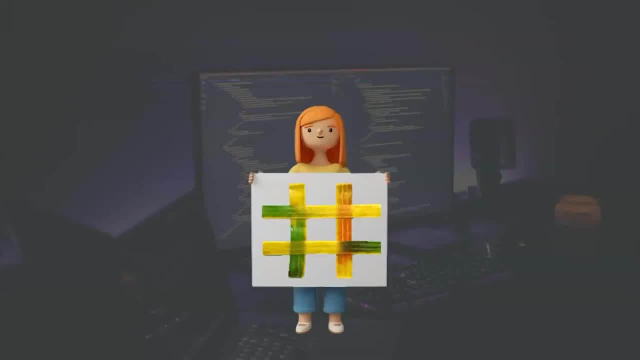 started to question how she could go on a winning streak. After a few games, Rachel started remembering the outcomes of each of her moves which contributed to her in previous games. By using those memories of her previous games, she started getting hold of the logic behind object placement in tic-tac-toe puzzle. 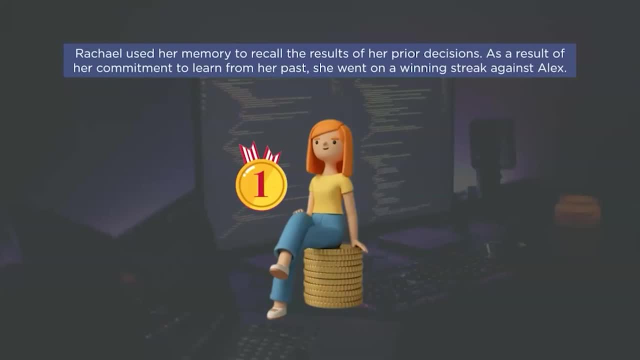 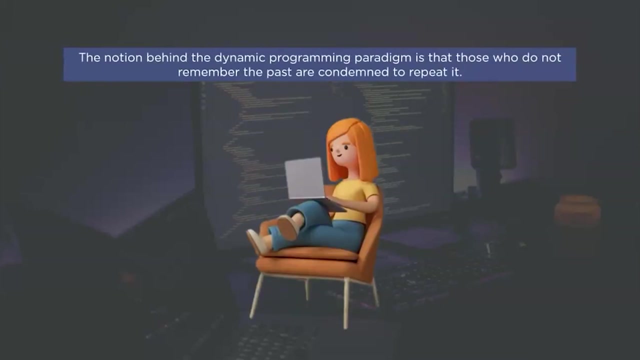 Rachel's ability to memorize things helped her decide where to place an object on the tic-tac-toe board. As a result of her hard work and commitment to learn from her experiences, she went on a winning streak against Alex To solve complicated permutation issues. the dynamic programming paradigm. 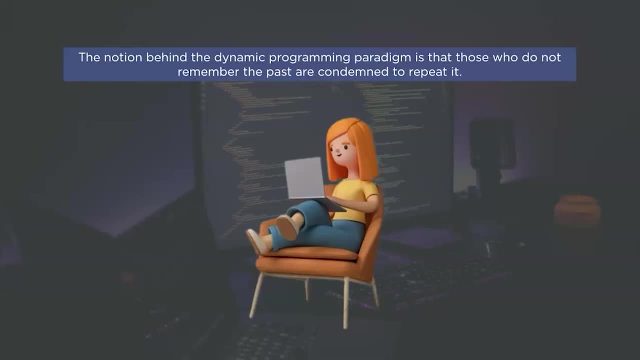 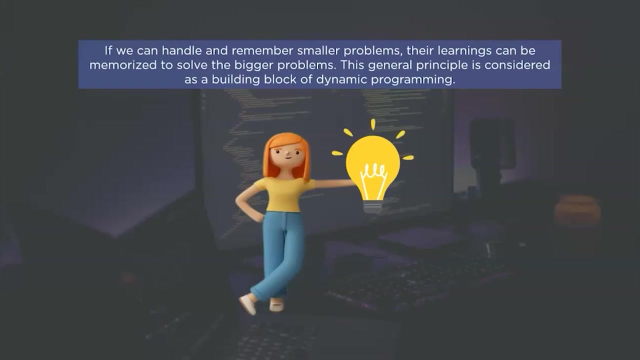 employs a similar concept of memorization. Furthermore, this dynamic programming paradigm is completely based on the philosophical idea that people who do not remember the past are condemned to repeat it. The dynamic programming principle states that if we can solve smaller sub-problems, then their 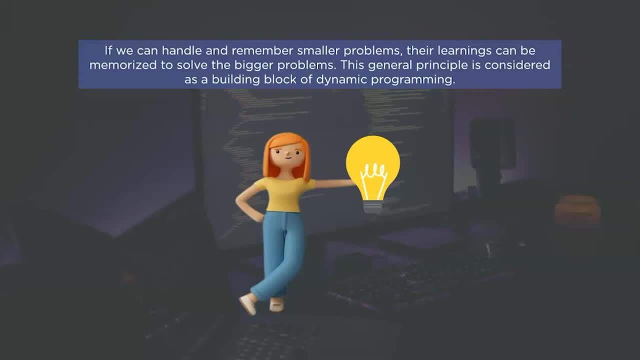 learnings can be memorized to solve the larger problems. This fundamental notion is acknowledged as a foundation of dynamic programming. Moving ahead, let's look at the dynamic programming paradigm. The dynamic programming paradigm employs a similar concept of memorization. Furthermore, this dynamic 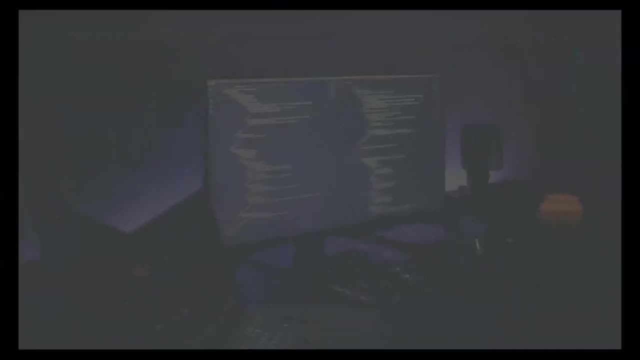 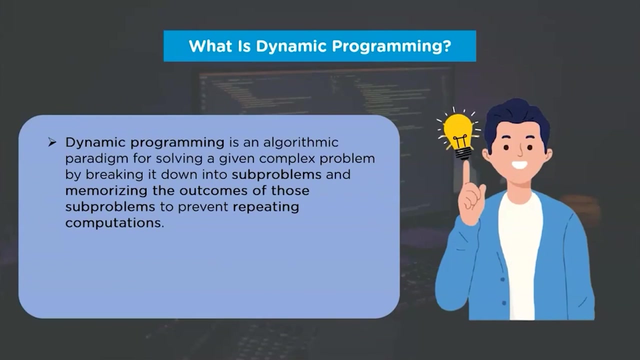 programming paradigm employs a similar concept of memorization. These are know, wide spectrum, sub problem basism and paradigm paths that lets her identify the combination of themselves and their own subproblems. The dynamic programming paradigm employs a similar concept of unconnected. 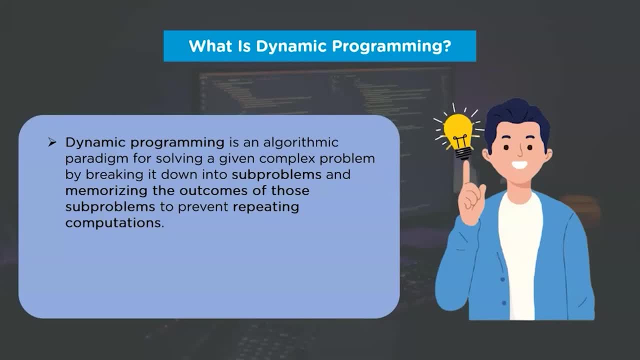 automatically kinder, dynamic, Horus-style number of by-e theft patterns For their targetistic of understanding sum we try to make minimize to see either the smaller subproblems. However, in divide and conquer the subproblems do not repeat themselves, whereas in dynamic programming the condition is entirely opposite. Well, that means dynamic. 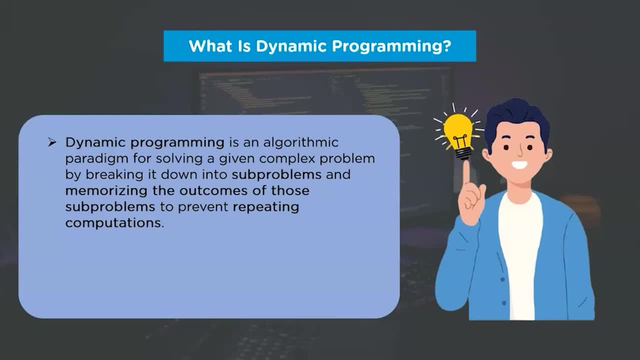 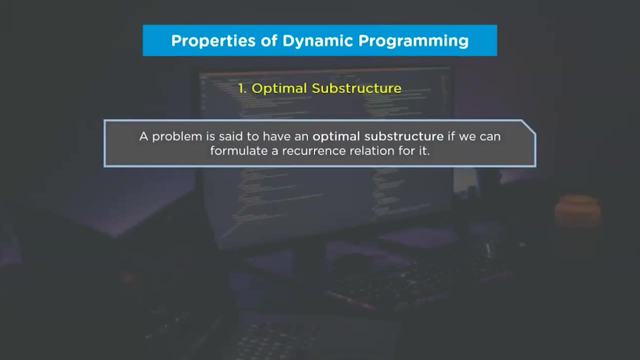 programming has different properties than the divide and conquer approach, And the problems which abide by those properties can only be solved using dynamic programming technique. So, moving forward, let's discover the properties of dynamic programming. The first property that we have is optimal substructure. If we can establish a recurrence relation for 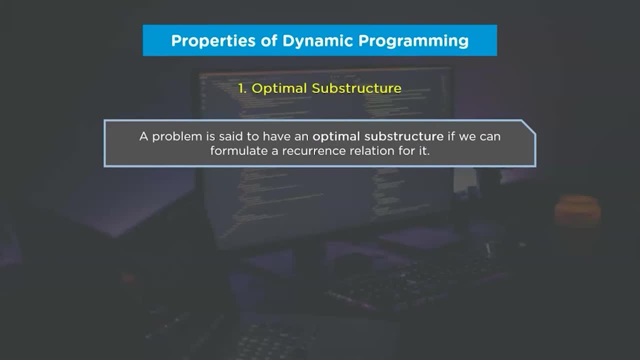 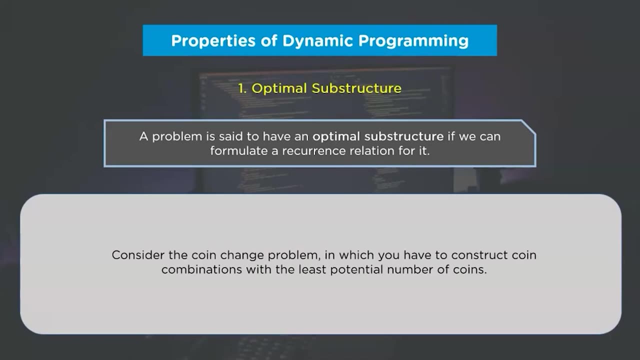 a given problem, then it is said to have an optimal substructure To understand this property. let's have a look at an example. The example that we are going to discuss is called the coin change problem, which is one of the most famous DP. 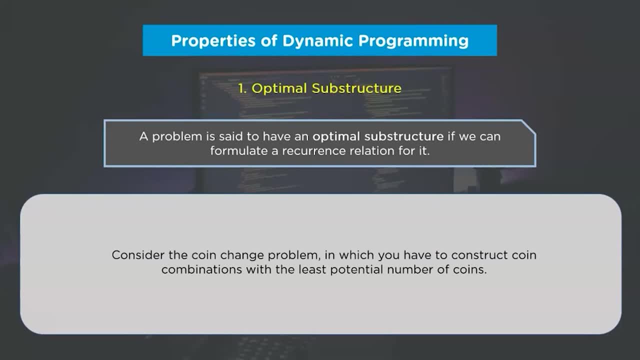 problems. In this problem we have to construct a coin combination with the least potential number of coins resulting in the desired final amount. Let's say we have a recurrence relation for a given problem. then it is said to have a limitless supply of $50,, $20,, $10, and $5 coins And the amount for which we need. 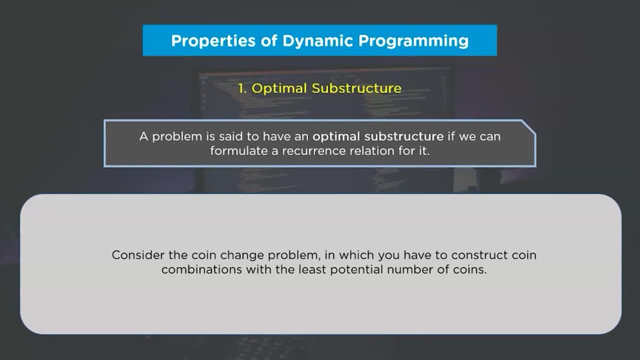 the least possible number of coins is $85.. So to formulate the solution, we'll have to traverse through all possible permutations of coins. The most logical solution to this problem is to add the coin of largest value at each iteration, which does not take us past. 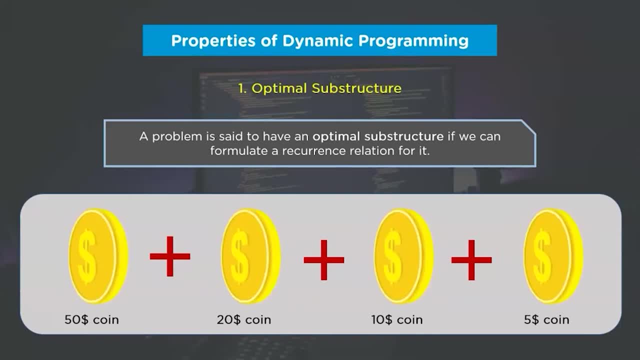 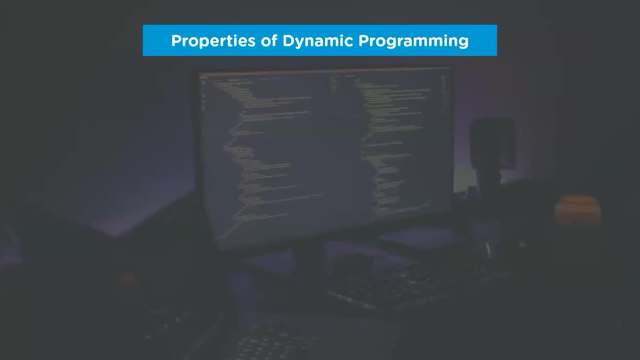 the expected amount, ie $85.. That means we break this problem into two parts. The coin of highest value at each iteration is the coin of largest value at each iteration. This conversion of larger problem into smaller subproblems is known as optimal substructure. 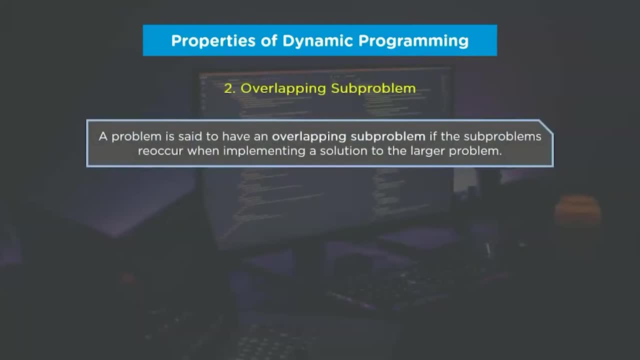 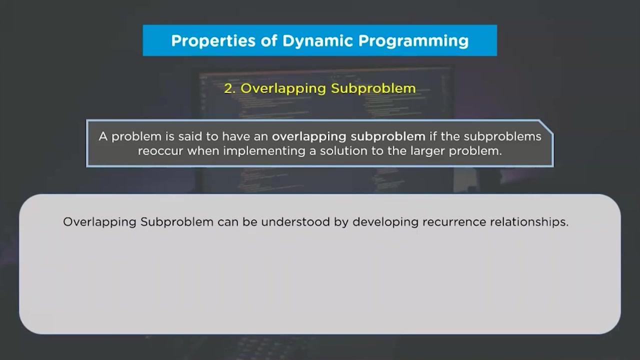 The next problem we have is an overlapping subproblem. If the subproblems recur while implementing a solution to the broader problem, then that problem is said to have an overlapping subproblem. Formulating recurring relation is the sole technique to determine if a given problem has an optimal subproblem or not. To understand this better, we'll have a look. 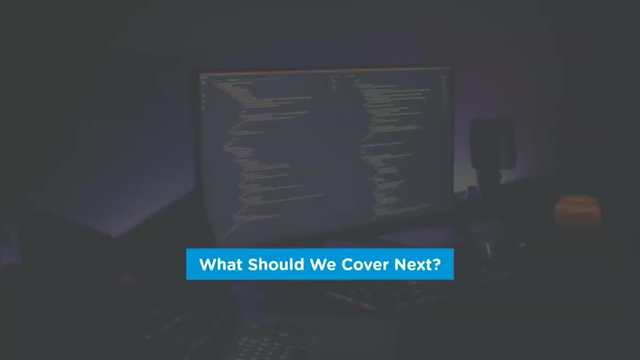 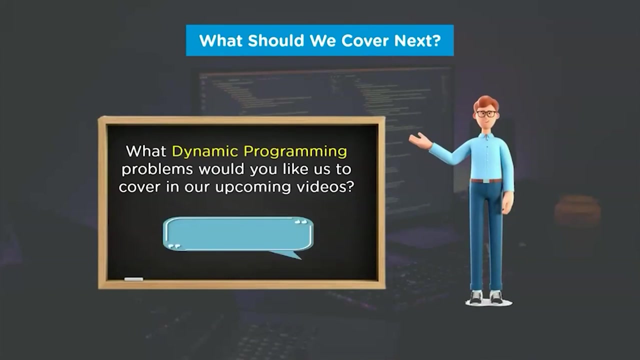 at an example of a Fibonacci series program. But before we get into details of that, we'd like to ask you: what dynamic programming or competitive programming topic would you like us to address next? You can mention the topics which you have doubts about in the comment. 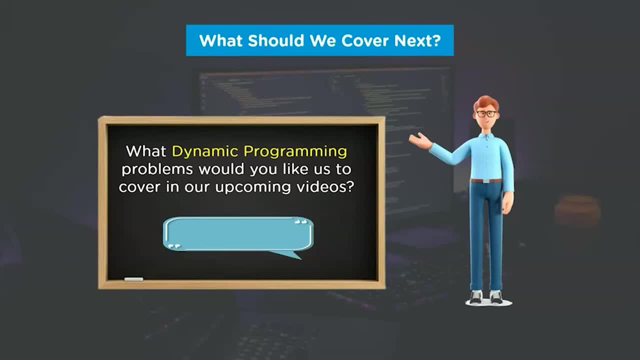 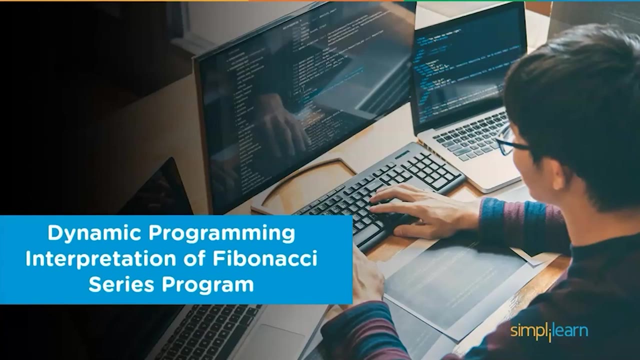 section below and we'll surely create an exciting video about it in the next few days. So, guys, make sure you post a comment with the DP or competitive programming topics you'd like us to cover in upcoming videos. Now, coming back to dynamic programming, we'll cover the 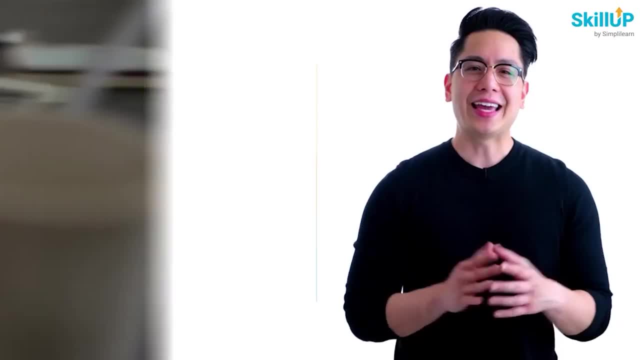 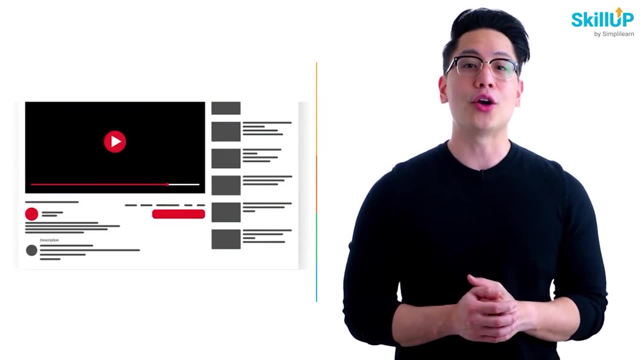 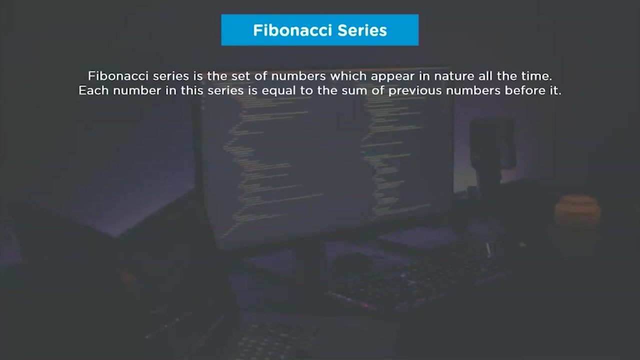 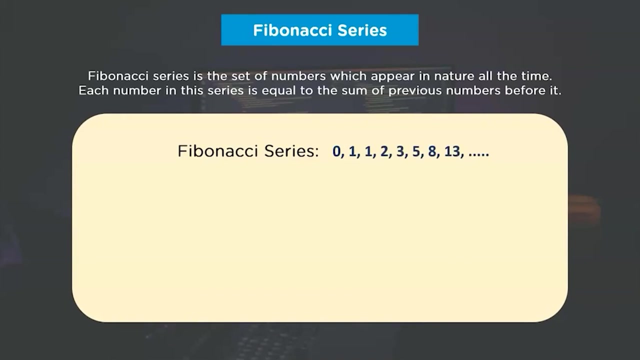 mathematical interpretation of Fibonacci series program. The Fibonacci sequence is a group of numbers that frequently appears in nature and are. Each number in this series is the sum of two previous numbers that come before it. The sequence goes like 0,, 1,, 1,, 2,, 3,, 5,, 8,, 13 and so on. 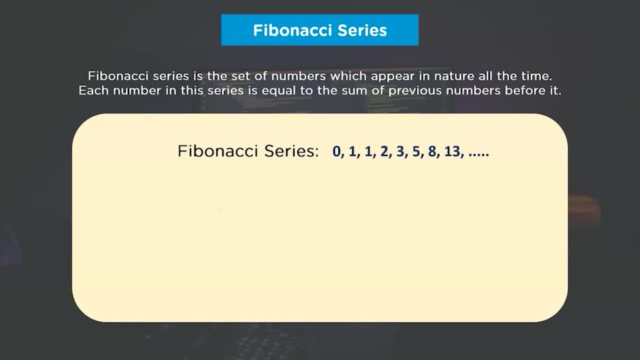 Let's say the n is iterator element to calculate consecutive Fibonacci numbers And for the first two iterations that are 0 and 1, the resultant Fibonacci values will be simultaneously 0 and 1.. Otherwise the Fibonacci values will be the sum of previous two Fibonacci numbers in the 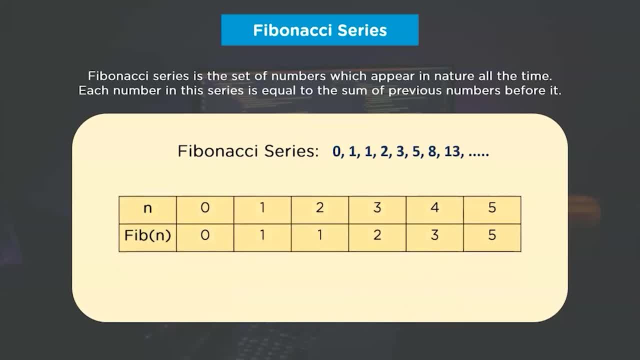 sequence. That means when the value of an iterator element becomes 2, the consecutive Fibonacci number for it will be the sum of previous two numbers, in the sequence that is 0 and 1.. So the resulting Fibonacci number will be 1.. 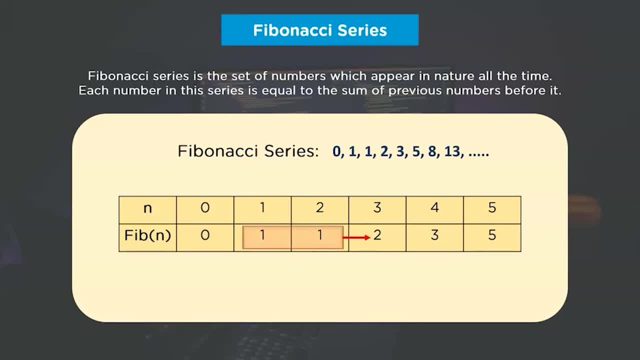 Now, when the iterator element n becomes equal to 3, the consecutive Fibonacci numbers for it will become 2.. For the next iteration, n is equal to 4.. The Fibonacci values will be the sum of 1 and 2, that is 3.. 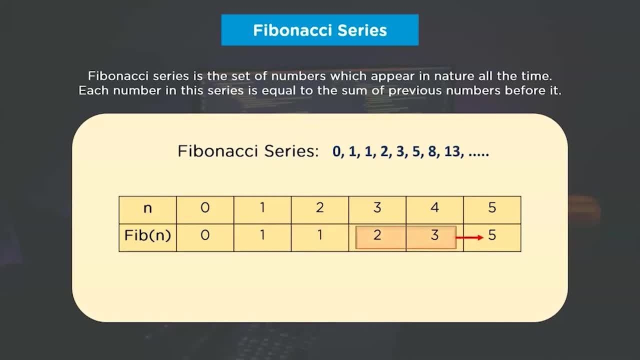 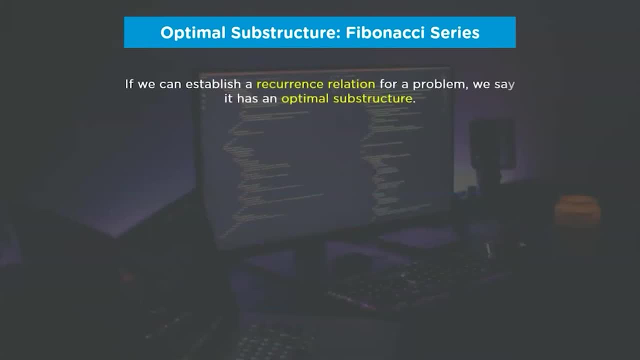 When n becomes equal to 5, the resultant Fibonacci numbers will be 5.. And similarly the further numbers in sequence can be calculated. And now, if you observe the Fibonacci problem closely, you'll see that the breakdown of bigger problem is done into smaller subproblems. in previous slide. 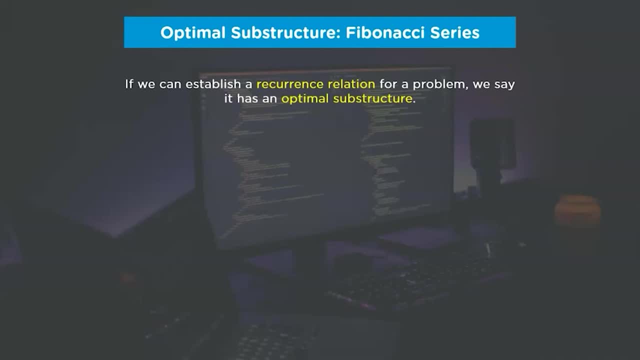 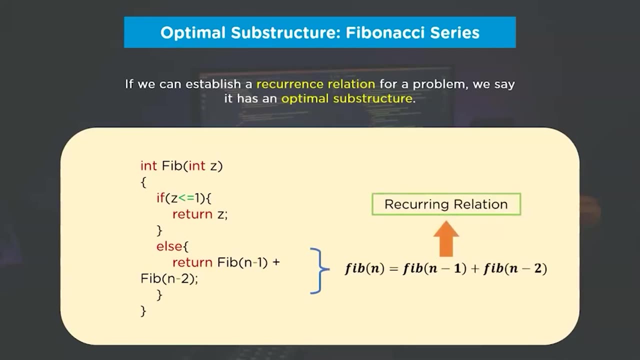 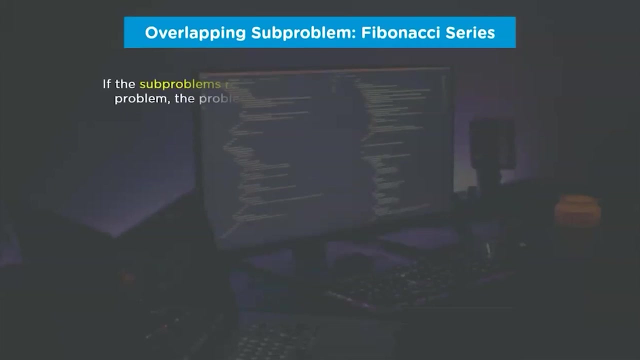 This means the Fibonacci sequence problem has an optimal substructure And the program for the Fibonacci sequence also represents the same. These highlighted statements are representing the recurrence relation in our Fibonacci program. Now, what about the overlapping subproblems? Well, a problem is said to have an overlapping subproblems if any subproblem repeats while 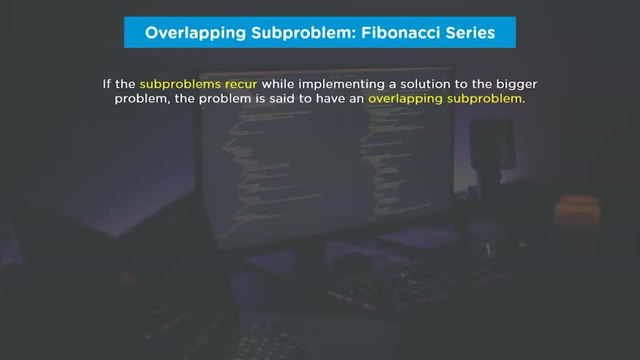 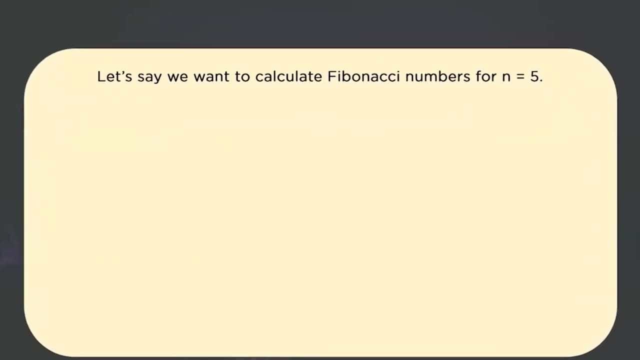 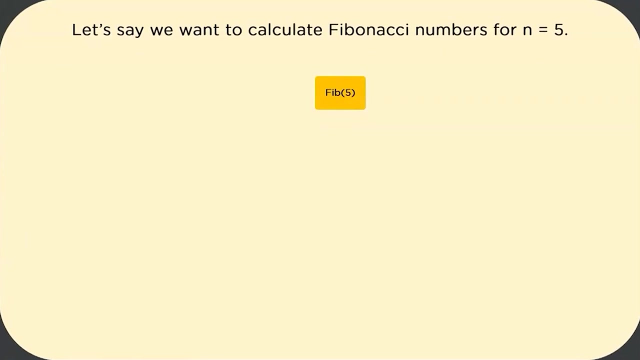 implementing the solution to the broader or larger problem. Let's say we want to calculate a Fibonacci number. The Fibonacci number for n is equal to 5.. The first activation record that will enter the memory stack will be Fib of 5.. And to calculate the Fibonacci value for number 5, our recursive program will call function. 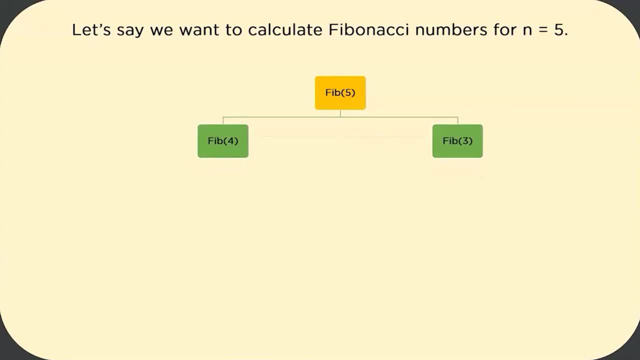 Fib4 and Fib3.. Further, to calculate Fib4, the IDEA will invoke Fib3 and Fib2.. Next, it will calculate the sum of Fib2 and Fib1 to calculate the value of Fib2.. And further, it will invoke Fib1 and Fib0 to contemplate the value of Fib2.. 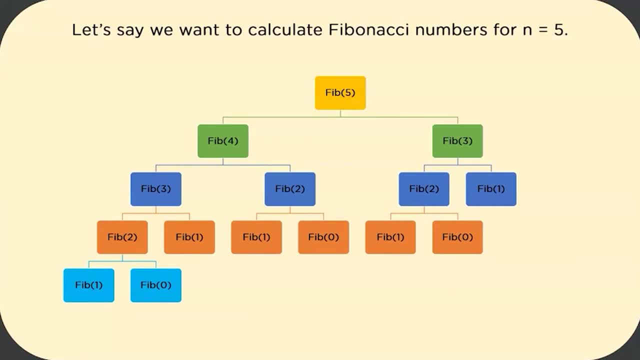 Now we have generated the right side of our call stack tree hierarchy. Similarly, the other missing pieces will get calculated by the compiler with the help of recursive calls. Now, if you observe this activation hierarchy, you will get that few subproblems are repeated in this problem. 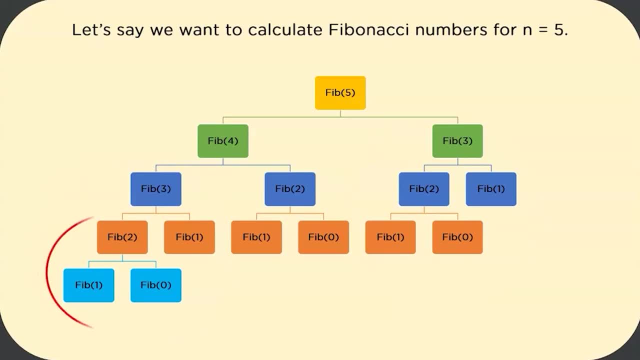 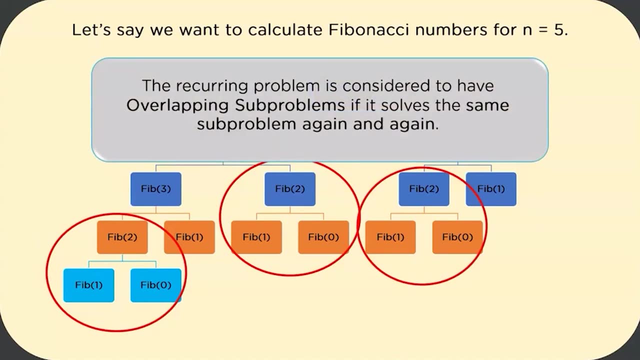 The Fib3 has been calculated twice And the Fib2 has been calculated twice And the Fib2 has been calculated twice And the Fib2 has been calculated three times. in our program, This repetition of the same subproblem while solving more significant problem is called 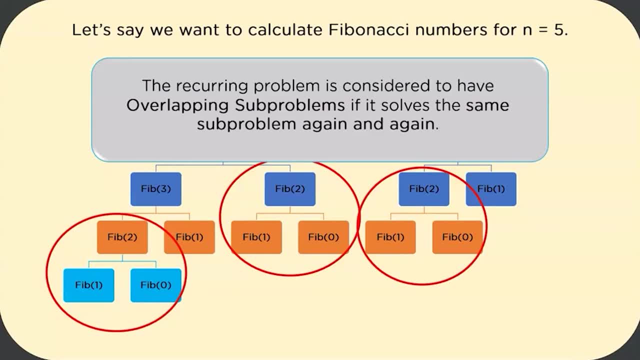 as overlapping subproblem property. Due to the multiple calls, the computational complexity of recursive programs almost increases exponentially And those calculations are entirely unnecessary. But before we understand how to avoid all unnecessary computation, let's try to figure out the time complexity of our Fib function. 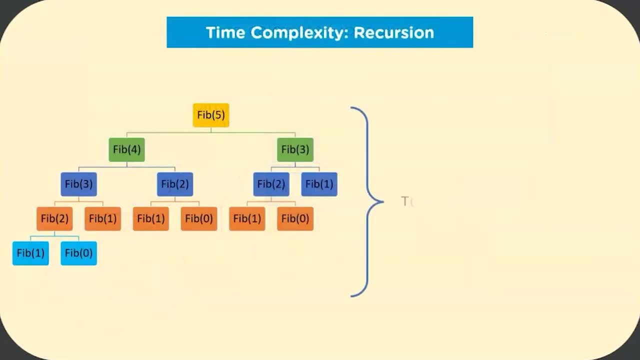 So let's start with the Fib function. Look at the time complexity relation written over here. This says that the time taken to calculate Fib n will be equal to the time taken to calculate Fib of n-1, plus time taken to calculate Fib of n-2, plus the time taken to add these numbers. 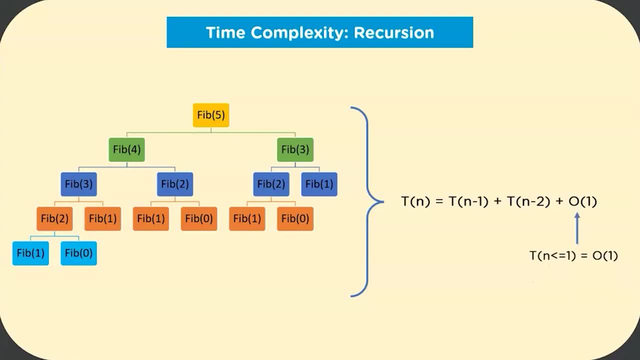 together. Clearly, for n is less than or equal to 1, the Fib of n is going to be big of 1, as we are not going to make any recursive calls for them. Also, intuitively, we can say that T of n will take big O of 2 to the power n. 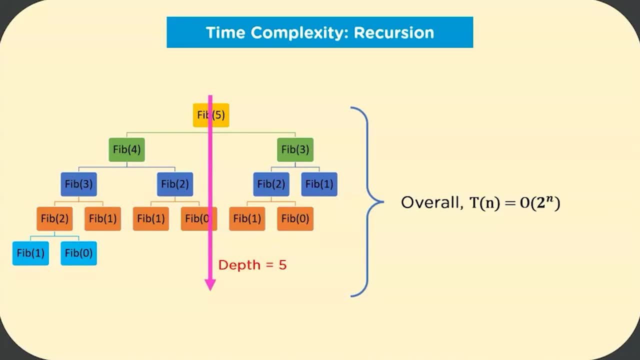 We can contemplate this from the recursion tree drawn on the left side. For n is equal to 5, we get a binary tree of depth 5.. For n is equal to 4, we get the binary tree of depth 4, and so on. 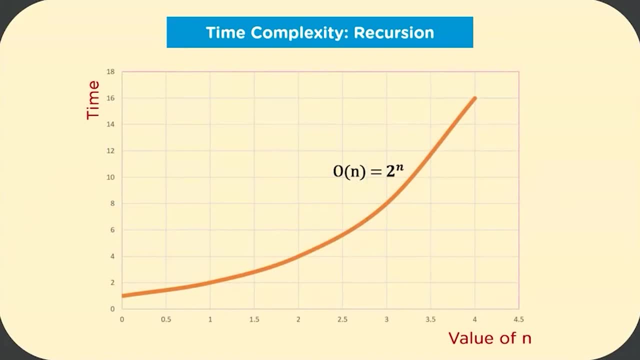 This implies that the time complexity of our algorithm grows at an exponential rate and graph shown on your screens depicts that. Let's talk about the time complexity of our algorithm. Let's start with the Fib function. We will be able to calculate the time complexity of our Fib over n-1 plus time taken to calculate. 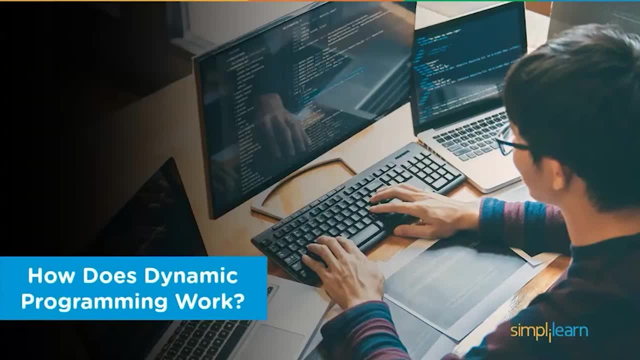 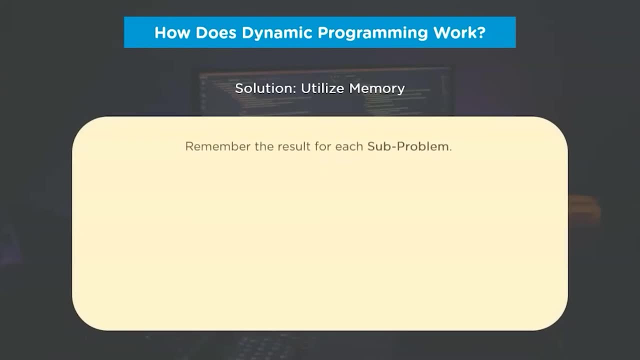 Moving ahead, we'll try to understand how we can reduce this computational complexity using dynamic programming. The computational complexity can be removed by memorizing the result of subproblems. In terms of computer science, we can refrain from doing unnecessary computations by utilizing the memory to store the results of subproblems. 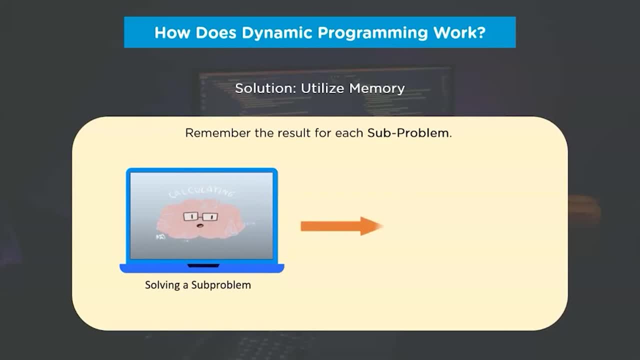 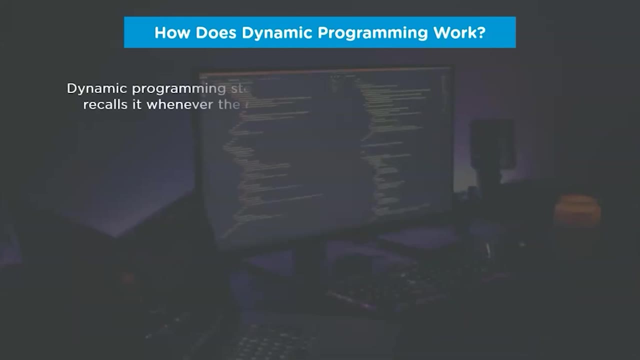 In dynamic programming, we calculate the result for subproblems and store it in memory allocated by an operating system. When that same subproblems get activated in our call stack, we access the memory in order to return the result that we have calculated previously. Now you must be thinking about how we can store the result in memory. 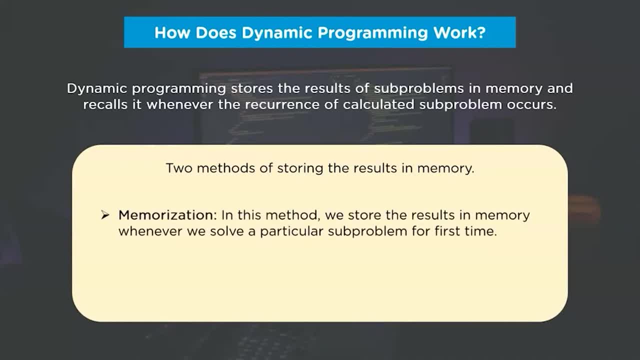 Well, we can store the results in two ways. The first one is memorization and the second one is tabulation. In the case of memorization, we store the result in memory whenever we solve a particular subproblem for the first time, Whereas in the case of tabulation. 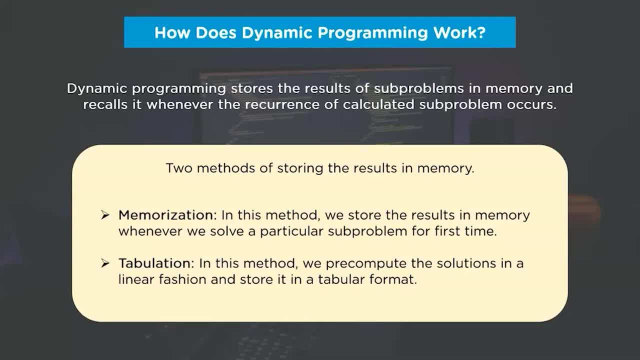 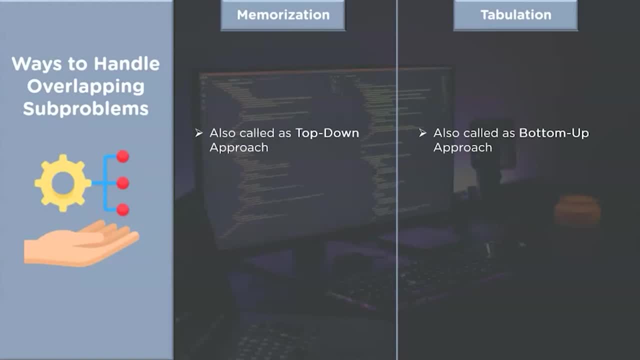 We perform the same task. We per-compute the solution in a linear fashion and store them in a tabular format. Memorization is also known as top-down approach, whereas tabulation is known as the bottom-up approach. In general, these names are assigned to these methods based on how they approach problem. 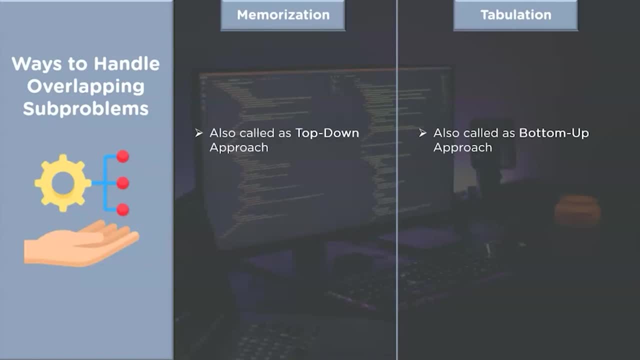 solving. The first one saves results in memory based on call stack occurrences. The second one, on the other hand, solves the subproblem in sequential manner. For the top-down approach, We maintain a lookup table. When we compute any subproblem, we store results in lookup table, and when the recurrence of 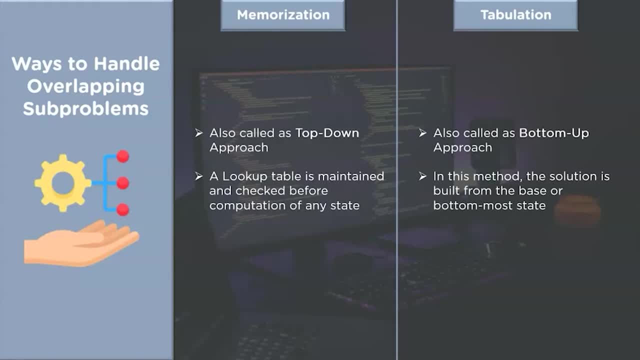 this subproblem happen. we directly fetch its value from our lookup table, Whereas in the case of bottom-down approach, the solution is built from the bottom most case. In addition, the memorization process is recursive. However, the tabulation process becomes iterative. 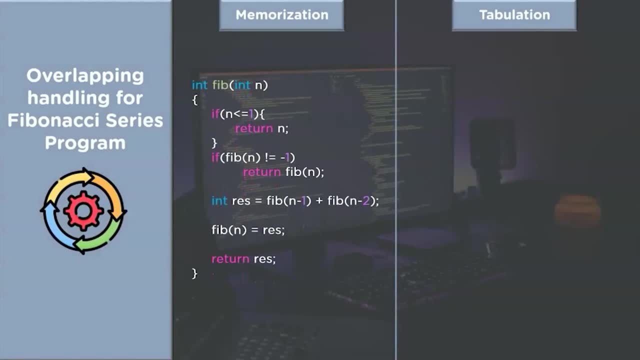 So if we implement the Fibonacci series program using the top-down approach, the answer will come out. We start the problem. All something is good, not a problem. We keep routine. we have excepted like a period. I renovate the problem options. 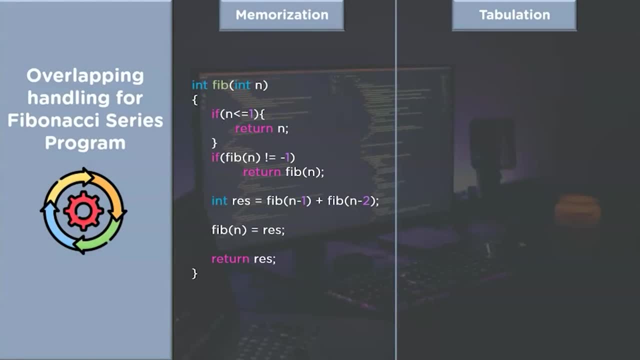 Then the code for function FIV will look something like this: And this one additional step- FIV- n is equal to res- will do the memorization job for us. If we develop a Fibonacci sequence program using bottom-up approach, our program will look something like this: 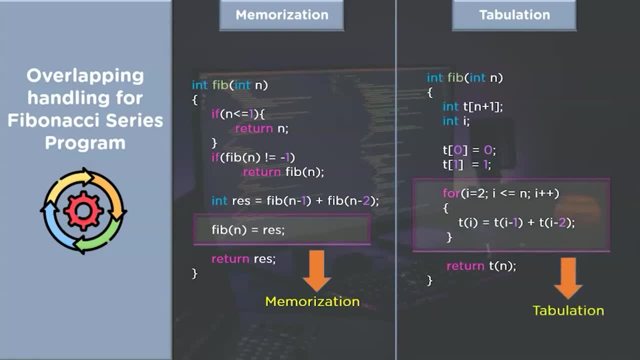 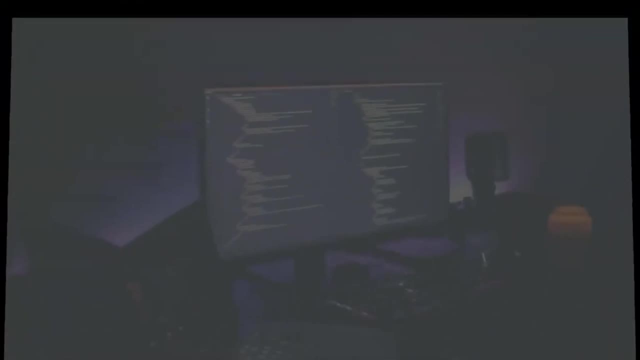 This highlighted for loop part calculates solution to all subproblems from the base case. I hope you guys are clear with both methods of dynamic programming. Now, moving ahead, we'll discuss when to implement dynamic programming solution for any given problem. Remember guys, you can solve any problem using dynamic programming which abides by the properties. 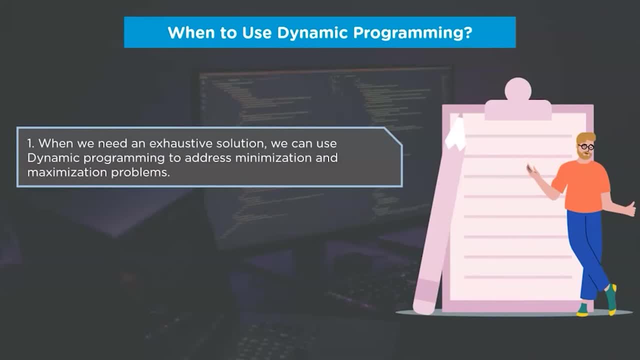 of dynamic programming. Most frequently you will come across the minimization and maximization problems, which are readily recursive in nature. If you need exhaustive solution for these problems, then you can solve them using the dynamic programming paradigm. The permutation combination problems Can also be solved using dynamic programming. 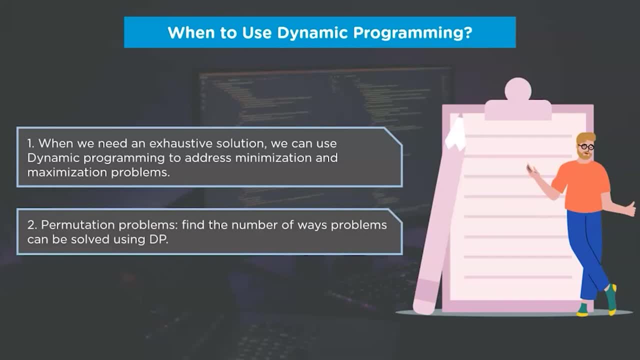 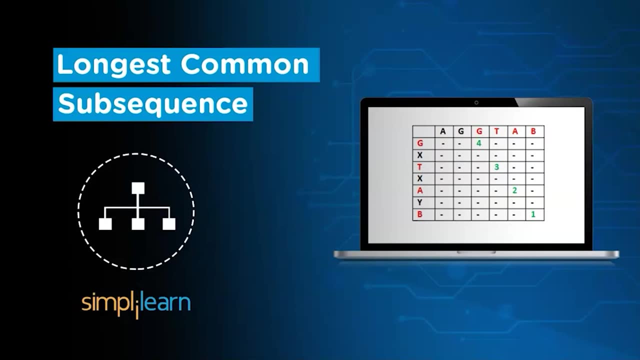 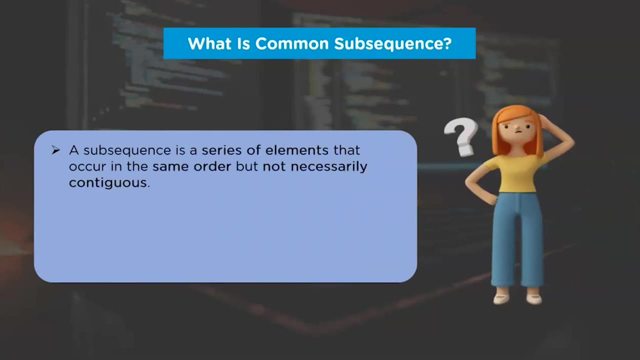 The problem statement, beginning with find the number of ways are the famous permutation problems that can be solved using dynamic programming approach. The term longest common subsequence clearly directs us towards some sort of relation between two sequences. A sequence is nothing but a series of elements that occurs in same order but are not necessarily. 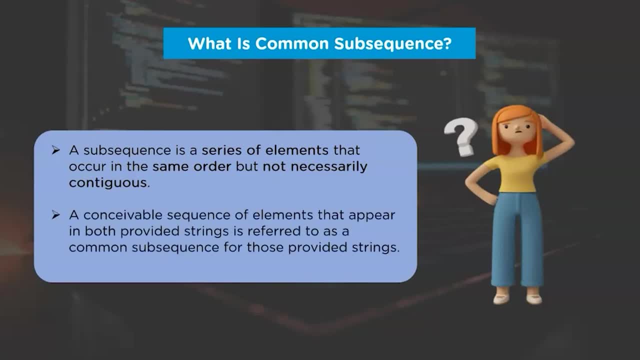 contiguous. From this definition we can conclude that a sequence is nothing but a series of elements that occur in same order but are not necessarily contiguous. From this definition we can say that the longest common subsequence will be the term that both given strings will contain. 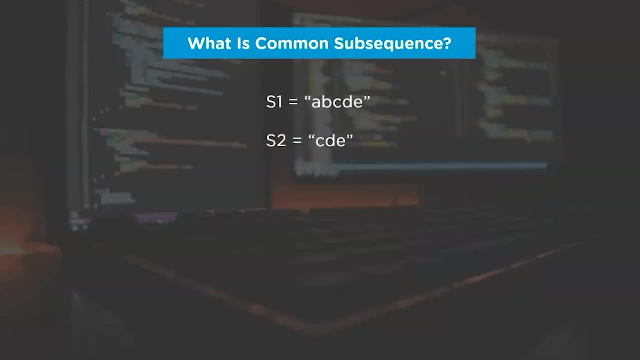 To understand it more clearly, let's have a look at an example. In this example, I have taken two strings. There is nothing like substring here, right? If you have studied the KMP algorithm, you will remember the problem as string and substring. 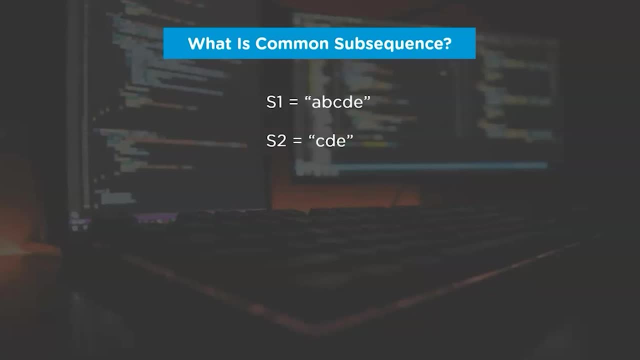 In that problem we had to find a substring inside a given string. But this scenario is totally different from that. different strings here. Here you can clearly see that string 1 is larger and string 2 is relatively smaller. Now for these two strings possible common. 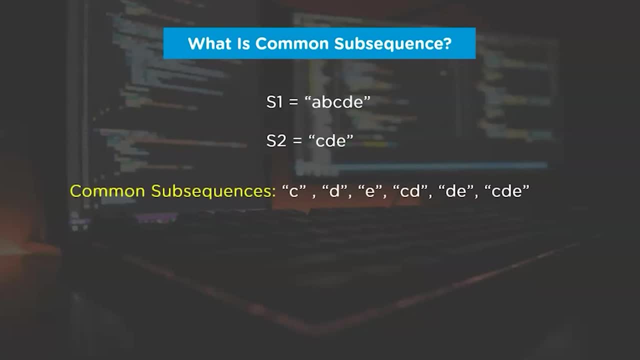 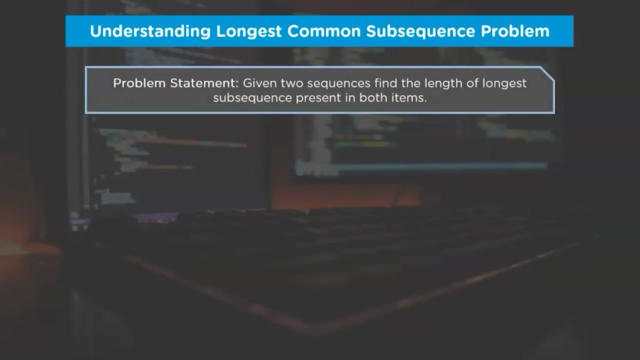 subsequences are as shown on the screen And from this you can clearly say that the longest common subsequence will be CDE, Moving forward. let's dive further into this LCS problem to understand the logic behind it. The problem statement for the LCS states that, given two strings, find the length of common. 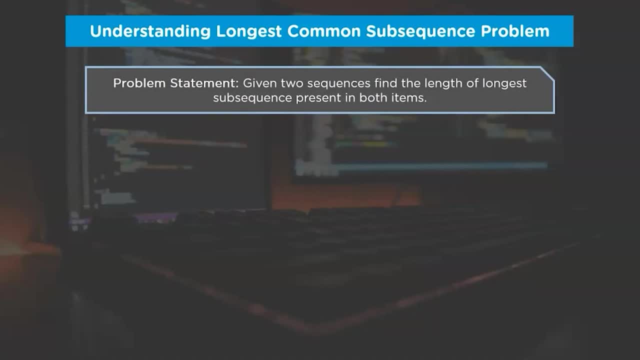 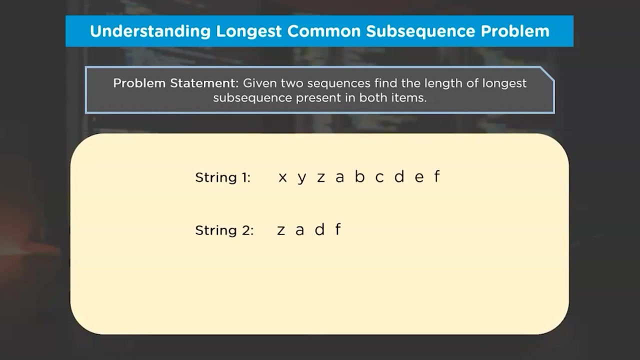 subsequences present in both the strings. That means in this problem we'll be given two different strings with length m and n respectively, And from these two strings we'll have to find the longest common subsequence with length k. Let's consider these two strings present on our screens. 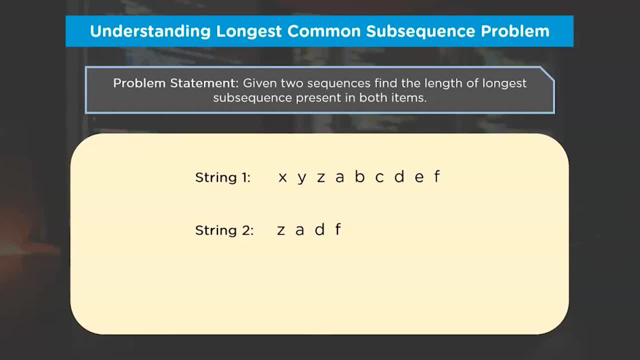 We'll try to find out the LCS for both of these strings here. We'll try to find out the LCS for both of these strings here We'll try to find out the LCS for both of these strings. here We'll try to map patterns present in string 2 to string 1.. 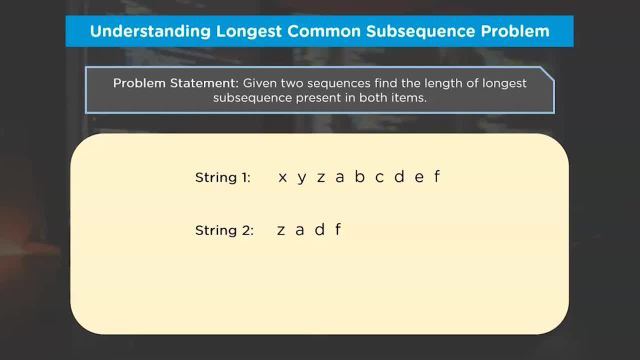 Now let's pick the first character in string 2, that is Z. Now we'll match this character to the character present in string 1.. And the first character is x, So we'll map it with x, But Z and x do not match. Hence we'll move towards the next character. 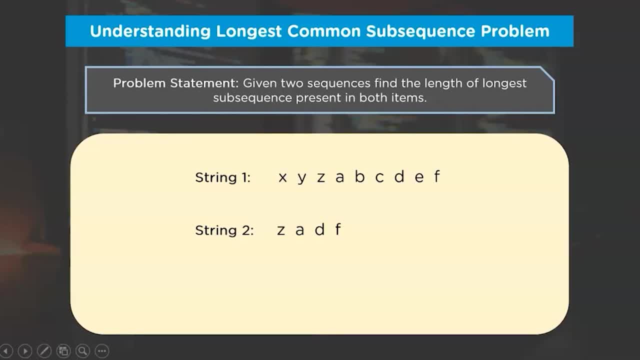 Next character is Y And Z, and Y also does not match, Hence we'll move to the third character, that is, Z the match. So what we'll do is we'll include z into our longest common subsequence. The next character in our sequence is a, and we have a in string 1 as well, Hence we'll. 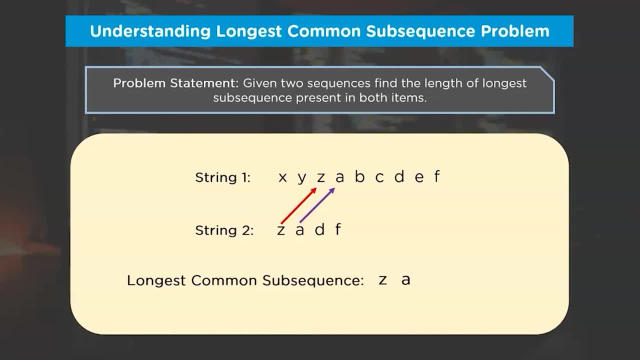 include a in our longest common subsequence. The next character in string 2 is d, and we have found match for d in string 1 as well, Hence we'll include it in our longest common subsequence. The final character in string 2 is f and we. 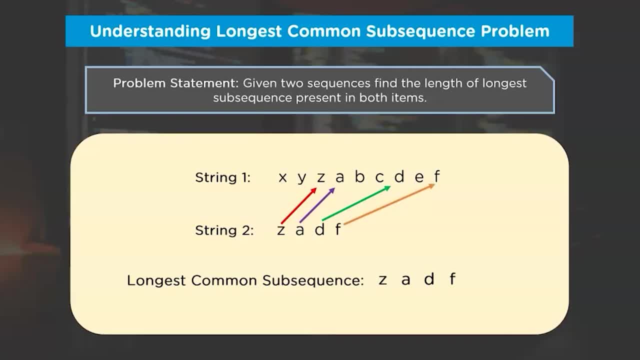 have found f in string 1 as well. Hence we'll also include it in our longest common subsequence. Finally, the longest common subsequence for string 1 and string 2 will be z, a, d, f Moving forward. let's discuss one more problem to understand LCS clearly. Here you can see: 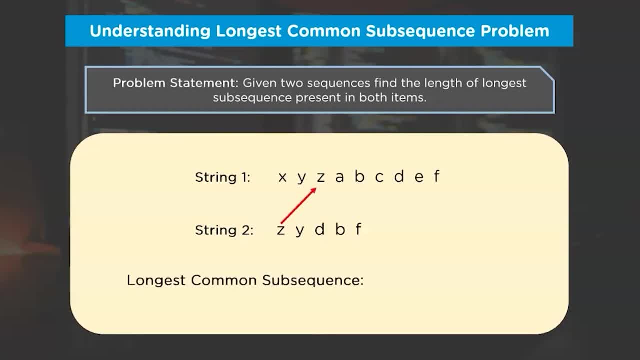 that z is present in both the strings. Thus we'll include it in our LCS queues string. The next character is y. It is also present in string 1, but the rule of LCS says that the sequence of character should not be changed, and here the 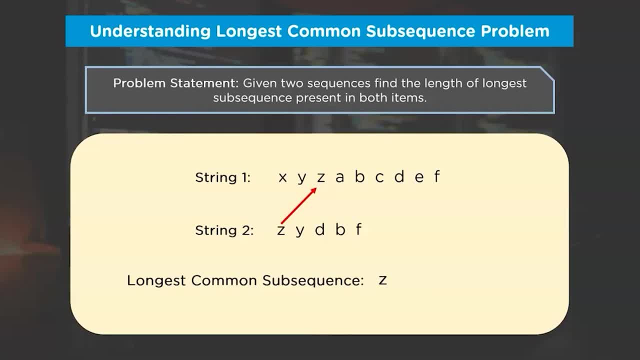 mapping line of z and y are intersecting, So we'll discard character y here and we'll pick the next character in string 2.. That character is d, and d is not intersecting with any other character, Hence we'll add it to our LCS string Now. 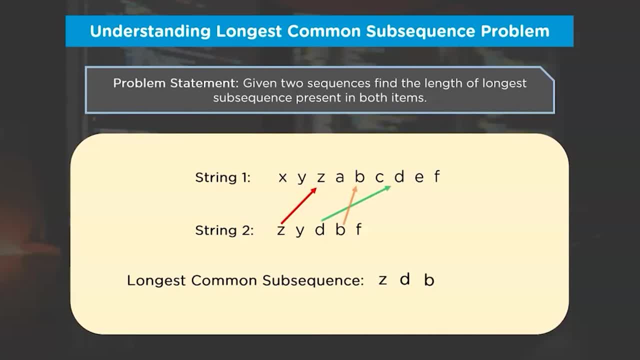 the next character b is also there in string 1, but we cannot insert it in our LCS string as it intersects with the mapping line of character d. Thus we'll discard this character. The next character f can be added to our LCS string as it does not intersect with any other mapping line. So the first LCS. 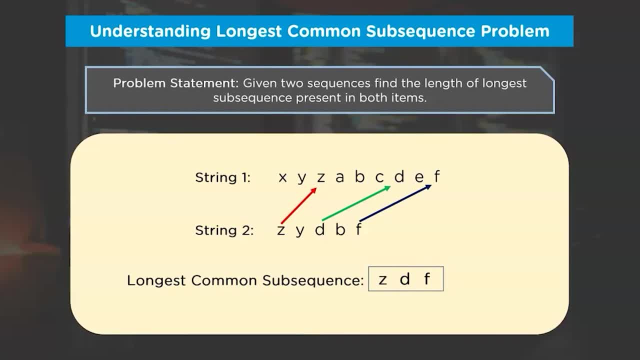 sequence will be z, d, f, and due to multiple intersections, there is possibility of having another sequence that can be larger in length than the previous sequence. For this sequence we'll begin from the second character of string 2, that is, y, and y is present in string 1.. Thus we can. 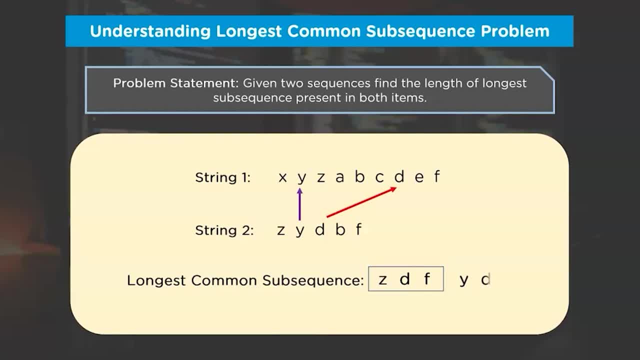 add it to the LCS. Next, we can add d to our LCS sequence. After this, we have b, but b cannot be inserted into LCS as it is intersecting with d, Hence we'll discard it. and finally, we'll include f into our LCS sequence. 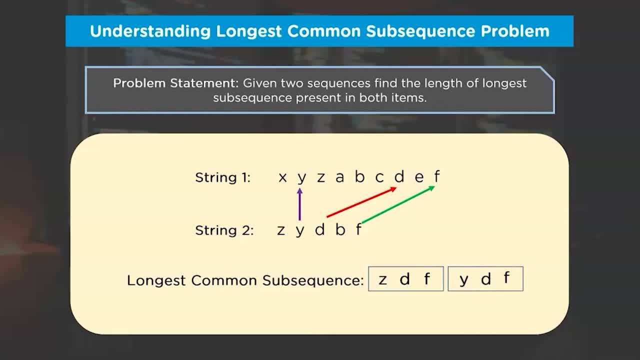 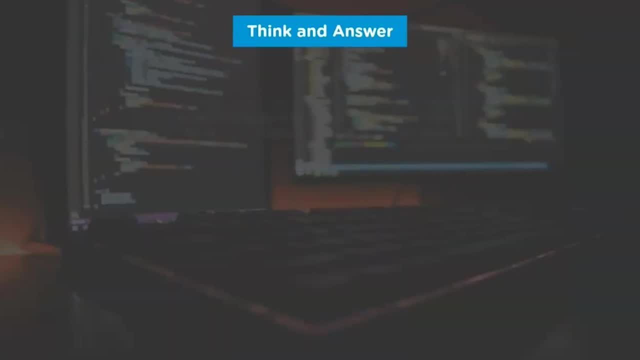 In this problem, both the sequences have the same length, Hence both of these sequences will be considered as Longish-Common Subsequences. I hope that you guys have understood the logic behind finding the Longish-Common Subsequences cause. we have a challenge for you guys to assess your understanding of the LCS. 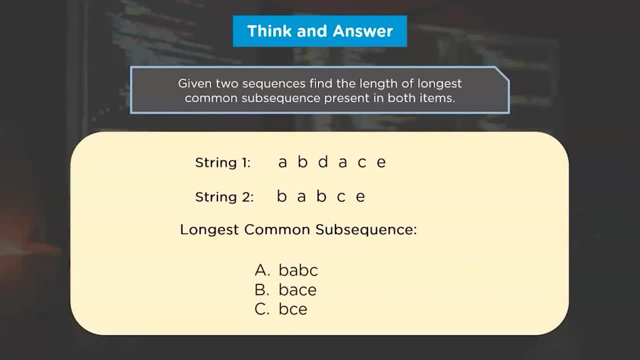 For these given sequences. you are supposed to find out the Longish-Common Subsequence. The options for this problem are b a, b c and b a c, d and BCE. You all can drop your answers in the comment box below. Let's see how many. 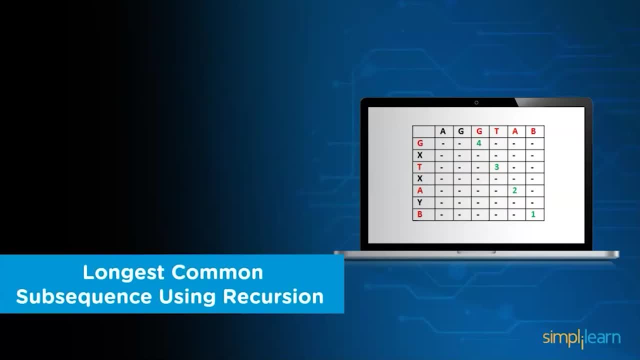 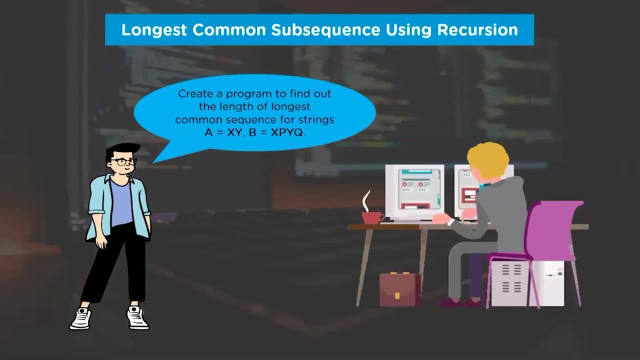 of us can get this right Now. moving forward, we'll build a solution for LCS using recursion. So let's visit the code editor and develop the C program for longest common subsequence. The two strings for which we are going to find LCS are xy and xpyq. Let's create a function. 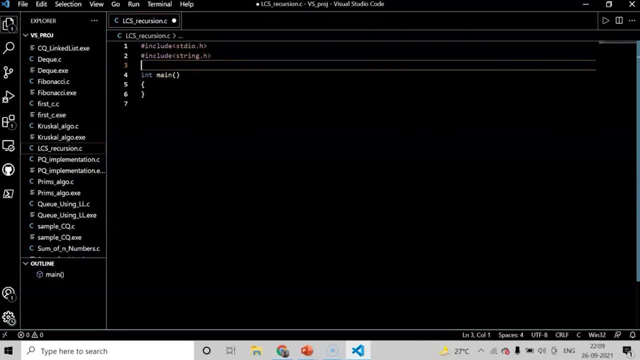 to get started with LCS implementation, I'm going to name this function as int lcs and inside this function will pass the references of two character arrays. The first will be char star a, comma. char star b. The next arguments will be the links of these character arrays: int x and int y. Now we'll move to the function. 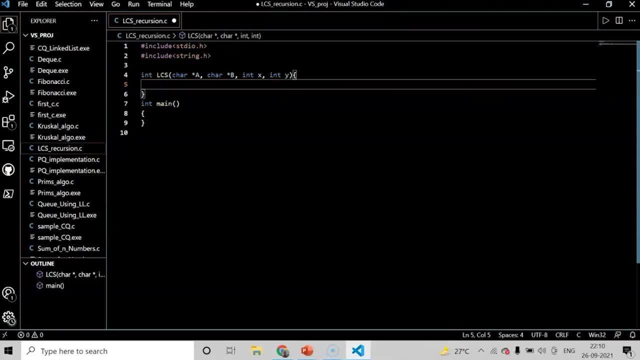 body of LCS. The first condition we'll evaluate is if the character array are empty or not, Because if character arrays are empty, then definitely there won't be any sequence to find out. So when we reach x equal to zero and y is equal to zero, we'll return zero. 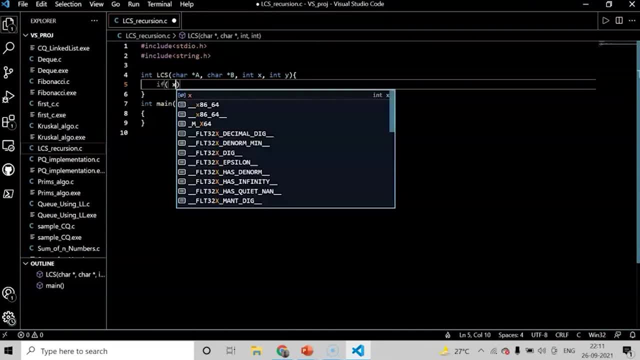 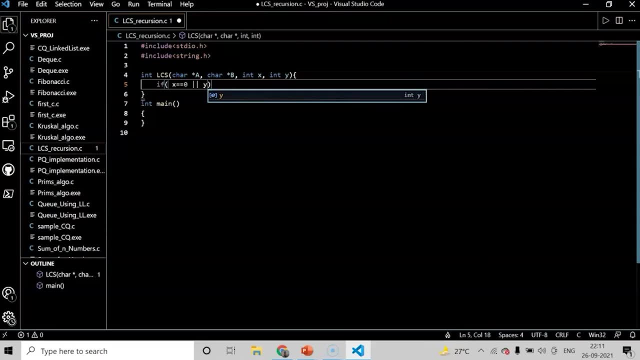 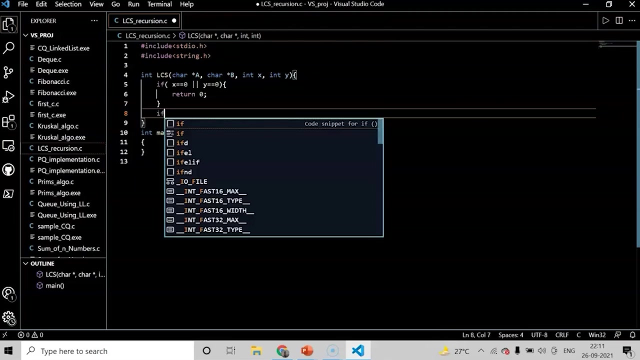 For that we'll write a condition if int x and int y are empty. Now the next condition: when both x and y won't be zero, we'll check if the last character of both character arrays match or not. For that we'll write another if condition. 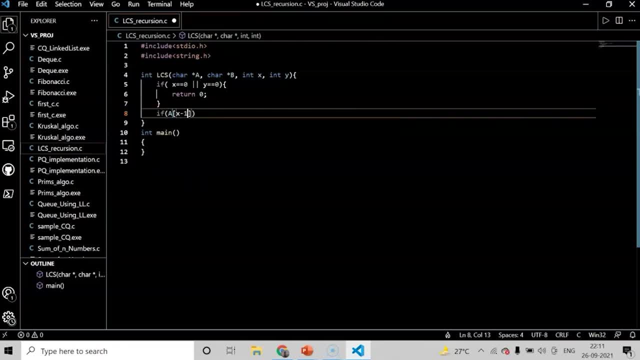 If a x minus 1 equal to equal to b x minus 1, then we'll return 1 plus lcs. a comma b comma x minus 1.. For this the first condition will be If b is equal to b y comma y minus 1.. 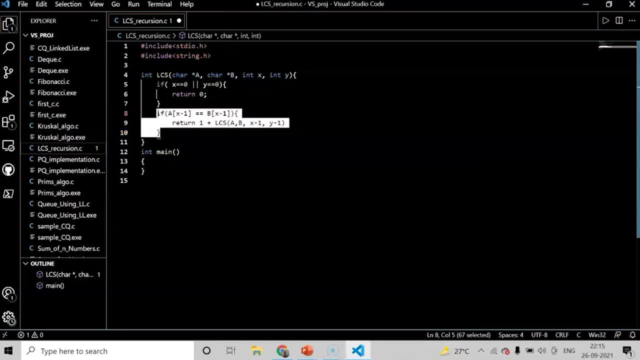 Now let's look at the second condition. If b is equal to b x minus 1, then we'll return 1 plus lcs a comma y minus 1.. Once this condition gets fulfilled, we'll return 1 plus recursive call to lcs function with: 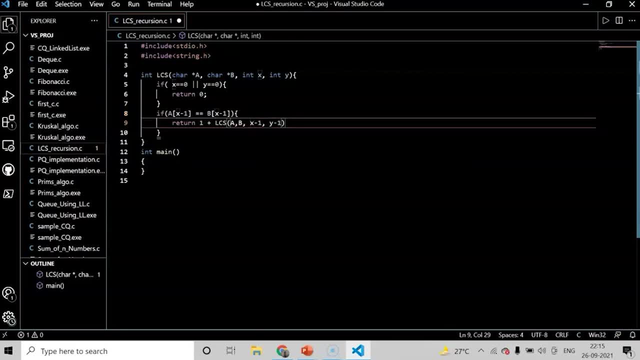 inputs decrease in size by 1. That is x minus 1 and y minus 1.. Now, if both the previous conditions fail, then what we'll do is go into this else part and inside this else part we'll return And 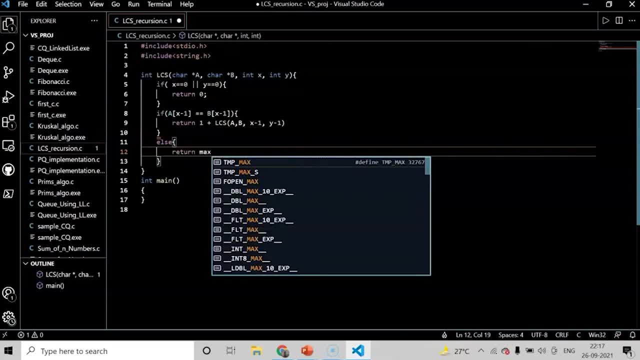 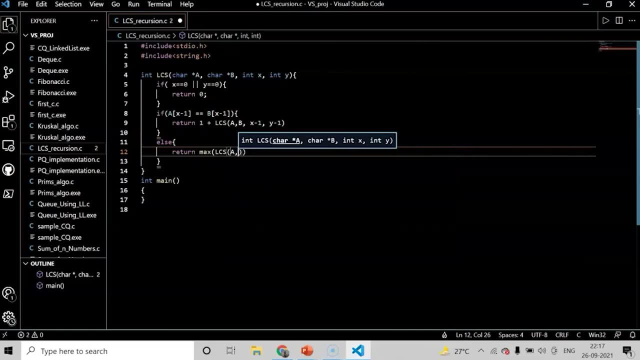 Run This MAX of LCS or LCS and dot here Now. this statement will get executed when there is no character match. If characters don't match, we'll move either way: one character in 1st string A or one character in 2nd string B. 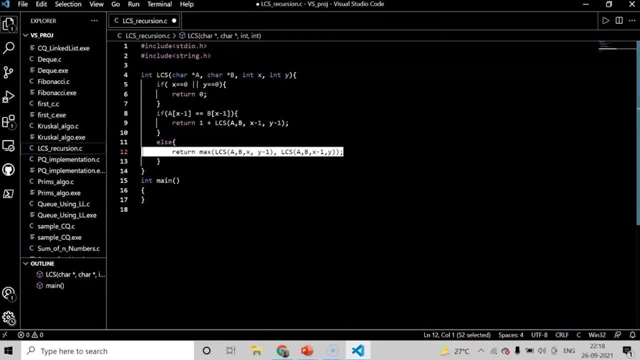 And check whichever gives maximum, and we will take that into consideration. Most of the time this condition will get satisfied. To find out the maximum we will have to create a manual maximum function. so for that we will create a new function that is int max and we will pass arguments: int m, comma, int n. 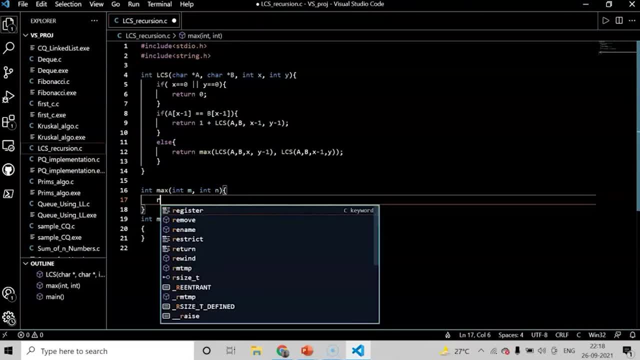 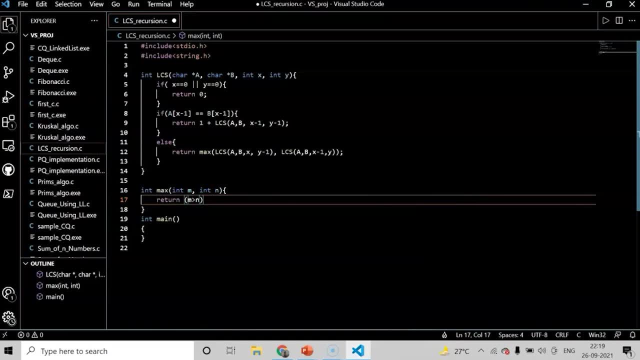 Now, inside this function, we will write a ternary condition that is return m greater than n question mark, m colon, n semicolon. So this will return the maximum value between m or n. With this we have successfully completed the LCS function. So moving forward, let's. 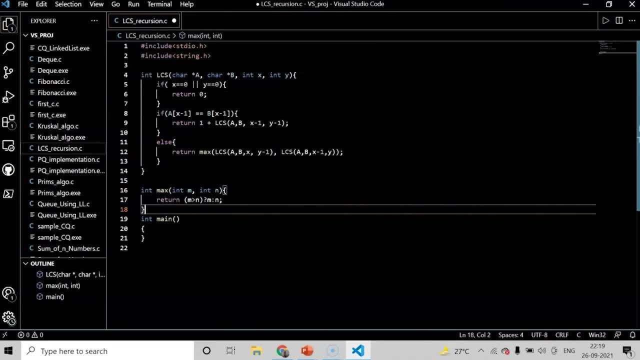 work on our driver function. In driver function what we will do is we will create two character arrays at first. So for that let's enter into this main function And we will create character array A and inside A we will pass x and y. 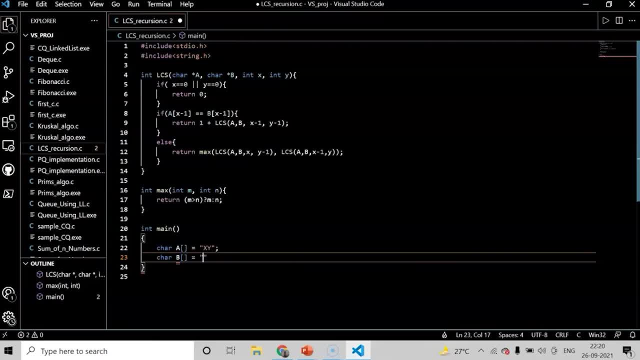 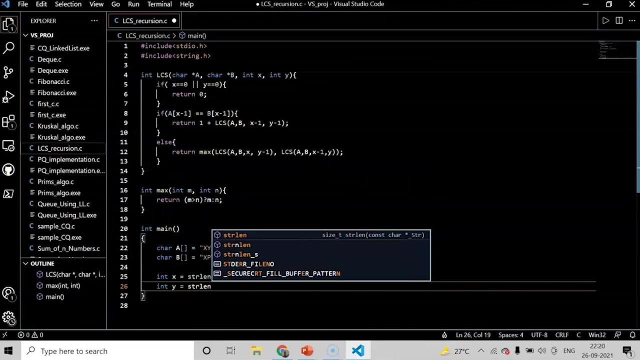 Inside character array B, we will pass x and y. Inside character array B, we will pass x and y, P, Y, Q, okay, and will store the lengths of these character arrays into X and Y. for int X is equal to STR len a and for int Y STR len B. let's semicolons here, and: 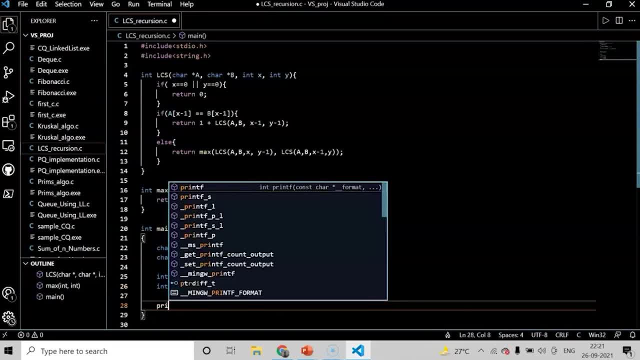 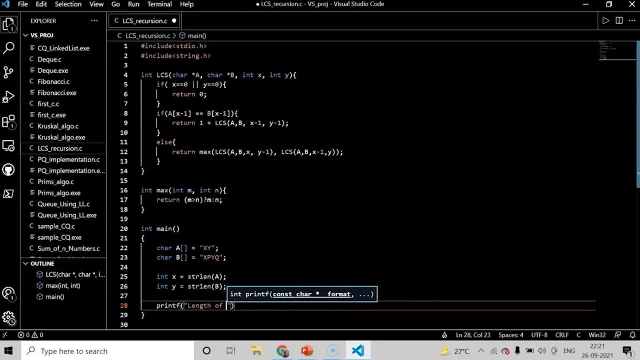 finally, we will make call to our LCS function using the printf statement. the printf statement that will write its length of LCS is modulus D comma LCS, a comma, B comma, X comma, Y semicolon. and finally we'll add return, return, return zero. I hope our code is bug-free now, so let's run it and check if it is bug-free. 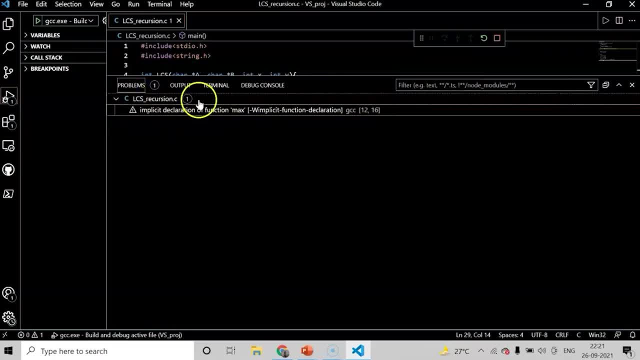 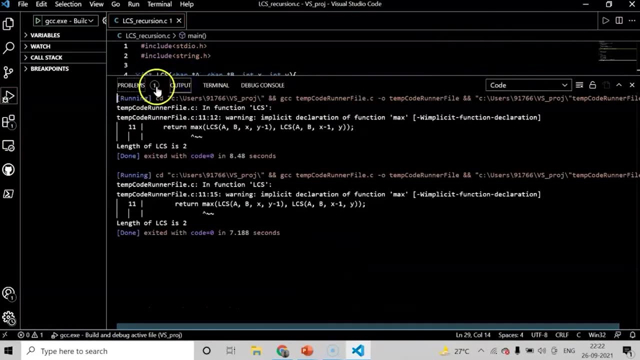 that's fine. here we are getting error, but it is not exactly an error. we have implicitly declared function max here, so that's why we are getting this flag problem. but we are actually getting output as well. so the output that we are getting is two here, and if you check both the strings, then 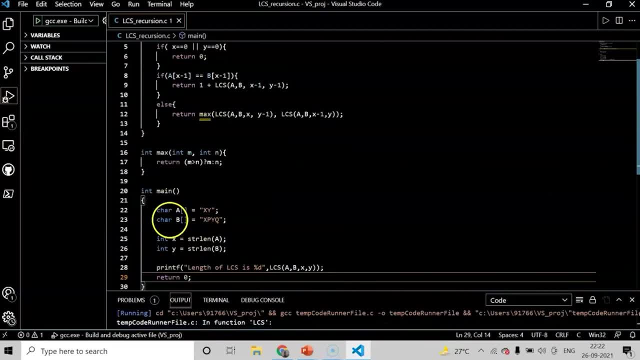 you can find out that character array a: it's implemented inside character array B, and the length of common sequence it's two here. so with this we can say that a recursive implementation of LCS is successful. so now moving forward, we'll visit PowerPoint to understand why recursion is not an ideal. 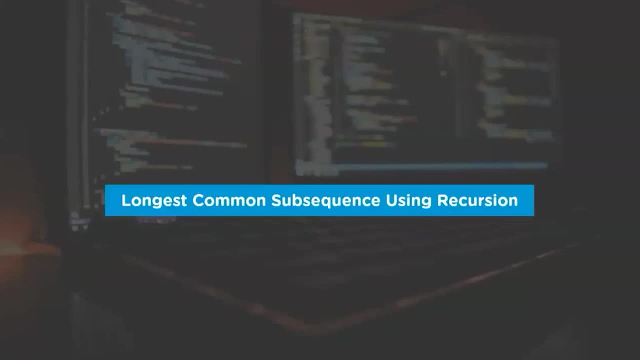 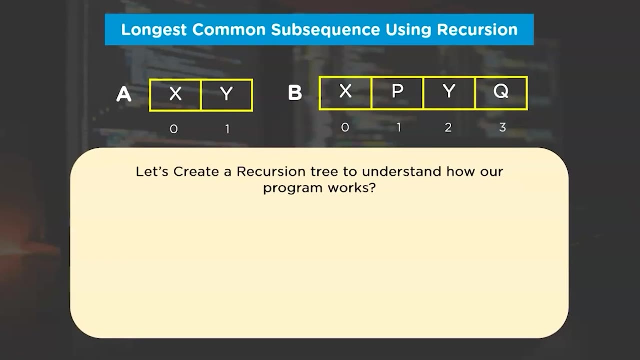 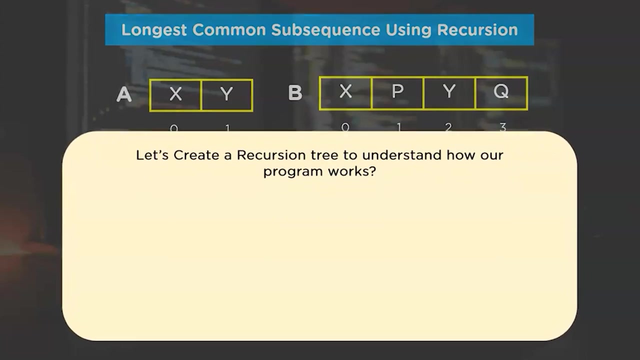 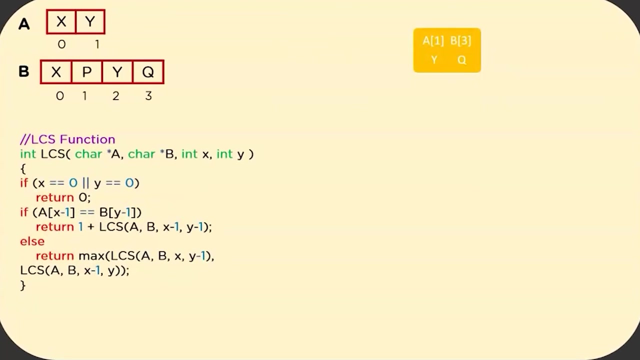 approach to solve this problem. to understand the complexities associated with longest common subsequence problem implementation using recursion, we'll formulate a recursive tree by going through the steps of a program that we have created previously. so let's do that here. as you can see, in this LCS function, the function is not the same as the previous one, so we 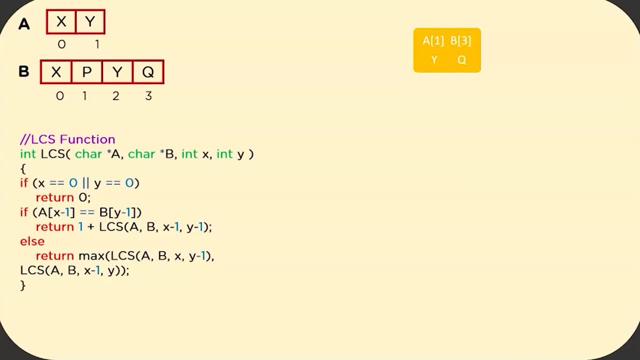 the first step. we perform it checking if both the strings are empty. if they are not empty, then we check if the last character of both strings matches or not. thus, the first call to the LCS function will check for the match of last two characters. if characters don't match, which is true in this scenario, we move. 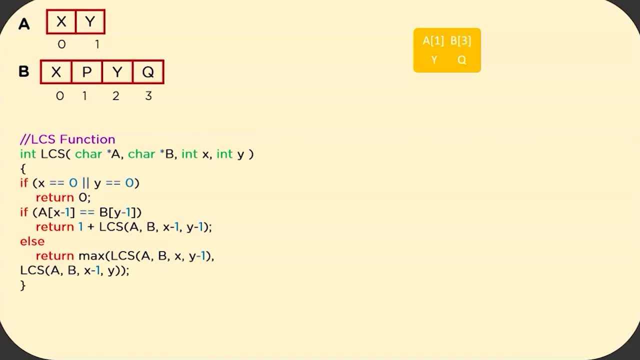 either one character in string a or in second string B and will choose whichever produces maximum value. so if we reduce B by one, 1 and keep the a same, then we have a character y in both the strings, Whereas if we keep b the same and reduce a by 1, then we have x and q which don't match with each other. 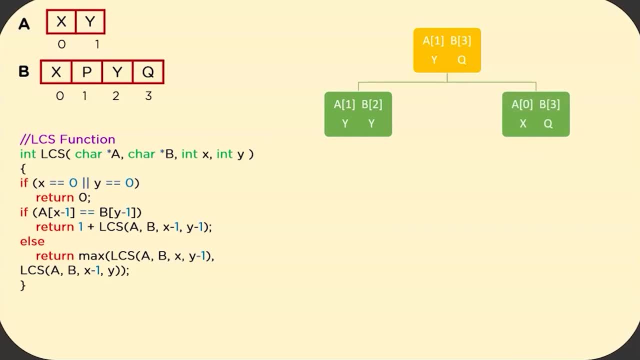 First we will evaluate the left side of our recursion tree and here we have a character match. thus we will enter if condition where characters do match. that is this condition and it says that return 1 plus both the character arrays with size reduced by 1 by doing that. 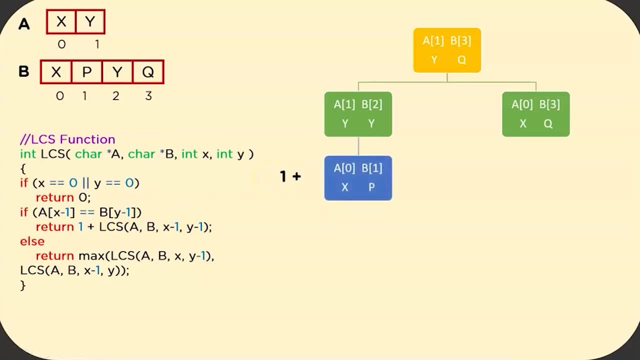 we get 2 different characters, x and p, here. Now, as these characters do not match, we will move position by 1 in both the strings. by doing that we get these results and here, if we observe, the left child has a character match. thus we will add 1 and reduce the size of both character arrays by 1, and with this 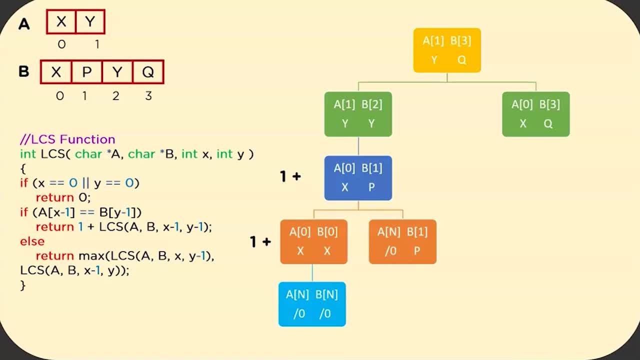 step we reach the end of ouroque strings. Now let's work on the right side of our recursion tree. In this case we have distinct characters. thus we'll move by 1 in both the character arrays and the resultant. 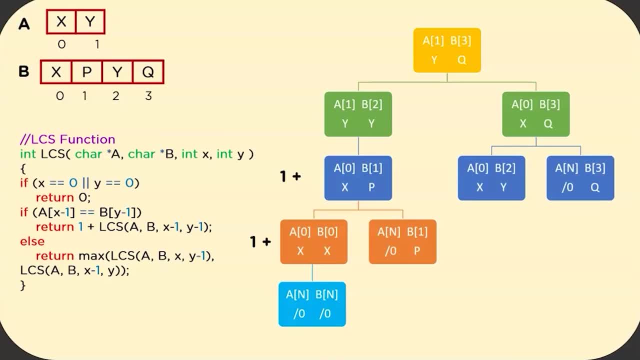 child nodes don't have characters that match. Furthermore, the right child reaches the null index. hence now we will just expand the left child. In addition to that, we can move positions only in character array B, as we have reached the end of character array A For this move. 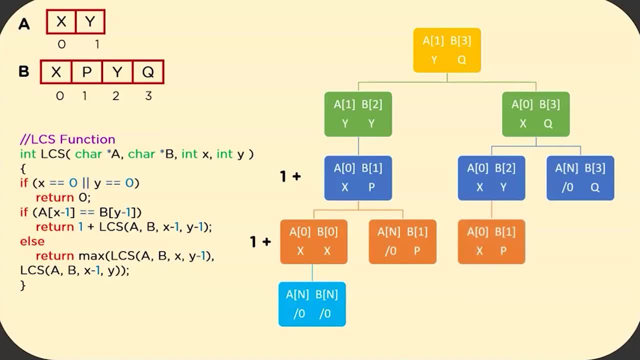 we do not have any match, so we'll reduce the position of B by 1 again, And here we get a match and also reach the end of both character arrays. Now the next step will be for evaluating LCS length by backtracking our recursive tree. 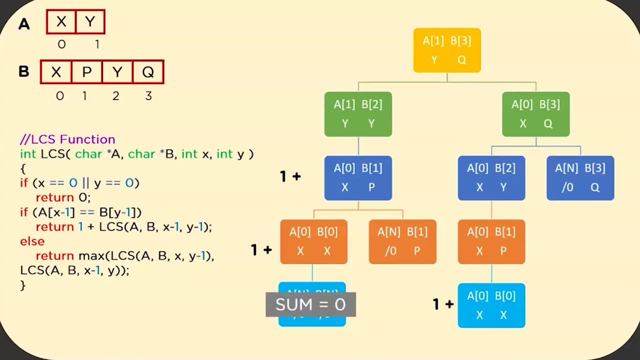 First we'll consider the left side. so let's begin from the bottom of left side. At the bottom, most child, we have some value equal to 0.. For the next step, we'll have some value 1.. And we'll add 1 here. For the next step as well, we'll have to add 1 to our sum value. 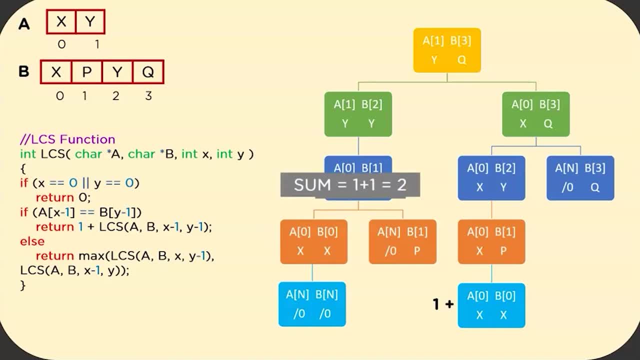 thus the sum value will become 2 here And the overall sum for the left side of recursive tree will result into 2.. Whereas for right side the sum will become 1,. as there is only one match Now, this side, which has maximum sum value, will be returned as a result of. 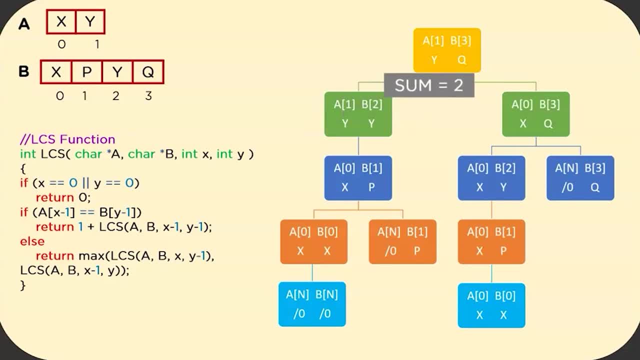 this LCS program, Which will be 2. in this case, The complexity for this recursive LCS program will be 2 to the power n. Now for these two strings which have small length, you can see that the complexity will be equal to 2 to. 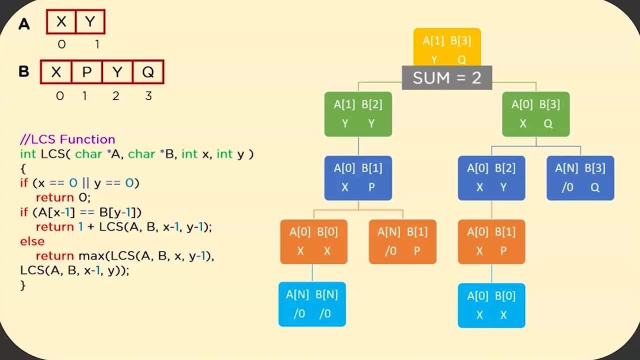 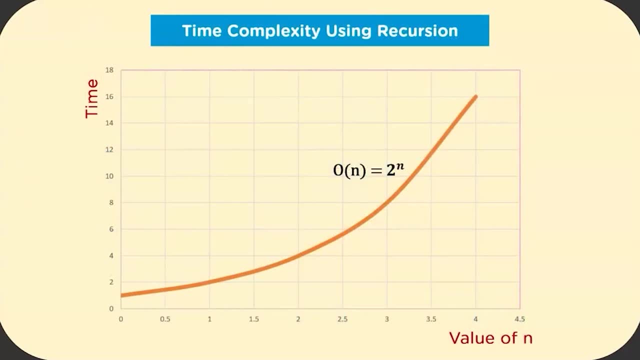 the power n, where n belongs to the depth of binary tree. That is huge complexity. If you look at the complexity graph, you'll get that. you'll get parabolic graph which will increase continuously or exponentially. However, this problem can be resolved by using dynamic programming, paradigm Moving. 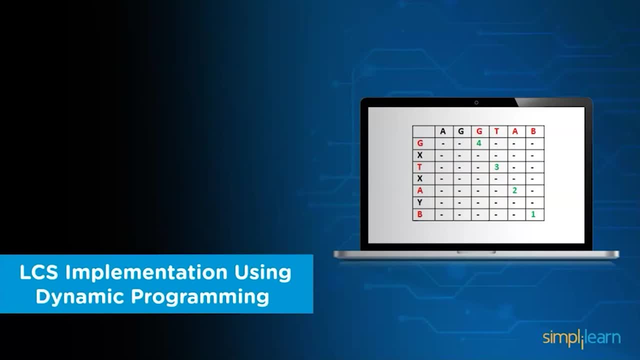 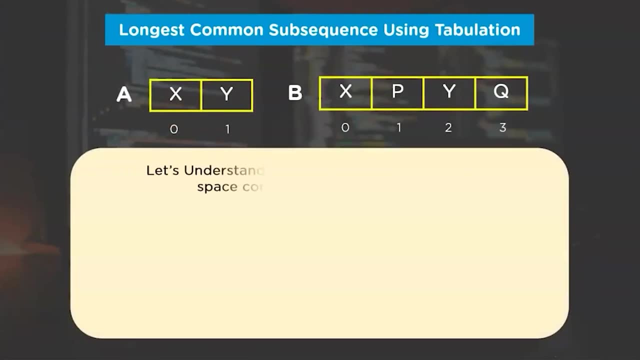 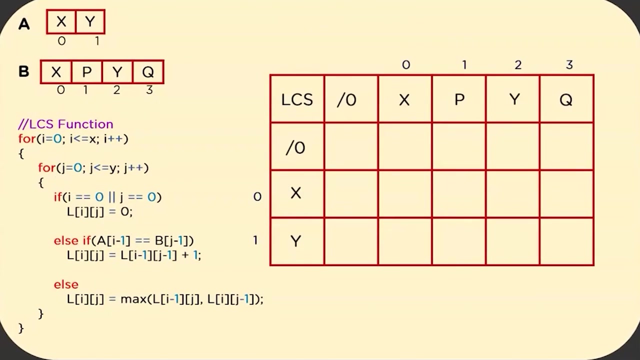 further we'll try to analyze how dynamic programming can reduce the computational complexity of LCS problem. Here we'll try to solve LCS problem using the tabulation method in order to understand how tabulation can reduce space complexity by making fewer computations. The LCS function for tabulation will be iterative, Hence we'll understand the computation with. 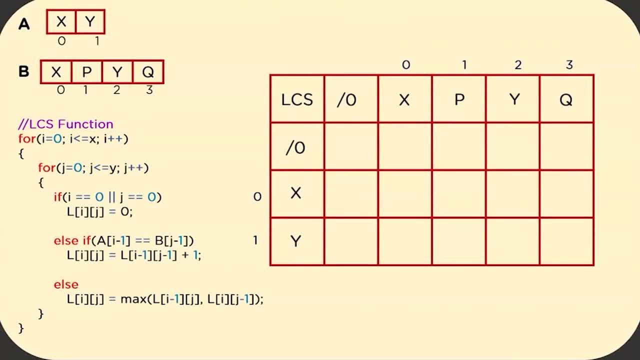 help of tabular representation. The columns will represent character array B and rows will represent character array A. Furthermore, we have added the null values to the table. Hence, initially, we will set the field values for null row and columns as 0.. Now here we. 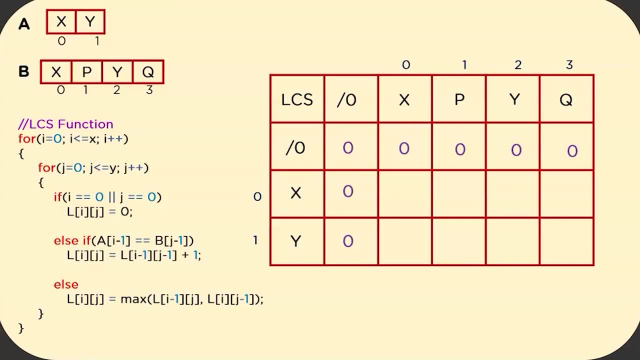 will move through the row of character x. For the first iteration we hit the match Hence we will add 1 to the diagonal element, So 0 plus 1 will become 1.. For the next iteration, we get x and p which do not match Hence we will continue with 1.. Next we have x and 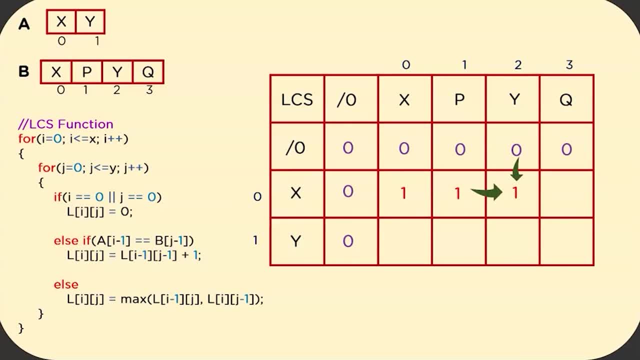 y, which also do not match. Hence we will continue with 1.. Remember guys, the highest value between these two fields will be picked every time. For the next move, the value 1 will continue. Now, moving forward, we will move towards the y row Here for both x and. 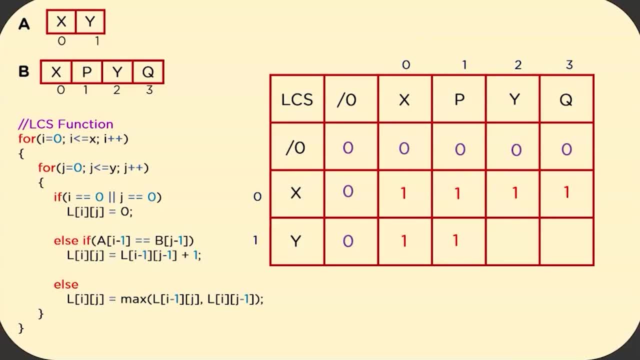 p, the values will remain 1, as we don't have the character match. But for the next field we will have a match, Hence we will add 1 to the diagonal field. The value for this particular field will become 2. now For the last field, the value 2 will get continued. 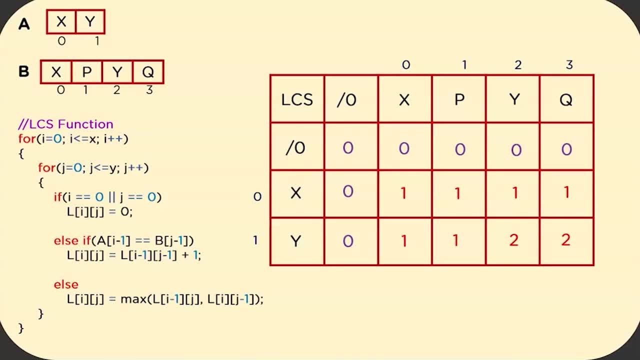 as it is the highest field than another comparative field, And you can see that we have found the accurate result here. I hope this tabulation logic is clear to all of you. Cause, moving forward, we will develop a C program for the same. 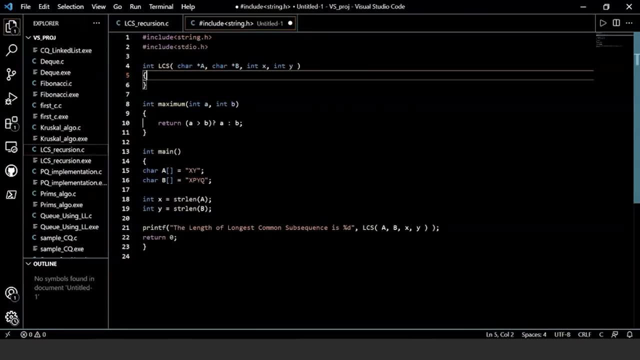 Now, in order to get started with this tabulation function, we have created intLCS function with few arguments. These arguments are similar to the recursion In this tabulation. LCS function will first create the 2D matrix for performing the computation. The statement: 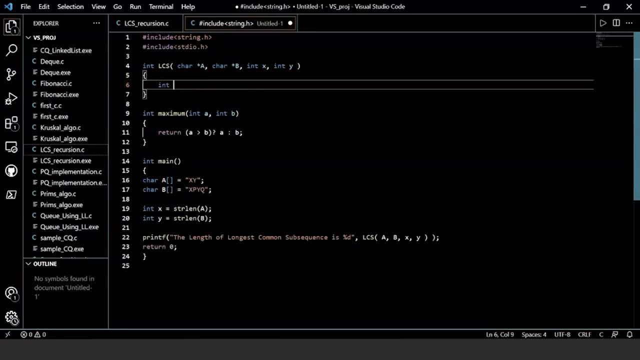 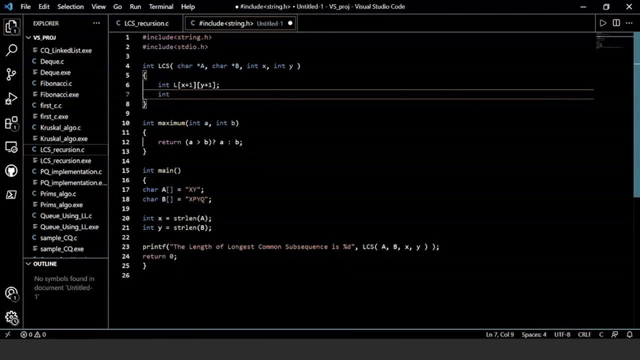 that will help to do that is int, L, x plus 1, x plus 1 and y plus 1.. So this will create a 2D matrix of size x and y. We will also initialize few variables for using them inside looping process, So I will 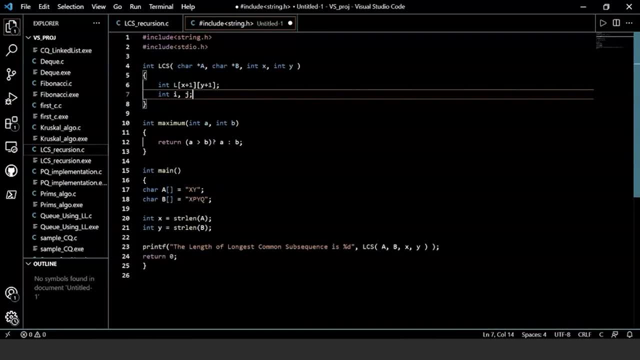 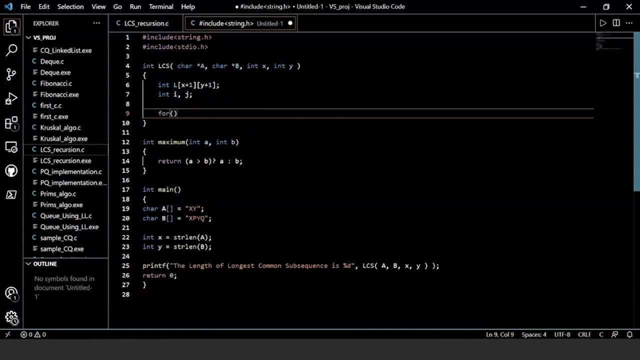 create two variables: int, i and j. Next, we will create a nested loops for traversing through both arrays at the same time and updating the computational table. For that we will create a for loop and inside this for loop we will begin from i is equal to 0 to i is greater than equal to x, and we will increment. 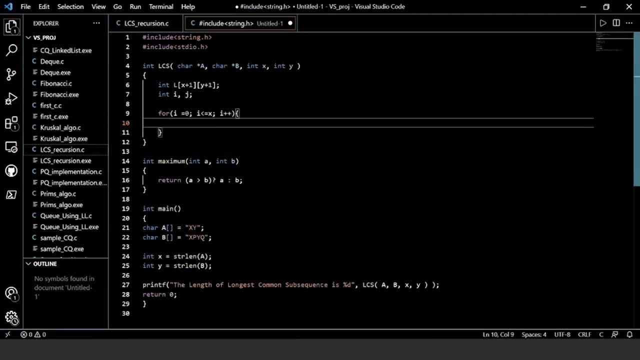 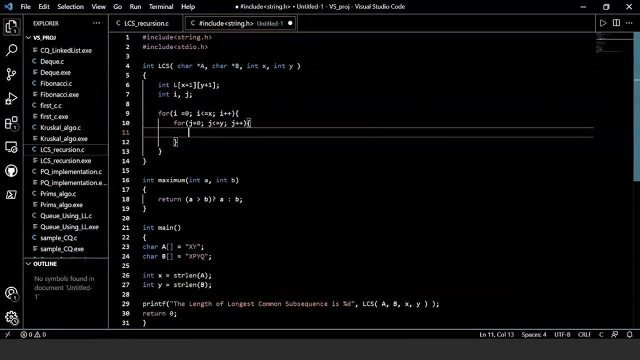 the i And insert this for. We will create another for loop and we will begin this with: j is equal to 0, to j less than or equal to y and j plus plus. After that we will write the first condition to set null values for the null row and column fields. 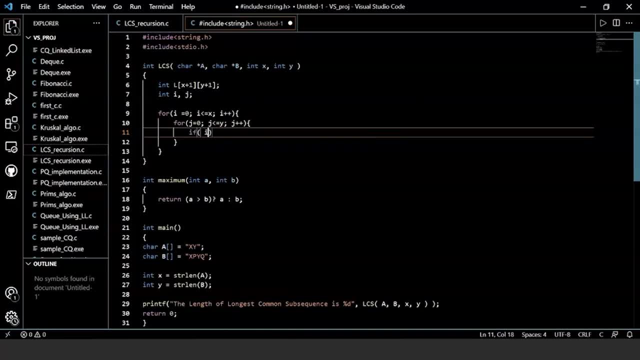 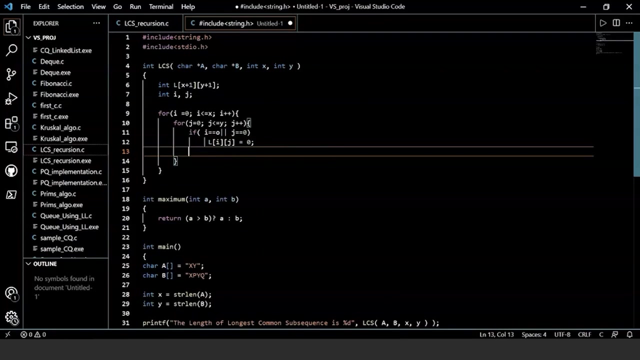 So the statement that we will write is: if i is equal to equal to 0 or j is equal to equal to 0. Then Set l i j equal to 0. If this condition fails, then we will check if the last character match with one another. 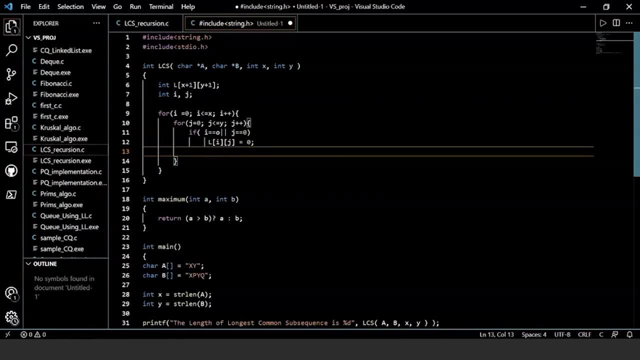 If they match, then we will return 1 plus both array fields reduced by position 1.. For that we will write condition. else, if a- i minus 1 equal to equal to b, j minus 1 and insert this, else if condition, We will set l: i. 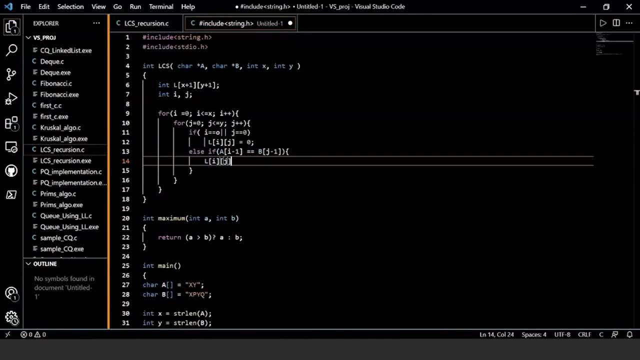 j is equal to l? i minus 1, j minus 1 plus 1, and if this condition fails, then we will enter into else loop And we will pick l i j as maximum of l i minus large l, and here as well it should be large l. 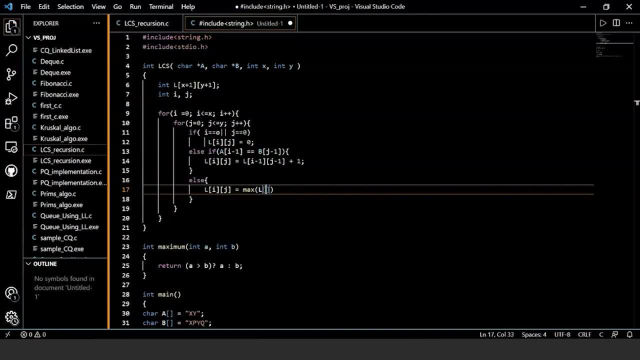 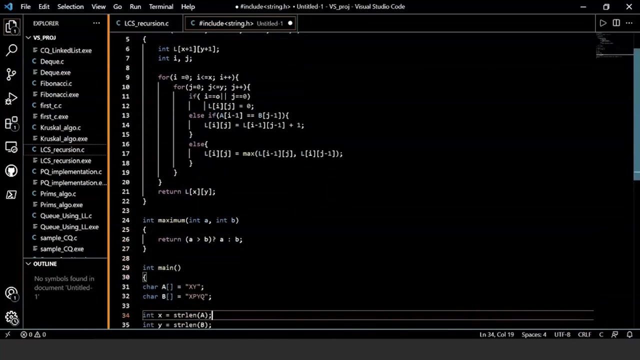 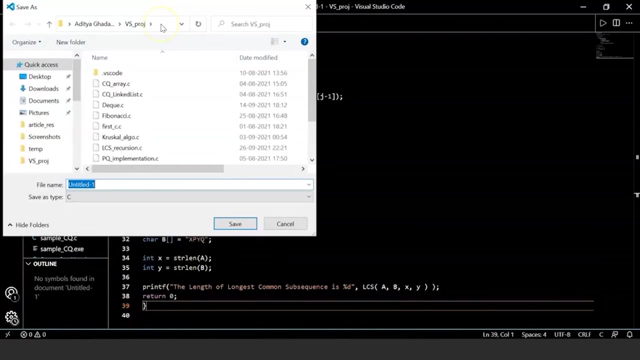 l i minus 1 j comma. l i j minus 1.. And we will get out of these four loops And We will return the output, that is, l, x and y. I hope this should be fine now. So let's run our code and check if there is something wrong. 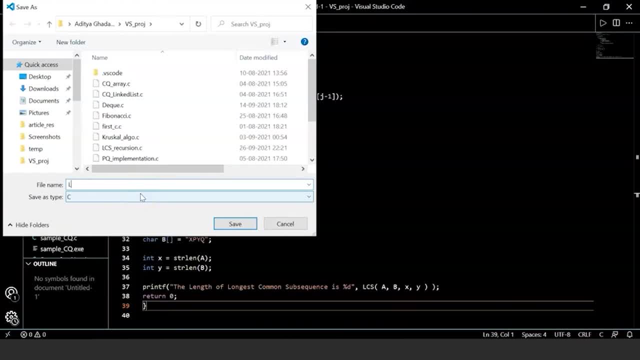 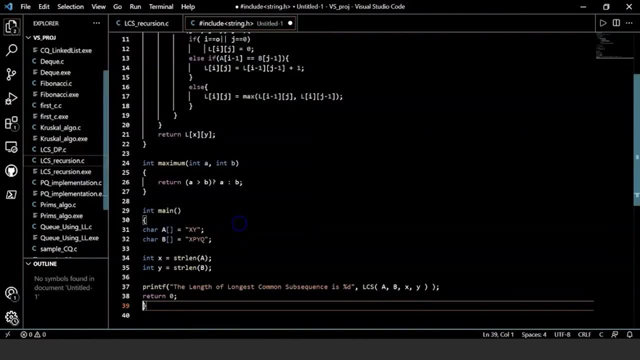 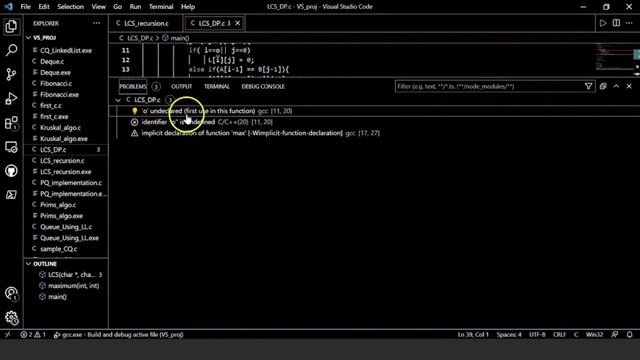 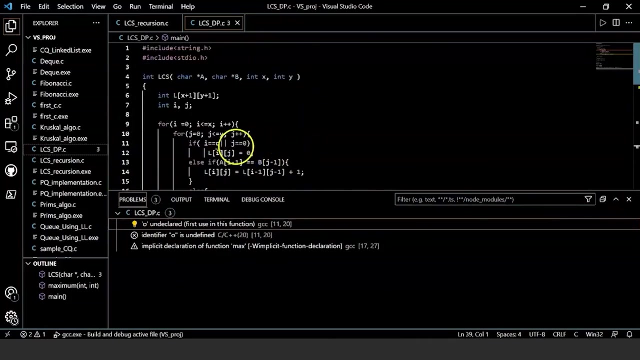 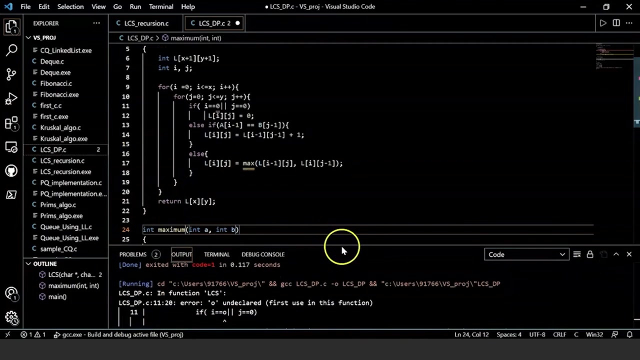 We will save this As Lcs Underscore DP. So we are getting three problems here. Okay, So I have inserted o here, Yep, m, m, m, m, zero. and there is one more mistake, so I have called function max as max here, and 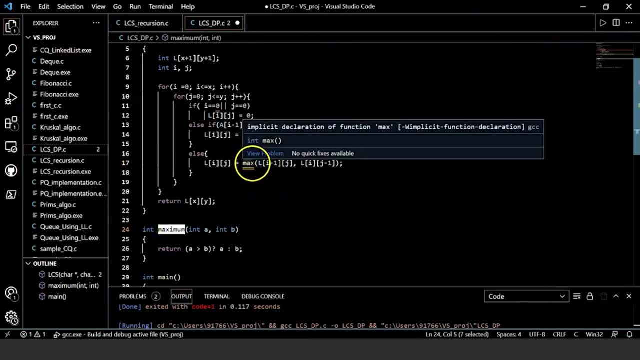 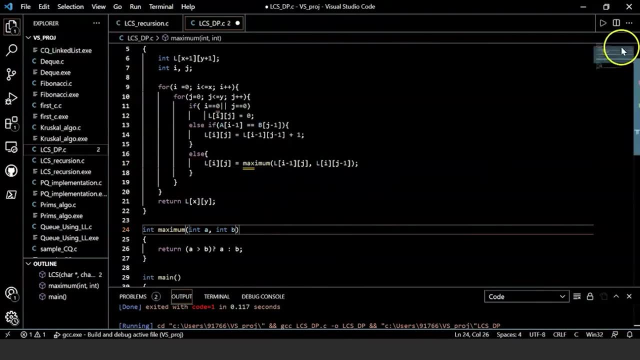 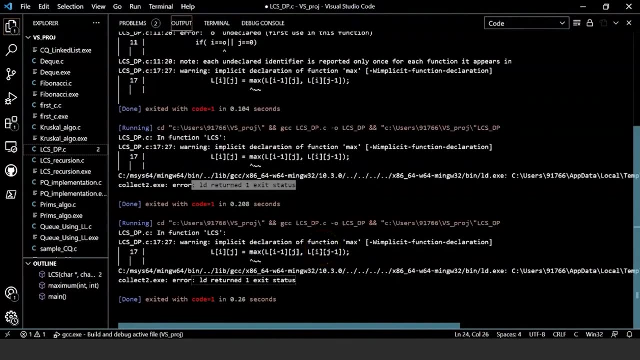 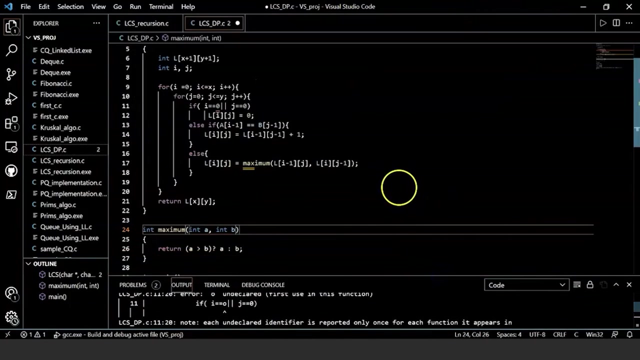 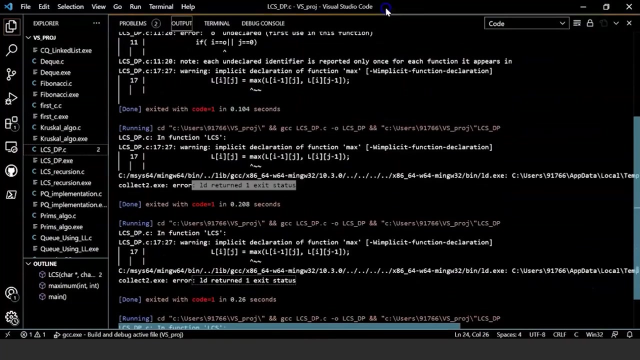 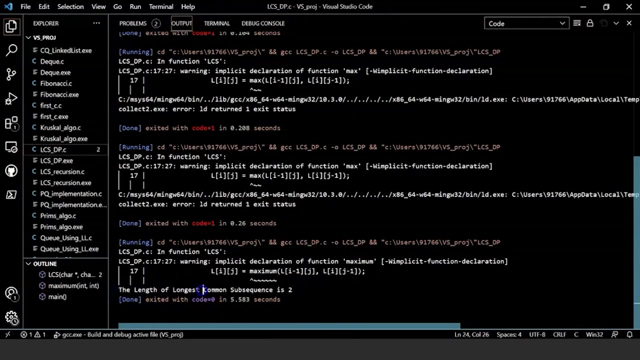 have named it as maximum here, so we'll have to change this to maximum. I think this should be fine now, so let's run our code again. okay, we'll have to save this, so we'll press ctrl s and we'll rerun it. yeah, so we are getting our output here. the length of longest common subsequence is: 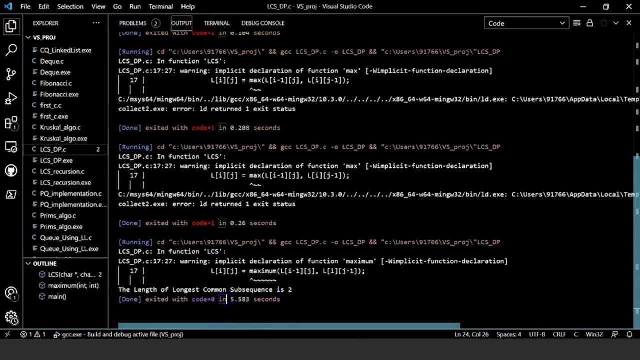 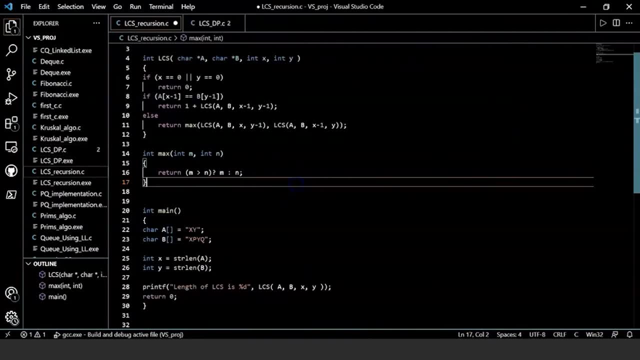 2. so if you observe here the output that we have got using dynamic programming, as in 5, 5, 5.58 second and the time that was taken for LCS recursion was around 8 seconds, so you can see that the complexity has been reduced, the time complexity and 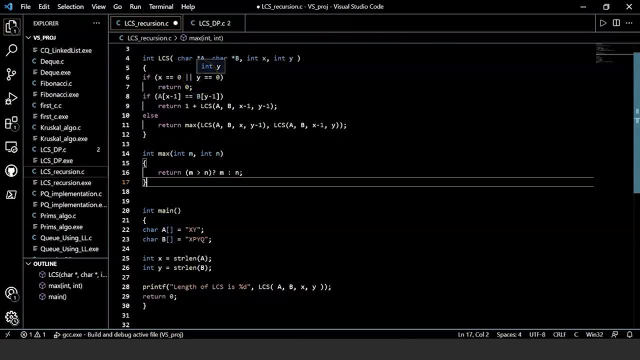 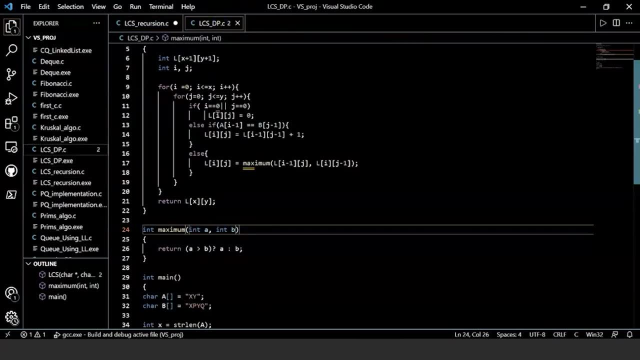 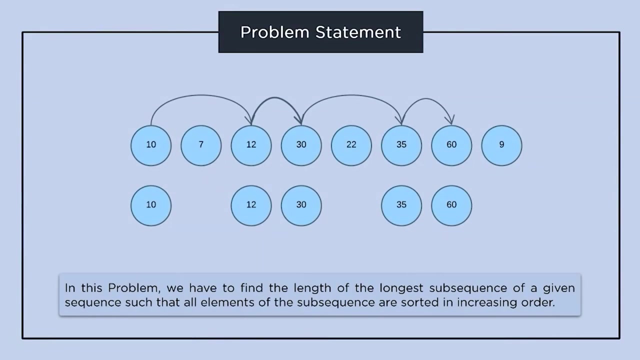 space complexity as well. so that is why the dynamic programming is better approach than recursive programming paradigm. I hope the longest common subsequence problem- implementation using dynamic programming- is clear to all of you out there. in this problem we have to find the length of the longest subsequence of a given sequence. 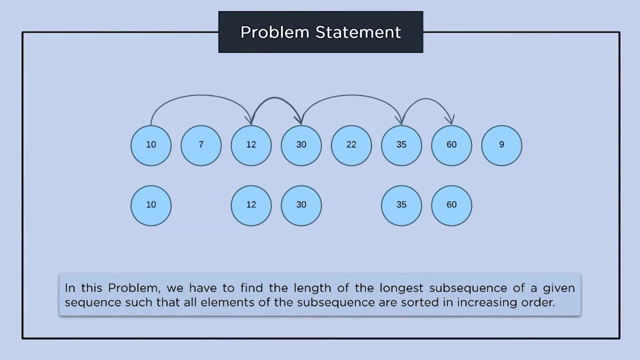 such that all elements of the subsequence are sorted in the increasing order. for example, as you can see in the picture, the length of the longest increasing subsequence for the set is 5 and the longest increasing subsequence is 10,, 12,, 30,, 35 and 60. 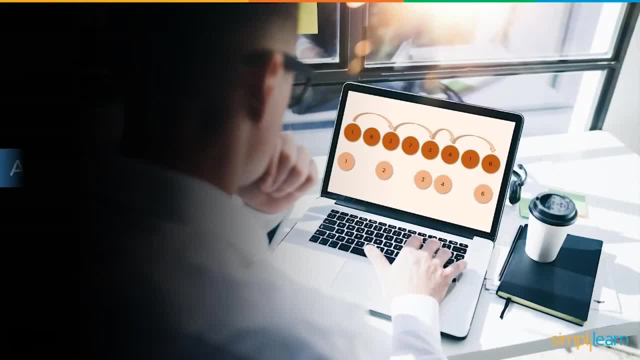 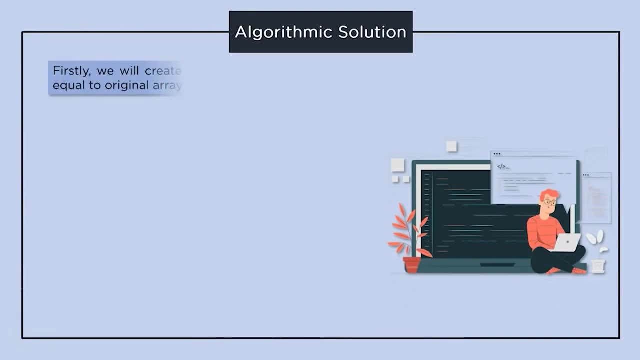 now lets discuss the algorithmic solutions. solution to the longest increasing subsequence. First we will create another array of the same size as the original array with element as 1.. Then we will discuss the nested loop and compare the value of array elements. If value comes out to be increasing order, then 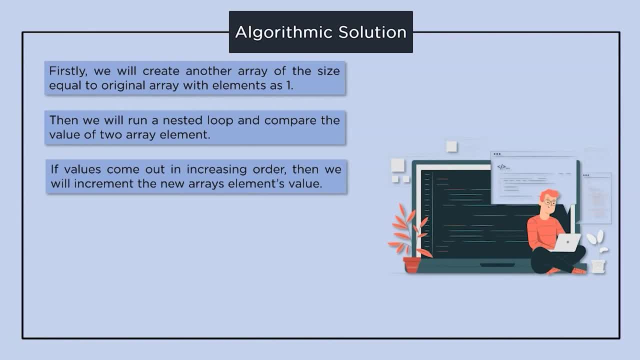 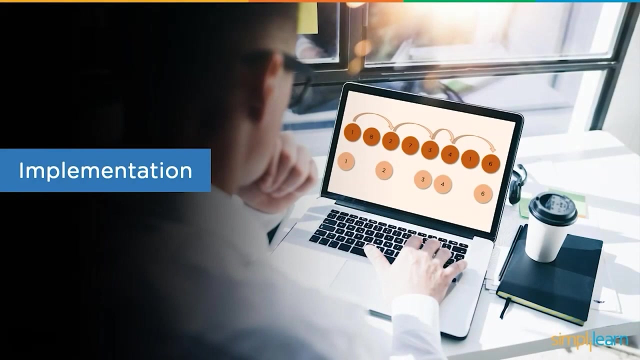 we will increment the corresponding new array elements value. Now we will repeat this for the every possible set until every set is exhausted. Now the Maximum element in the new array will be considered as the length of the R longest increasing subsequence. We have now discussed the problem statement and the algorithmic solution to the longest. 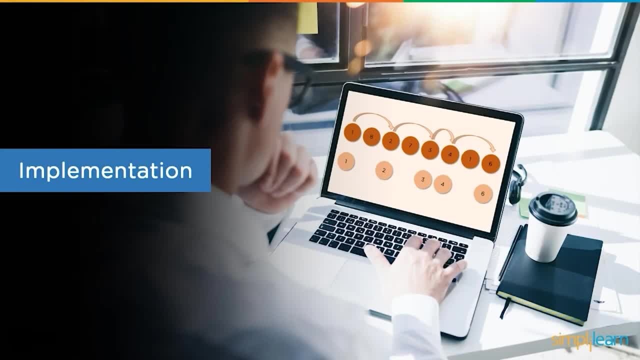 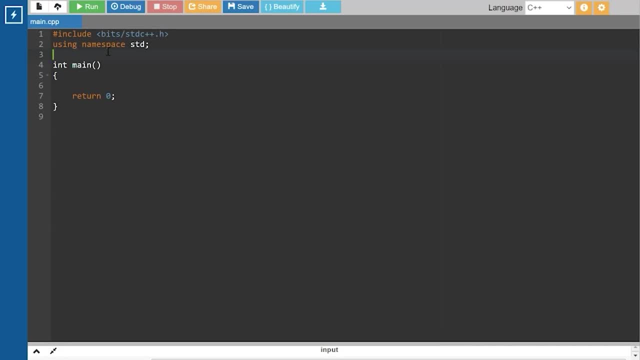 increasing subsequence problem. Now let's implement this solution in the code editor. we will start with a function that will return the length of the longest increasing subsequence in the procedure, the array ARR of size n, So int lis argument will be int array ARR comma, int n. 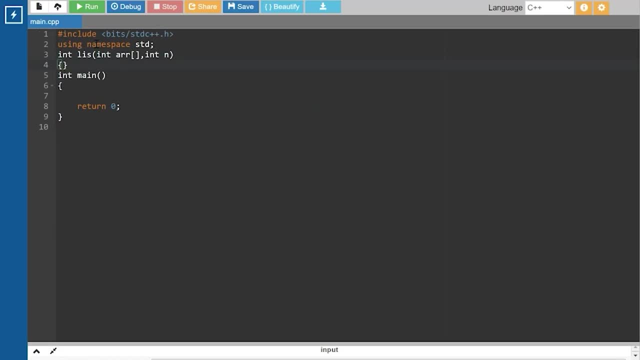 We will declare int, lis n. Now lis at 0 will be equals to 1.. Now we will compute the optimized lis values in the bottom-up manner. so for int i is equals to 0, i less than n, i plus plus. 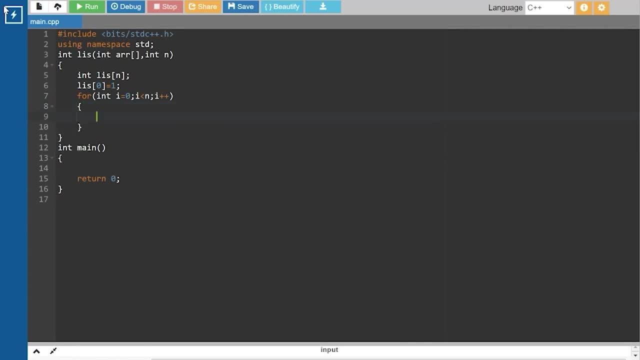 Now we will give lis at every i-th position is equals to 1.. Now we will insert another for loop inside as a nested manner. so for loop int j is equals to 0.. 0, j less than i, j++. Now if ARR at i is greater than ARR at j, 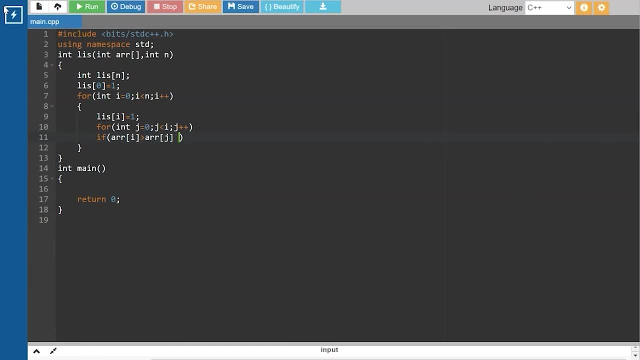 and less at i is less than less at j plus 1, then we will update: less value at i is equals to less value at j plus 1.. After that we will return the maximum value of less, so return star max underscore. 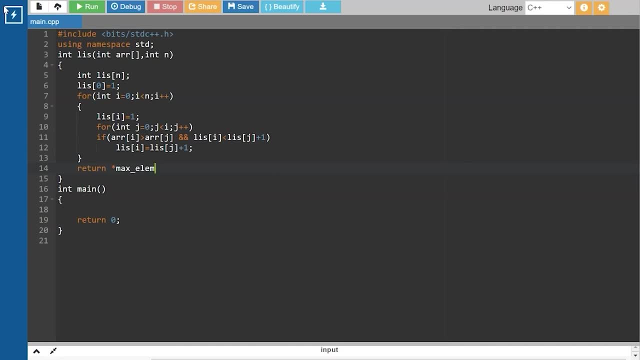 elements: less comma, less plus 1, plus N. Now we will write the main block. we will declare int The array, its elements as: 10, comma 7, comma 12, comma 30, comma 22, comma 35,. 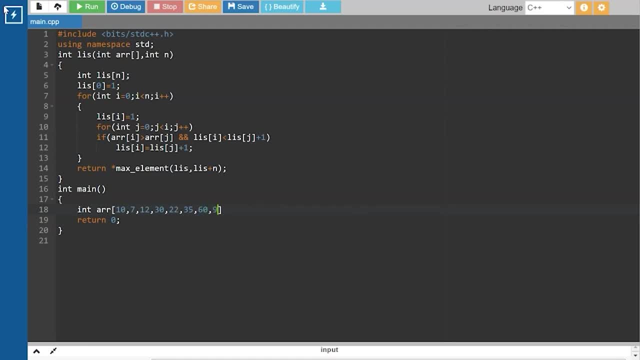 comma 60,, comma 9.. Then we will find the size of this array. so int N is equals to size of ARR divided by size of at ARR at zeroth location. Now we will print cout. 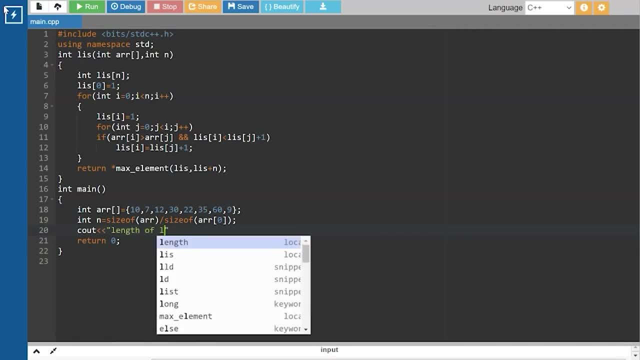 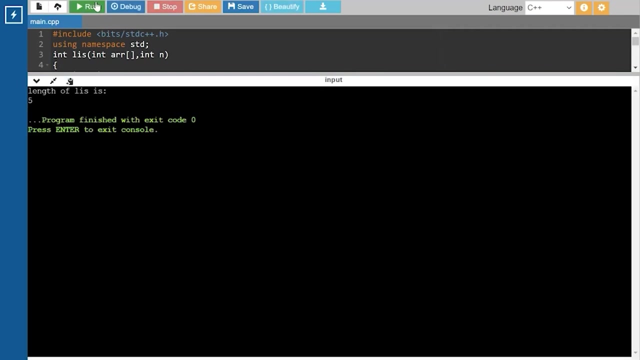 cout List clarified. our loop call is basically hitting the possible n. Let's execute this. As you can see, we are getting the length as 5, just like we. 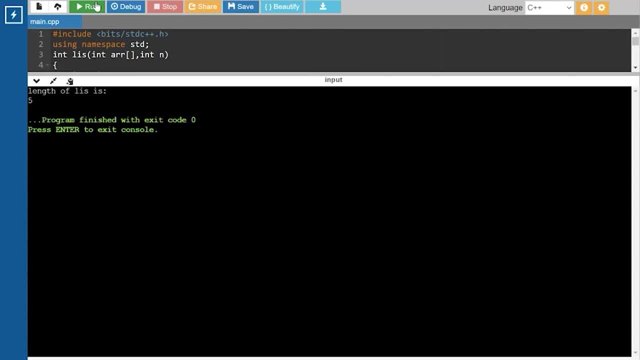 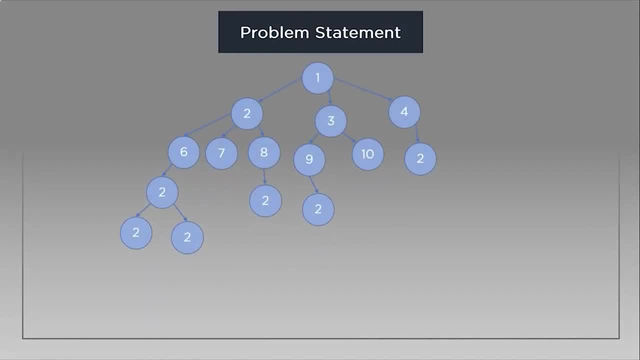 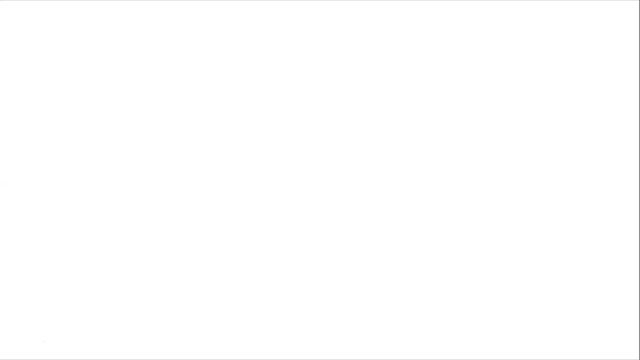 have discussed during the algorithmic solution. Let's get started with the problem statement. We will be given a set of non-negative integers and a value of variable sum, and we must determine if there is a subset of given set with a sum equal to a given sum. 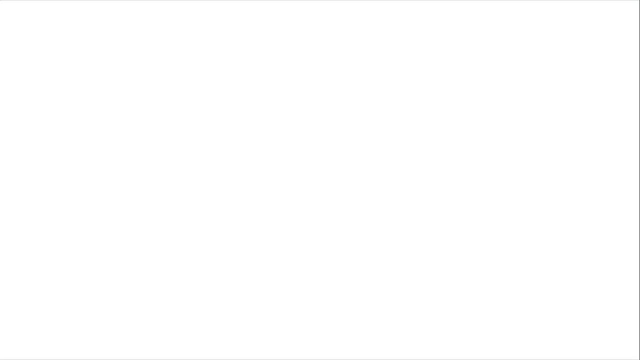 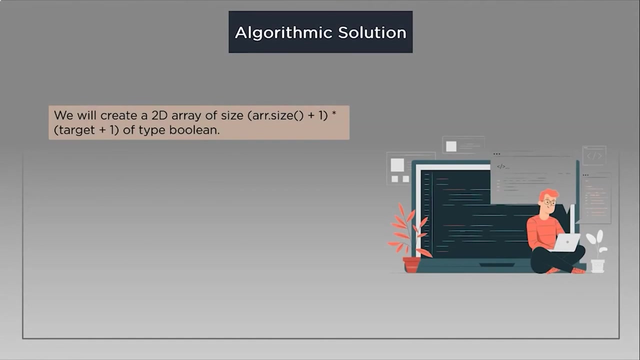 Now let's discuss the algorithmic solution to the subset sum problem. First, we will create a 2D array of size, ARR size plus 1, multiplied by target plus 1 for the type boolean. Next, the state dp will be true if there exists a subset of elements from a, from 0 to i, with 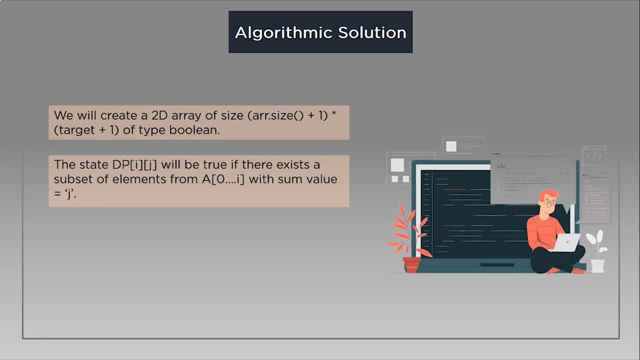 a sum value equal to j. Let's look at the pseudo code Here. if the current element has a value greater than the current sum value, we will copy the answer for previous cases And suppose the current sum value is greater than i-th element. in that case we will see. 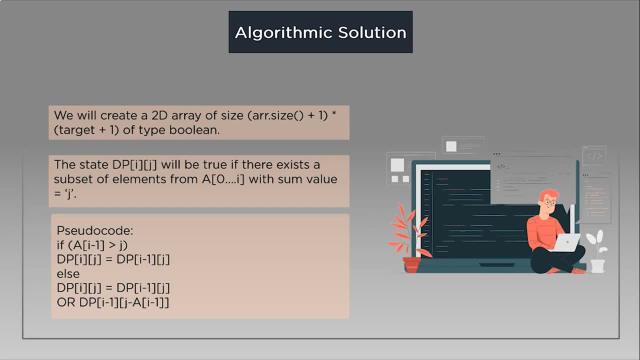 if any of the previous elements are greater than the current sum value. Now let's see if any of the previous states have already experienced the sum equals to j, or any previous states experience the value j minus a at the i value, which solves our purpose. 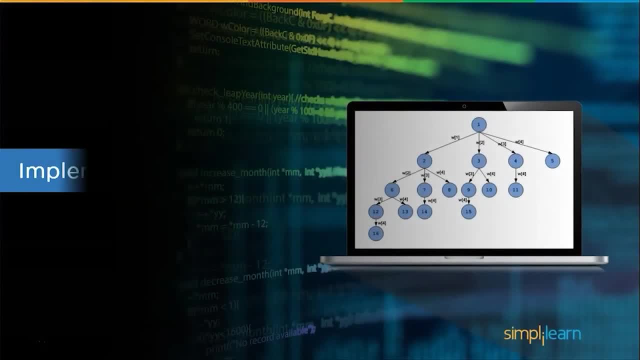 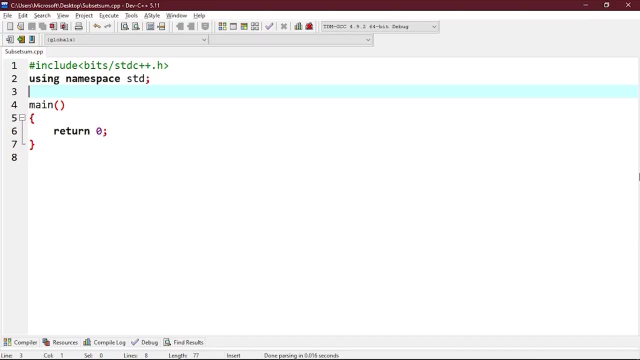 We have now discussed problem statement and algorithmic solution to subset sum problem. Now let's implement this solution in the code editor. We will start with the boolean function isSubsetSum, which will return true if there is a subset of set. The project will return true if the set is not equal to the given sum. 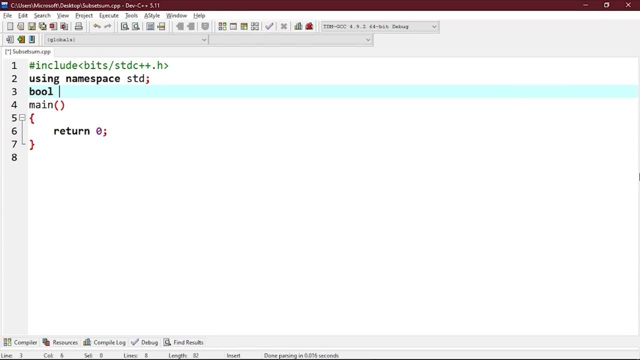 So boolean isSubsetSum and int arr, int, n, int sum, and if there is no subset of sets in the code editor, then it will return 0.. Now the problem statement will be true and we will not be able to solve this problem. 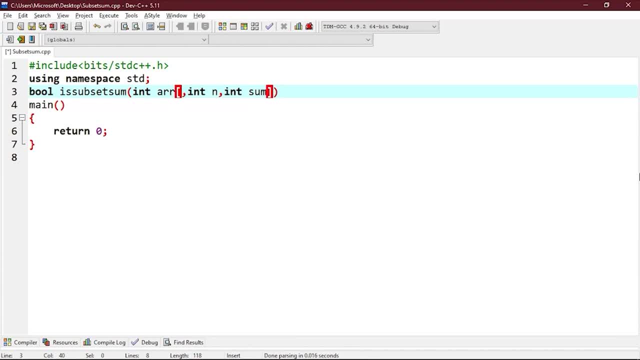 problem. Now, the value of the subset ij will be true if there is a subset of set from 0 to j-1 with sum equal to i. So bool subset n plus 1 to sum plus 1.. Now, if sum is equal to 0, then the answer will be true. 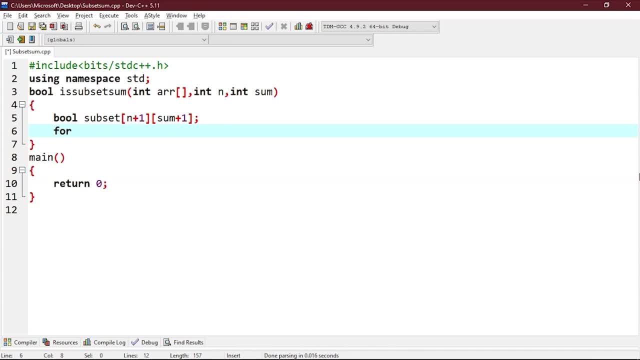 So 4 and i equals to 0, i less than equals to n. i plus plus subset at i comma 0.. Now, if sum is not 0 and set is empty, then we will answer false. So 4 and i equals to 1, i less than equals to sum. i plus plus subset at i comma 0. 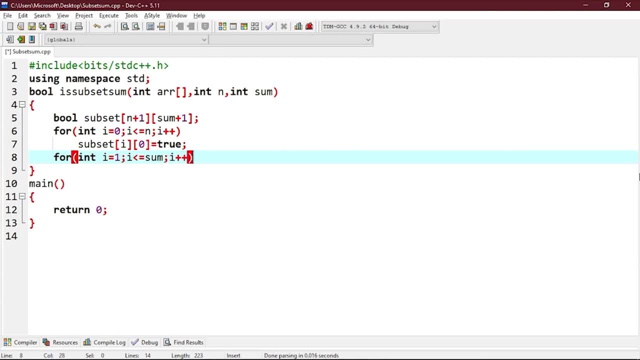 So bool subset n plus 1 to sum plus 1.. So bool subset n plus 1 to sum plus 1.. Now, in this case we will check at subset 0, comma 1, i equals to false. Now we will fill the subset table in bottom-up manner. 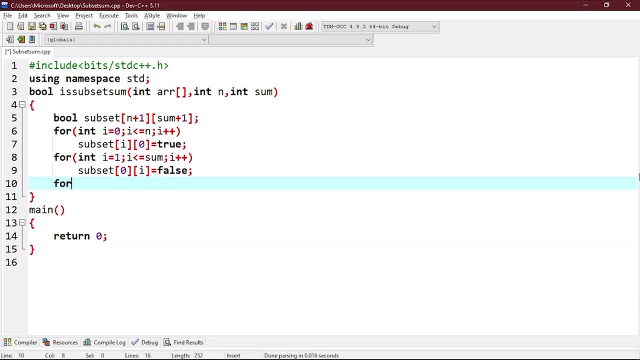 So 4.. and i equals to 1, i less than equals to n and i plus plus. we will add another for loop. and j is equals to 1, j less than equals to sum: a plus plus. now, if j is less than ARR, i minus 1. 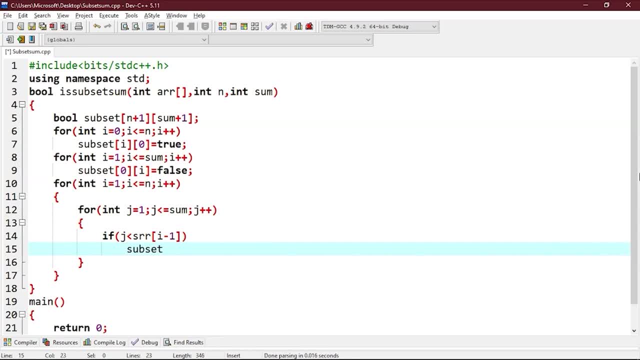 then subset i, comma j, will be equals to subset i minus 1 and j. now, if j is greater than equals to ARR at i minus oneじゃりました, then subset at i, j will be equals to subset i-1 to j. 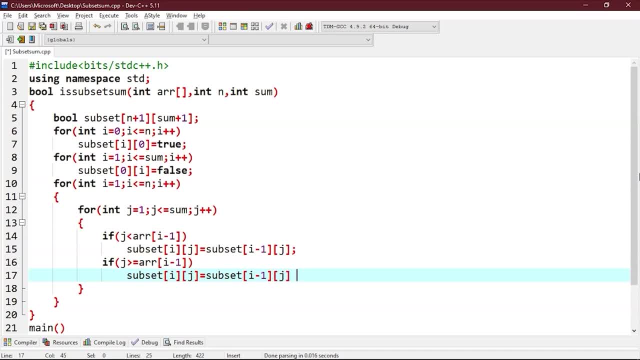 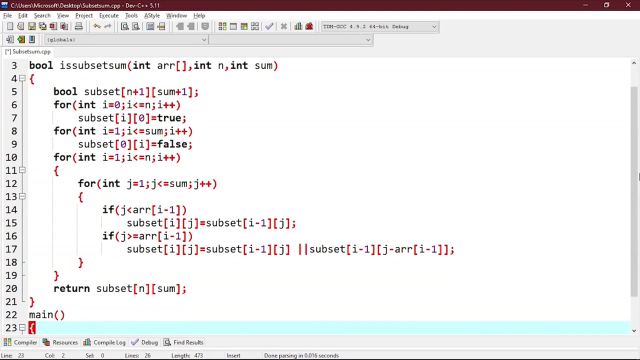 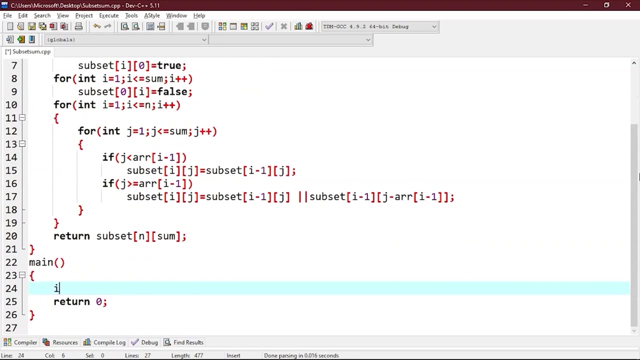 i or subset i-1 to j-arr. i or subset i-1 to j. Now we will return Subset at n sum. Now let's write the main block. So we will create and set Which will be equals to. 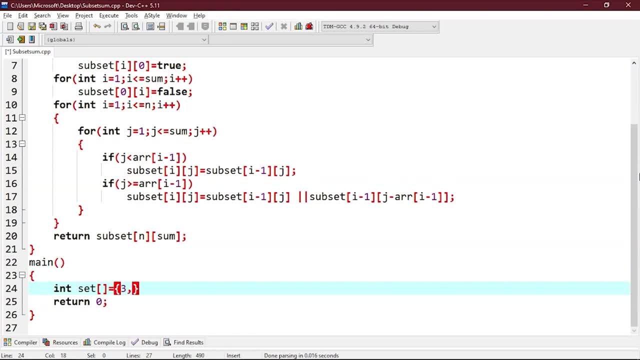 Values like 3,, 34,, 4,, 12,, 5,, 2 and so on, And we will have to find a subset with a sum equals to Sum equals to 9.. Now let's find the size of this set. 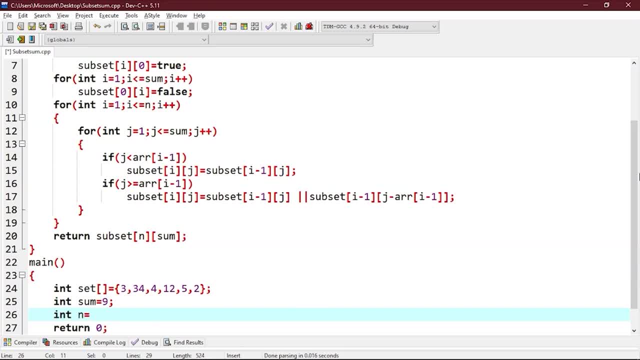 So int N equals to Size of Set Divided by Size of Set at 0th position. Now if Is subset Sum With With arguments as set N Sum Is equals to True. 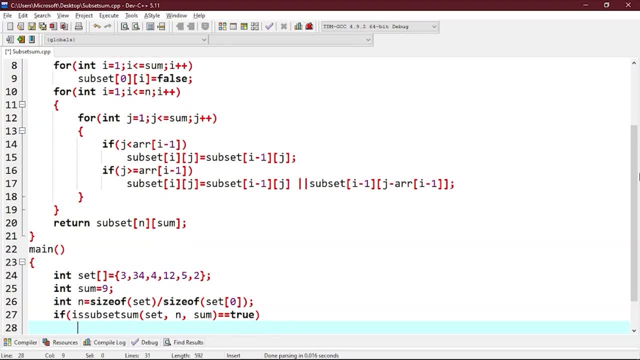 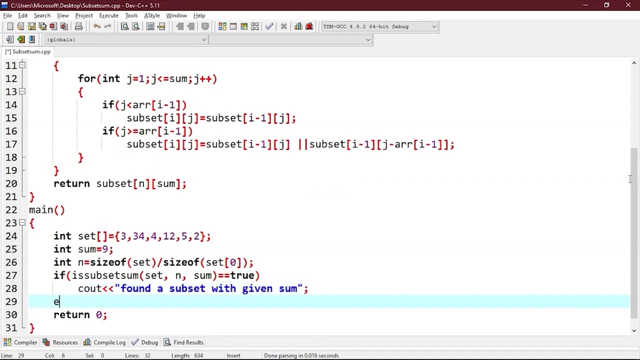 Then See out: Found A subset With Given Sum. Else See out: No Subset With Given Sum Is Found. Basically, If This Is Subset, Sum Gives True. 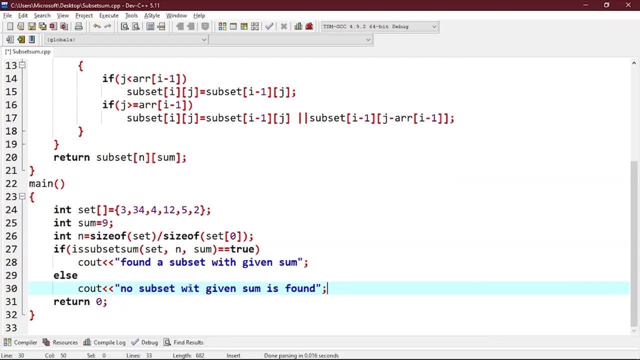 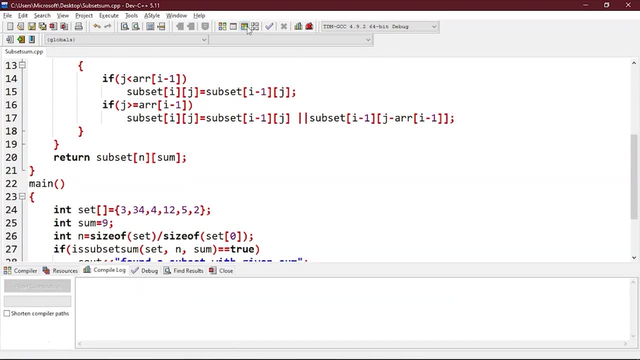 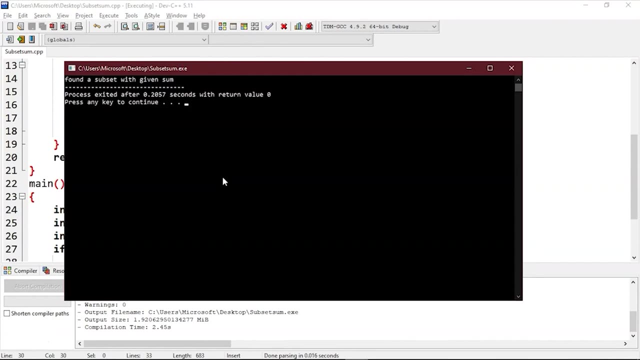 Then we will print the Found A subset With Given Sum. Otherwise We will print: No, Let's try To Execute This. As You Can See, We Are Getting A. 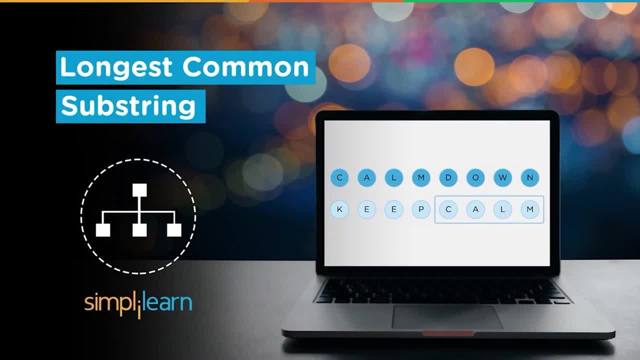 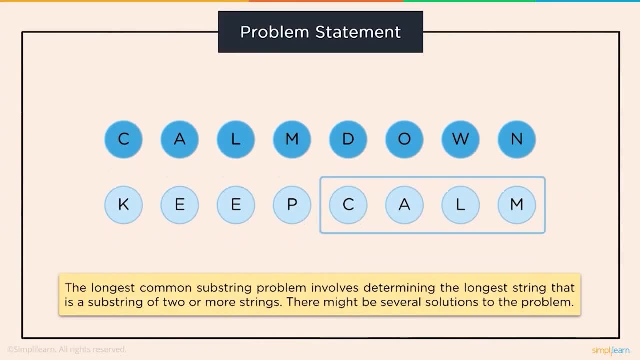 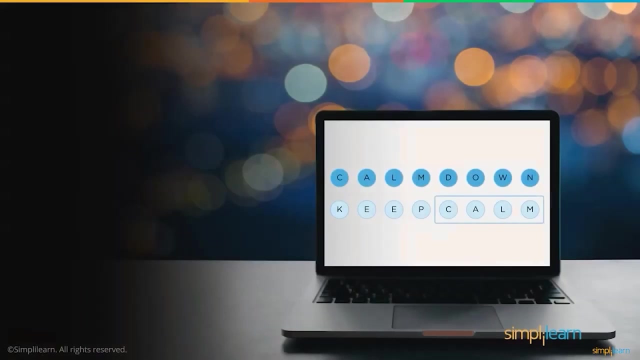 Found A Subset With Given Sum, Which Means We Have Found A Find The Length Of The Longest String, That Is, The Sub String Of. 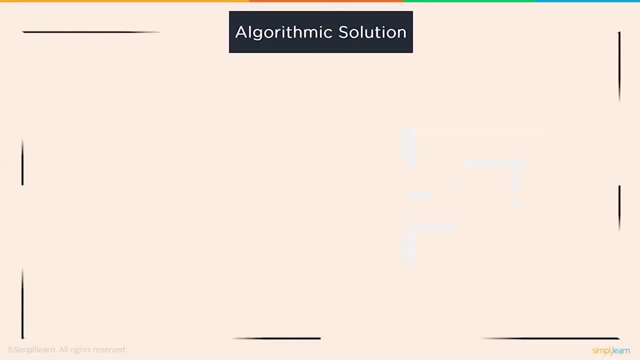 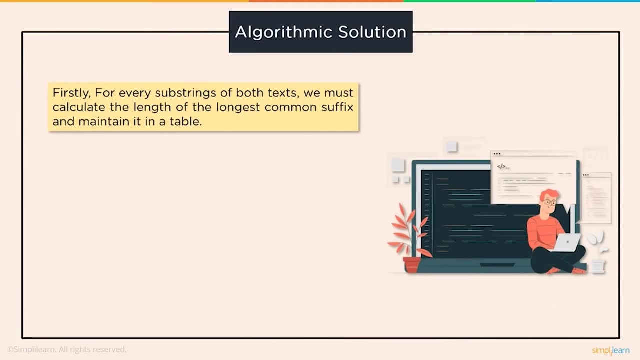 Two Or More Strings. There Might Be A Number Of Solution To A Situation Now If The Last Characters In The Longest Common Suffix Match. 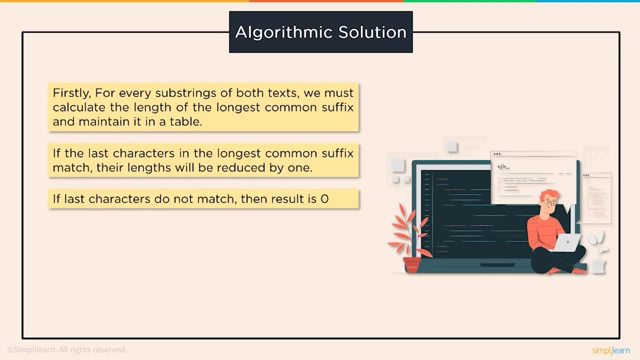 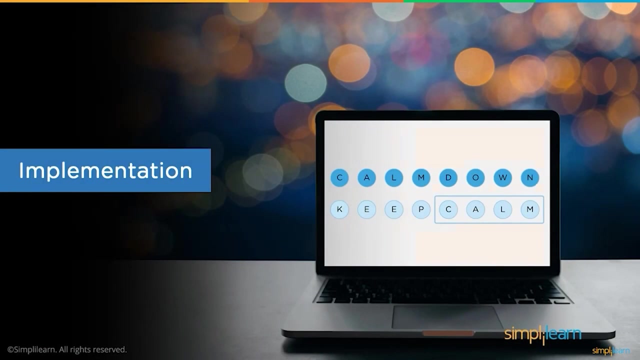 Their Length Will Be Reduced By One. Or If The Last Characters In The Longest Common Suffix Do Not Match, Then Use The Problem Statement. 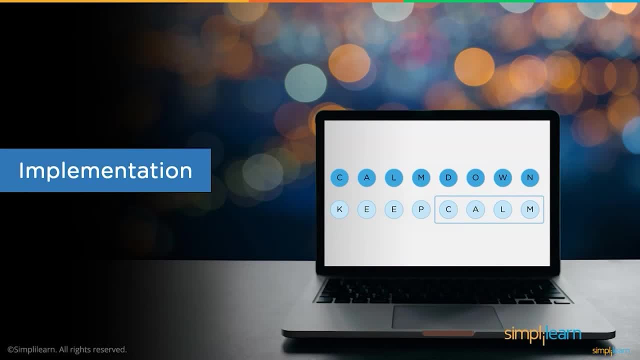 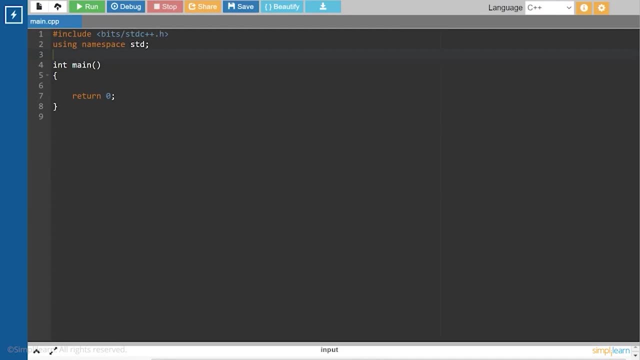 And The Algorithmic Solution To Find The Longest Common Sub String. Now Let's Implement This Solution In The Code Editor. We Will Start With. 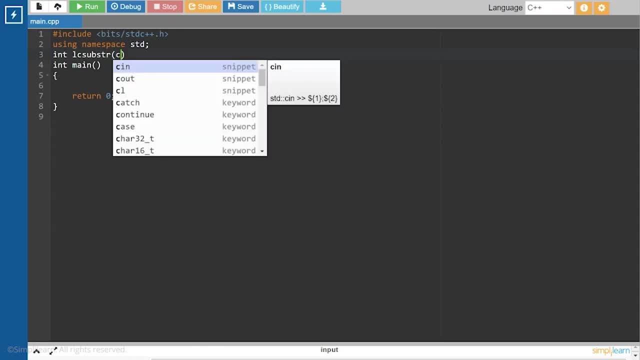 A. It's Argument As Star, Care X, Comma Character, Pointer Y And The Longest Solution Will Be Reduced By One. The Longest Solution Is: 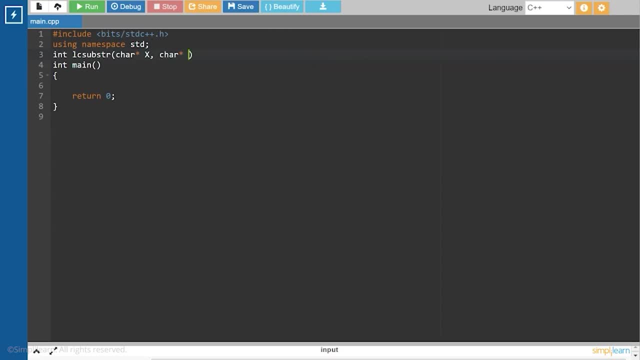 The Longest Solution Is The Longest Solution. Comma End: The Size Of The First String: X. Comma End, And This Will Be The Size. 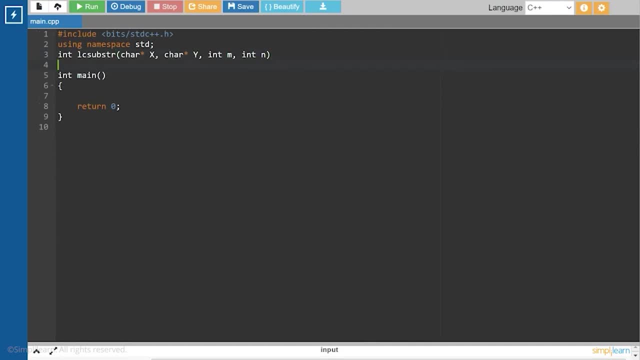 Of The Another String, Y. Now We Will Create A Table To Store The Length Of Longest Common Suffixes Of String. Now We Will 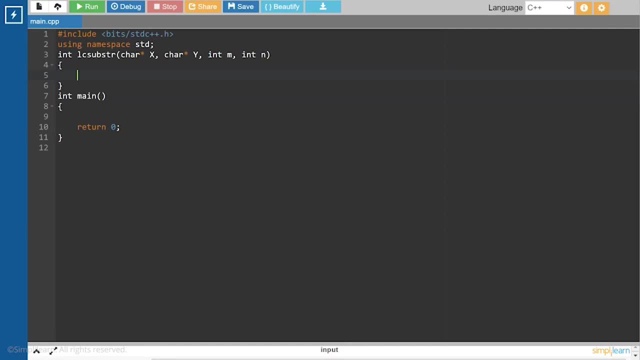 Create A Array LC Surf To Store The Length Of The Longest Common Suffix. So End LC Surf And N Plus One And Another Variable. 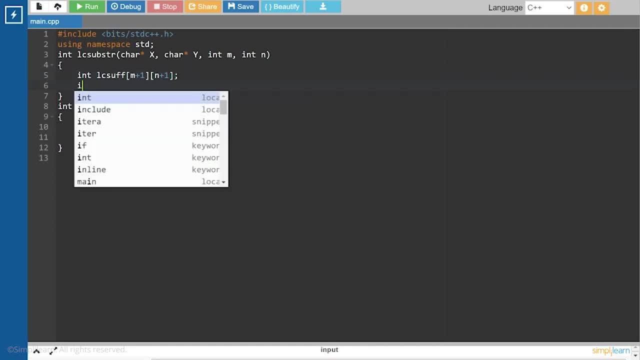 Result Equals To Zero. This Will Be Used To Store The Length Of The Longest Common Sub String. Now We Will Follow The Steps To. 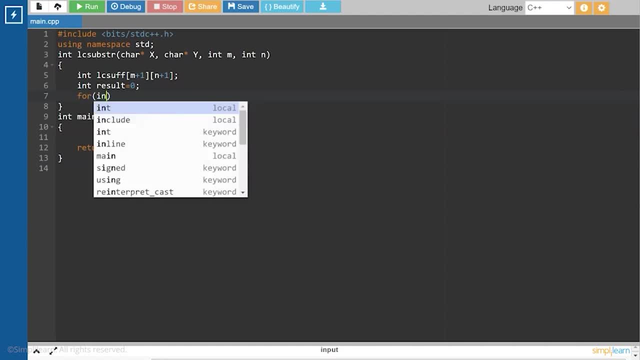 Build The LC Suffix In The Bottom Of Passion. So For Int, I Equals To Zero. I Less Than Equals To M. I Less Than. 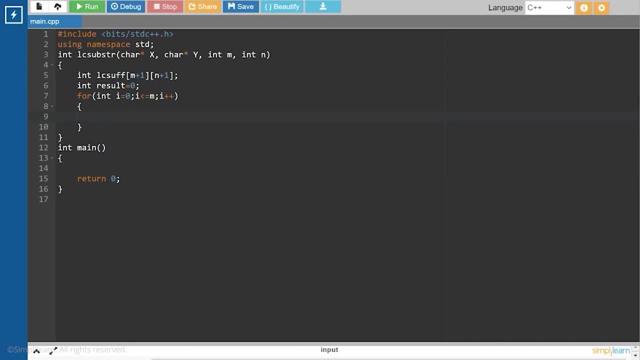 Equals To Another Nested Loop, For And J Is Equals To Zero, J Less Than Equals To, And J Plus Plus, And J Less Than Equals. 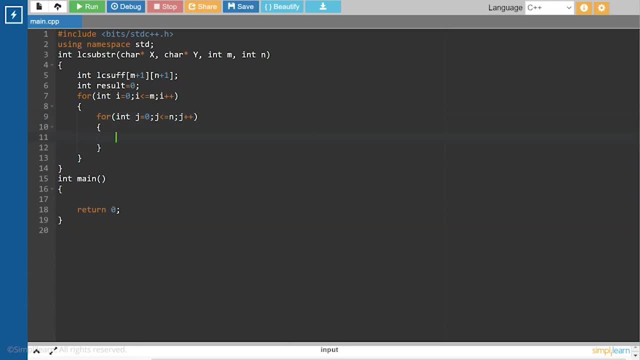 To And Zero. Now, The First Row And The First Column Entries Will Have No Logical Meaning. They Will Be Used Only For The Simplicity. 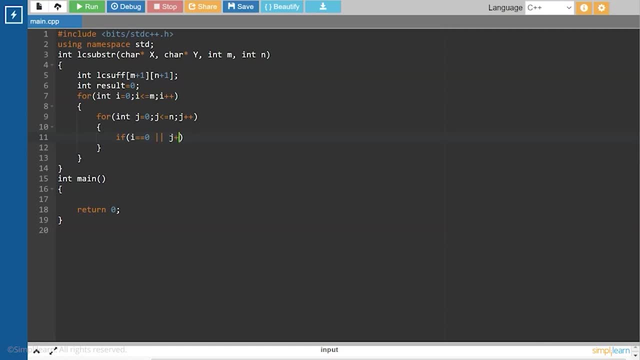 Of The Program. So If I Is, Then Else Is Of At I. J Will Be Equals To Zero Else If X At I Minus. 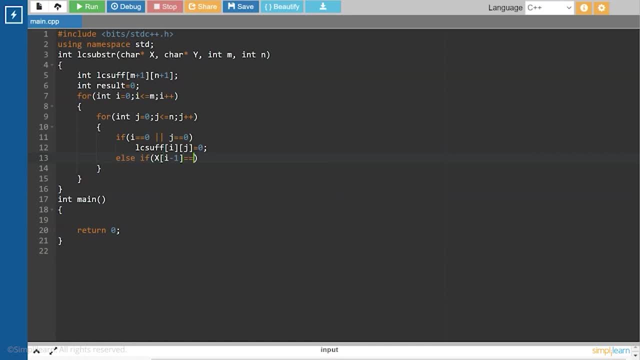 One Is Equals To Y. At J Minus One, Then Else Is Of. At I Minus One, And J Will Be Equals To Else Is. 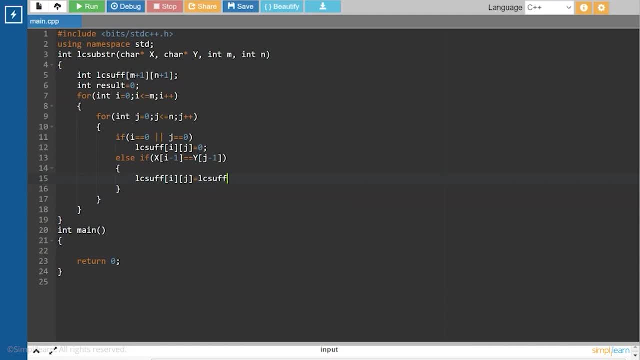 Of At I Minus One And J Minus One Plus One, And The Result Will Be Equals To The Maximum Of Result Comma Else. 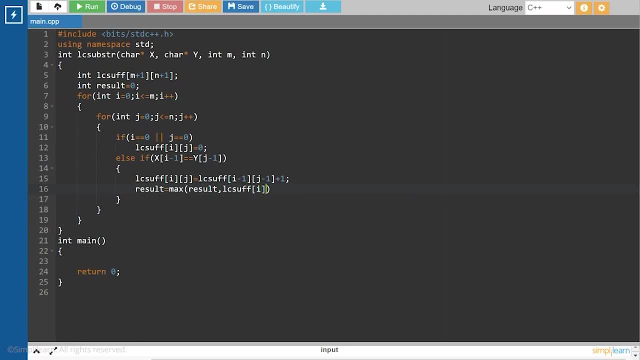 Is Of At I, Comma J. Else Is Of, Else Is Of At I, Comma J, Will Be Equals To Zero And We Will Return. 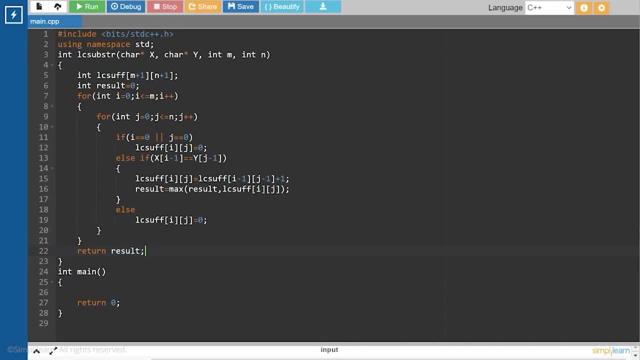 Result. Now Let's Write The Mean Block So, For X Is Equals To Comma Down And Another String Care. Why Is Keep Comma Now? 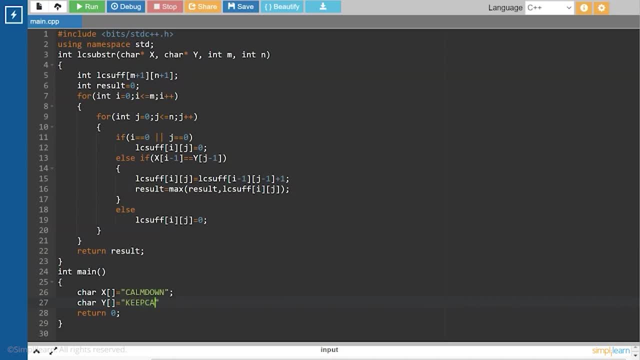 We Will Store The Length In M Equals To S T R L N Of X. Now We Will Store The Length In M Equals To: 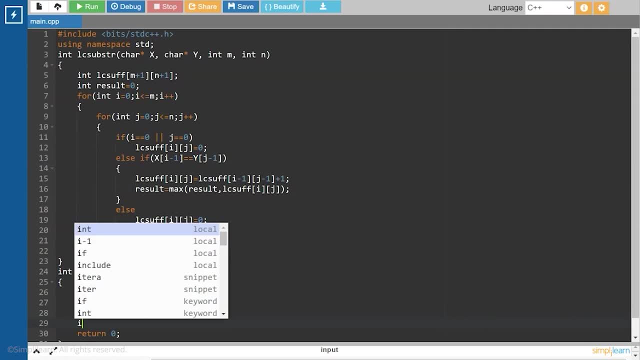 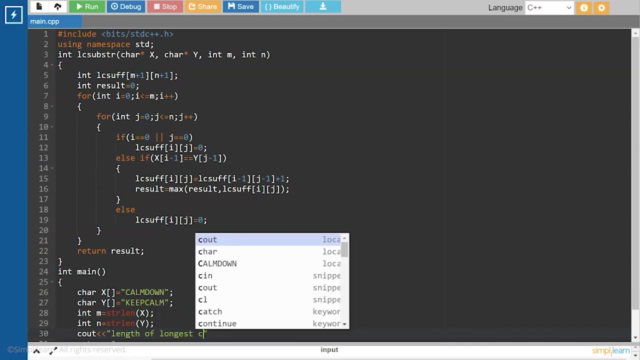 X And Int N Will Have S T R L N Of Y. Now We Will Print The Length Of Longest Common Sub String L C. 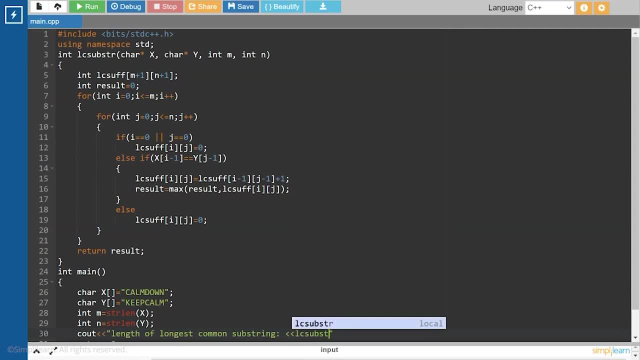 S Sub S T R At X, Y, M, N, X, N? S. Now Let's Try And Execute This. As You Can See, We Are. 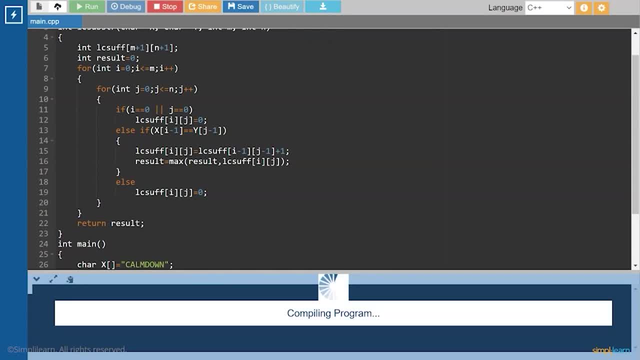 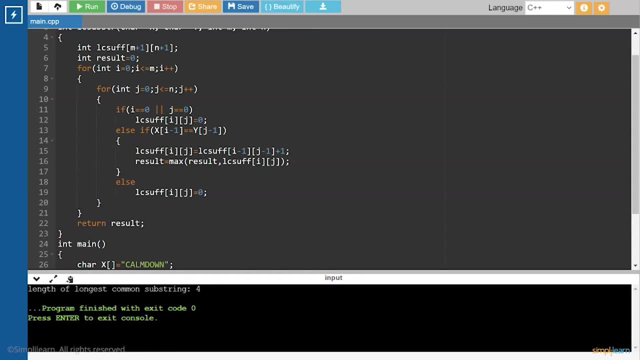 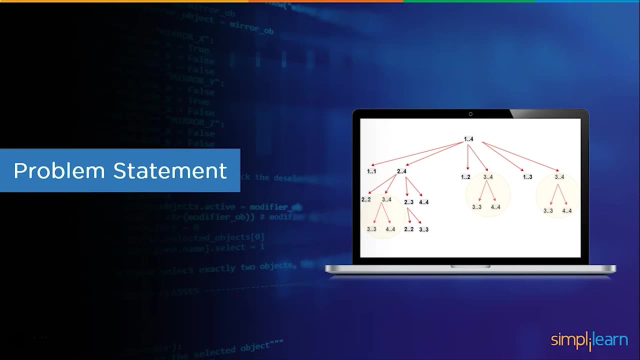 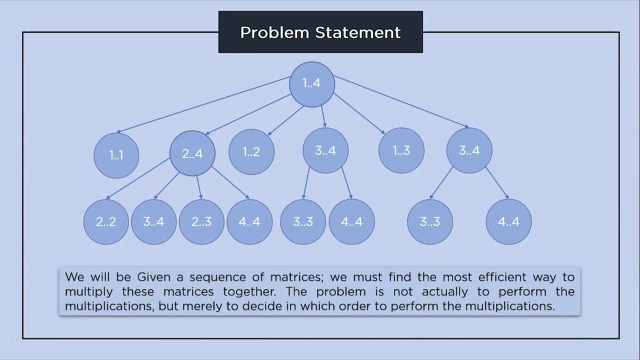 Getting The Length Of The Longest Common Sub String Is Four, Which Was Calm. Let's get started with an problem statement. We will be given a sequence of matrix. We have to find the most efficient way to multiply these matrices together. The problem is not. 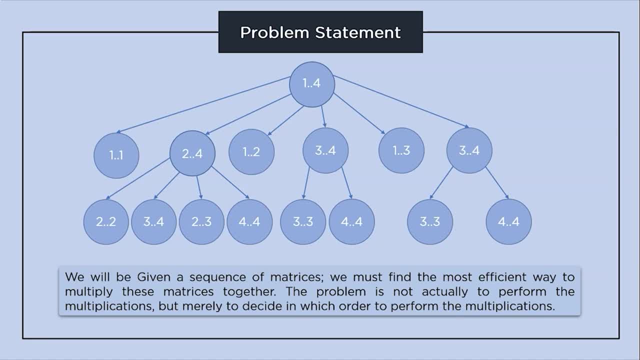 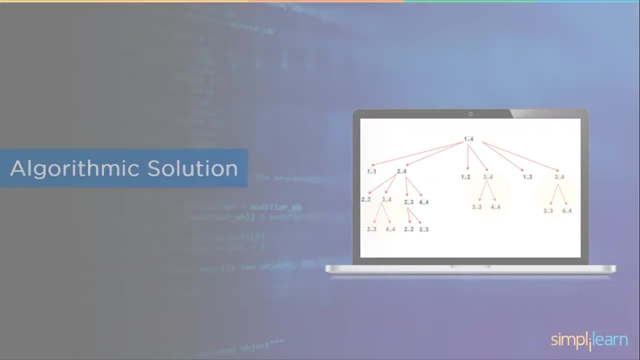 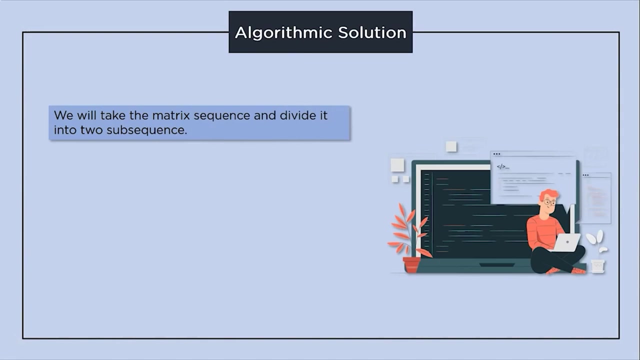 actually to perform the multiplication, but merely to decide in which order to perform the multiplication to get the minimum operations on a multiplication. Now let's discuss the algorithmic solution to the matrix chain multiplication. First we will take matrix sequence and divide it into two subsequence. Then we will calculate the minimum cost of 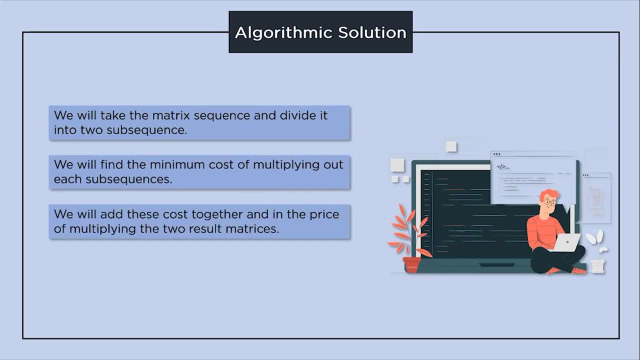 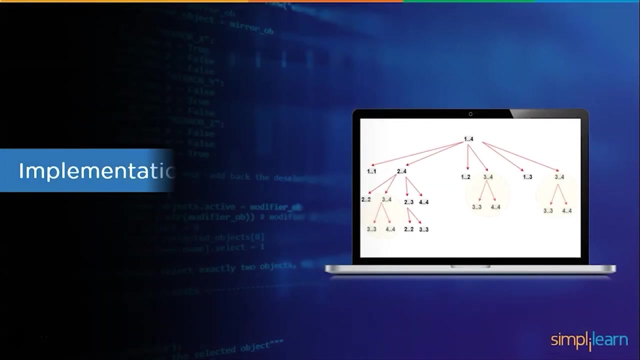 multiplying out each subsequence, Then we will add these costs together and in the price of multiplication, the two result matrices. Finally, we will repeat these steps for every possible sequence of matrices that can be split and take a minimum over all of them. We have now discussed the problem statement and the algorithmic solution to matrix chain. 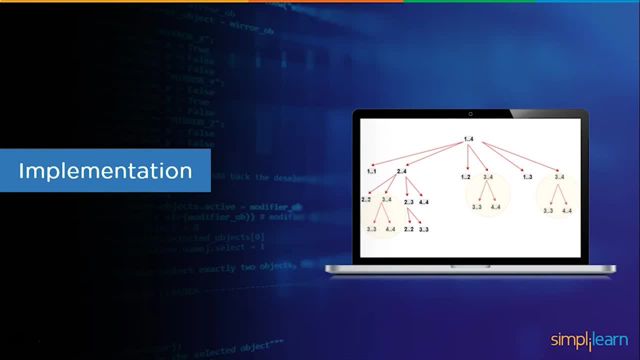 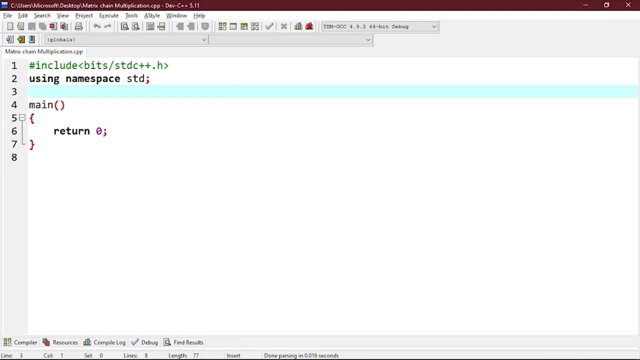 multiplication. Now let's implement this solution in the code editor. First we will define max10.. So hashtag: define max10.. Now we will lookup tables to store the solution to already computed subproblems. So int: lookup tables. 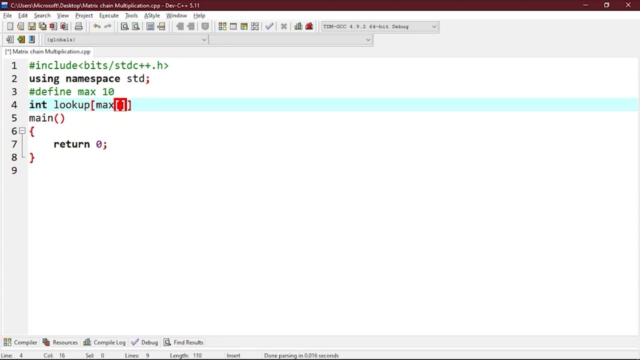 With dimension is max, max. Now we will write a function to find the most efficient way to multiply a given sequence of matrices: int, mcm, int, mcm, int, i, int, j. Now we will write our base case. that is one matrix, So if j is less than equals to i plus one. 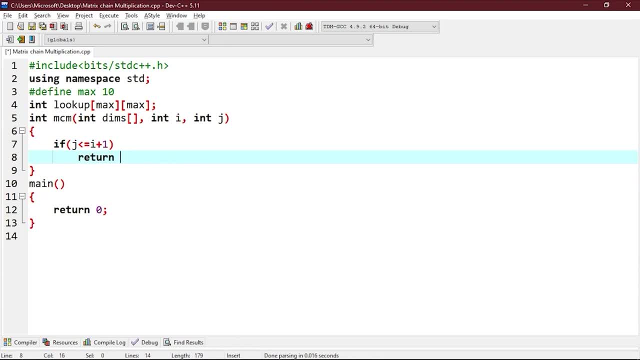 then we will return zero. Now what if it stores the minimum number of scalar multiplication that is, cost needed to compute matrix: m i plus one to m j, which is equals to m i to j. So int min should be equals to m i plus one to m j, which is equal to m i to j. So 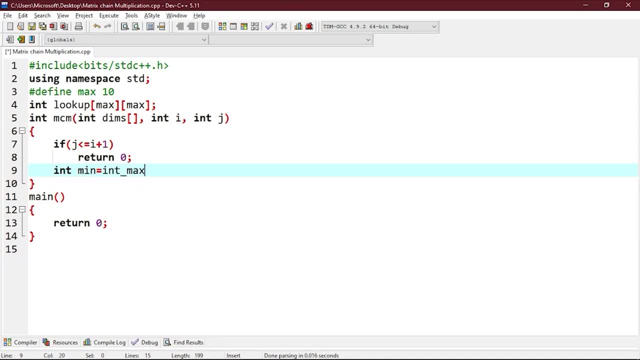 int underscore max. Now, if the subproblem is seen for the first time, then we will solve it and store its result in the lookup table. So if j is sin at the但是 self, Let's find it and see how it functions. lookup j: at i comma. j is equals to 0.. 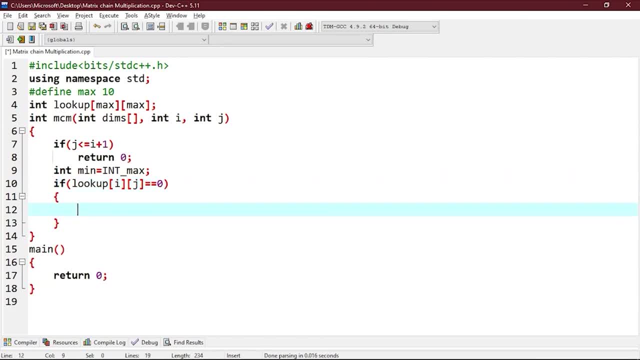 Now bus also will look up to 0. at i comma, j is equal to 0. So we will take the minimum over each possible position at which the sequence of matrices can be split. So mj is plus m j and y and mj is equal to m? j between each. So mj of m j. 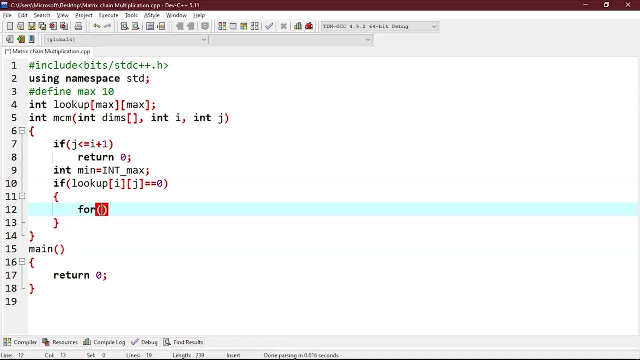 And k is equals to i plus 1, k less than equals to j minus 1 and k plus plus. Now we will recurve for m from i plus 1 to mk to get an ixk matrix. int first will be equals to mcm. 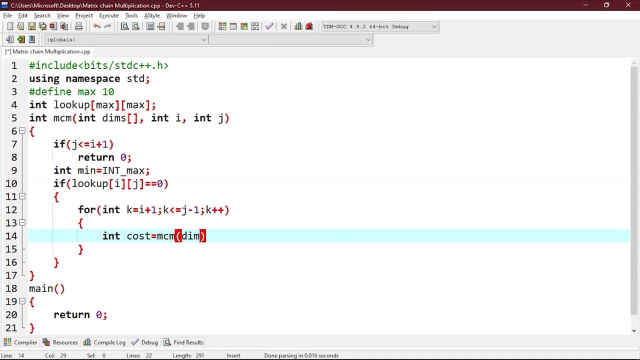 int first will be equals to mcm. int first will be equals to mcm. Now we will recurve for mk plus 1 to mjto get an kxj matrix. So qq班 wkp dk dxb. 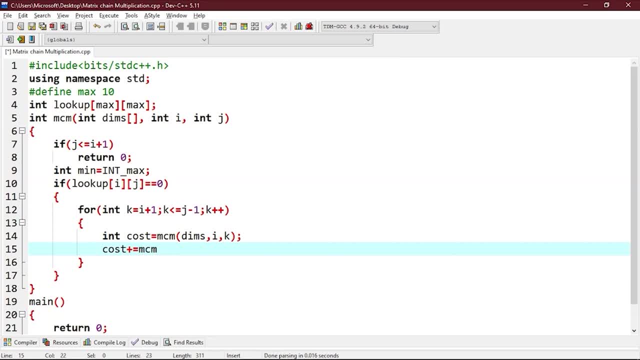 equals to MCM DEMS, comma K, comma J. then we will write the cost to multiply to IXK and KXJ matrix. so cost plus equals to DEMS I multiplied by MCM DEMS, DEMS K multiplied by DEMS at J. now if 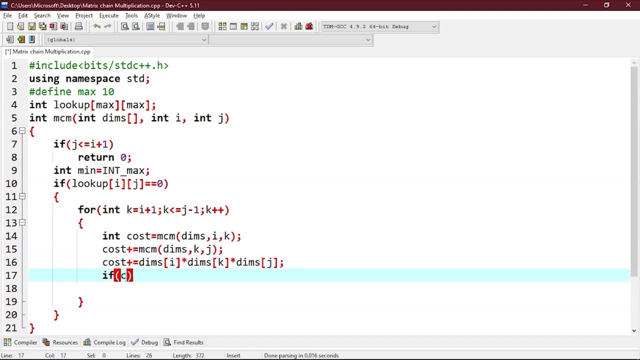 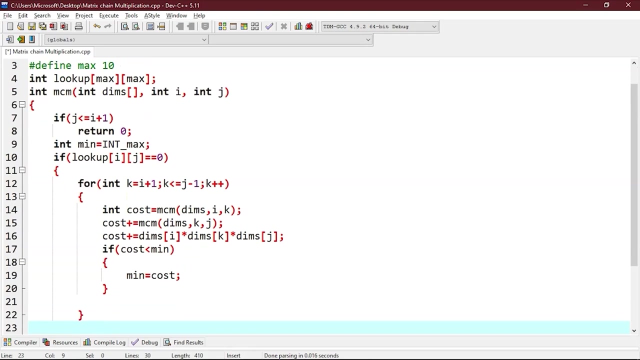 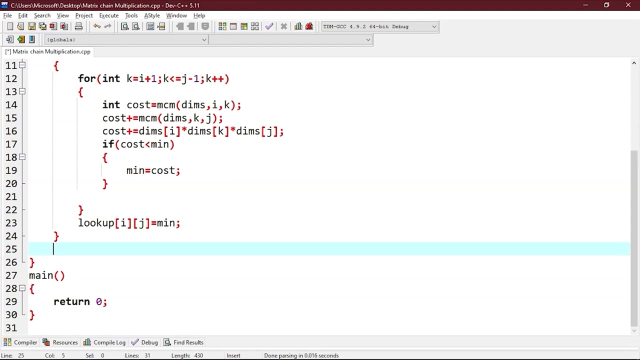 cost is less than min, then min will be equals to cost. now we will store the cost min at lookup at ij. Now we will return the minimum cost to multiply mj plus 1 to mj. So we will return lookup at ij. Now let's define a matrix. 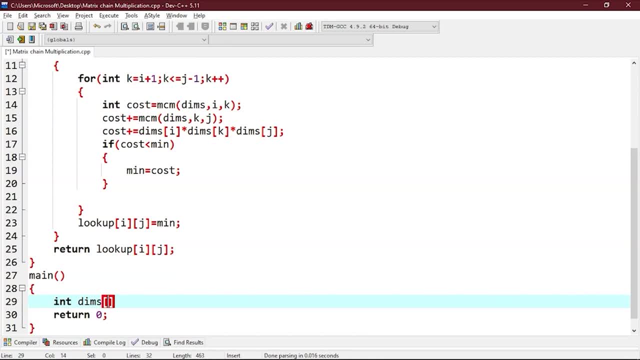 int dems equals to 10,30,5,60. Now we will find the size of this dems array. int n equals to size of dems divided by size of at dems com- 0. Now see out. the minimum cost is mcm. 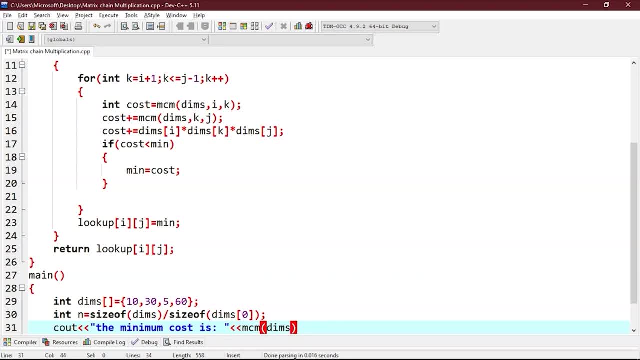 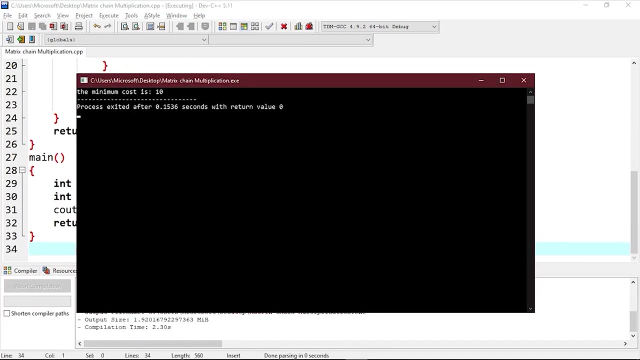 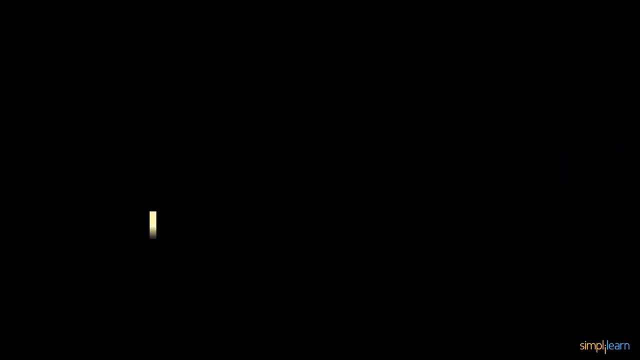 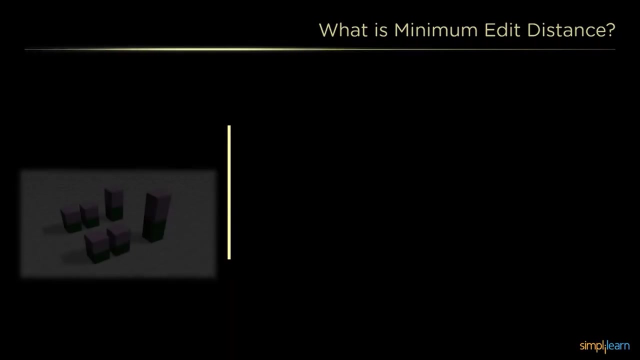 at dems: comma 0, comma n minus 1. Now let's execute this. As you can see, we are getting the minimum cost as 10, So our function is working flawlessly. What is minimum edit distance? So the answer for this question is: The number of editing operations required to convert one string into another is defined as minimum edit distance between two strings. 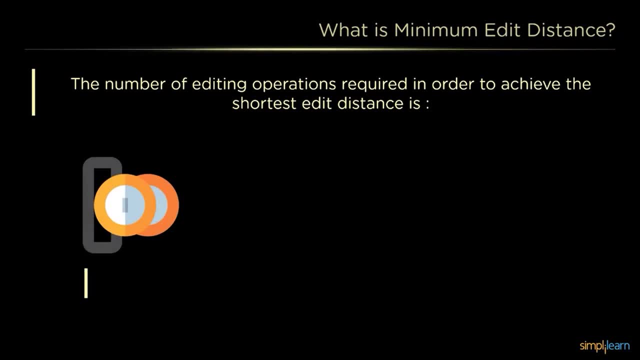 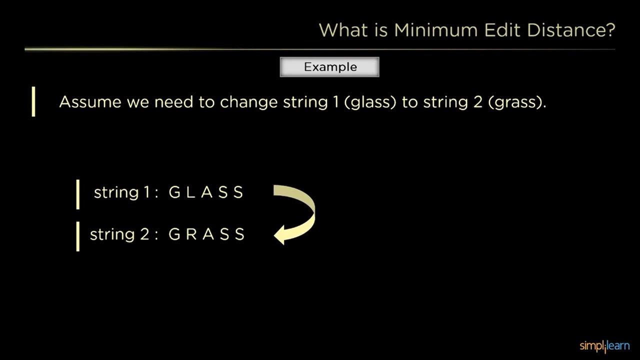 The number of editing operations required to achieve this shortest distance is called as minimum edit distance. The insert operation is used first in the minimum edit distance, followed by the remove operation and finally the replace operation. Now let us look into a small example to understand minimum edit distance in a much better way. 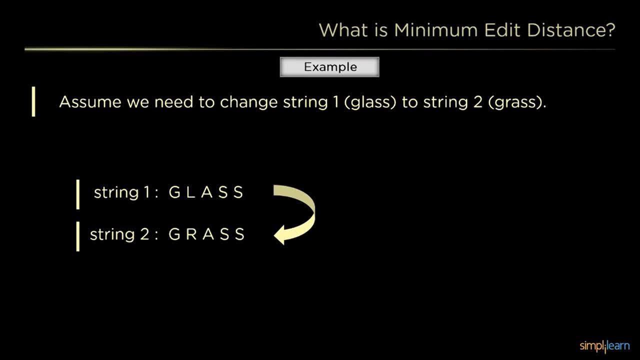 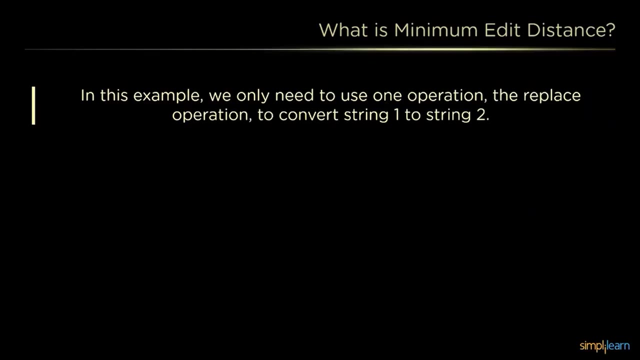 Assume that we need to convert string1- that is glass- into string2- that is grass. To convert glass into grass, apply the replace operation to the character r in the string2.. In this example, we only need to use one operation, that is, the replace operation, to convert the string1 into string2.. 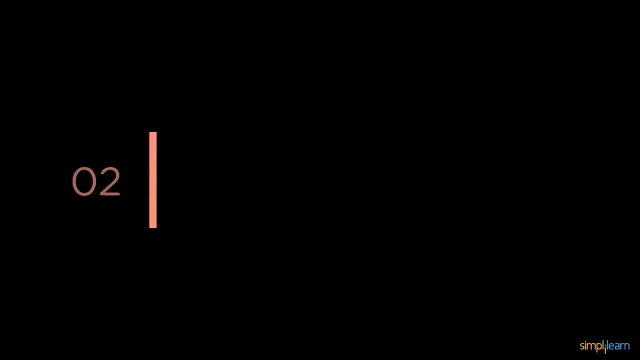 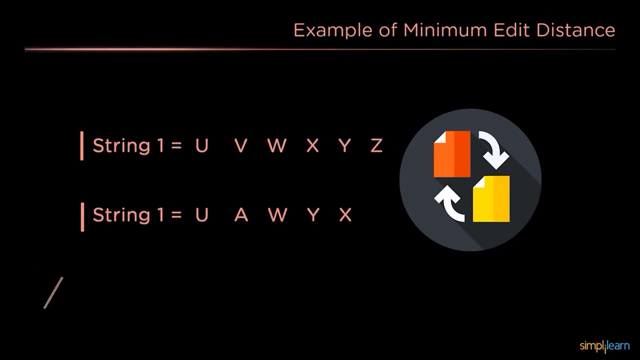 Next we will look into another important example to see how minimum edit distance works in practice. In this example we must convert string1, that is uvwxyz, into string2, that is uawyx. So first we will look into the first character of the string1, that is u. 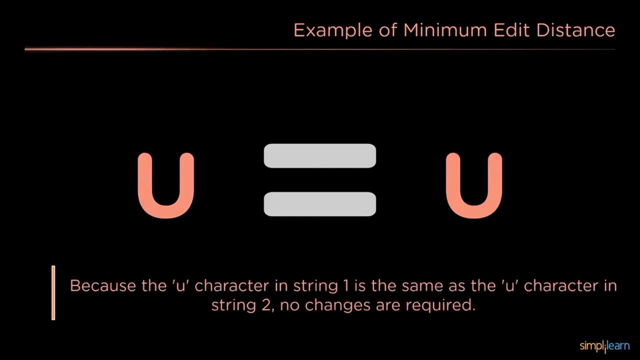 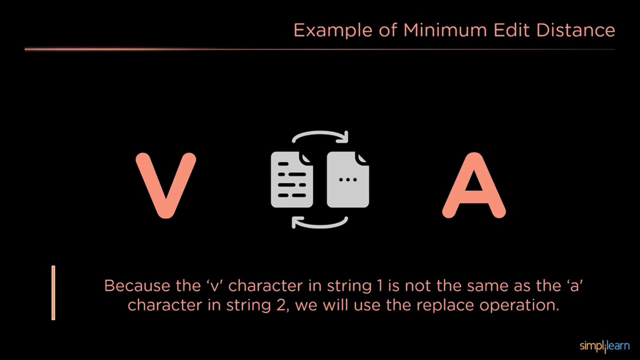 And the first character of string2, that is also u. No changes are required because u character in the string1 is same as the u character in the string2.. Next we will compare the second characters of string1, that is u, With the string2, that is u. 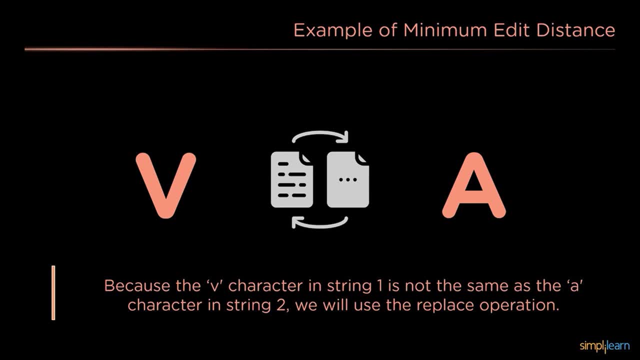 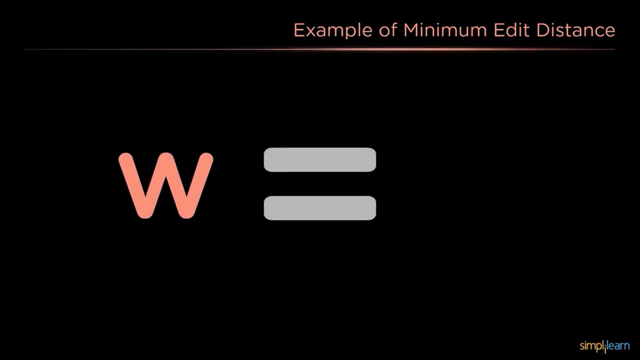 We must use the replace operation because v character in string1 is not same as a character in string2.. We are now comparing string1's third character with string2's third character, that is w. for the same, No changes are required, because w character of string1 is equal to the w character of string2.. 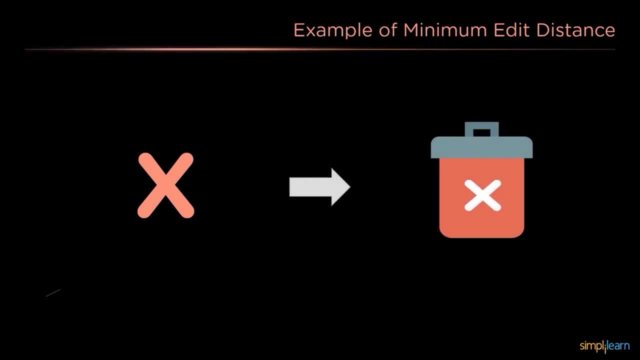 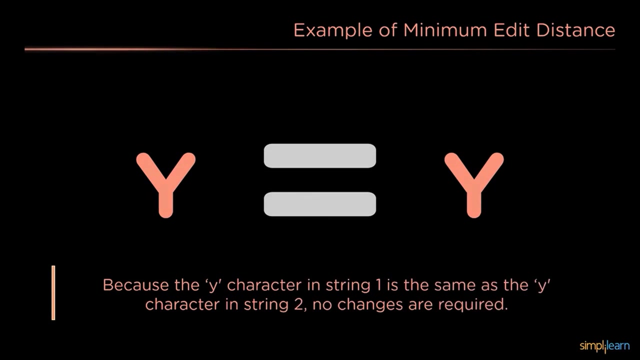 Now we will look into the next character of string1, that is x, Because x character in string1 is unnecessary, So we will remove the x character using the remove operation. The next character in string1 is y. We will compare it to the next character of string2, that is also y. 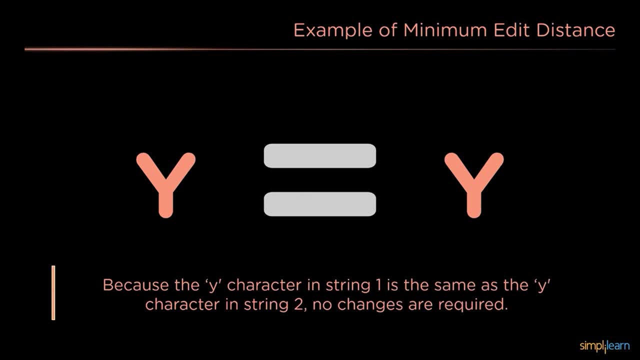 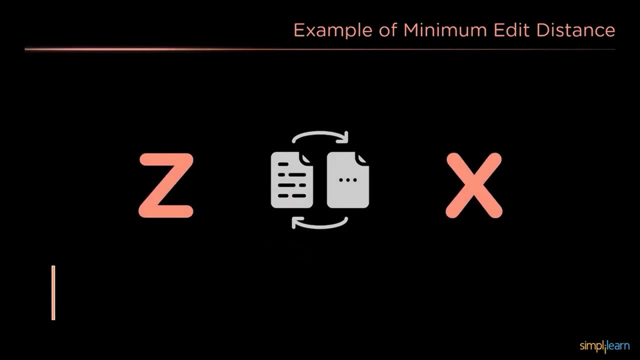 So no practical changes are required here, since both the characters are equal to each other. Finally, we have the comparison of z characters: Z character from string1, and we will compare that to the last character of string2 that happens to be x. Now we will have to use the replace operation, because z character of string1 is not equal to the x character of string2.. 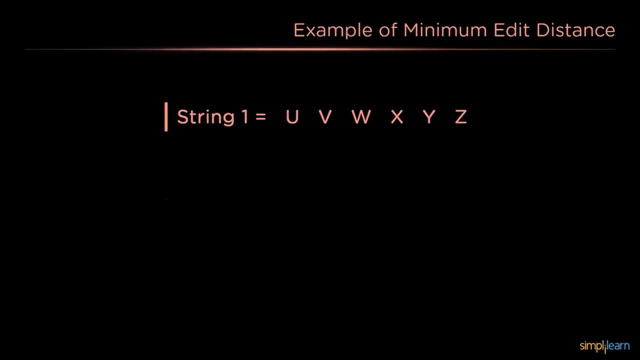 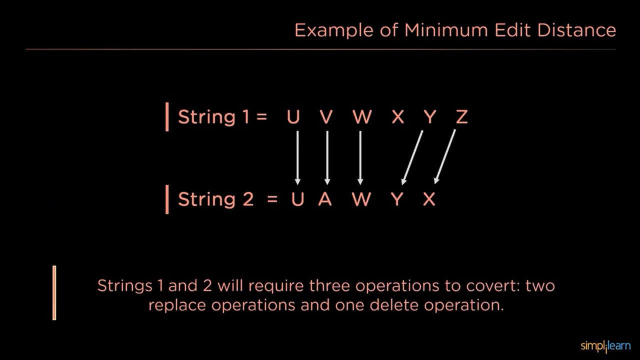 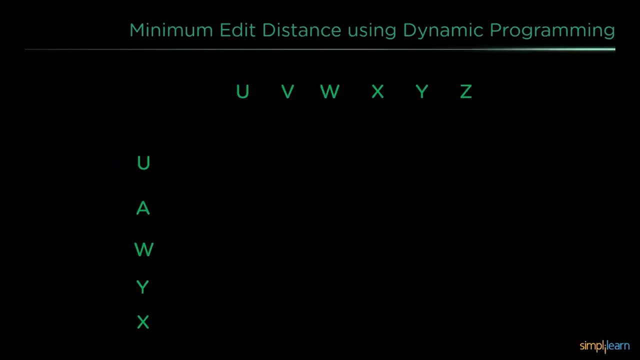 Now, to convert string1 into string2, we require three operations, That is, two replace operations and one delete operation. So the final topic in this session is Minimum edit distance using dynamic programming. Using the same example as before, We will continue with the minimum edit distance using dynamic programming. 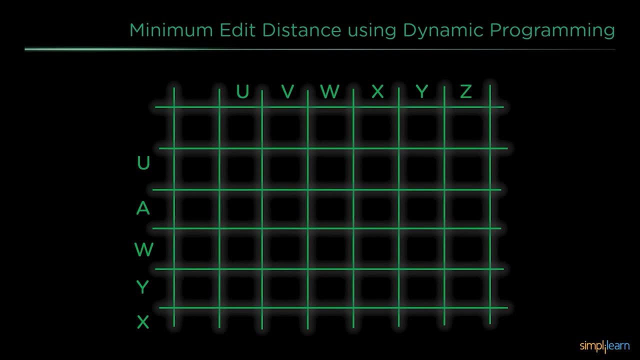 So in this example we have a string that is uvwxyz on the row side And another string that is uawyx on the column side. We will use dynamic programming to convert one string to another To find the minimum number of operations required. 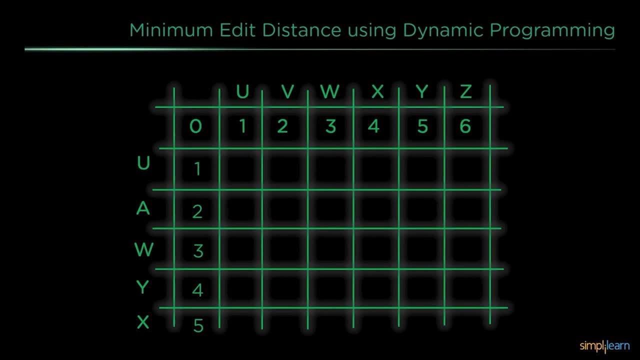 To perform this conversion. So our first row contains the first string, that is uvwxyz, And our first column contains the second string, that is uawyx. We then have an extra column and row Stating that string1 will require six edits to convert string2.. 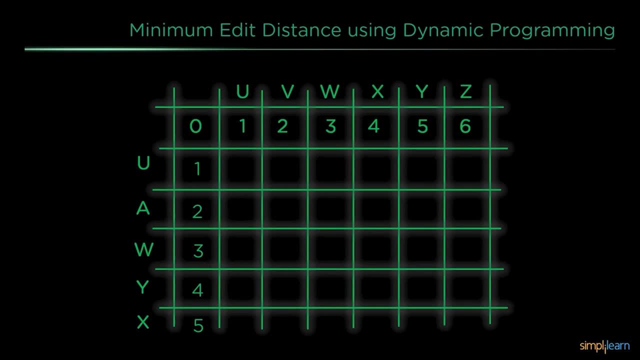 And string2 will need five operations to convert to string1.. Let's get started on filling out the rest of the matrix. So, since the first character of string1 is u And second character of string2 is also u, So converting the? u will not require any operations. 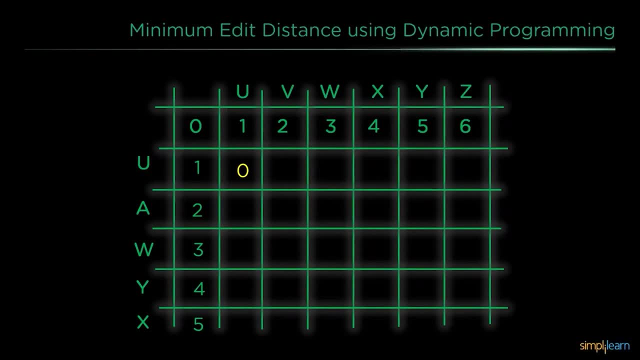 So we have 0.. Now string1 has two characters of u and v, And string2's first character is u, So it will take only one operation to convert from this to that. Next we have uv and w in string1. 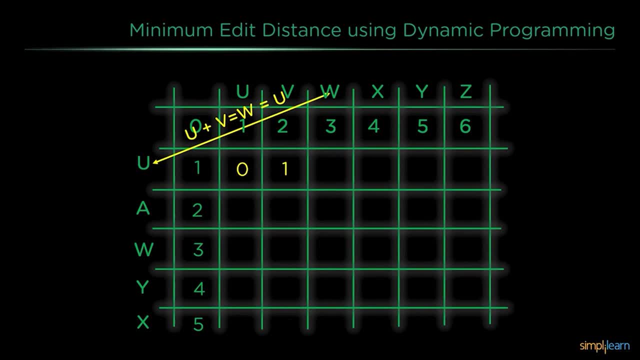 And u in another string. Converting them will require two operations, With uvw and x in string1 and in string2.. It would take three operations to convert If we have uvwx and y characters in string1. And u characters in string2.. 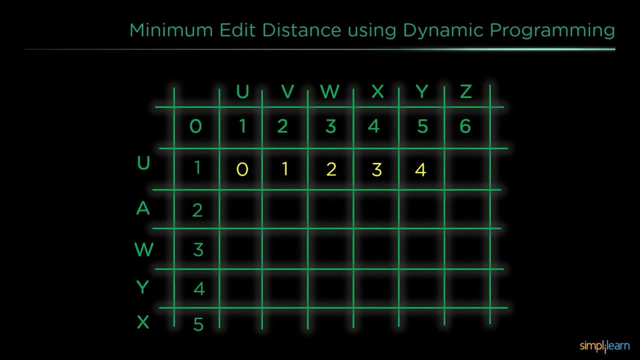 We will need to convert them using four operations. Next, we will have six characters- uvwxy and z- And u character in string2.. It will take five operations to convert them. Let's fill up the second row with u characters in string1.. 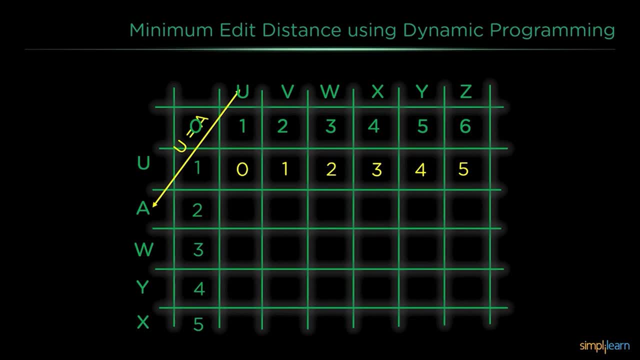 And u and a in another string, To convert u to u plus a in one operation. Next, we have u plus v in string1.. And u plus a in another string. So converting them will take one operation Because we have uv and w in string1. 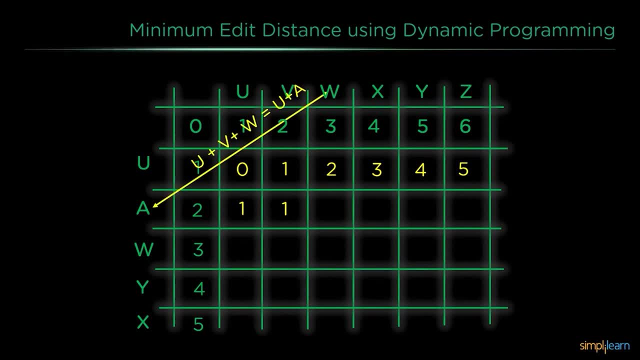 And u and a in string2.. Converting these characters would require two operations. Next we have uvw and x in row side And u and a on the column side. These will be requiring three operations to convert. Next we have uvwx in row side. 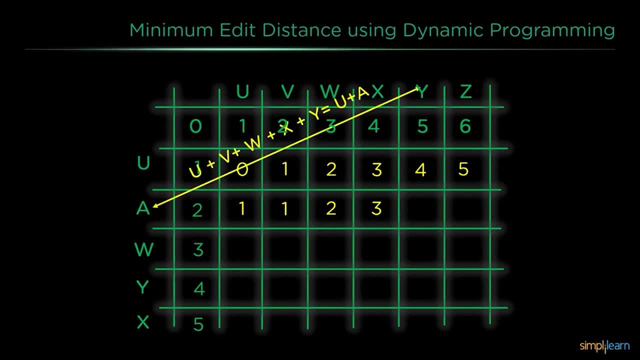 uvwx and y in string1. And we need to convert it to u and a character of string2.. This conversion will take four operations And now we have all six characters in string1.. uvwxy and z. 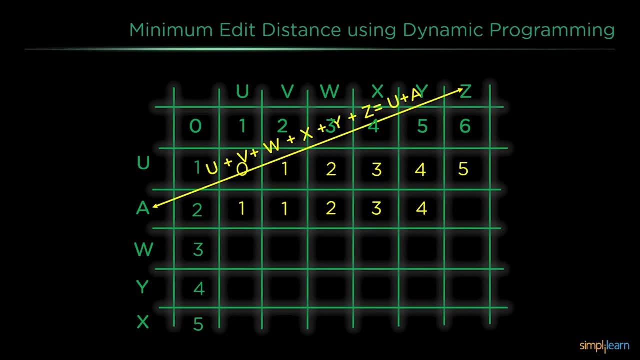 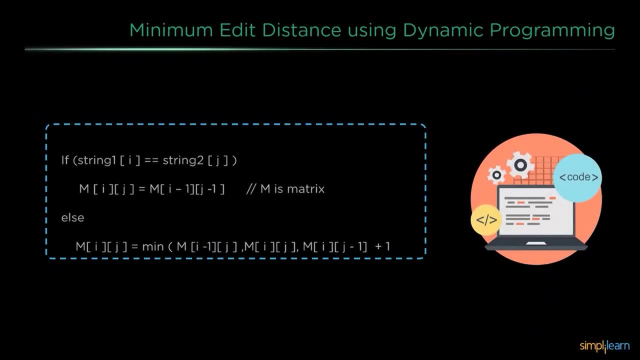 And we need to convert it to u and a character from string2.. This conversion will take five operations. If you found it challenging to compute the number of operations using this method, We devised a new formula That states that if the character of string1 is the same as the character of string2.. 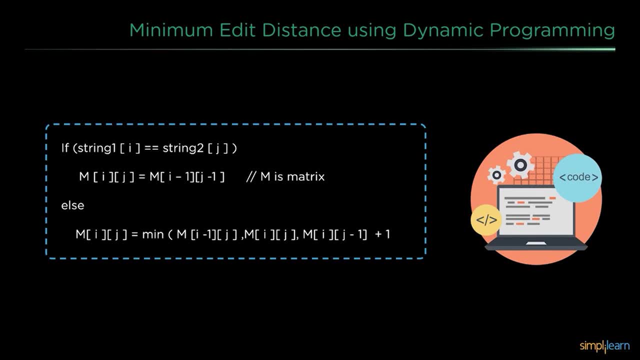 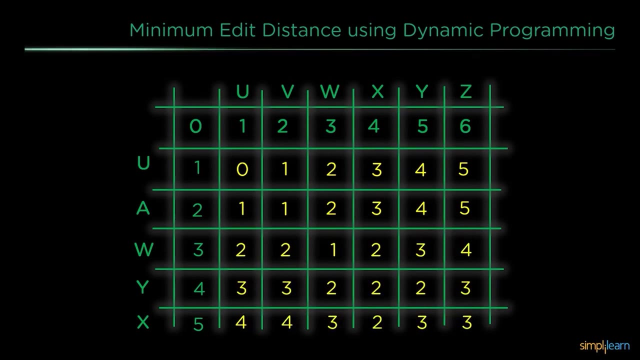 We get the diagonal value as the number of operations, But if the characters of both strings differ We have minimum of let top and diagonal values plus one. So using this formula We filled all the matrix values to convert string1. That is, uvwxyz to string2.. 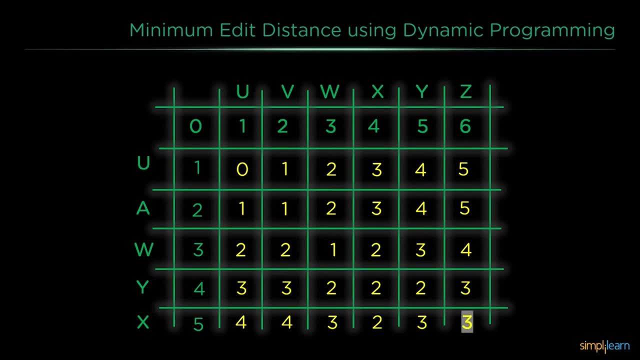 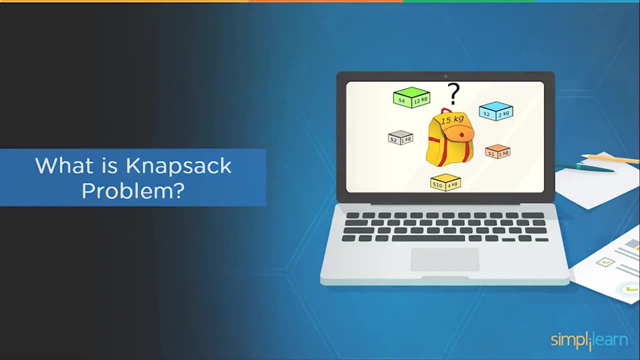 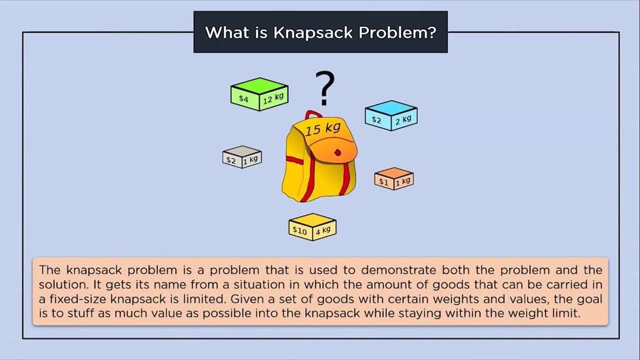 That is uawyx, So the last value of the matrix, Which is our answer. Both string1 and string2 require three operations to perform the conversion. Let's get started with the topic. What is knapsack problem? The knapsack problem is used to explain both the problem and the solution. 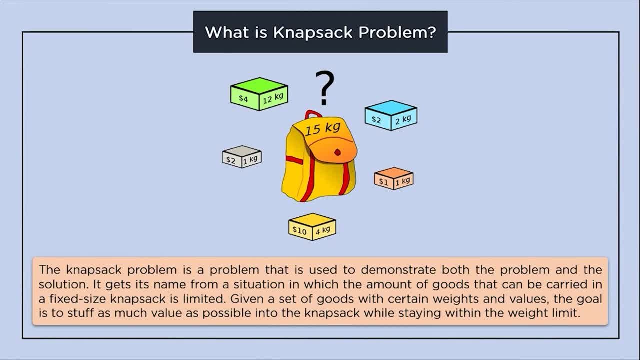 It derives its name from the fact that the limited number of things That may be carried in a fixed size knapsack Given a set of items with varying weights and values. The goal is to pack as much as value as possible into the knapsack. 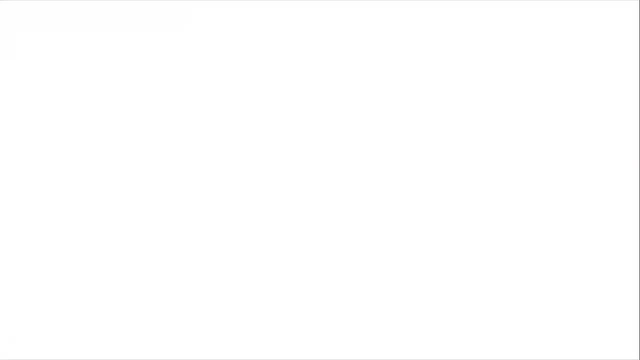 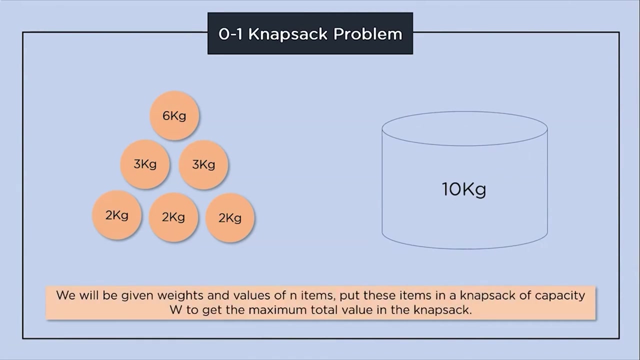 While staying within the weight limit. Now let's discuss zero-one knapsack problem. First, we will be given weights and values of n items, In this case six items on the left. We will put these items in a knapsack of capacity. w or in this case, 10 kgs. 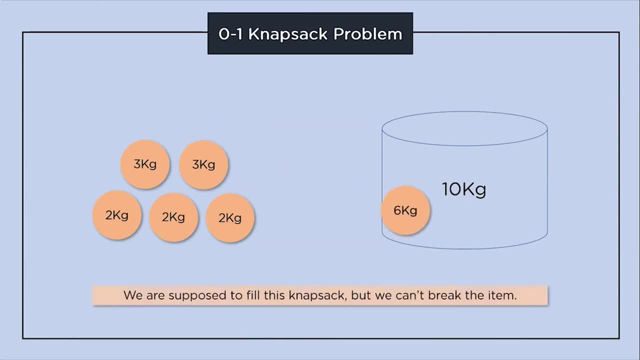 To get the maximum total value in the knapsack, Then we will have to fill this knapsack, But we can't break the item, So we must either pick the entire item or not pick at all. Due to this, sometimes it may even lead to a knapsack with some spare space left with it. 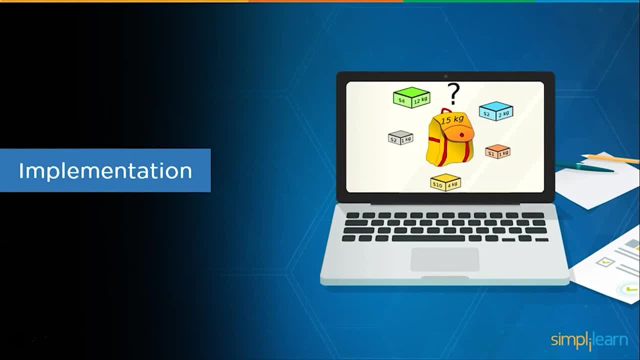 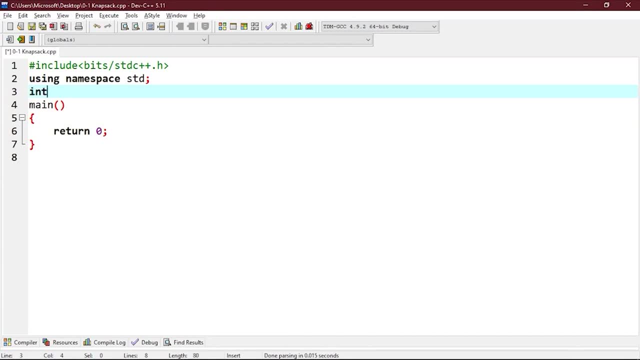 Now let's try to implement this in the context. We will start with the utility function that will return the maximum of two integers, int max. We will return f is greater than b, Then a Else b. We will now write a function to return the maximum value that can be put in a knapsack of capacity: w. 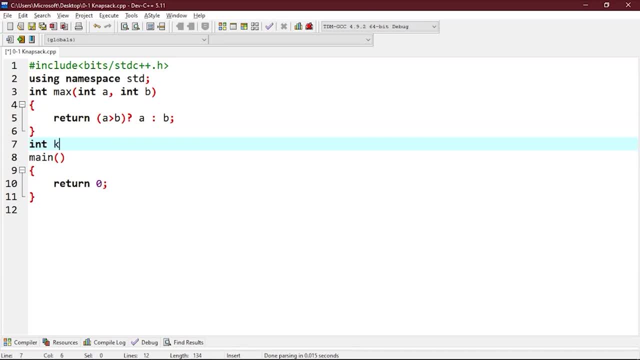 int knapsack, int capital w, int wt for the weight: int value, int value, int n, int value, int value, int potential. We will declare int i, w. We will create a vector. Inside a vector, We will use the key A, n plus 1 comma: vector. 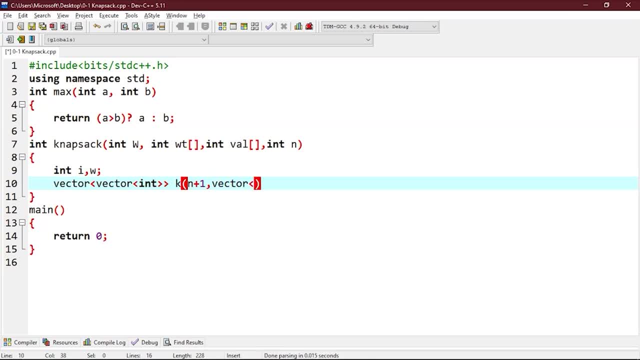 int capital w plus 1. now we will build the table k in bottom up manner. so for i equals to 0, i less than equals to n, i plus plus, we will have another for loop inside it, for loop with small w equals to 0. this small w will be less than equals to capital w. 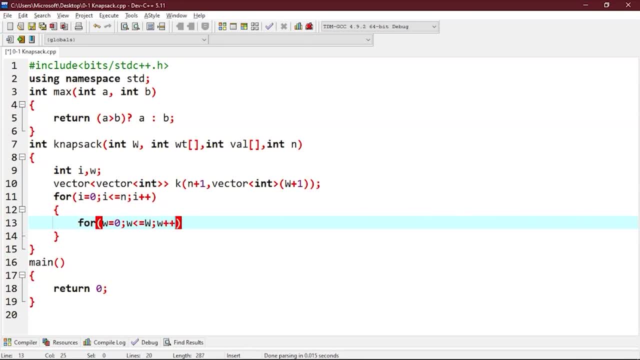 with small w plus plus. now, if i is equals to 0 or w is equals to 0, then we will have k i comma w is equals to 0, else if, if the weight at i minus 1 is less than equals to w, then k at i comma w. 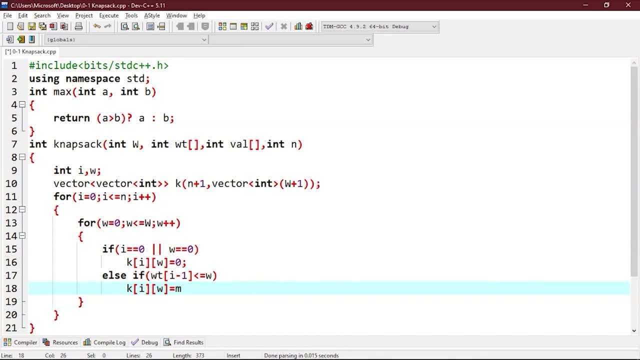 will be equals to max of k at i minus 1 comma, 1 minus i. 1. i i minus k. volume. at i minus 1 plus v value. at i minus 1 plus k. at i minus 1 comma, this will be equal to the. 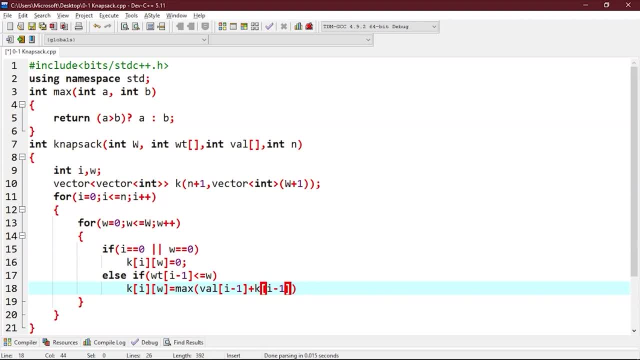 value at i minus 1 comma, at i minus 1 minus 1, i minus 1 W minus Wt, where Wt is at i-1, k at i-1, W, Else we will have k at i. W is equals to. 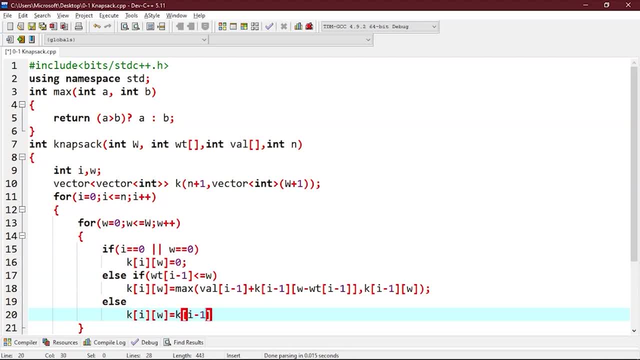 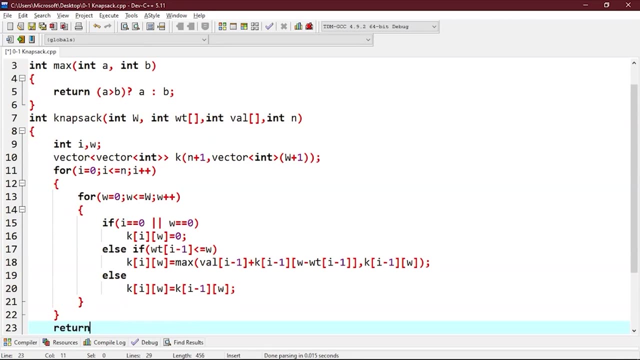 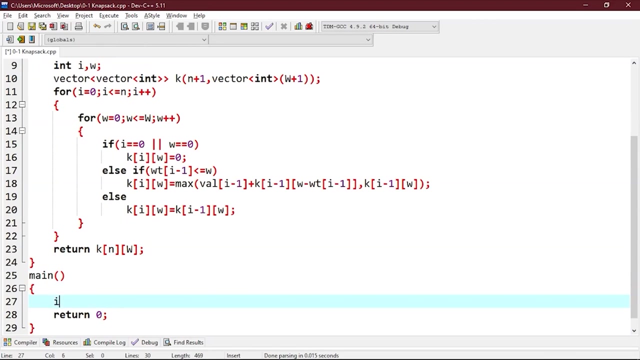 k at i-1, W. Now we will return k at n, W. Now we will write the main block. Now we will write the main block. We will start with int, int, valueArray, which will have, which will have elements as elements as: 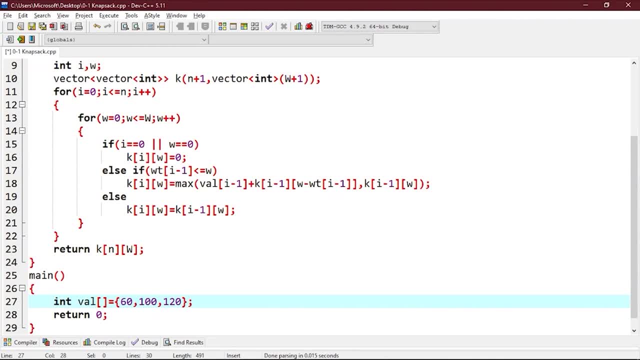 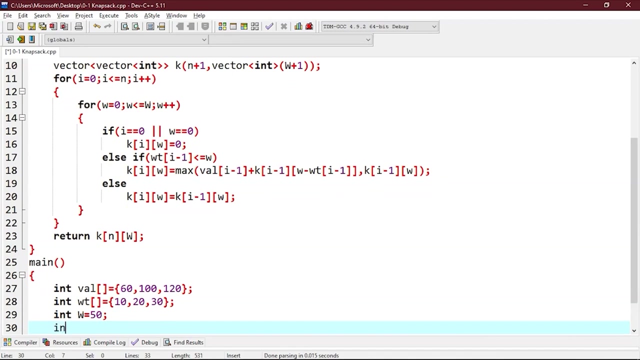 int, int, int, int, int, Then int, int, int, do, dou, dou, and the maximum capacity, the capital W, will be equals to 50. now let's find the size of the value array. so and n is equals to size of well divided by eyes off well at 0 location. 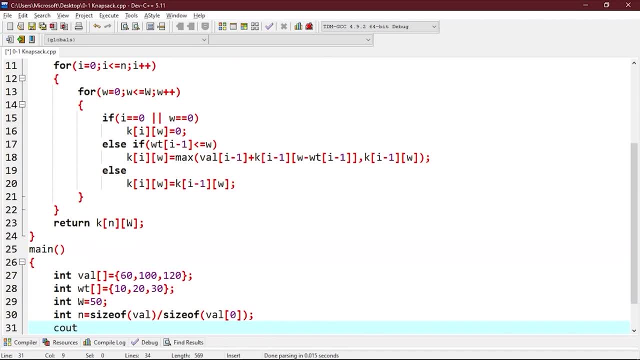 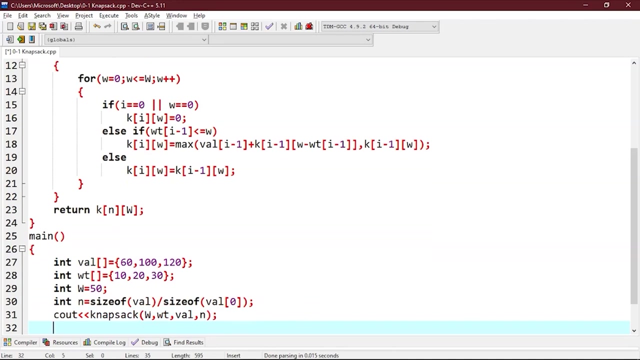 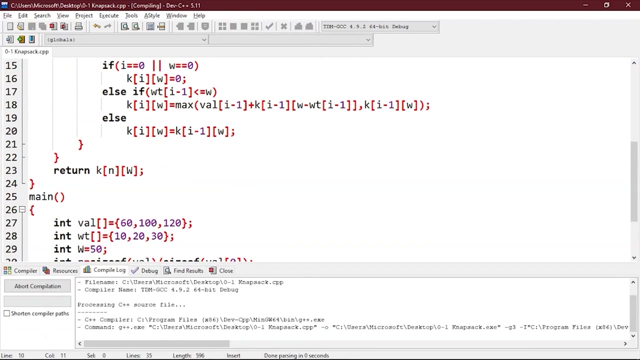 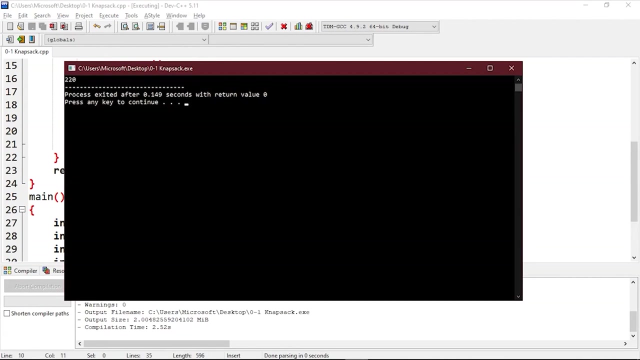 now we will print C of knapsack at capital, W comma, WT comma- well, my end- and return it as zero. let's compile it. as you can see, we are getting the value as 220, which means we are getting it because we are taking the elements with weight equals to 20 and 30. 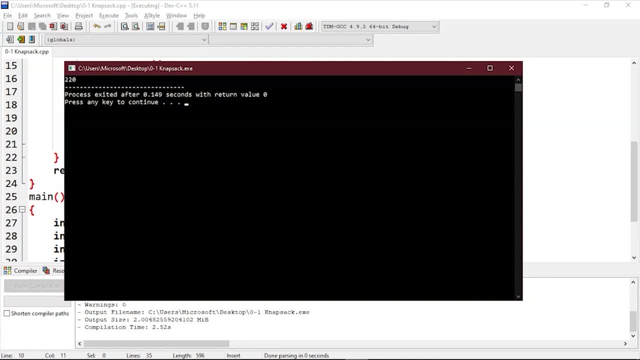 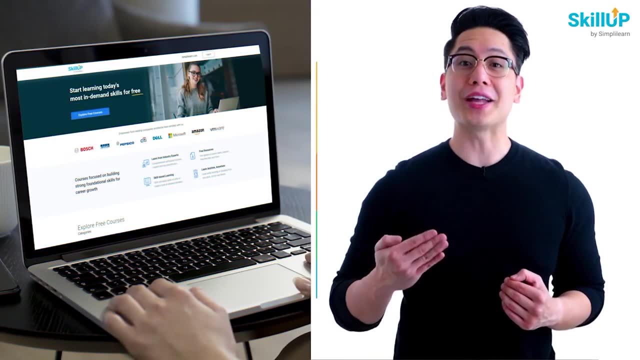 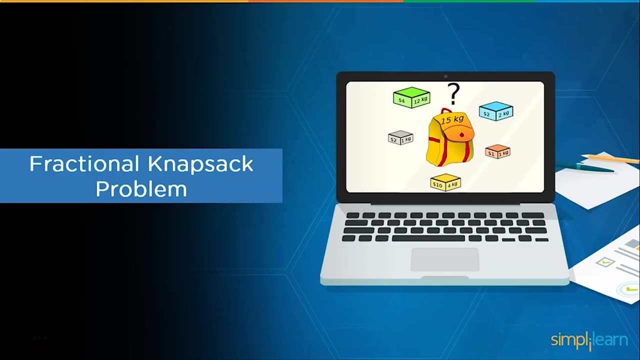 which comes out to be as 50. let's get back to our slides. if getting your learning started is half the battle, what if you could do that for free? visit, scale up by simply learn. click on the link in the description box below. link in the description to know more. we have now discussed 0: 1 knapsack problem. 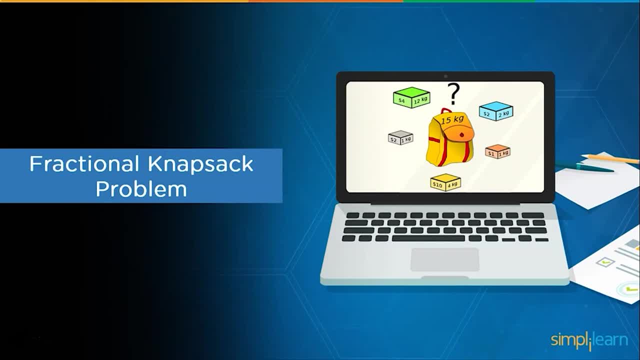 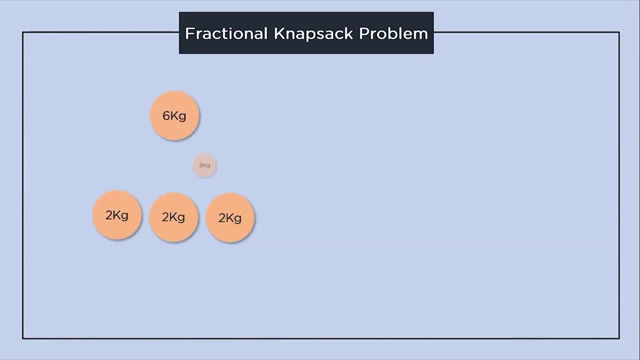 now let's discuss the fractional knapsack problem. similar to the 0- 1 knapsack problem, we will be given the weights and the value of n items, in this case 6 items. on the left we will also be getting a knapsack with capacity, W or in. 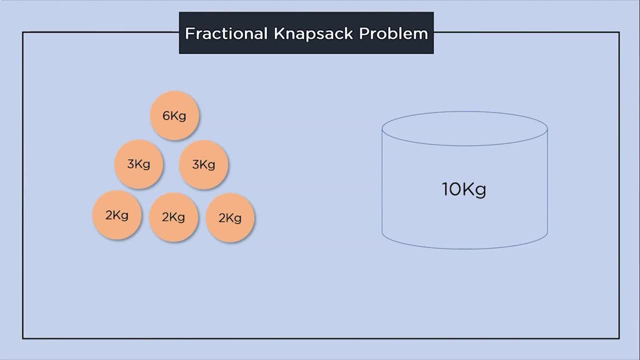 our case 10 kgs to the right. now we have to get the maximum total value in the knapsack. then we will have to keep filling this knapsack but unlike 0- 1 knapsack, we can break an item to get a maximum value of knapsack. 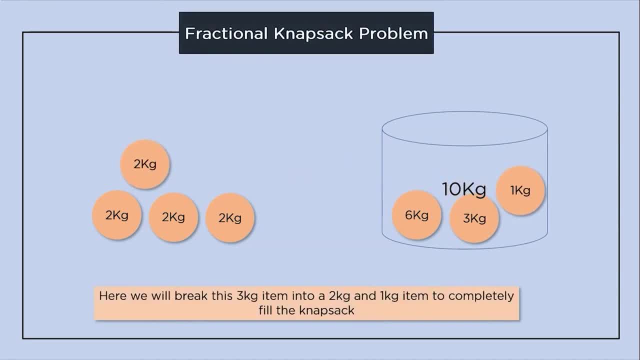 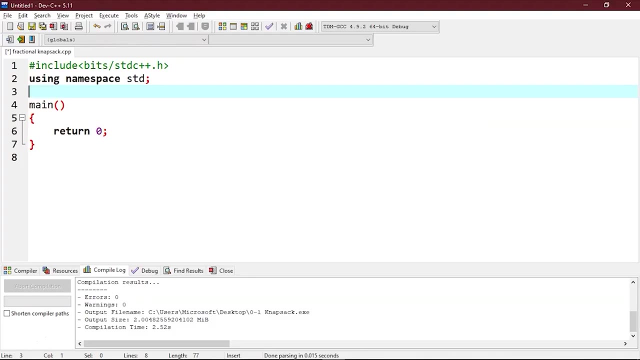 here we will break this 3 kg item into a 2 kg and 1 kg item to fill the knapsack. now let's try to implement this in the code editor. we will start with the structure for an item that stores weight and corresponding value of item. so 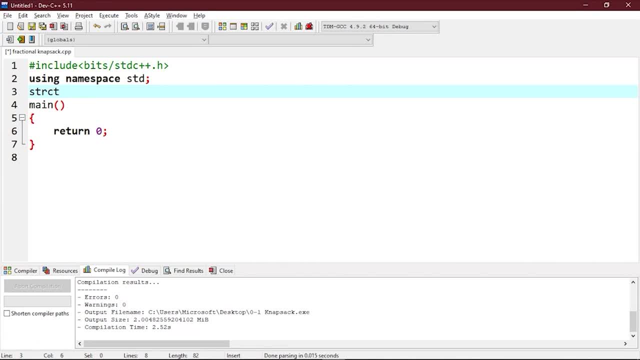 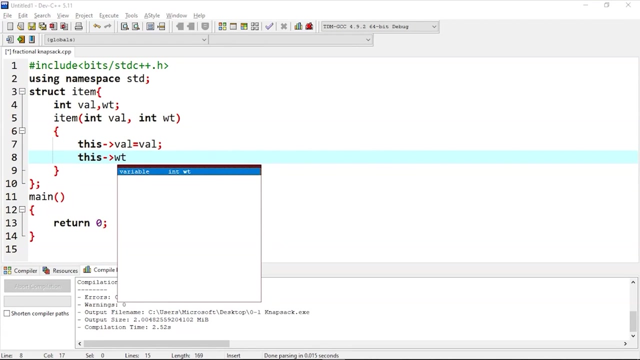 struct item: int value value- comma weight value- comma weight value- comma weight. we will write the constructor as item with argument as int var, as item with argument as int var, where this value will be equals to val and this weight will be equals to weight. Now we will write a comparison function to sort items according to value by weight ratio. 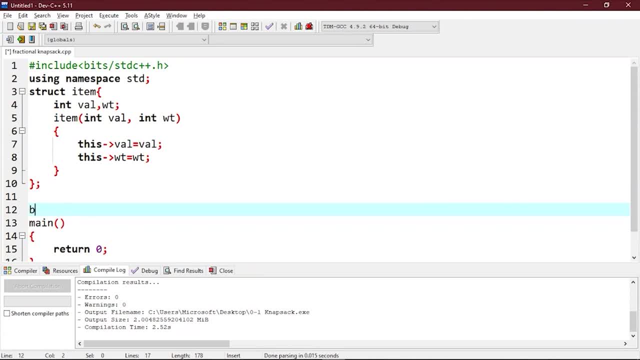 So Boolean function CMP with argument as: struct item A, comma, struct item B. Now level R1 is equals to double A dot value divided by double A dot weight. Similarly, we will write it double R2, which will be equals to double B dot value. 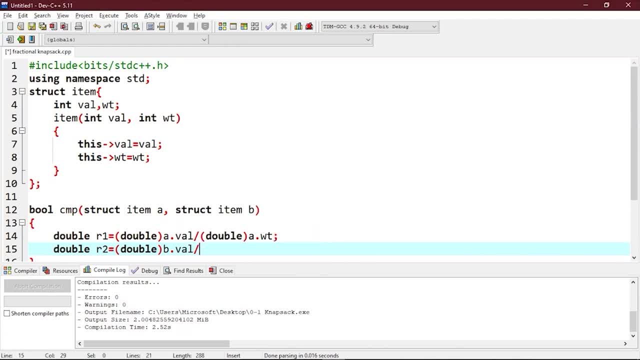 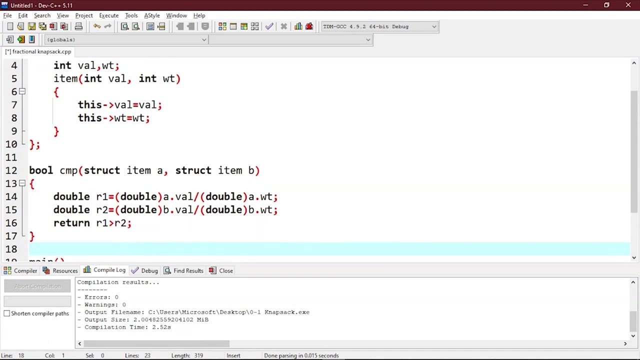 divided by double R2, E dot weight. Now we will return R1 greater than R2, which means it will return true if R1 is greater than R2.. Now we will write the main function to solve the problem. So double FNAPSEC. 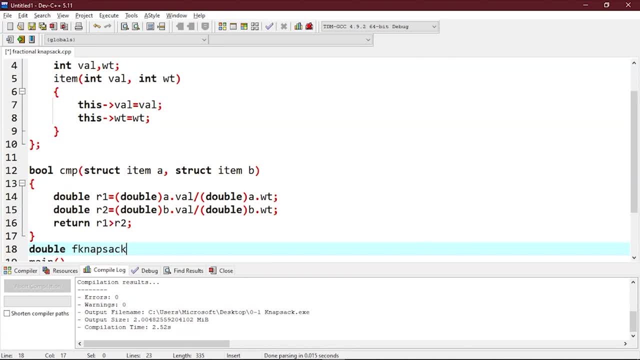 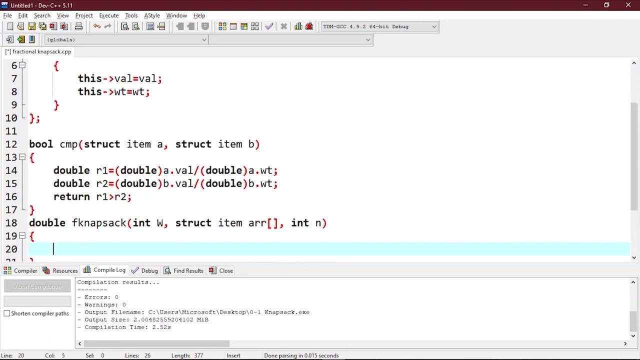 with argument: as int capital W comma struct item B, So double FNAPSEC. item ARR comma int N, We will first sort the item or the basis of ratio. So sort ARR comma, ARR comma int N. ARR plus N comma CMP. 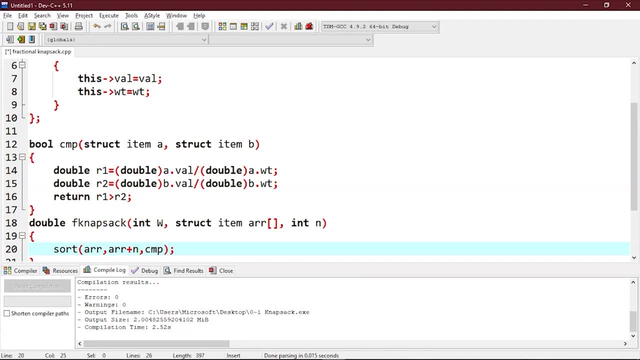 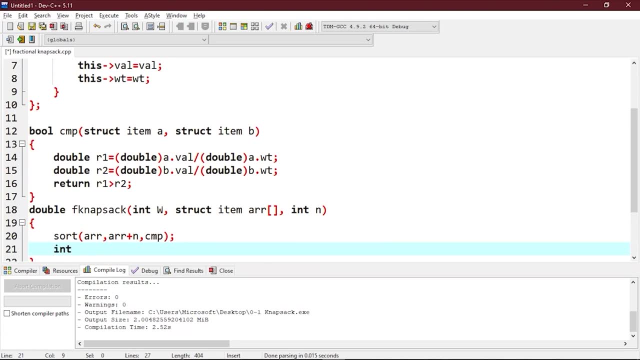 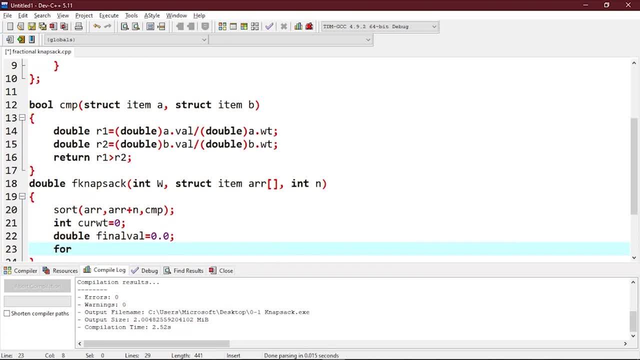 this will be result value in knapsack. this will be result value in knapsack. so for: and i is equal, and i is equal, and i is equal to zero, to zero, to zero where i is less than n, where i is less than n, where i is less than n, and i plus, plus. 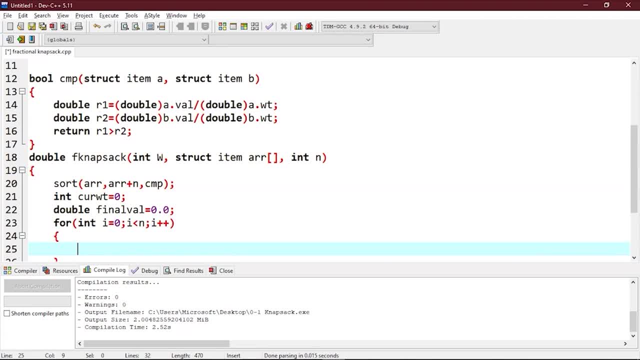 now, if adding the item won't overflow now. if adding the item won't overflow now, if adding the item won't overflow, then we will add it completely. so if current weight, current weight, current weight plus plus plus plus ar, ar, ar, ar at i at, i at i dot weight. 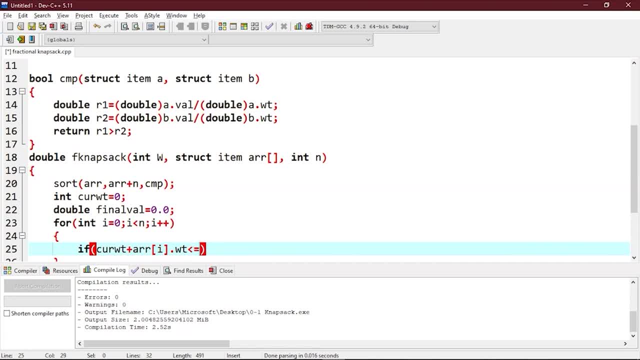 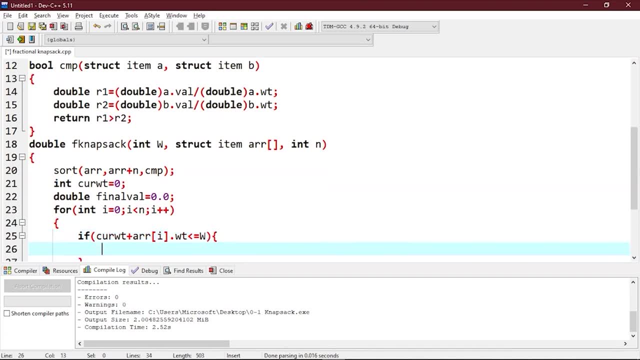 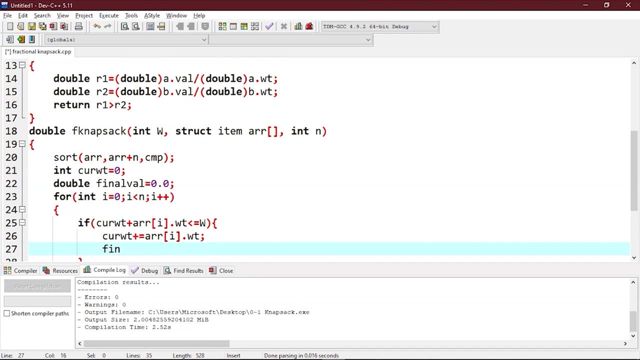 is less than is less than is less than equals to capital w, then then then current weight plus equals to, then current weight plus equals to, then current weight plus equals to arr dot weight and final and and final value will be plus equals to, and final value will be plus equals to arr at i dot value. and final value will be plus equals to arr at i dot value and final value will be plus equals to arr at i dot value. now, if we can't add a current, and final value will be plus equals to arr at i dot value now, if we can't add a current. 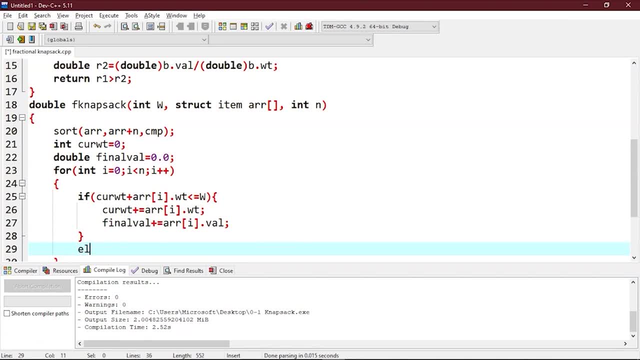 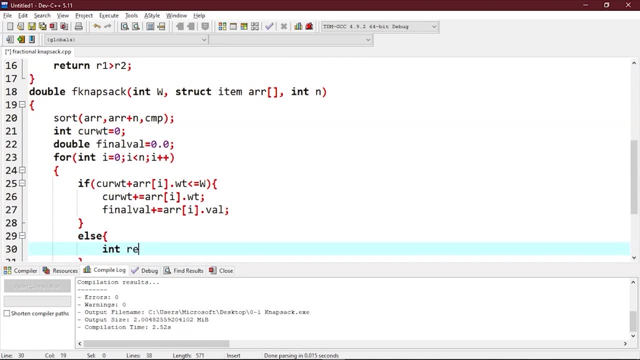 and final value will be plus equals to arr at i dot value. now, if we can't add a current item item, then we will add fractional part of it, then we will add fractional part of it, then we will add fractional part of it. so else, and and. 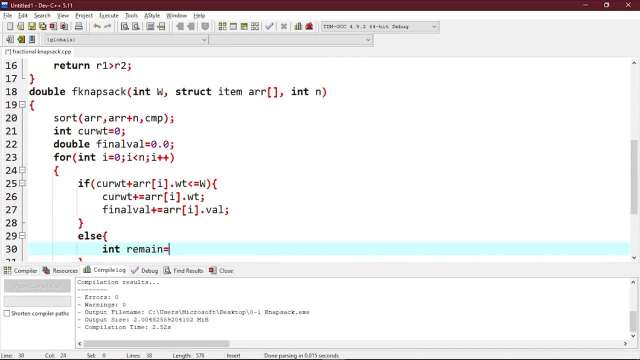 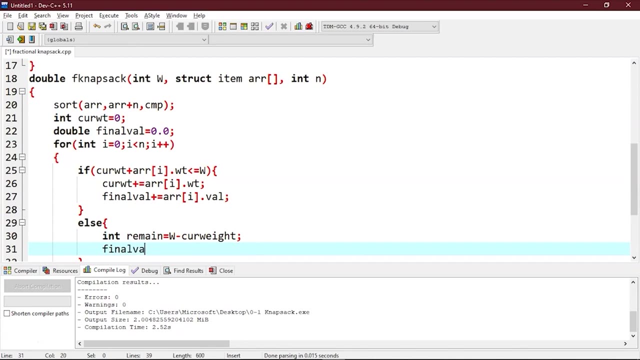 and remain is equals to w, is equals to w, is equals to w minus, minus minus current weight. then, then, then, final value, final value. final value will be plus equals to, will be plus equals to, will be plus equals to. arr at i dot value, arr at i dot value. 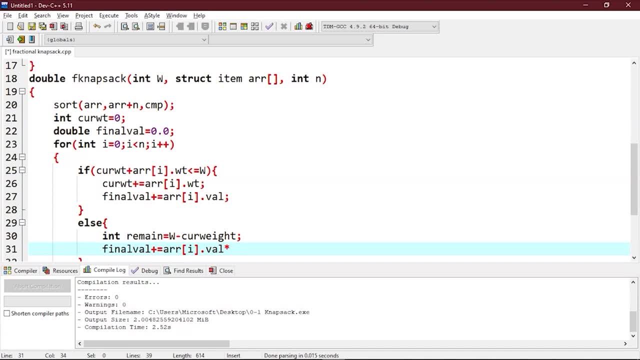 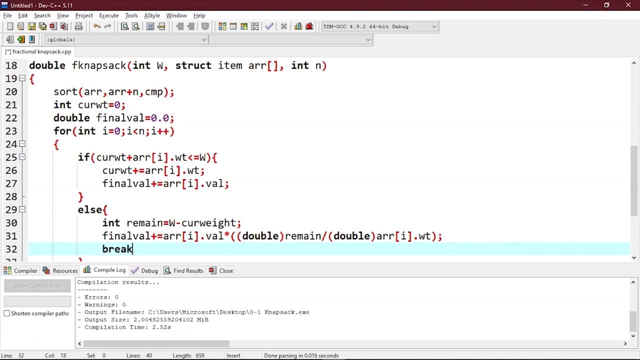 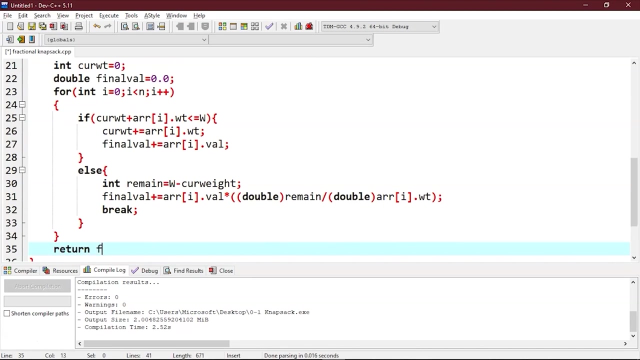 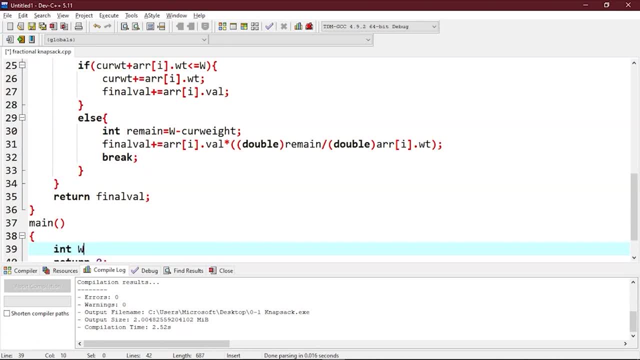 now let's write our main block. now let's write our main block. we will start with defining and we will start with defining and we will start with defining. and w equals to 50, w equals to 50, w equals to 50. this will be weight of the knapsack. 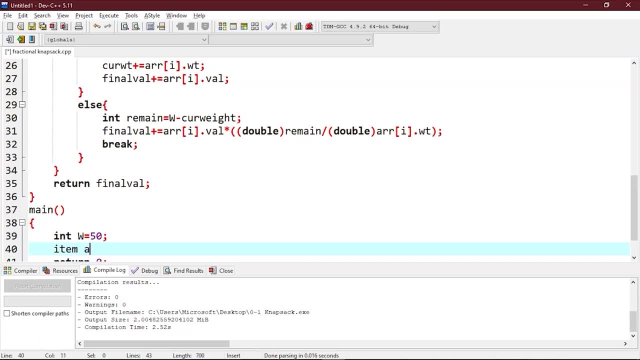 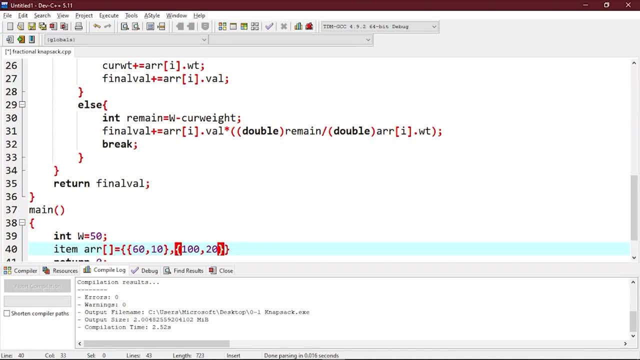 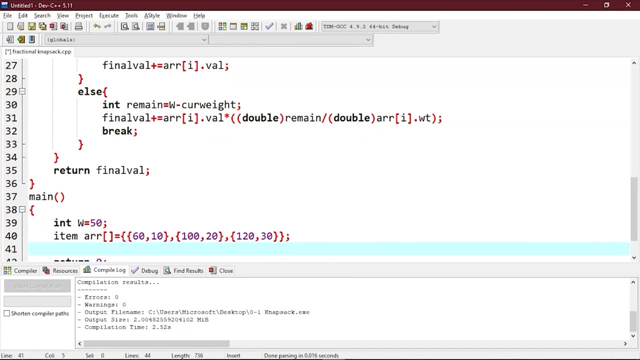 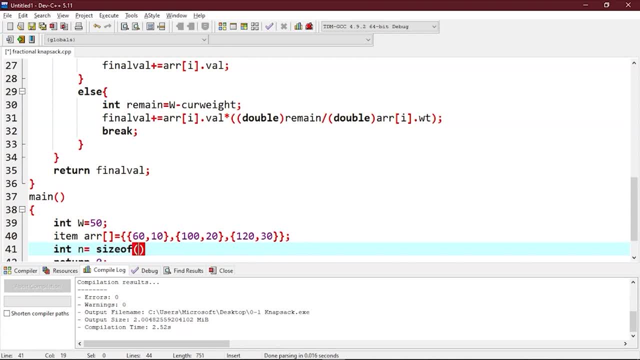 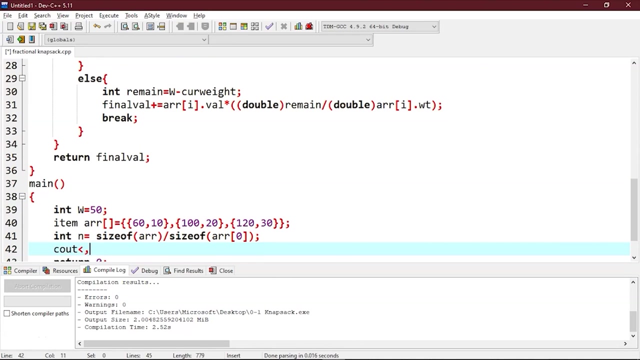 size of ar divided by a size of arr, arr, arr, arr, arr, arr at zeroth location. now we'll make that function call. now we'll make that function call. now we'll make that function call. so cout, so cout. maximum value will be obtained. FAPSEC. 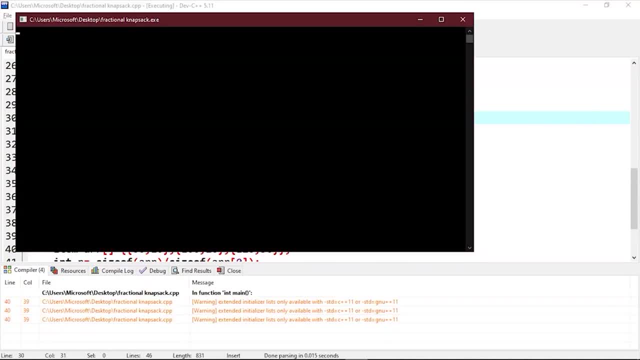 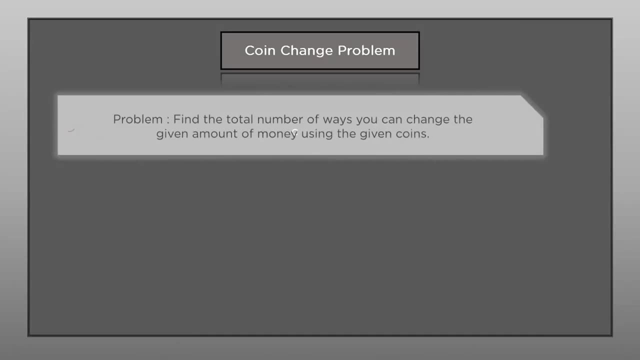 Let's execute this. As you can see, we are getting the maximum value as 240. That means our function is working flawlessly. The coin change problem is defined as the total number of ways you can change the given amount of money using the coins, And we are provided with different types of coins or 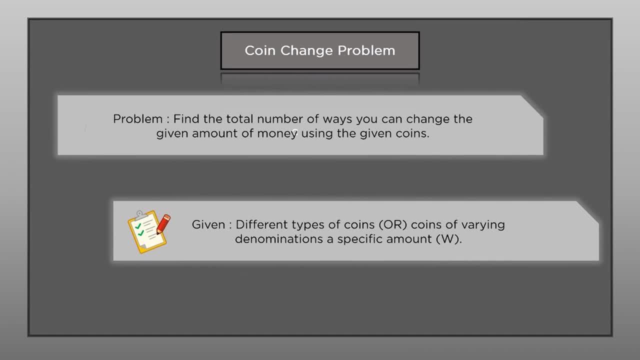 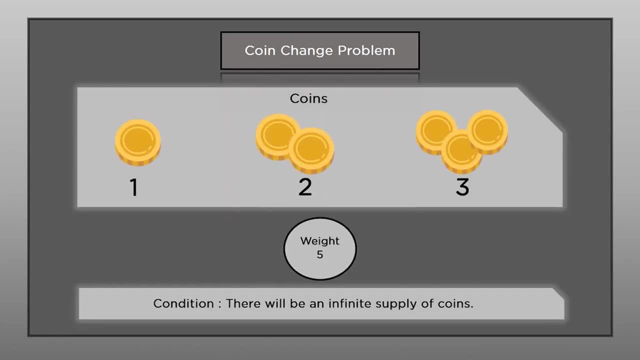 Coins of varying denominations and a specific amount, that is W. Let's look into an example. The denominations of the coins are 1,, 2 and 3, And 5 is the weight. So how can we achieve a weight 5 with 3 coins? There are number of ways to do this. First, we will need 5: 1 rupee coins. The second way to make 5 is to use 3: 1 rupee coins and 1, 2 rupee coin. The third way of doing it is using 2: 1 rupee coins and 1: 3 rupee coin. 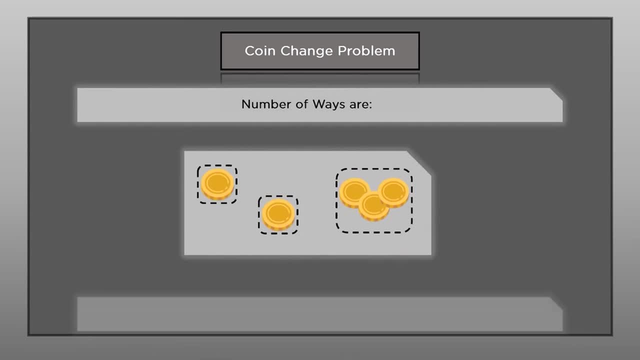 The fourth way is to use 1, 2 rupee coin and 1, 3 rupee coin. And the last way is using 1, 2 rupee coin and 1, 3 rupee coin. There is no other way to make the number 5 using 1,, 2 and 3 rupee coins. 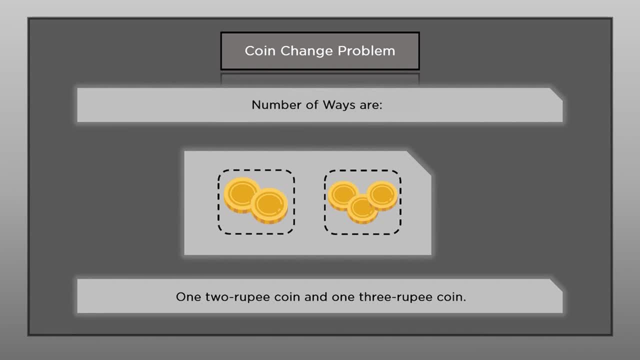 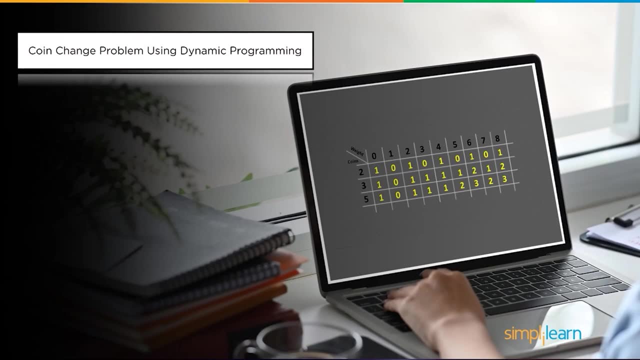 So in total we have 5 ways to make weight equal to 5 using these coins. Now we will see how dynamic programming can be used to solve the coin change problem. Let us suppose we have a different demonstration of coin as 2,, 3 and 5. 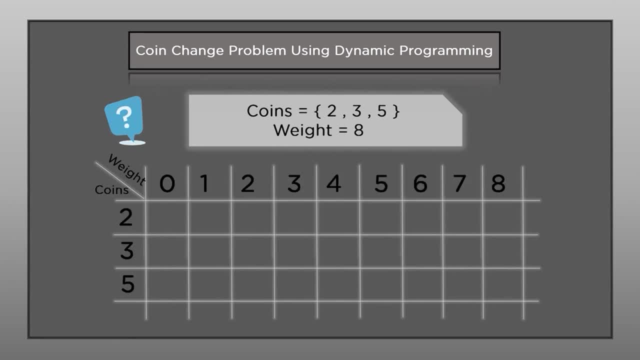 And we have to make the total sum weight as 8, With the same condition that we can use an infinite number of coin supplies. We must generate a table in the coin change problem using dynamic programming, Because we will store the results and use them later. So in this table, the column side will have coin values of 2,, 3 and 5. 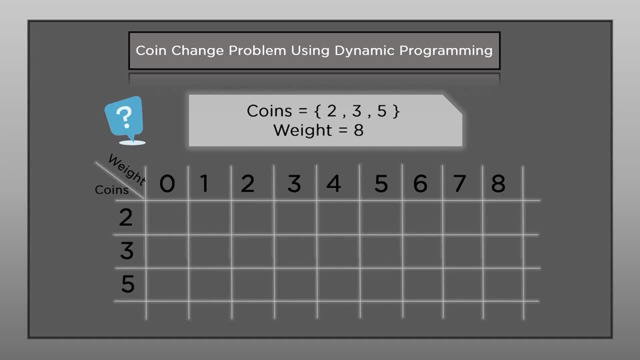 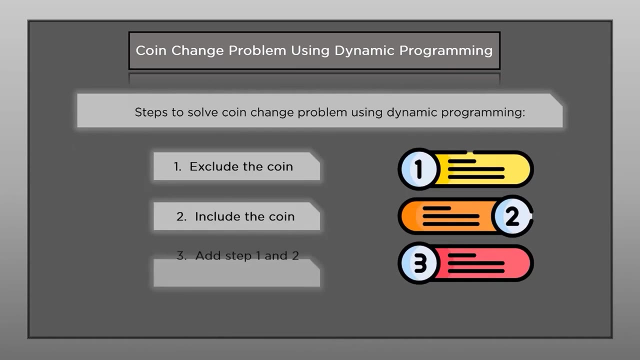 And the row will have to store the weight by dividing it into smaller weights, Because in dynamic programming we will divide problems into sub problems that are 0,, 1,, 2,, 3,, 4 until 8. Here are 3 simple steps of solving the coin change problem with dynamic programming. 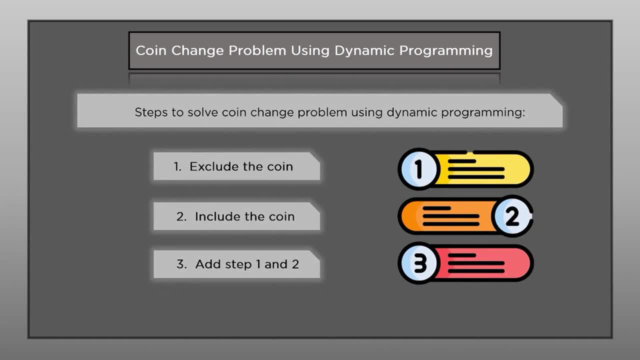 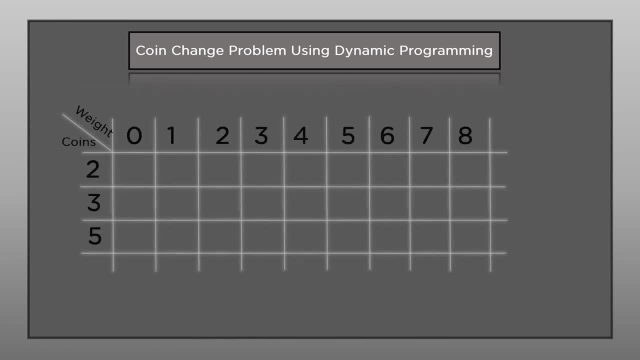 The first step is to exclude the coin, The second step is to include the coin And the final step is to add the first and second steps. Let us start with the coin of demonstration 2 And the sum is 0, So there is only one way to go. 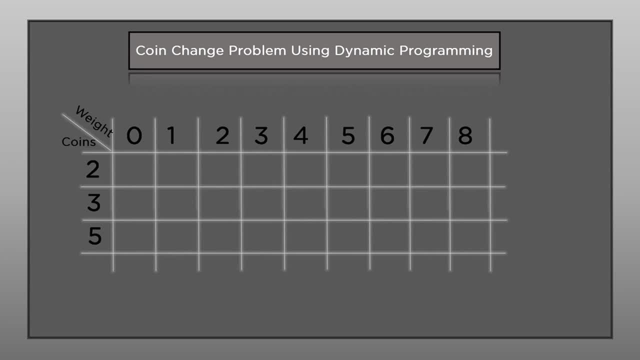 Because if we don't choose the coin value 2, We will obviously make sum or weight as 0, And the same goes for coin 3 and 5, So we will write 1,, 1 and 1 below the sum of 0, Now that the sum is 1. 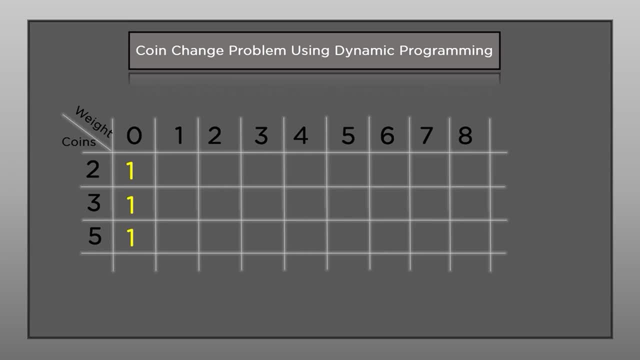 We can make it 1 using a coin value of 2. The answer is no. We can't make it 1 using a coin value of 2, So we will fill 0 in here. Next, we must make the sum 2 using 2 rupee coin. 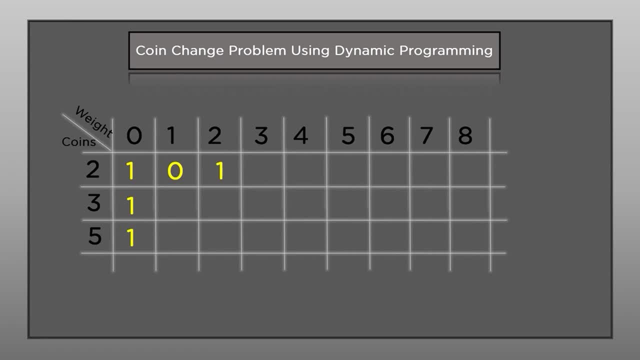 And there is only one way to do so: Use one 2 rupee coin. Next, we can make a sum of 3 using a coin of denomination 2. The answer is no, So we will mark this entry as 0. We can now make a sum of 4 by using a coin. 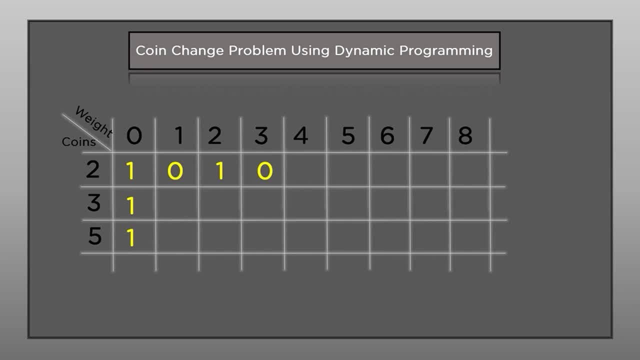 With a value of 2 rupee coins in only one way. So we will update 1 as the location changes. In the same way, we will update the entire row of coin denominations. 2, Now that we have a new coin with a denomination of 3. 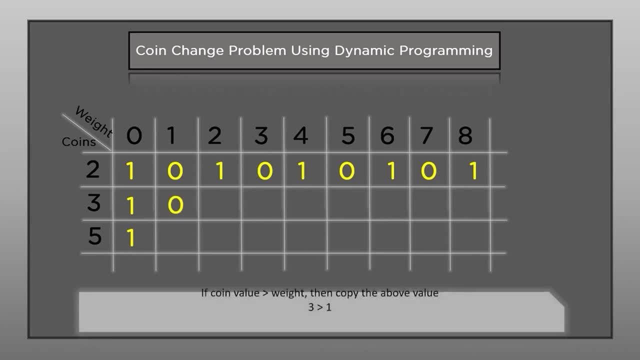 We will have one trick. If the coin value is greater than the sum, Simply copy the first values above. For example, if the coin value is 3 and the sum is 1, We will simply copy the value which is above, Which is 0. Again, the coin value is 3 and the sum is 0. 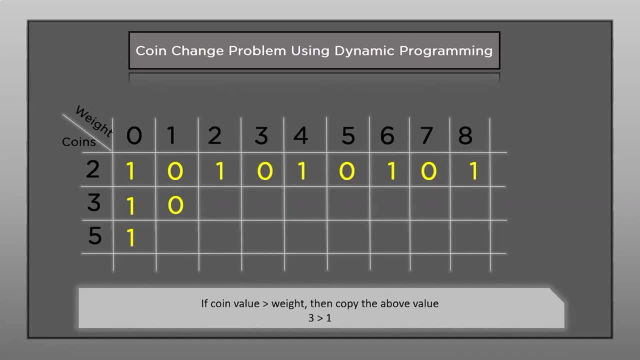 Which is less than the coin value. So we will simply copy the value above, which is 1. Next we have sum of 3 and coin value of 3 That is not greater than 3. We will now proceed with those simple 3 steps, If we exclude coin value 3. 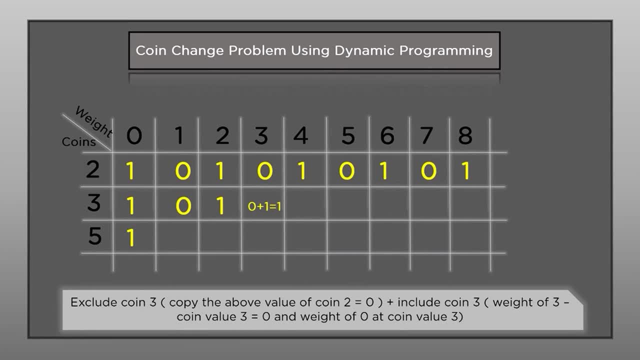 We simply copy the value above, which is 0, And if we exclude coin value 3, We subtract that same row, weight, That 3, with coin value. that is also 3, Which gives us 0, And what we have below weight 0 In the same row is 1. 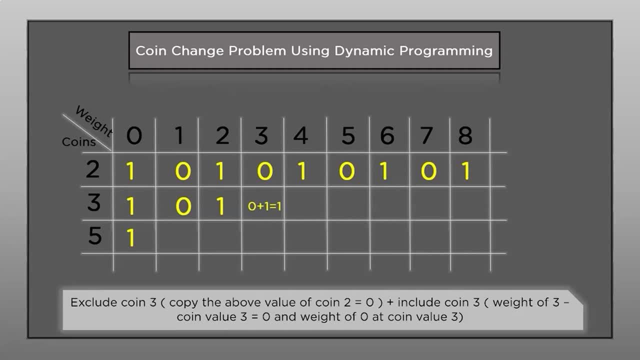 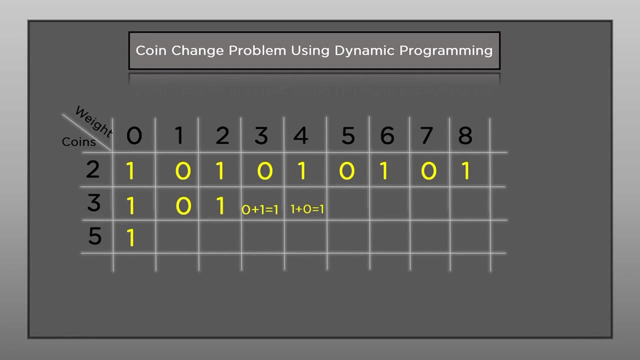 So we will add both values, that 0 and 1, Which gives us 1. Next, for sum 4, We exclude coin value 3. We must simply copy the value which is above, Which is 1, And by including 3 We must subtract the sum value, which is 4. 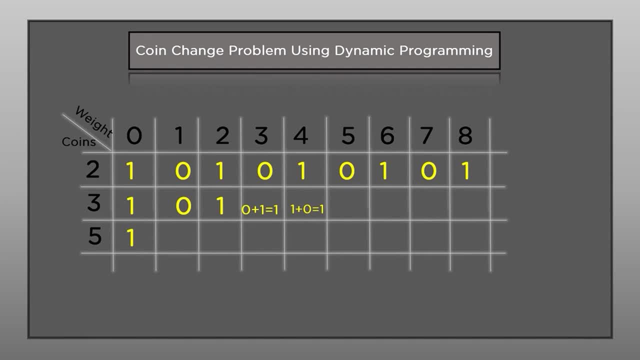 From the coin value, which is 3, Which gives us, And what we have below. sum 1, In the same row, is 0, So we add 0 and 1, Which is 1. So in the same manner We will fill out all the entries For sum 5,, 6,, 7 and 8. 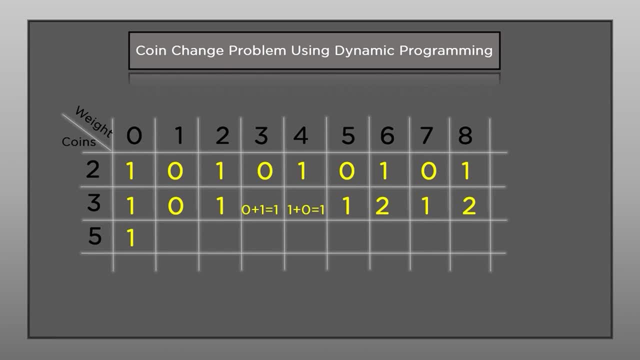 Of 3 coin denominations. Now that we have coin value 5, We use the same trick. If coin value 5 is greater than the sum of 1, Which is true, We simply copy the values which are lying above the row. So we have done for the first row, that is, 0. 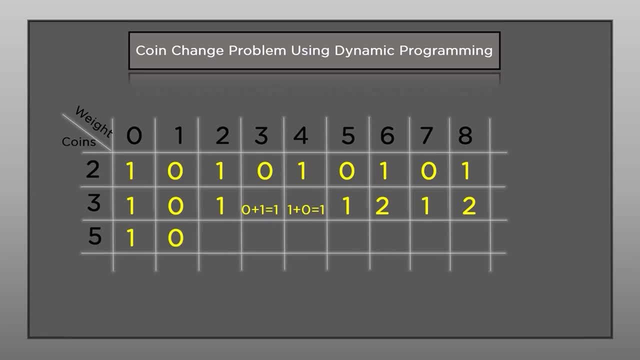 So by excluding coin value 5 And we are left with 2 and 3, And what we have of coin 2 and 3 In the same row is 0 And 1 and the sum of 0 and 1, Which gives 1. 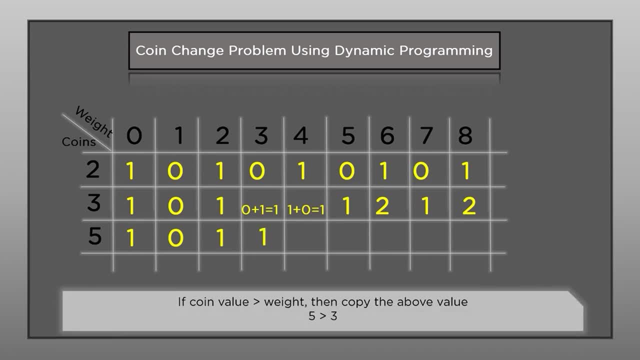 And by including coin value 5, We have to subtract sum to coin value 5, Which gives 0, And what we have below The sum of 0 of the same row, Which is 1. So 1 plus 1 gives 2. So we update the same. 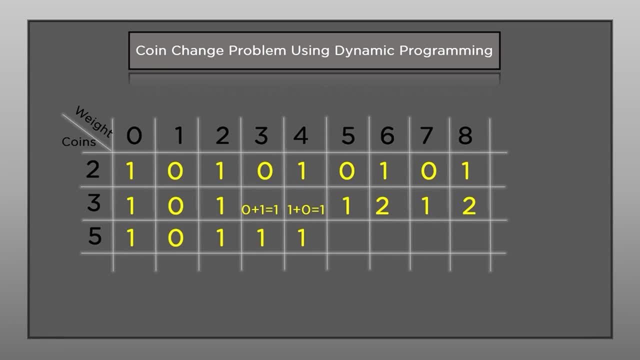 The sum is now 6 And the coin value is also 5. So if we exclude coin, The value 5, We are left with 2 and 3, And What we have of coin 2 and 3 Is the same row Is 1 and 2. 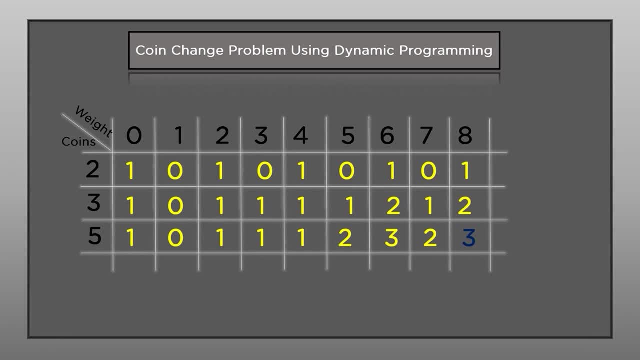 And the sum of 1 and 2, Which gives 3, And we include coin value 5. We have to subtract sum of 6 with coin value 5, Which gives us 1, And what we have below The sum 1 of the same row. 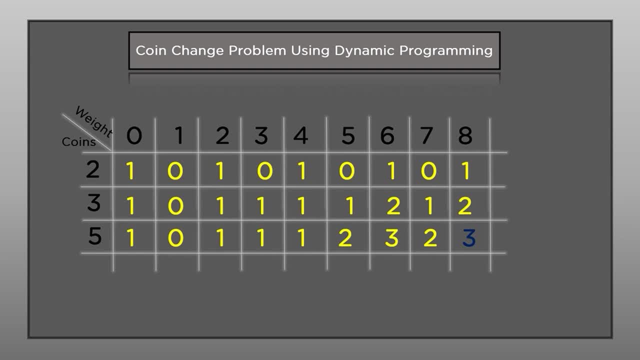 Which is 0. So sum of 3 plus 0 gives us 3 And we will update the same. So, in the same manner, We will fill out all the entries of Sums of 7 and 8 of 5 coin denominations. So in the end we got 3, which is our answer. 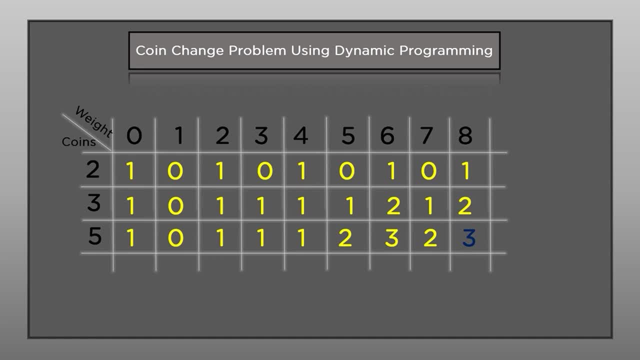 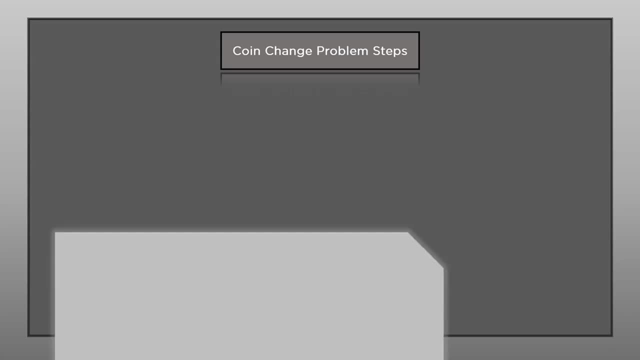 Indicating that we have a minimum of 3 ways To make the sum of 8 using Denomination coin value, which is 2,, 3 and 5. Now in this video, we will go over All the steps that we went to Solving the coin change problem. 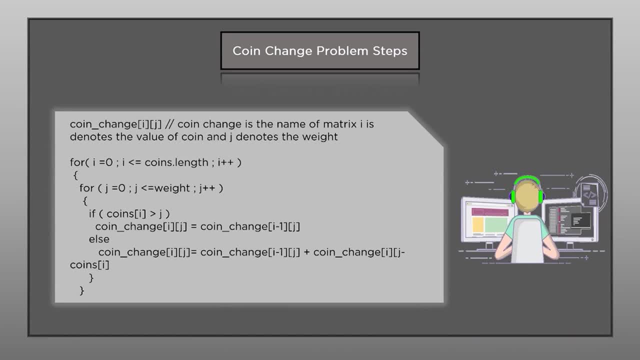 With dynamic programming. First we had a 2D array named coin change, Which has i as the number of rows And j as the number of columns. Now in this algorithm We will have Two for loops: One for i and another for checking The values of columns within i. 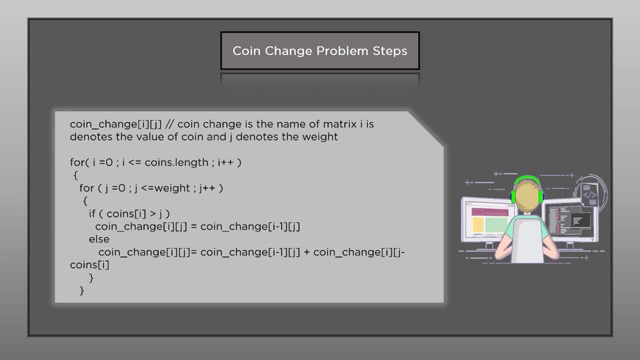 That is row. So the first loop runs from 0 To the maximum length of the coin, Which is the coin dot length, And the second loop runs for The first column to the weight. If coins of i Are greater than j, Then we simply copy coin change Of i of j. 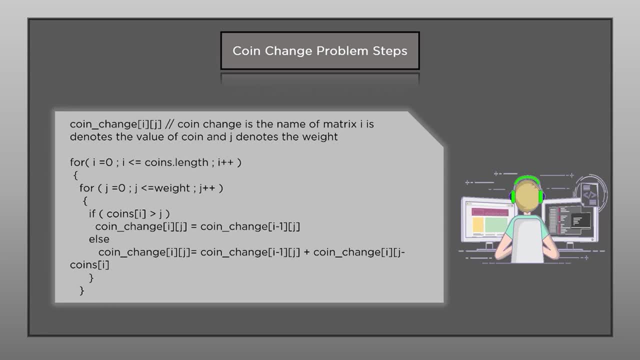 Is equal to the coin change If i minus 1 of j. Otherwise, we must apply The three step formula. Coin change of i of j Is equal to coin change of i minus 1 of j, Plus coin change of i of j minus coin of i. Lastly, 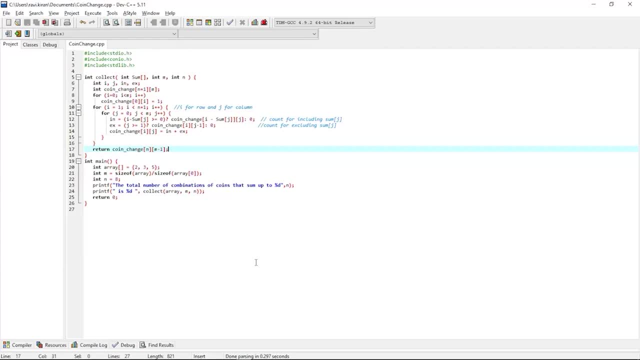 We will see the practical implementation. So on my screen You can see a program example For coin change problem. First we finished all the necessary Header files, Standard library, standard library strings, Which all the strings are defined, And console input output library. So first We have a function called collect. 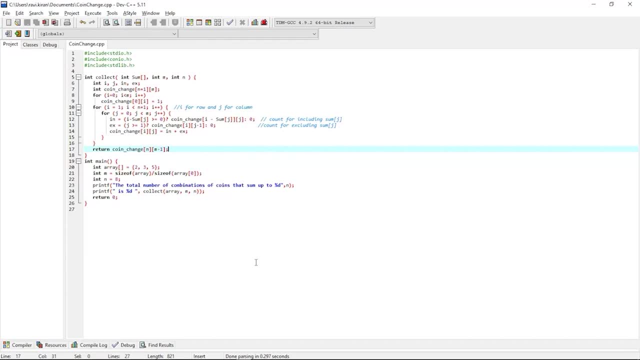 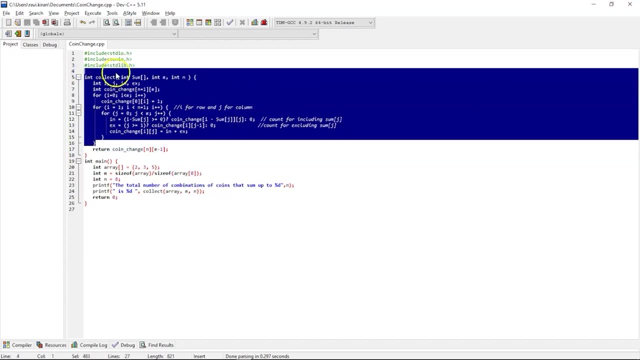 Which has an array Called sum and two variables Called m and n, For number of coins And number of weight. So this is our first function. So m is number of coins And m is number of weight. Then in this function We declared four variables, Two counter variables And in variable 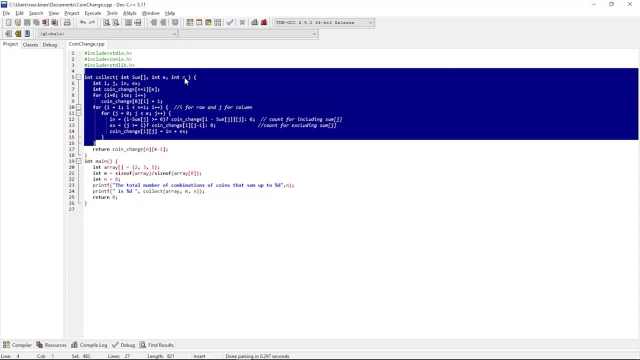 For including the coin value And x variable For excluding the coin value. Then we declared our 2d array, Which is a coin change array In which we need n plus 1 rows Because the coin change Is built from the bottom Of using base case 0. 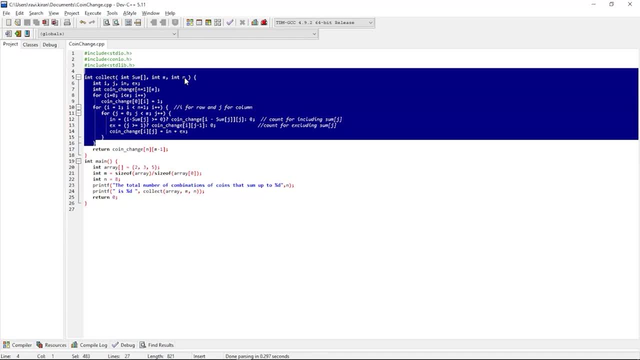 Next we have two for loops For the coin length is reached And another for column That will run until the sum or weight Is reached. In this for loop We will first include the coin value j. We get the value after Substracting the j value from the coin value i. 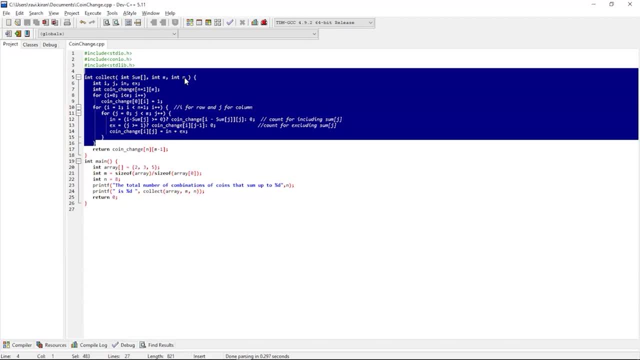 If the coin value i Is greater than 0, We simply assign the coin change Of i minus the coin change Of the same column. If we exclude the coin value from this, We have the condition that If the coin value is greater than 1, We assign coin change. 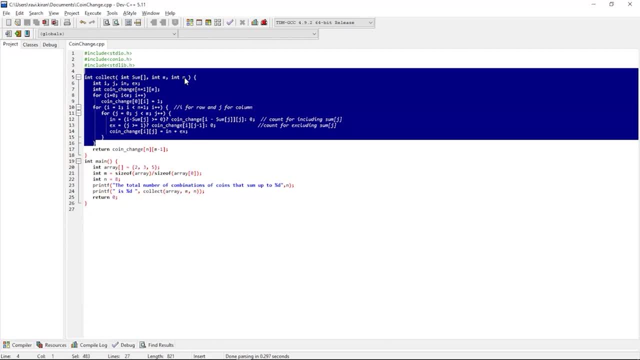 Of i of j minus 1, Otherwise we assign 0. Alternatively, Simply return the coin change From n of m minus 1. Next we have the main function, In which we declare The array of coin values And assign the coin values of 2,, 3 and 5. 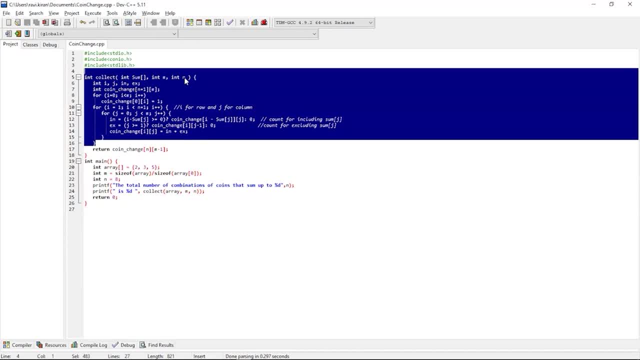 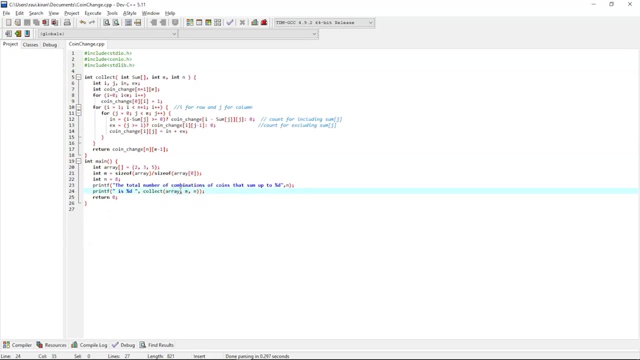 Then we have the same m variable In which we divide the Coin, and then we have The variable n in which we have Sum as 8, and finally We print the total number of coin combinations. That sums up. Now let's quickly execute This program and see the output. 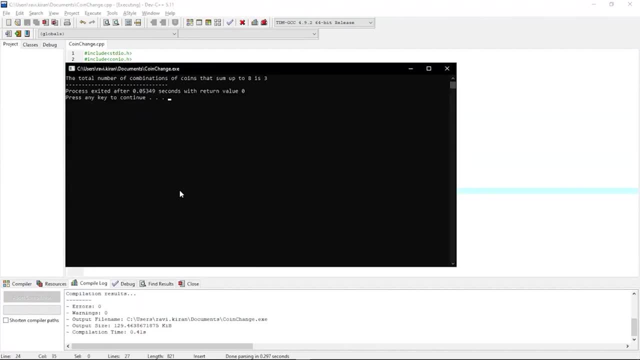 So there you go: The program got successfully executed And we have the output over here, And this example We considered is the same Which one we have discussed before, And the final value is 3. That you can see over here And you can see the answer as The number of coin combinations. 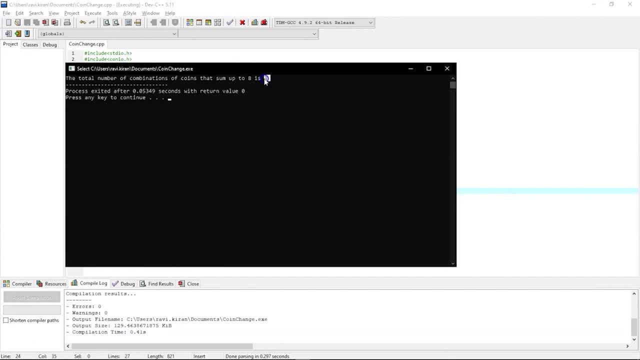 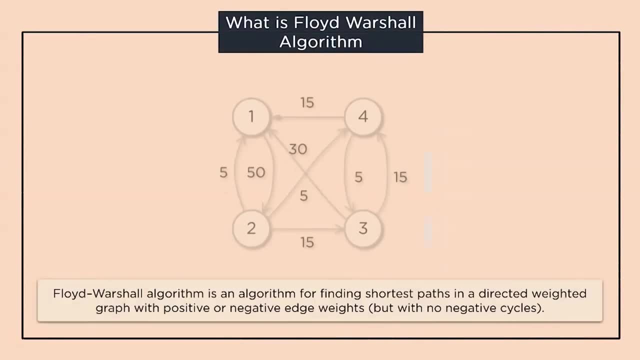 That sums up to 8s3. Let's get started with the topic. What is the Floyd-Warshall algorithm? The Floyd-Warshall algorithm Is for solving the all pair Shorted path problem. The problem is to find The shortest distance between Every pair of vertices. 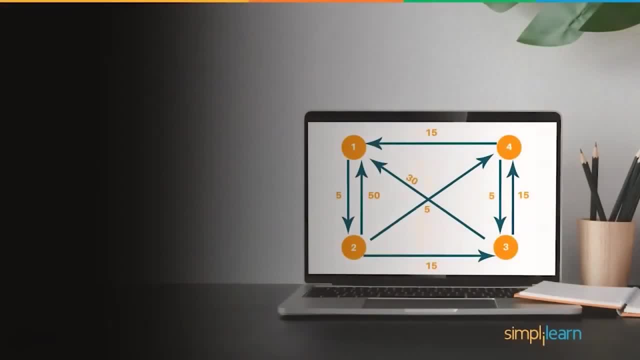 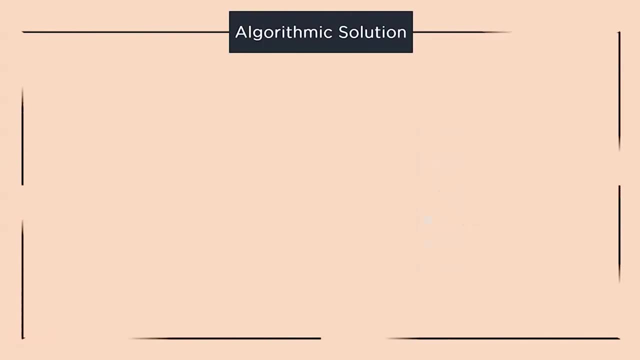 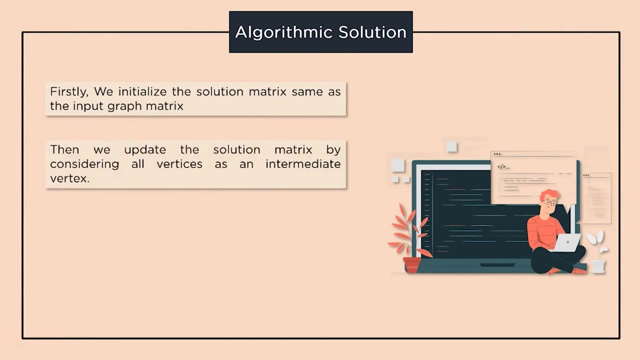 In the given edge weighted Directed graph. Now let's discuss the algorithmic Of all pairs: shortest path problem. First We will initialize the solution matrix, The same as the input graph matrix. Then The solution matrix is then Updated by treating All vertices as intermediate vertices. Our main goal. 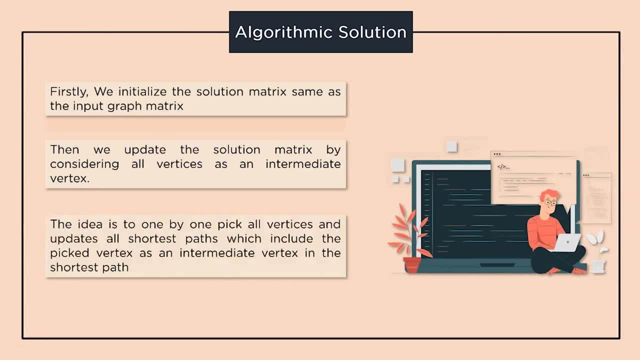 Is to pick All vertices one by one And update all shortest paths. That involves the picked vertices As intermediate vertex. We have now discussed The Floyd-Warshall algorithm And the algorithmic solution To all pairs shortest path problem. Now Let's implement this solution In the code editor. 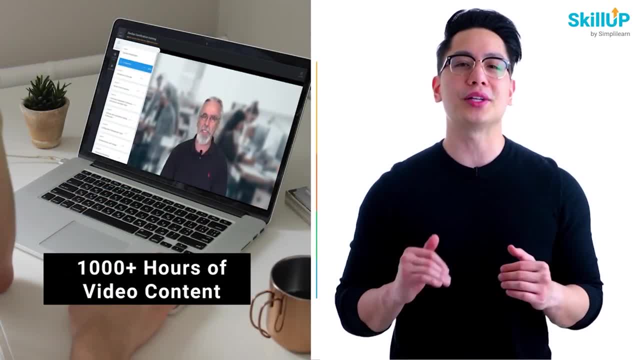 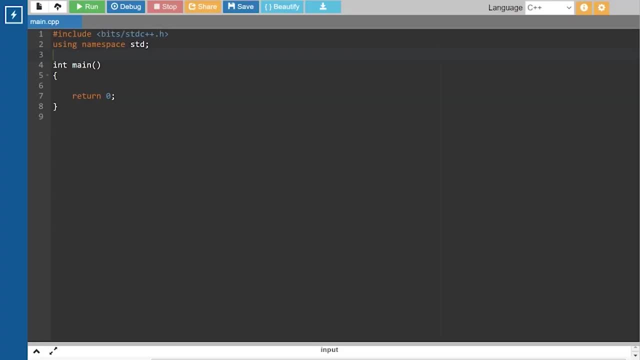 Choose from over 300 in-demand skills And get access to 1000 plus hours Of video content for free. Visit skillup by simply learn. Click on the link in the description To know more. We will start by defining vertices. We will have 4 vertices, So hashtag define. 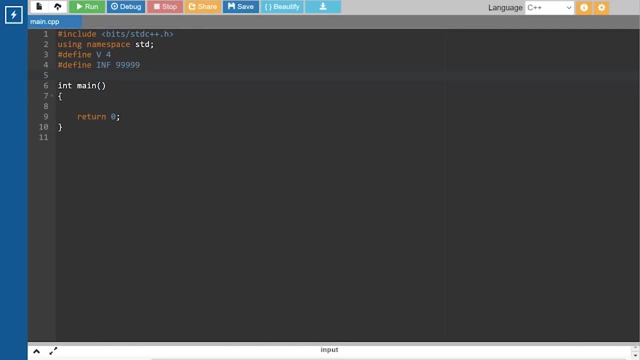 Inf, which will be equal to 9999. Now Let's write a function To print the solution matrix. So void print Solution With the argument as Int. Two-dimensional array List With its y as v. We will Come back to its definition later on. Now We will write a function. 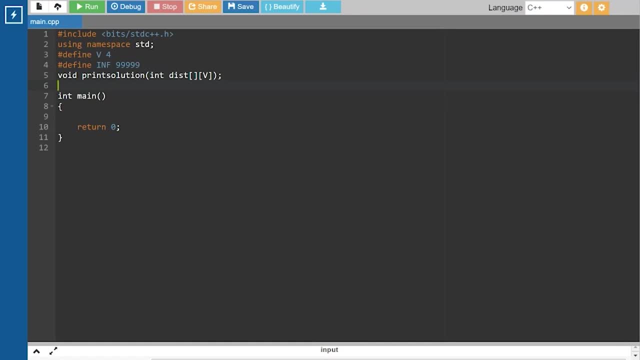 To solve the pair shortest path problem Using Floyd-Warshall algorithm. So void Floyd-Warshall Int graph. This will also be the 2D array Which has y as v. Now we will define Dist 2D array. It will be the output matrix That will finally have the shortest 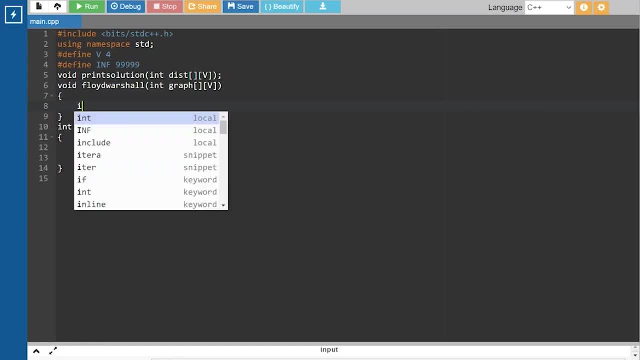 Distances between every Pair of vertices. So int Dist It's x and y Will be Vijk Vijk. Now we will Initialize the solution. matrix- Same as input graph matrix Same as input graph matrix. Or we can say that the initial value Of shortest distance are based. 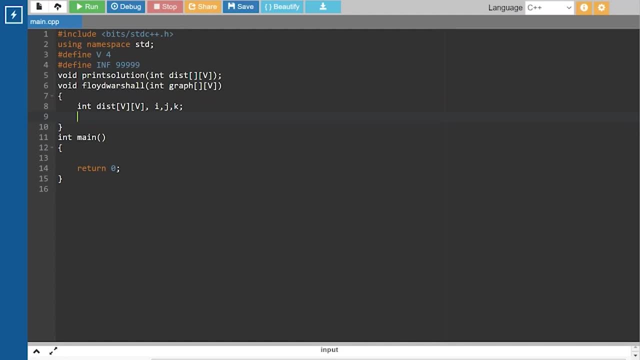 On shortest path, considering No intermediate vertex. So for I is equal to 0, I less than V, I plus plus Another nested loop: For j is equal to 0, J less than v, J plus plus So distance At i comma, j Will be Equals to Graph at i. 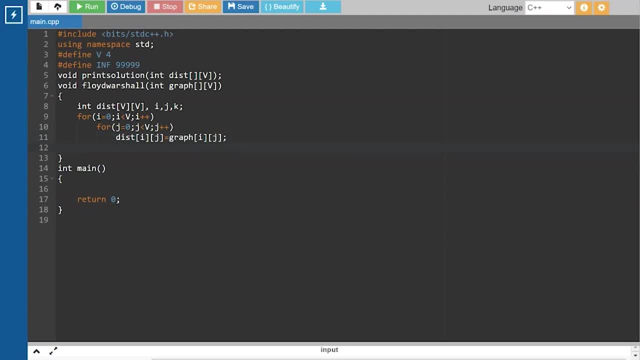 Comma j. Now we will add all vertices One by one to the set Of intermediate vertices. So before start of an iteration We will have the shortest distances Between all pairs of vertices, such that The shortest distance considering All the vertices is set From 0 to k minus 1. 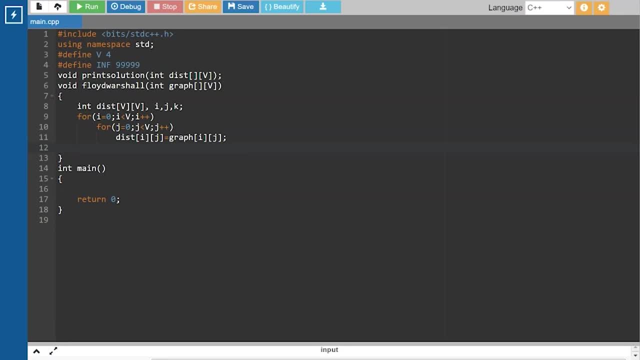 As intermediate vertices, And after the end of An iteration vertex, number K is added to The set of intermediate vertices And the set becomes From 0 to k. So for loop K is equal to 0, K less than v, K plus plus. Now we will pick all vertices. 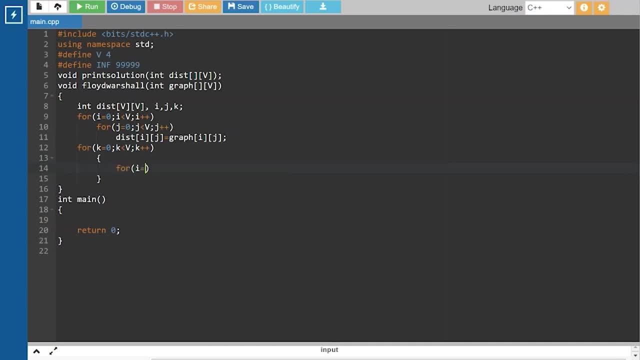 As source for one by one, I is equal to 0 I less than v I plus plus Now. we will pick All vertices as destination For the above picked source. So for j is equal to 0 J less than V, j plus plus Now. if vertex k 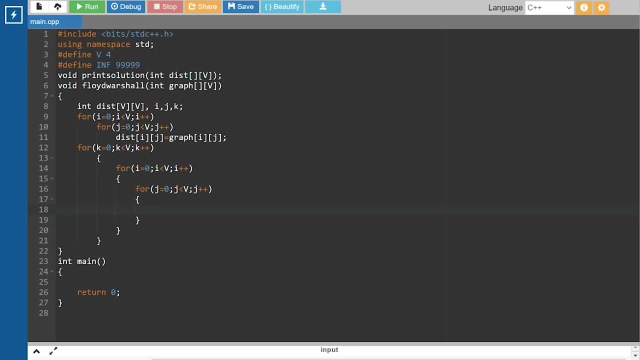 Is on the shortest path From i to j, Then we will update the value of Distance i comma j. So if distance At i comma j Is greater than Distance At i Comma k Plus distance At k Comma j, And Distance At k Comma j Is not. 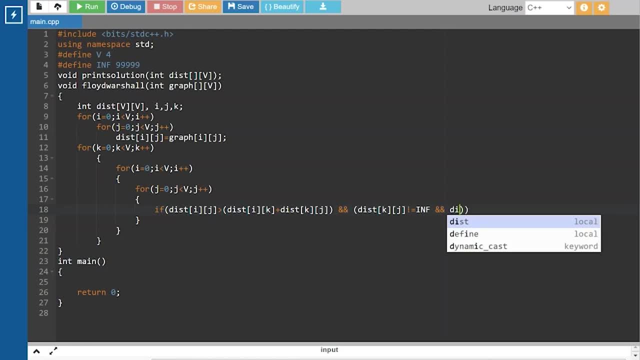 Equals to i and f And Distance At i Comma k Is also not Equals to i and f, Then Distance Will be equals to Distance At i Comma k Plus Distance At k Comma j. Now we will call The print solution function For test. Now lets write. 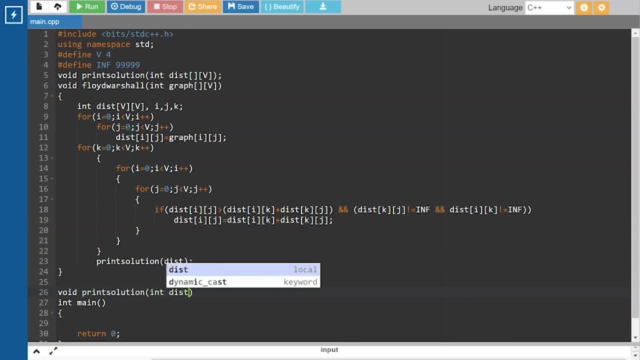 So void print solution And test. We will start with. See out. the following Matrix will show The shortest Distance between Every pairs Of vertices. For loop and i is equals to 0- i less than V. i Plus plus. for loop And j is equals to 0- j less than. 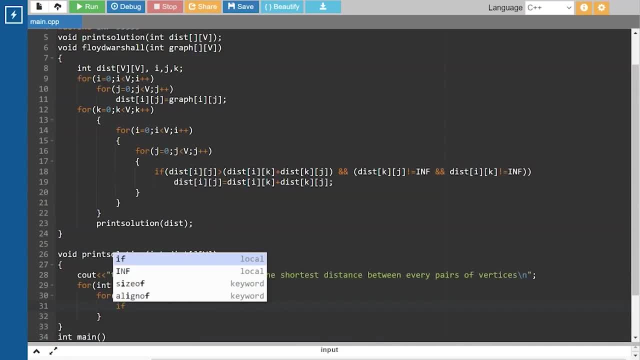 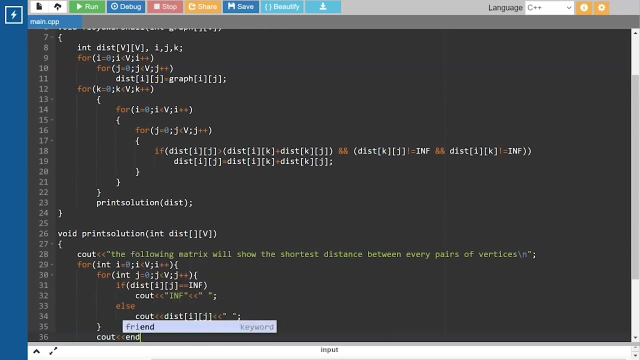 V, j plus plus. If Distance at i, comma j Is equals to i and f, Then we will see out i and f. Else We will see out the distance At i, Comma j. Now we will see out And l. this will change the row For the matrix. 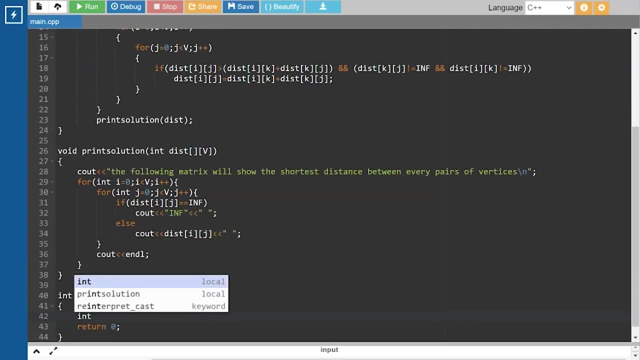 Now lets write the main block. We will define the matrix As: int Graph V, comma v, Which will be equals to 0. comma 5, Comma i and f. Comma 10: Next row: i and f. Comma 0. Comma 3. Comma i and f. 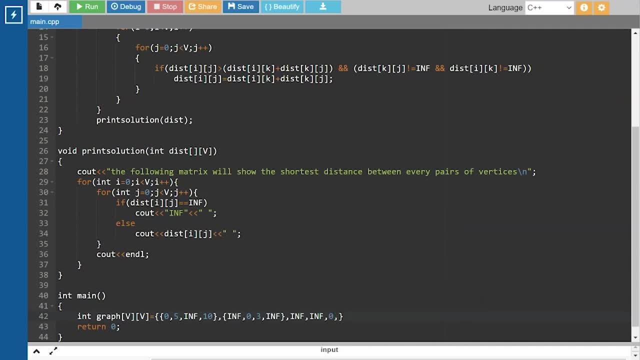 Next row: i and f, Comma 0, Comma 1. Last row: i and f, Comma i and f, Comma i and f, Comma 0. Now we will call the floyd warshell function, So floyd warshell For argument graph. Lets execute this. 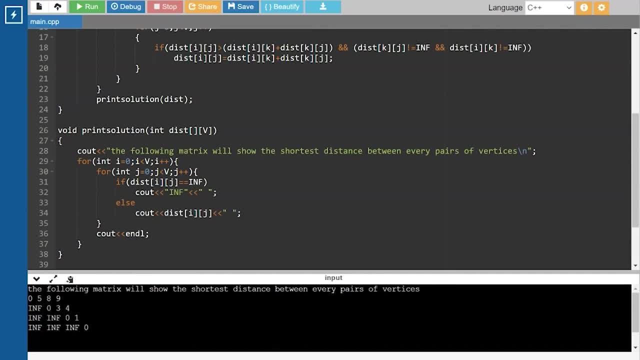 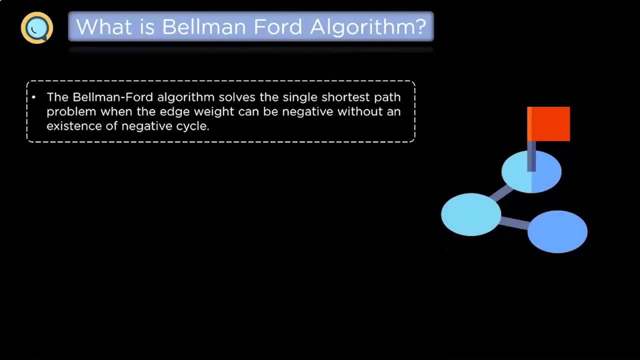 As you can see, we are getting an updated matrix Which shows the shortest distance Between every pair of vertices. So This algorithm Solves the single shortest path problem. When the edge weight can be negative Without a negative cycle, When some of the edges of the dedicated graph Have negative weight. 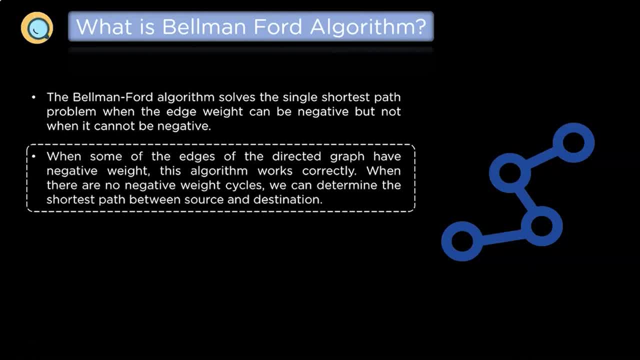 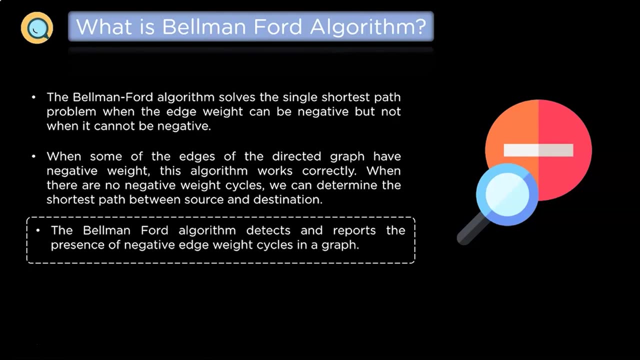 The algorithm works correctly When some of the edges of the directed graph Have negative weight. This algorithm works correctly When there are no negative weight cycles. We can determine The shortest path between source And destination. Bellman ford algorithm detects and reports The presence of negative edge weight cycles. 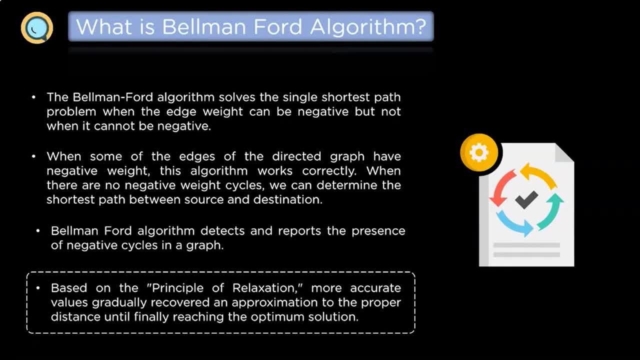 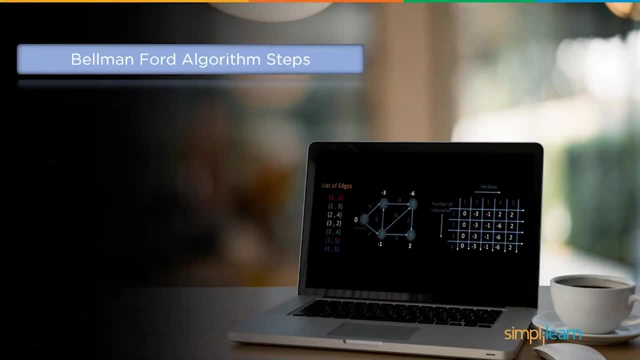 In a graph Based on the principle of relaxation, More accurate values gradually recovered, An approximation to the proper distance, Until finally reached The optimum solution. After understanding what exactly is Bellman ford algorithm, We will now look into some of the steps Followed by the bellman ford algorithm. 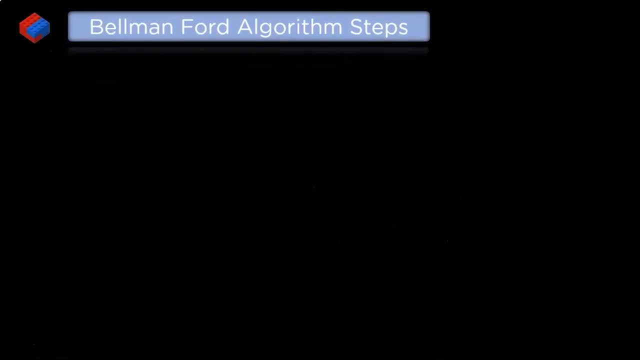 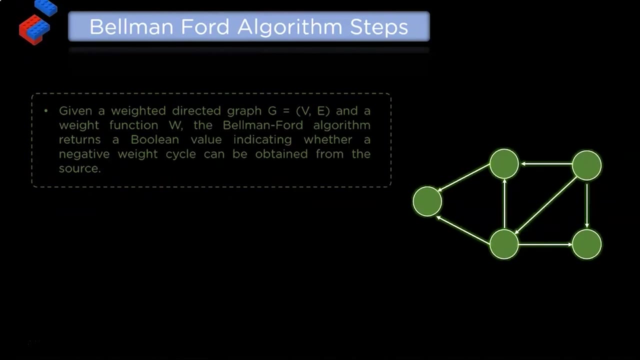 But let us look at One scenario. Given a weighted directed graph, G is equal to V comma e, that is, vertices and edges, And a weight function W, The bellman ford algorithm returns A boolean value indicating whether A negative weight cycle Can be obtained from the source or not. 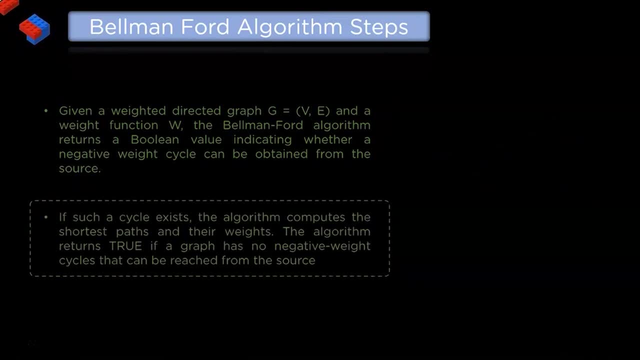 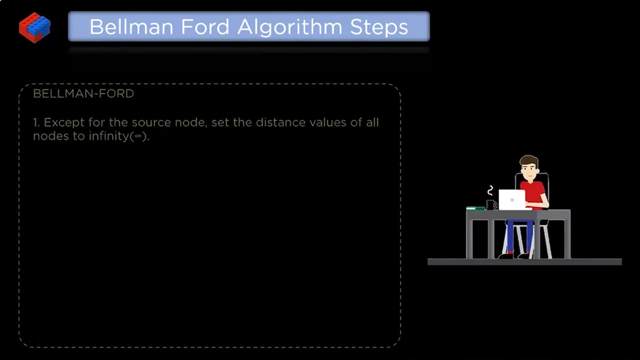 If such a cycle exists, The algorithm computes the shortest Paths and their weights. The algorithm returns true If a graph has no negative weight cycles, That can be reached From the source. Let us start with the bellman ford steps For the algorithm and see how it works. Set the distance values. 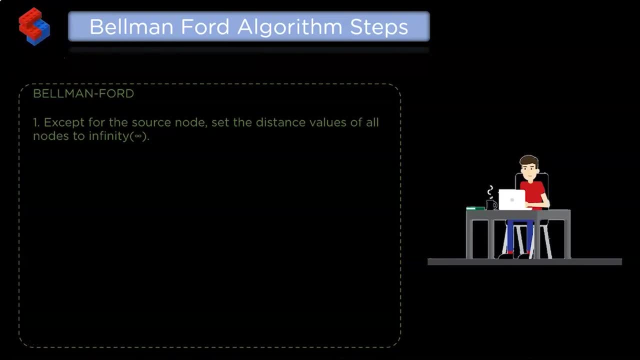 Of nodes to infinity, Except the source node. In the first we must repeat The relaxation step V minus one times, Where V is the number of vertices. So if we have an edge From U to V, Where U is the source node And V is the destination node, Then V will be updated with a new distance value. 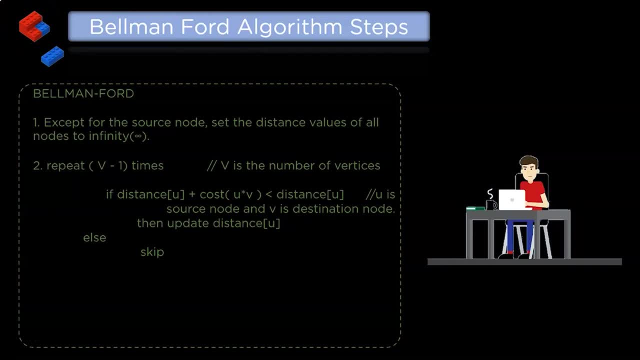 If the distance of U Plus the cost of the edge U- V is less than the distance Of V node. Otherwise we will not update it And we will skip it. All vertices should be relaxed Once more. We have a negative edge weight cycle If we find a new, shortest distance value. 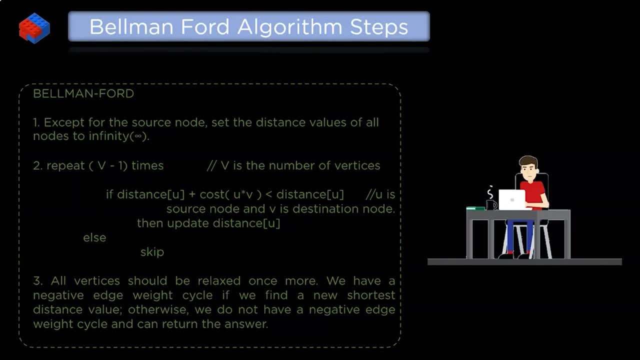 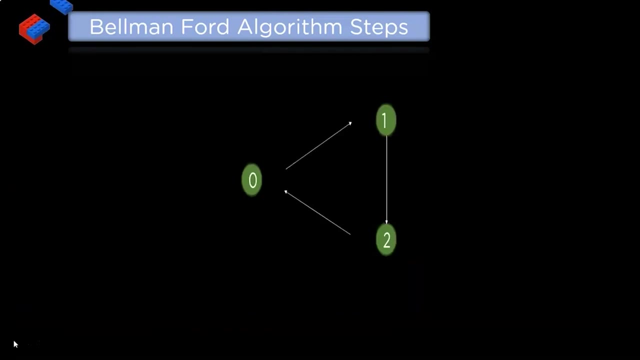 Otherwise, We do not have a negative edge weight cycle And can return to the answer In the last step. We have heard that The bellman ford algorithm Is used to detect a negative edge weight cycle In the graph for a long time. Let us see How the bellman ford algorithm 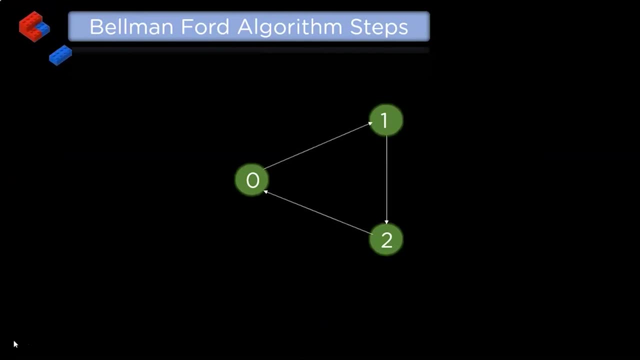 Detects a negative edge weight cycle In the graph. Let us assume that we have a graph With three vertices, with initial value As infinity as the weight of the graph. Because this graph has three vertices, We will relax it V minus one times, That is, two times In the first time of relaxation. 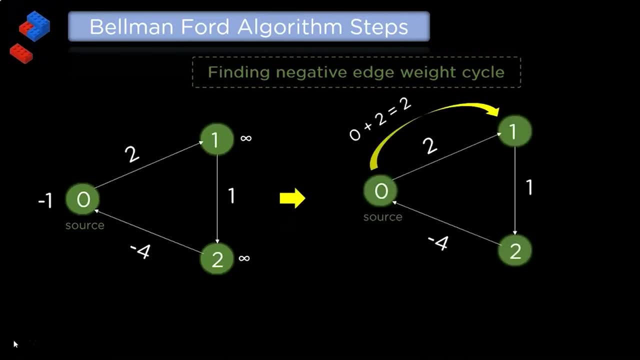 The weight from zero to one Is two. So the cost of zero to one Will be Zero plus two, Which is equal to two. So because two is less than infinity, We will replace infinity by two. Now, From one to two, The cost will be two plus one, Which is three. 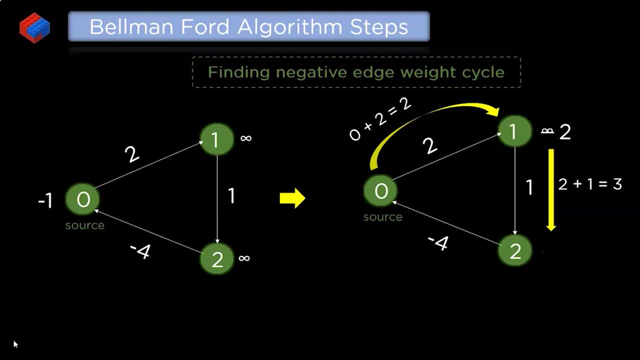 Which is less than infinity, So that we will replace by infinity By three. Two to zero, The cost will be Three plus minus four, Which is equal to minus one, And as we know that minus one Is less than zero, We will replace it two In the second time of relaxation. 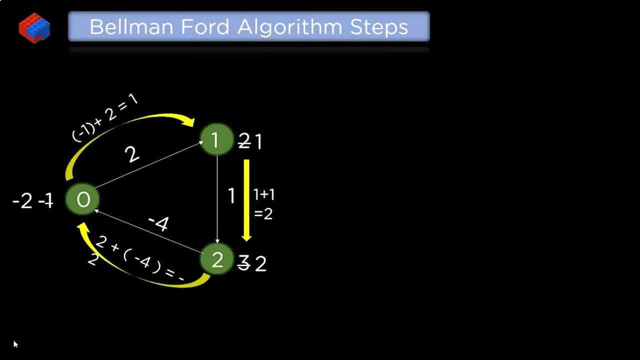 The weight from zero to one Is two. So the cost from zero to one Will be minus one plus two, Which is equal to one, And one is less than two. So we will replace Two by one. Now, from zero to one, We have the weight as one. The cost will be one plus one. 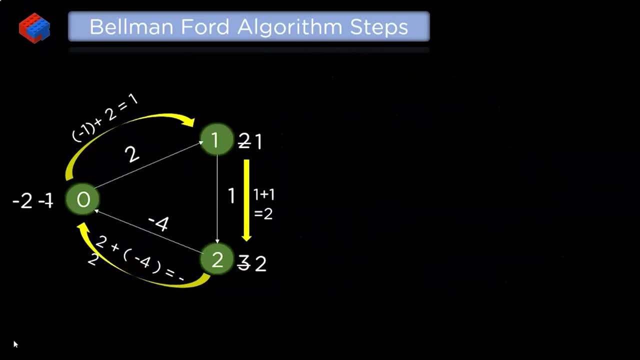 Which will be equal to two, And we know that It is less than three, So we will replace three by two. Finally, From two to zero, We have weight as minus four, So the cost will be Two plus minus four, Which is equal to minus two, And minus two is less than minus one. 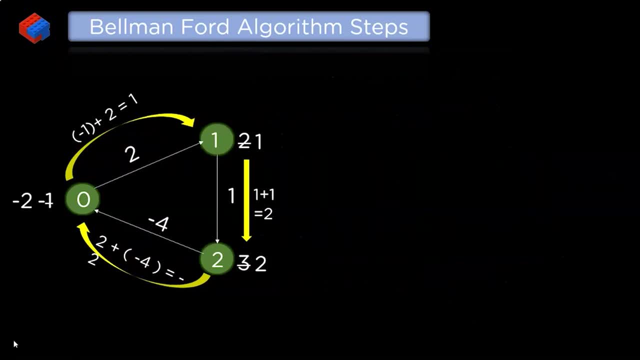 We will replace minus one By minus two. We have finished the first two times Of relaxation, So let us try the third time. In the third time of relaxation, We have the weight from zero to one As two, And the cost will be minus two plus two, Which is equal to zero. 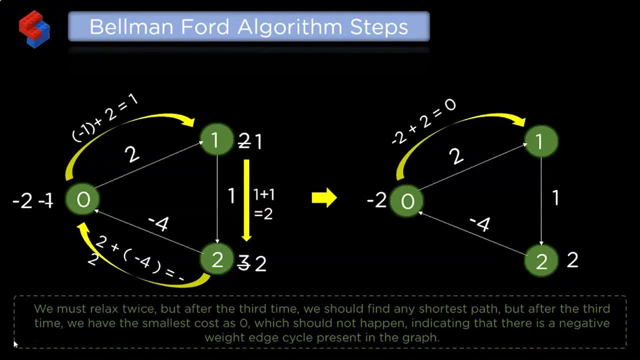 And zero is less than one, So we will replace One by zero. So after performing the third time, We have minimum distance as zero, Which should not happen Because we only had To relax it twice. We must relax twice, But after the third time We should find the shortest path. 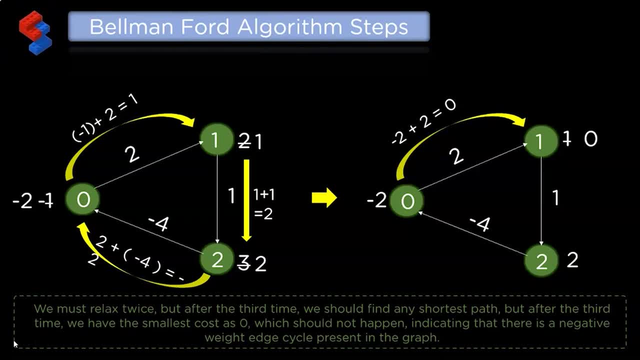 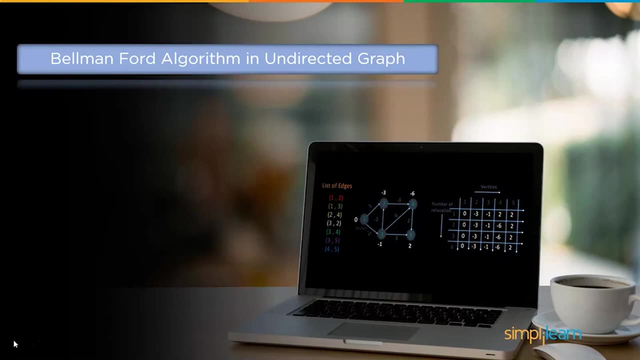 But after the third time We have the smallest cost as zero, Which should not happen, Indicating that There is a negative weight edge cycle Present in the graph. Next we will see How the Bellman-Ford algorithm Works on an undirected graph, For example. Here we have a graph of 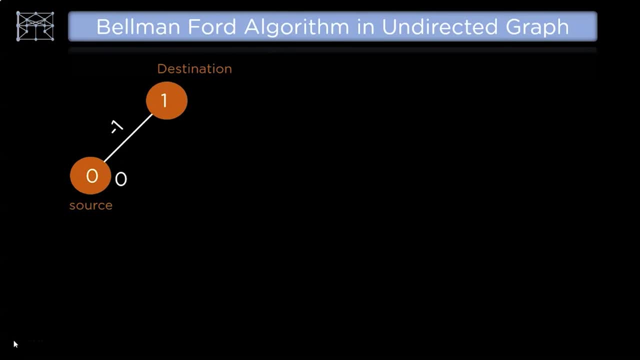 Two vertices: zero and one. So when we go from Undirected edge zero to one, The cost will be calculated as Zero plus minus one, Which is equal to minus one. Now, From edge one to zero, The edge will be Minus one plus Minus one, Which is equivalent to minus two. 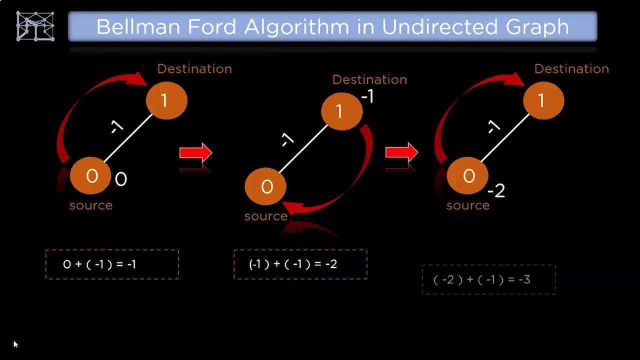 Now again To calculate the minimum cost. It will be minus two plus minus one, That is minus three, And this will be turned as An infinite loop. So here we come With the two points. The Bellman-Ford algorithm works only If all the edges are undirected. 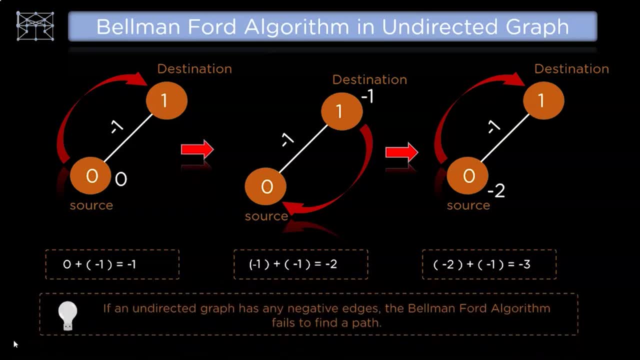 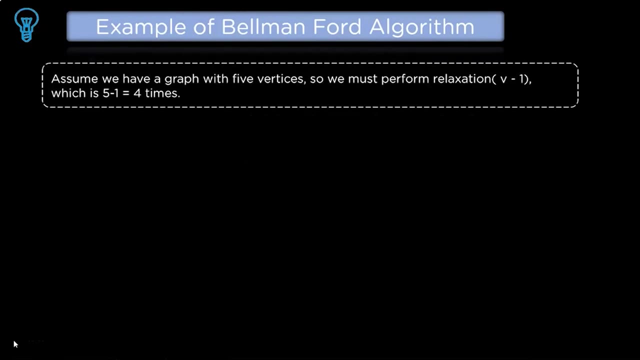 Graph are positive. If an undirected graph has Any negative edges, The Bellman-Ford algorithm Fail to find a path For better understanding. Let us look at an example For Bellman-Ford algorithm. Assume that we have a graph With five vertices, So we must perform relaxation. 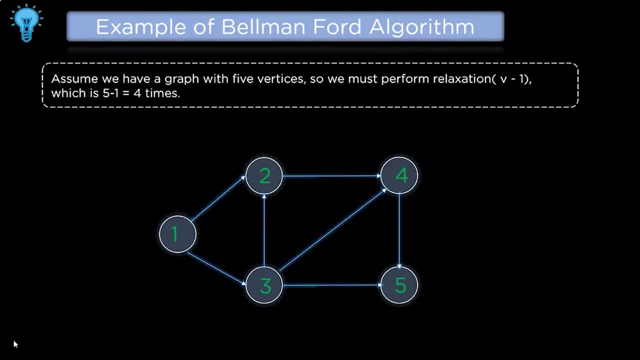 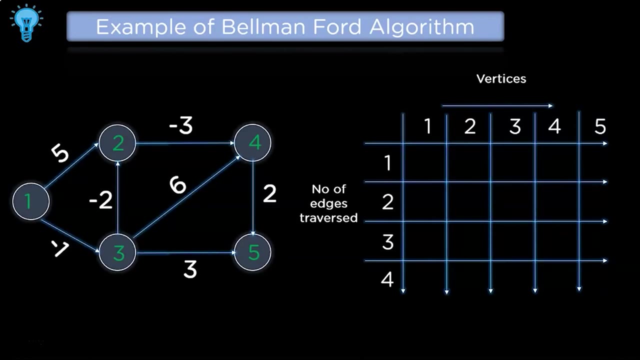 V minus one times, That is five minus one times That is four. Following, that is a table In which we will update The minimum cost of the edges Of this graph, Where the column is for vertices And edges is for the number of edges traversed. Next we have a list of edges. 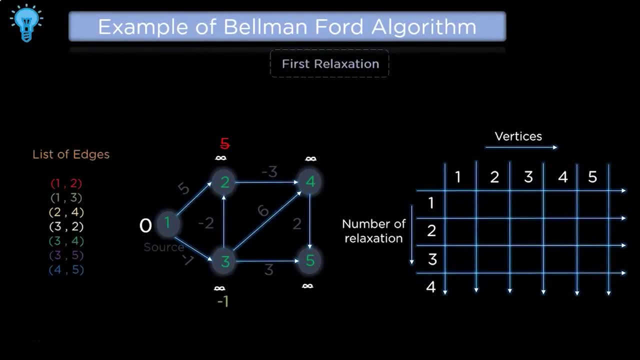 From one to three, Two to four, Three to two, Three to four, Three to five And finally four to five. From one to two edge, The cost will be Zero plus five, Which is equal to five, Which is less than infinity, So that we will replace it with five. 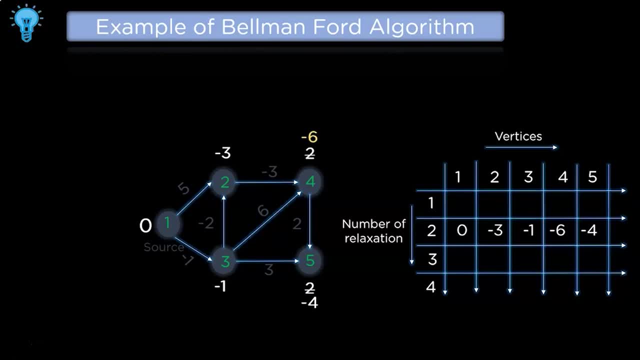 From one to three edge, The cost will be Zero minus one. Now, from two to four edge, We have the weight as minus three, So the cost will be Five plus minus three, Which is equal to two, And two is less than infinity, So we will replace it with two. 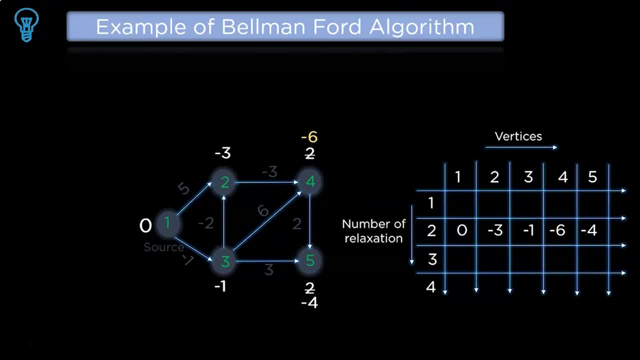 From three to two, We have the weight of minus two, So the cost will be Minus one plus minus two, Which is calculated as minus three, And minus three is less than five, Which is equal to minus three. Now, from three to four, We have the weight as six. 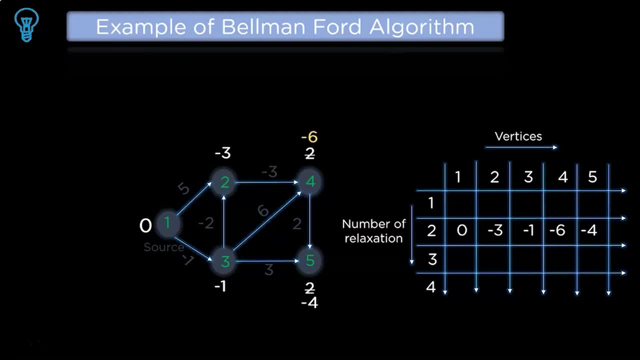 So the cost will be Minus one plus six, Which will be calculated as five. But five is greater than two, So we will not replace it. Now. we have an edge of Three to five, Where the weight is three And the cost is calculated as Minus one plus three. 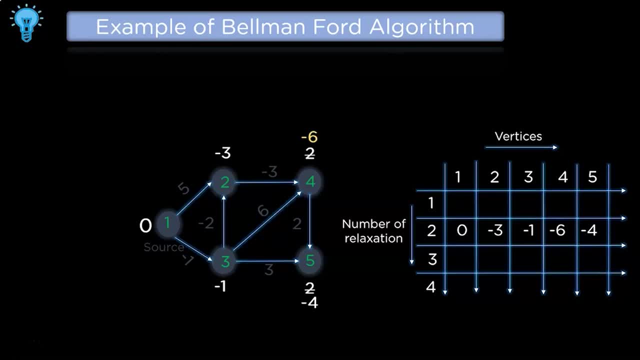 Which is two, And two is less than infinity. So the cost will be Four to five, Where the weight is two And the cost is calculated as two plus two, Which is four. But four is greater than two, So we are not going to replace it. So in the table of the first relaxation, 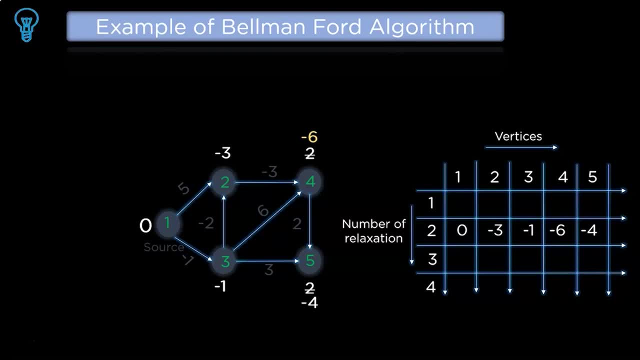 We will now update all the vertices With minimum cost. Now let us move into second relaxation From one to two edge. The cost is zero plus five, Which is equal to five Greater than minus three. The cost is zero Plus minus one, Which is equal to minus one, But we already have minus one. 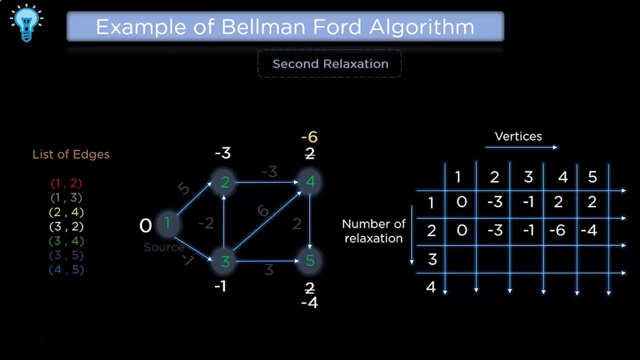 As vertex number three, So we will not update it Now. we weigh minus three From the two to four edge, So the cost is Minus three plus minus three, Which is equal to minus six, And minus six is less than two, So we will replace it by Minus six. 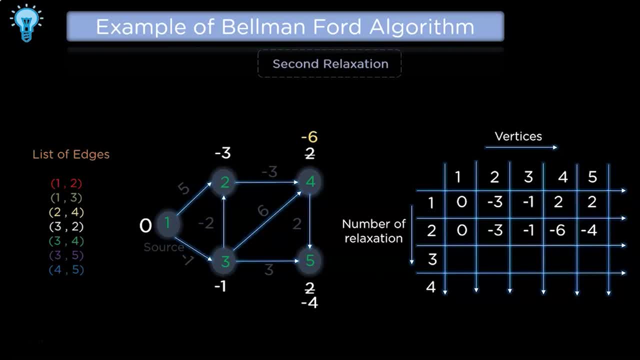 From three to two, Which is equal to the weight of minus two. So the cost will be Minus one plus minus two, Which is equal to minus three, And minus three is already there, So we won't update it Now that we weigh six. from Three to four. 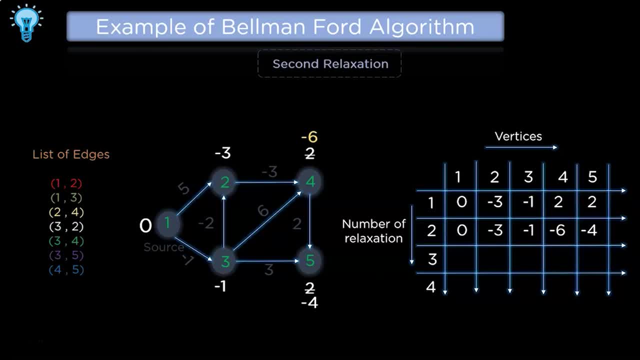 The cost will be Minus one plus six, Which is calculated as five. But five is greater than minus six, So we will not be replacing it Now. we have Three to five edge And the cost is calculated as Minus one plus three, Which is equal to two. 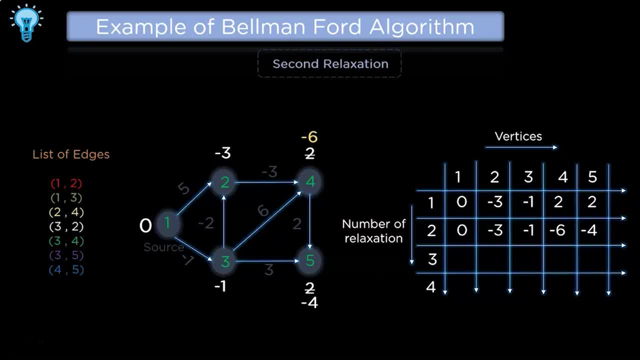 And two is already there, So we won't update it. Finally, we have a Four to five edge, where the weight is two And the cost is calculated as Minus six plus two, Which is equal to minus four, And minus four is less than two, So we will replace: 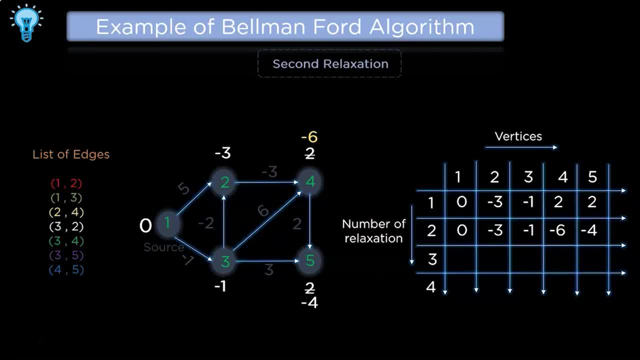 Minus four by two. So in the table of second relaxation We will update all the vertices With minimum cost. Now let us move to third relaxation stage. From edge one to two, The cost is zero plus five, Which equals five, Which is greater than minus three. So we will not replace it. 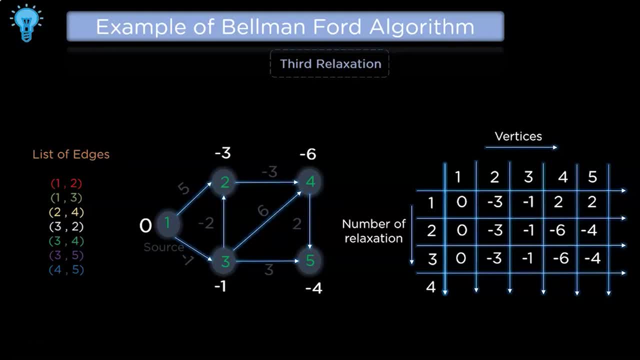 From the edge one to three. The weight is minus one And the cost is estimated as Zero plus minus one, Which equals minus one, But we already have minus one As vertex number three, So we will not update it. Now. let us weigh Minus three from the edge two to four. 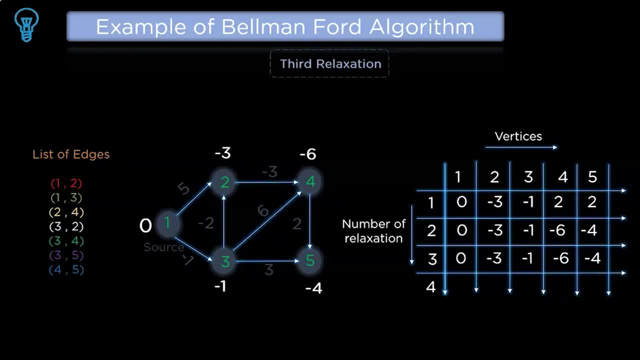 So the cost is Minus three plus minus three, Which equals to minus six. And minus six is already there, So we will not update it. From three to two. We have the weight as minus two, So the cost will be Minus one plus minus two, Which equals to minus three. 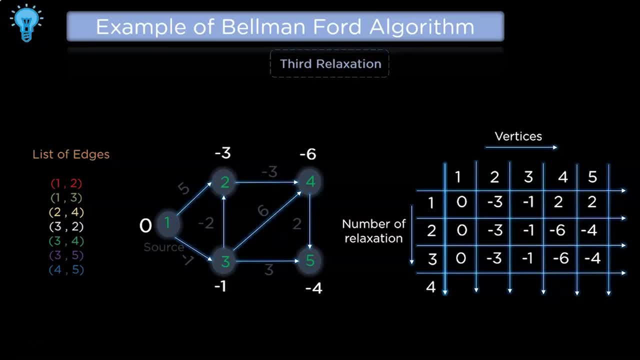 And minus three is already there, So we won't update it. Now that we weigh six, The cost will be Minus one plus six, Which is calculated as five, But the value of five is greater than minus six, So we will not replace it. Now we have the edge. 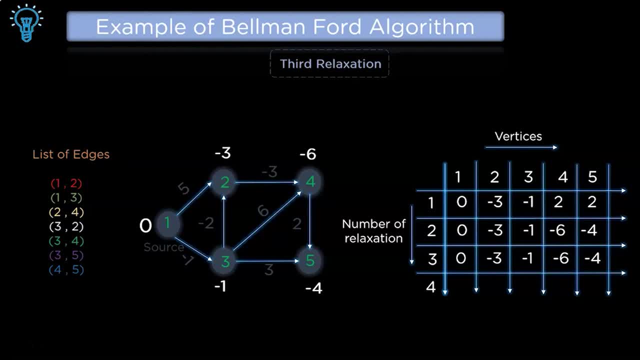 Three to five, With the weight as three And the cost is calculated as Minus one plus three, Which equals to two And two is already there, So we won't update it. Finally, we have a four to five edge Where the weight is two, Which is calculated as: 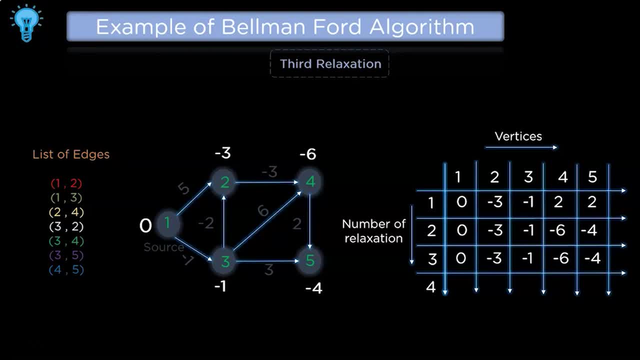 Minus six plus two And it is minus four, And minus four is already there, So we will not do anything. So in the table of third relaxation We will now update all the vertices With minimum cost. As we can see, We got the exact minimum cost For the third relaxation. 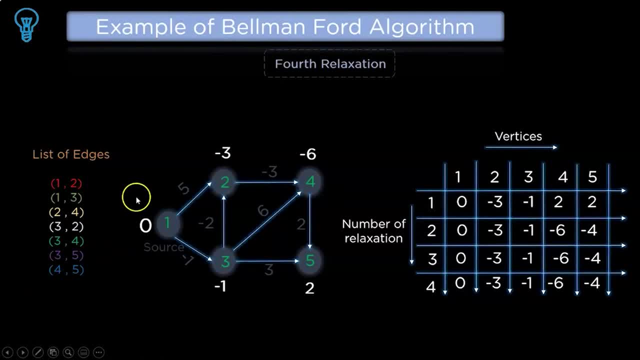 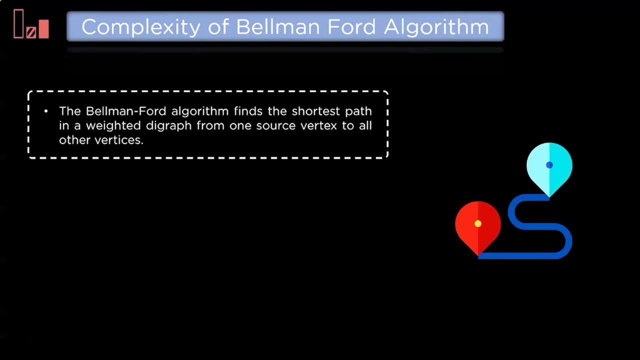 As we did for the second, Which means we will get the actual minimum cost For the fourth time of relaxation. And now we have calculated All the edges. Following that, we will examine The complexity of Bellman-Ford's algorithm. The Bellman-Ford algorithm Finds the shortest path in a weighted 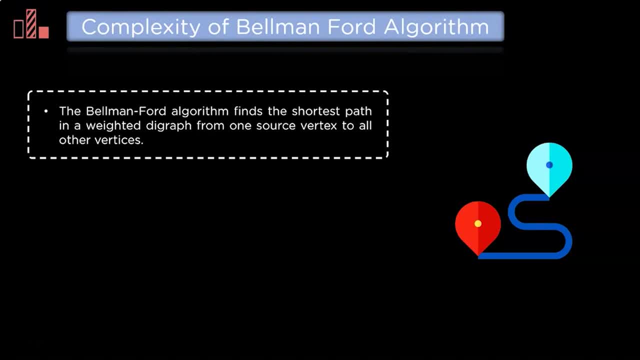 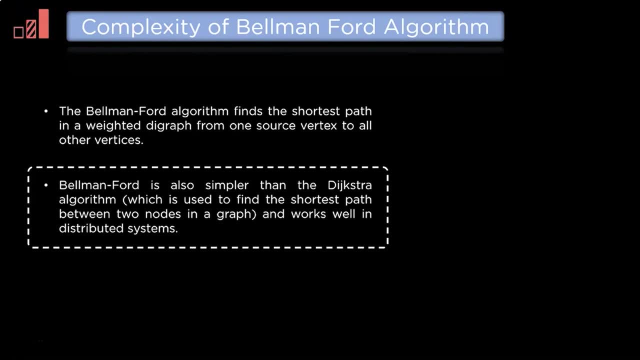 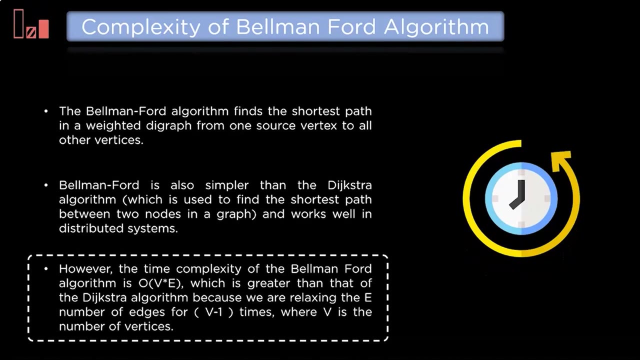 Diagraph from one source vertex To all the vertices. Bellman-Ford is more straight forward Than the Dijkstra's algorithm Used to find the shortest path between Two nodes in a graph, And works well in distributed systems. However, The time complexity of Bellman-Ford algorithm is 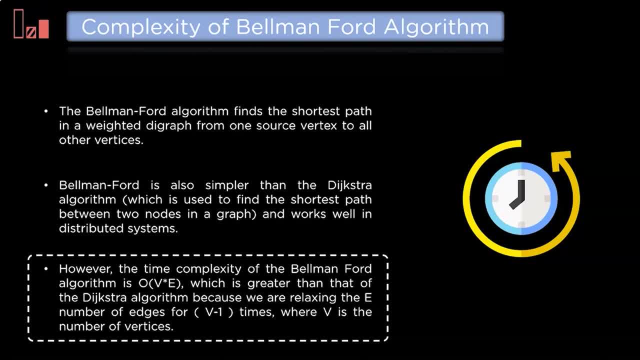 The number of v into e, Which is greater than that of the Dijkstra's algorithm, Because we are relaxing The edges. e number By v minus one times, Where v is the number of vertices. Now, these were the complexities Of Bellman-Ford algorithm. Now let us get into practical mode. 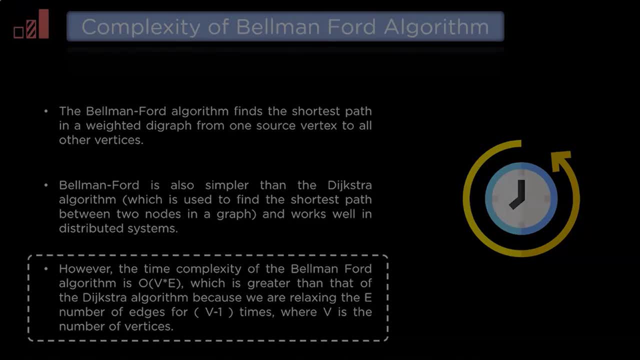 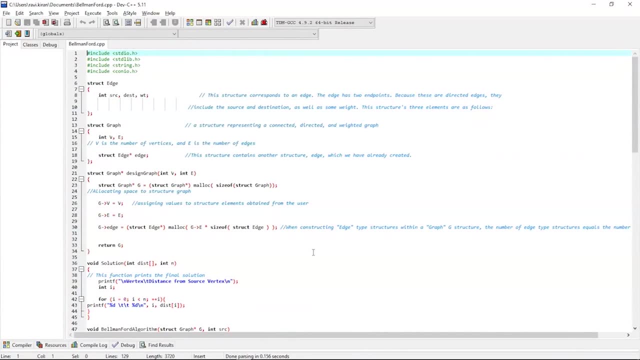 Where we will be executing an example Based on Bellman-Ford algorithm. Now on my screen you can see an example Based on Bellman-Ford algorithm. First, We finished all the necessary header files, Standard input output, Standard library String and all the console input output libraries. 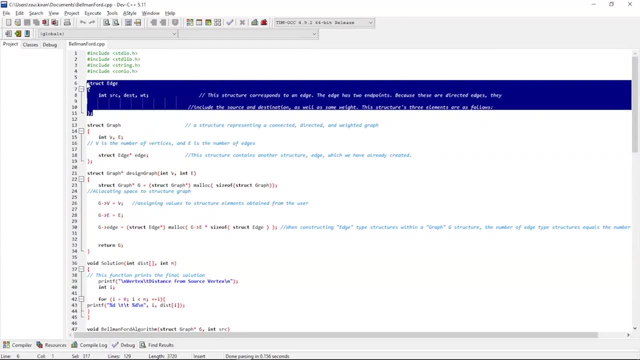 Then, Using the struct keyword, We created an edge. This structure is equivalent to an edge. There are two endpoints to an edge, Because these are directed graphs. They include the src as the source And dest as destination And Some wt as weight, Where three components of the structure are. 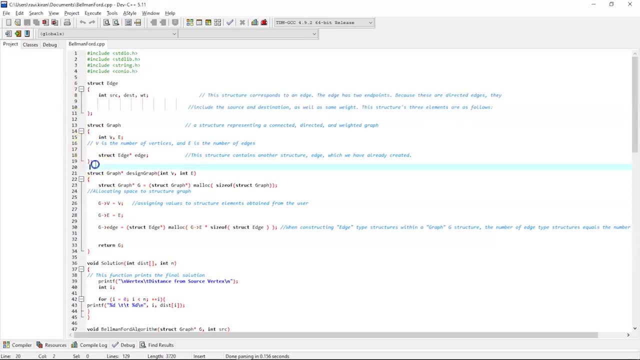 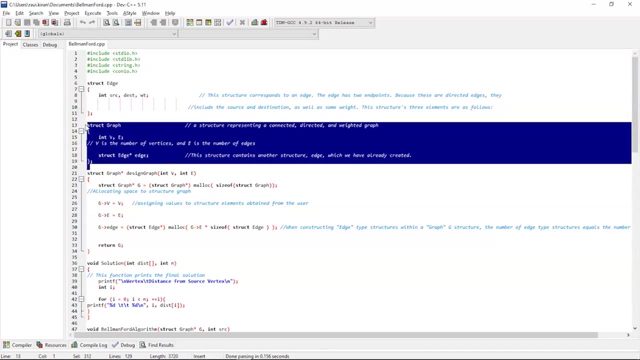 As follows. We used the struct keyword to create a graph With two variables, v and e, Where v is the number of vertices And e is the number of edges. We also made an edge And this structure contains another structure edge Which we had previously created. Now We have created a function called 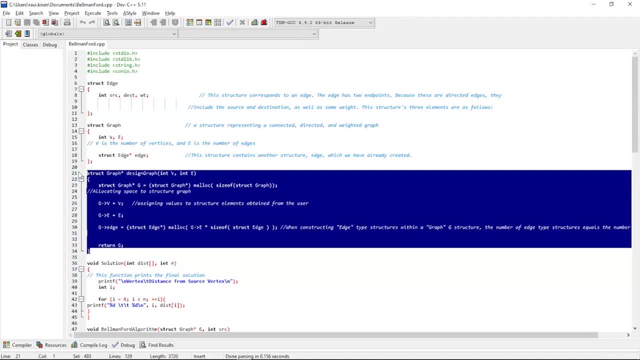 DesignGraph Which contains v and e. Using the malloc function, We created a graph in this function Which contains v and e values To the structure elements obtained from the user In this graph. Then we make an edge And return the graph. Now we have created a solution Which is a function. 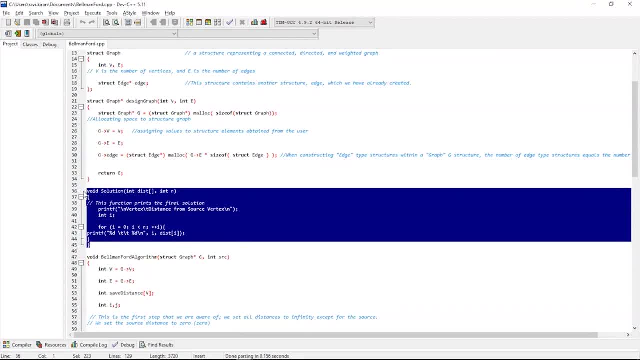 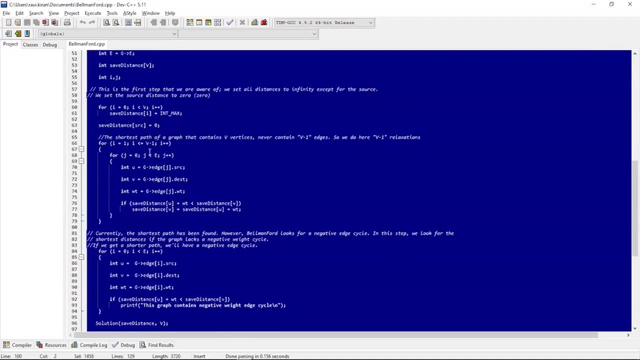 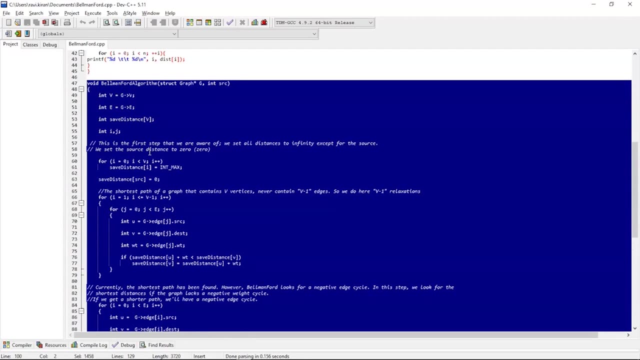 And this function prints the final solution too. We print the distance from source vertex. For this We make a loop from 0 to variable n And print the distance. Then we created the Bellman-Ford algorithm function With graph and source variables As parameters And edges to the graph again. 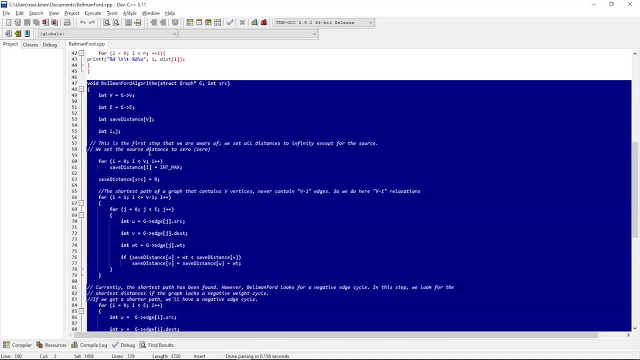 Finally, we make an array called SaveDistanceWithSize as a vertex. After that We declare two counter variables, i and g. After that We run a loop from 0 to the number of vertices, And in this loop We set all distances to infinity, Except the source. 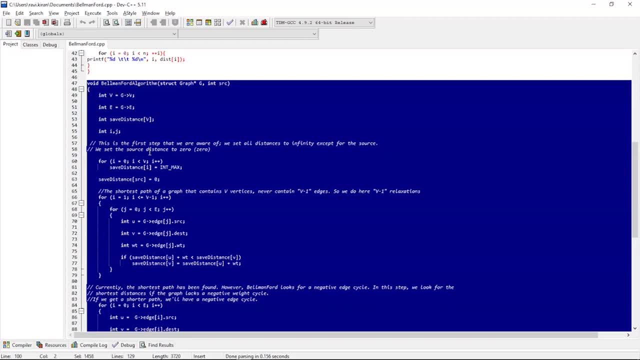 Which is set to 0. Now we run a loop from 1 to v-1 times, Followed by another loop For the edges. We have three variables: u, where we assign the graph's source, v, where we assign the graph's destination, And wt, Where we assign the graph's weight. 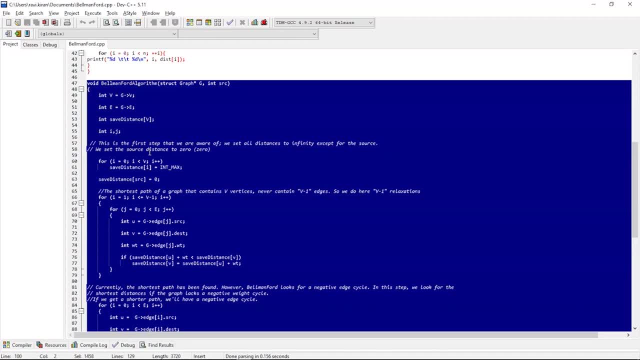 Now we have a condition That if the distance of the source node And the weight of the uv-edge is less than the distance Of the destination node, We update the destination node To be the distance, the source node Plus the weight of the uv-edge. Now We run a loop from 0. 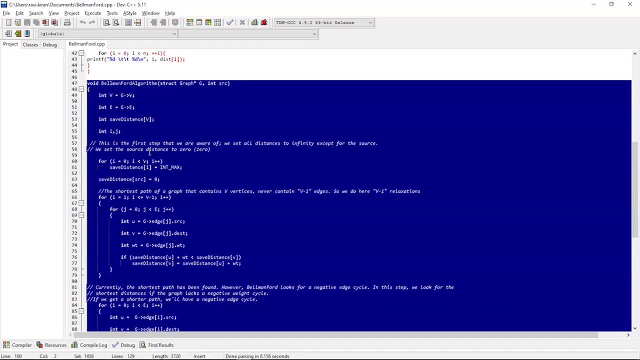 After that We set all distances to infinity, And in this loop We declare two counter variables, i and g. After that We run a loop from 0 to the number of vertices, And in this loop We set all distances to infinity And wt, Where we assign the graph's edge. 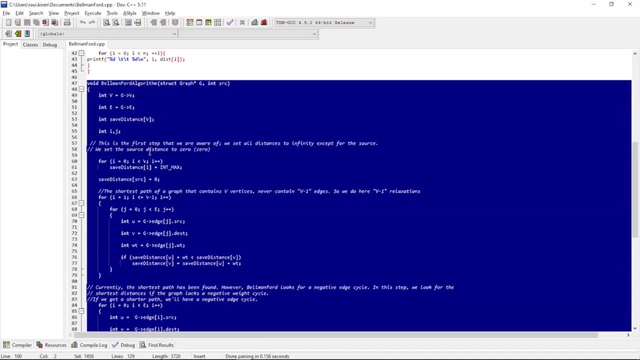 uv and assign all source, Destination and weight of the graph, And we have the condition To print the number of vertices And s, where v is the number of vertices, e is the number of edges And s is the source vertex. And we ask the user to print the number of vertices. 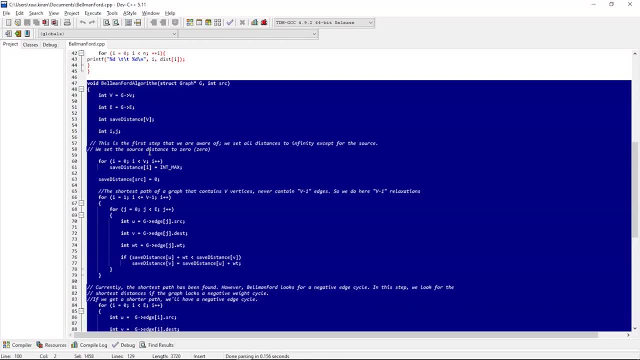 Edges and source vertex, After which We call the design graph function, Which prints the source, destination and weight Respectively, And finally We call the Bellman-Ford algorithm function To implement the Bellman-Ford algorithm. Now I hope I made myself clear with the code. 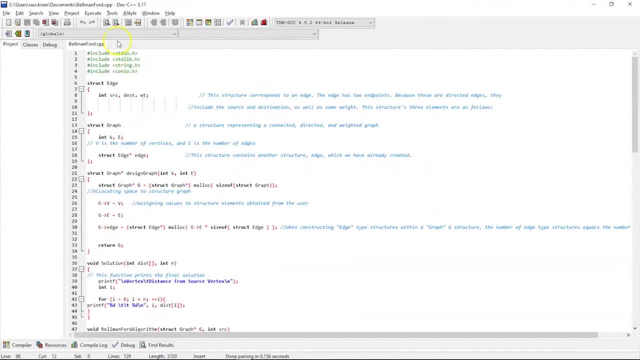 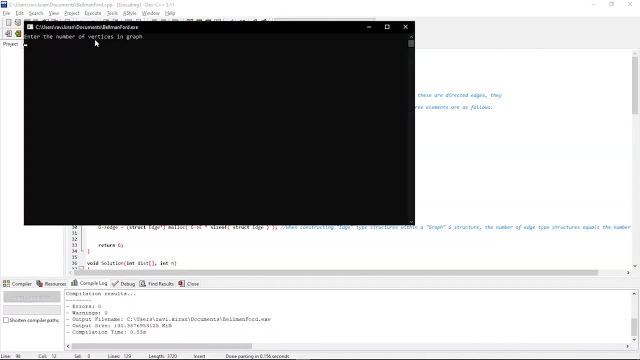 Let's try to run this code quickly, To run the output. So to run this code, We might want to press on the execute button Now. let's press the compile and run option. Now you can see that The code got successfully executed And now it is asking for input. 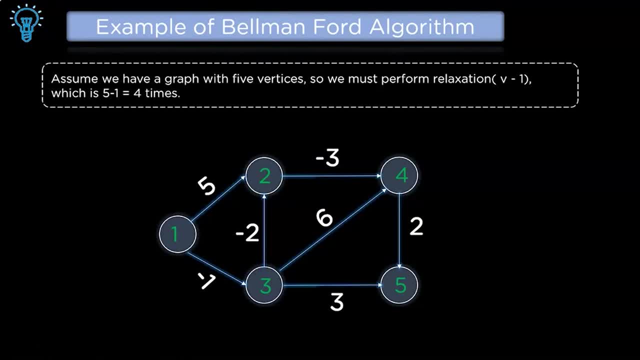 Now we will consider the same example That we have seen in the PPT, Which is this particular example With 5 vertices and 7 edges And all the weights Which are present in this particular image. Now let's get back to the output window And try to provide the inputs. 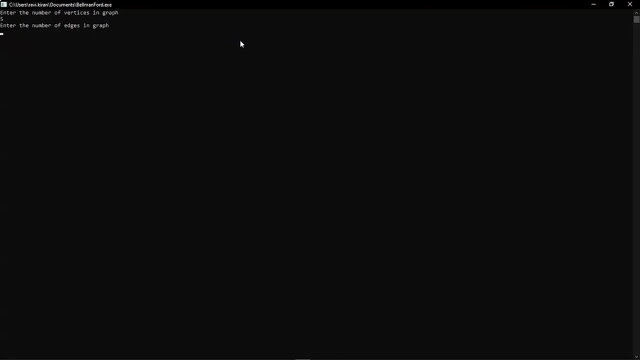 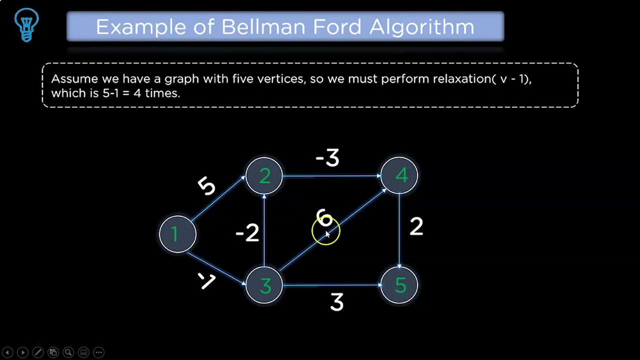 So enter The number of vertices in the graph. So we have 5 vertices In this particular graph. As you can see, we have 5 vertices And enter the number of edges In the graph. So let's count the edges. So 1,, 2,, 3,, 4,, 5. 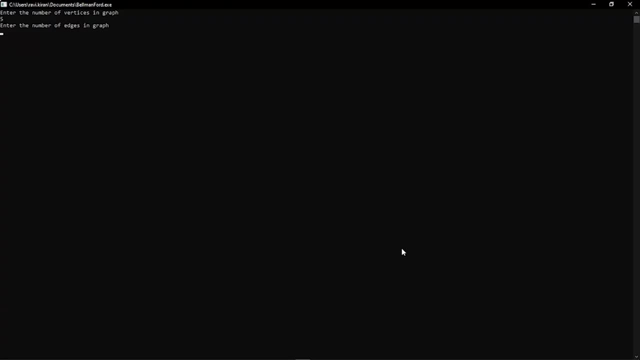 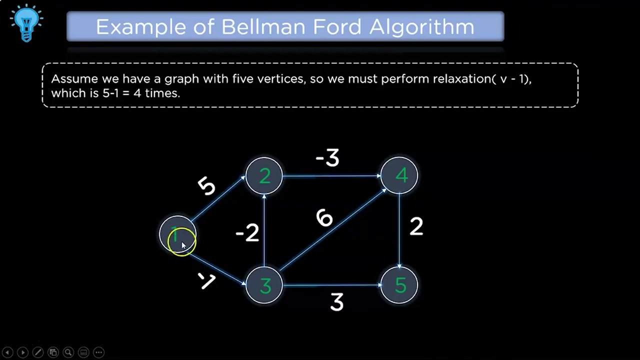 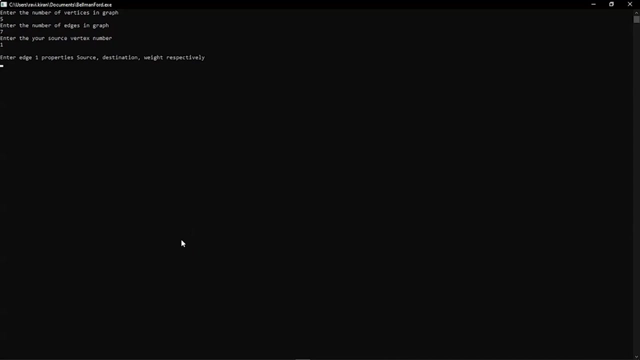 6 and 7. So we have 7 edges in the graph. Now enter the Source vertex number. So the source vertex number is: So let us provide 1. Now enter the Edge 1 properties. So we have to enter The source of the edge 1. 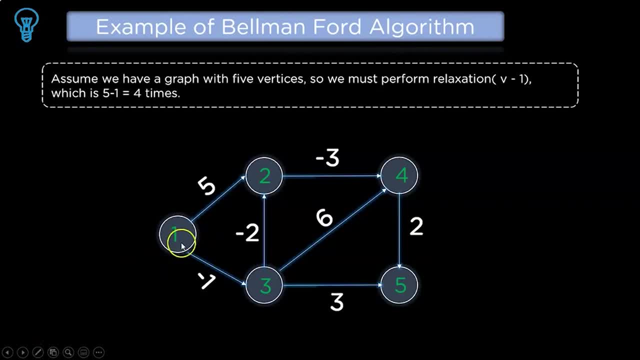 Its destination and its weight Respectively. So here we have the first Edge, that is 1 to 2. So the source is 1 and the destination is 2 And the weight is 5. So we have to enter 1,, 2 and 5. 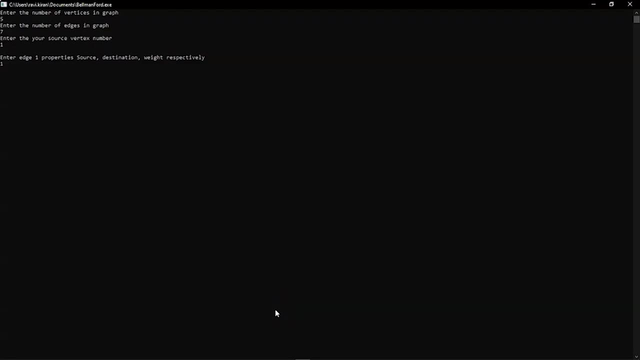 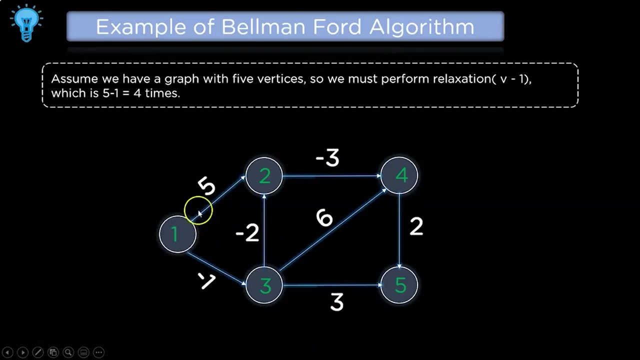 And so on. So the source is 1, Destination is 1 And the weight is 5. Now it will ask for the next Edge, that is, edge 2. Let us finish all the edges from vertex 1. So again We will provide the source as 1. 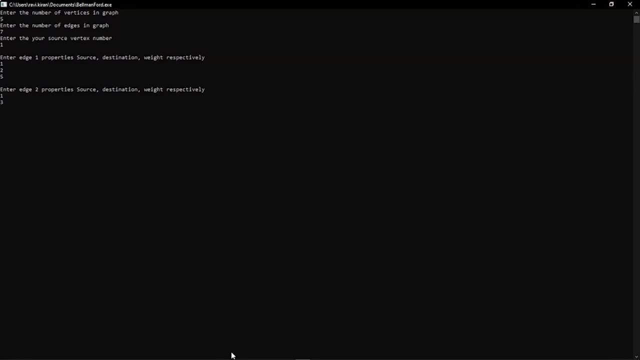 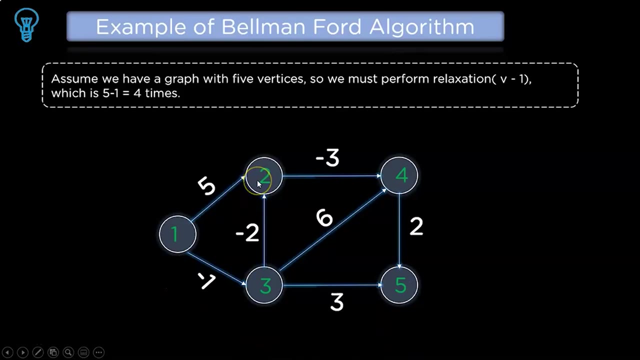 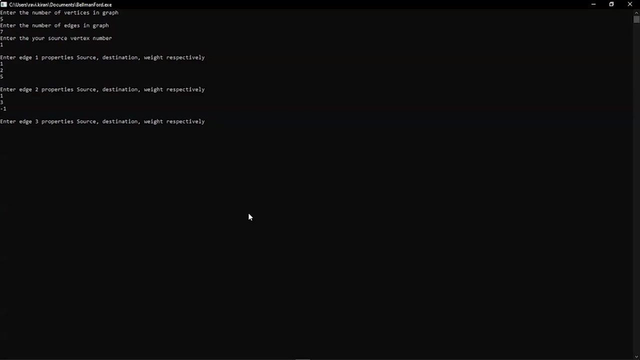 And destination As 3, So the weight is minus 1. Now enter the Edge 3 properties. Now let us go to the vertex 2. So from vertex 2 we have just 1 edge which is going towards 4. Let us enter the data: Source is 2. 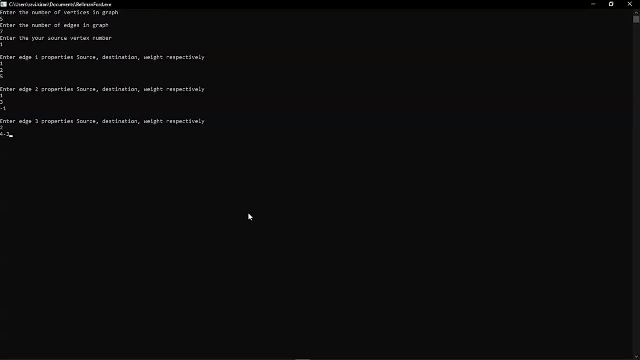 Destination is 4 And weight is minus 3, So let us go to the next vertex, That is 3. So from 3 we have 3 edges. So let us enter the data 3 and the first Destination is 2, With weight minus 2. 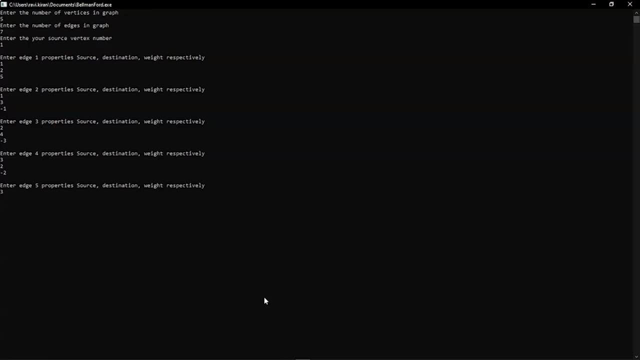 Now the source will be 3 again. This time it is going towards 4 with weight 6. Another last edge, That is from source 3 To destination 5 with weight 3. Now the 7th edge, That is 4 to 5, So the 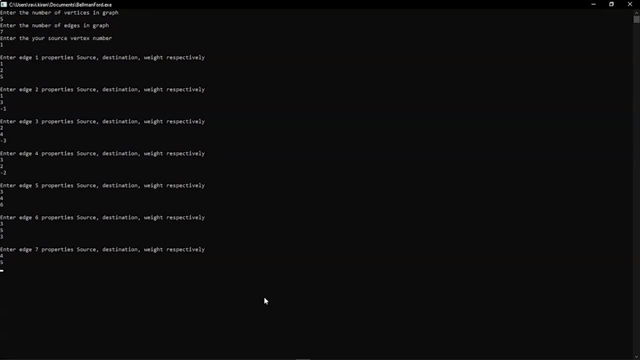 Source is 4, destination is 5 And the weight is 2, So let us enter and we will have our Answer. So the vertex, distance from the source vertex- is Here. you can see the answers. So from 1 we have 0 And from 2 we have. 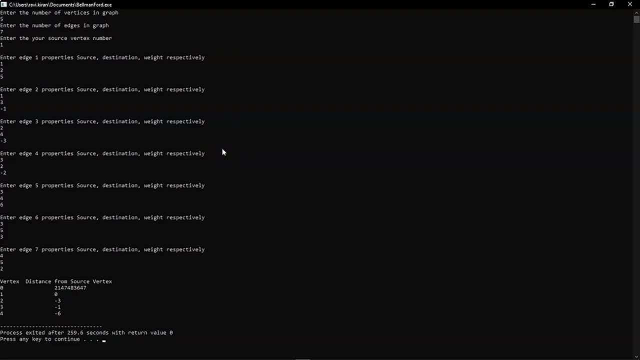 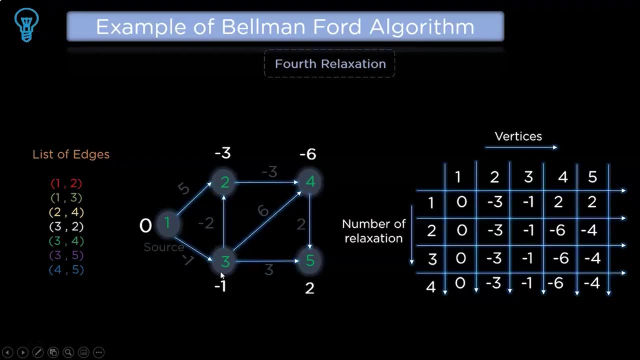 Minus 3, that is here, And from 3 we have 1, which is over here, And from 4 we have minus 6, which is over here. And this is how you get the Result for Bellman Forge algorithm And this is how you implement it. 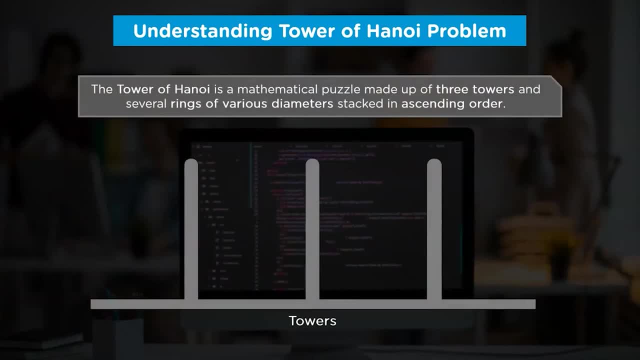 The tower of Hanoi is a Mathematical puzzle made up of 3 towers and multiple rings, Arranged in ascending order of their Diameters. the number of rods Or tower is fixed, Whereas the number of rings can be changed By the player. The setup of this game looks something like this: 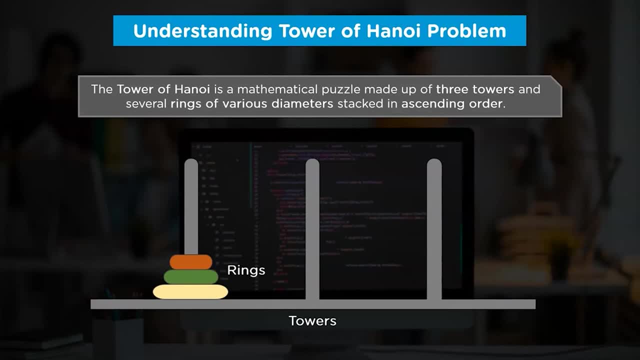 There are 3 towers in this diagram, And one of the tower Is decked with several number of Discs or rings, Such that the largest disc is at the Bottom and the smallest disc Is at the top. A player's goal is to move These discs, one at a time. 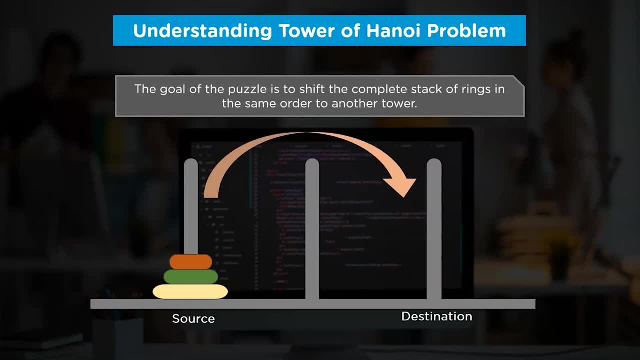 To a particular destination tower In the same specific configuration At the start. That means the order of disc Should not be changed after being Transferred to the destination tower. Before you get ahead of yourself And deem this problem to be trivial, There is one crucial aspect To consider. 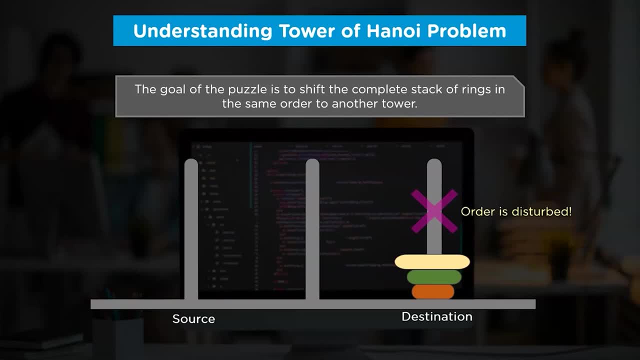 In this problem. you are not allowed to transfer A larger disc on the top of a Smaller disc at any stage. This rule makes solving this problem Substantially difficult. However, this problem Can be solved using the auxiliary tower Or helper tower By altering the position of disc. 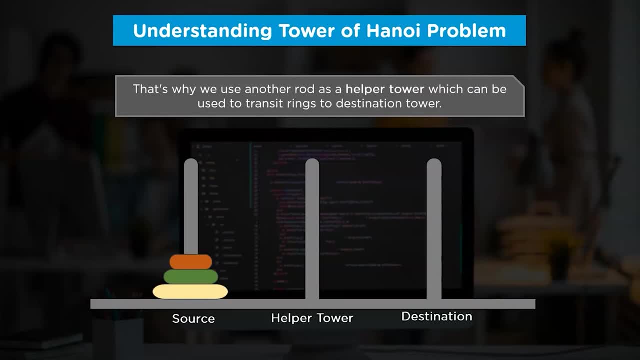 Between 3 towers, We can take all the disc present at Source tower to the destination tower. This is quite confusing, right? So to make this understandable To all of you, Let me give you a rough example. In this tower of hana problem, We have 3 rings at the source tower. 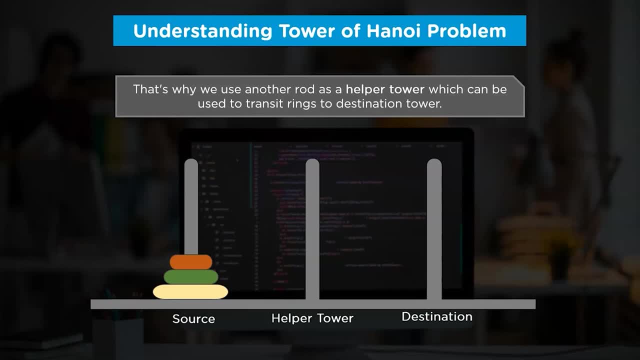 Now to attain the same sequence. At the destination tower, We will move the top 2 rings To the helper tower. After that we can move a ring With highest diameter. Now, if we just move the 2 rings Present at the helper tower To the destination tower, We will solve our problem. 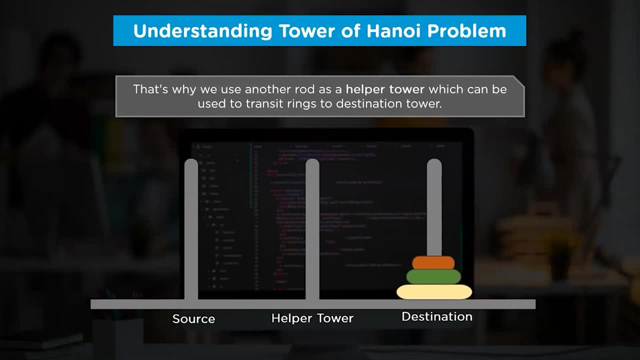 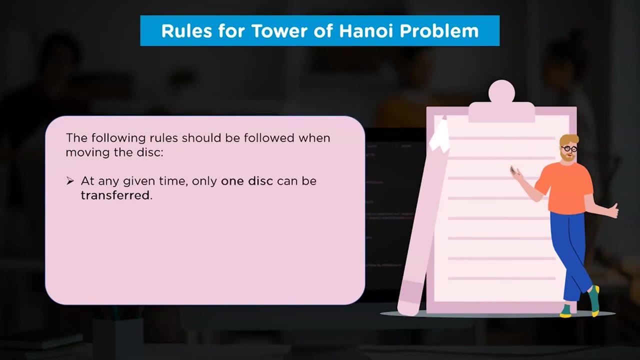 But let me tell you guys That this explanation Was just to make you visualize This problem more straight forward manner. In reality, this problem becomes more complex When the rules for the movement Of rings are applied. So, moving forward, Let's look at those rules for Ring movement in the tower of hana problem. 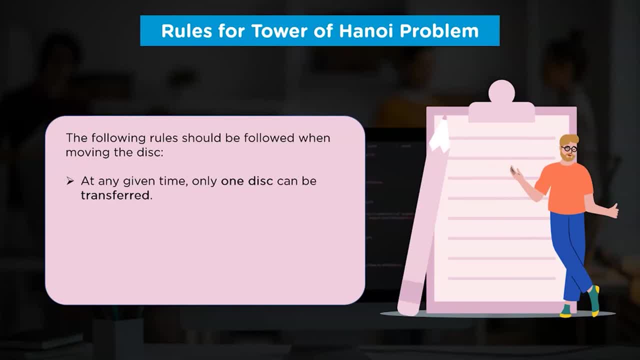 The first rule that we have Is that in any instance, Only one disc can be moved from the tower. That means we cannot move More than one disc at a time. The next rule on our list Conveys that a disc can only be moved If it is the uppermost disc. 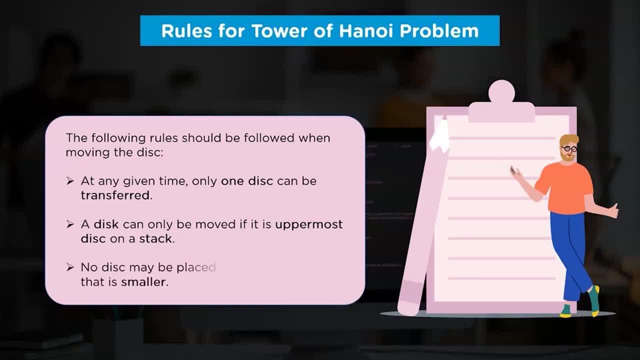 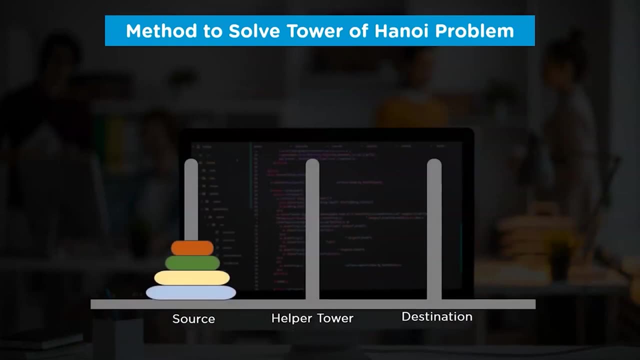 Of the stack. The last and essential rule Is: no disc should be placed On the top of another disc That is smaller in size. So let's look at another tower of hana problem To build solution using These set of rules. In this problem We have four discs to increase. 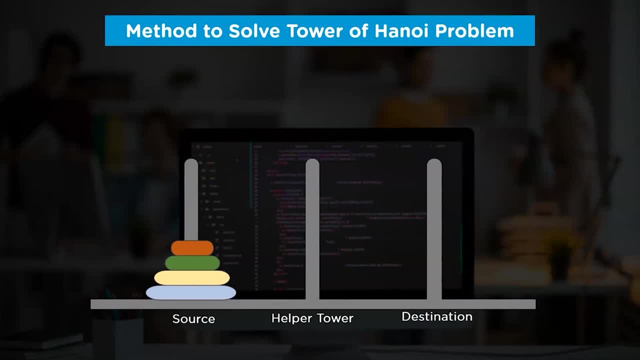 Our problem's complexity, Whereas the number of towers Remains the same. In order to formulate the solution, We are allowed to move these rings Into different towers. So the first move we are supposed to do Is moving the orange disc To the helper tower. Next, we can move green disc. 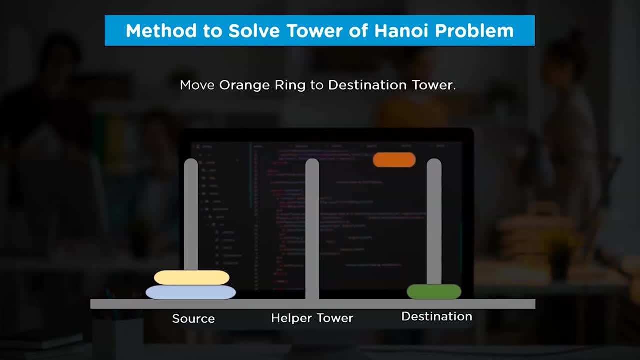 To the destination tower And after that We can move the orange disc. To place this orange disc Over the green disc. Now our helper tower is empty, So let's take out our yellow ring From the source tower to the helper tower. Now we will move the orange ring. 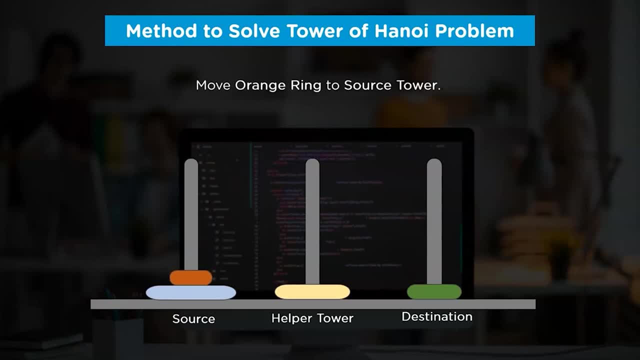 To the source tower. Further, We will move green ring To the helper tower. This movement will make our Destination tower empty So that we can bring this larger disc To it. Next, we will move orange ring To make room for the transfer of Largest disc to the destination tower. 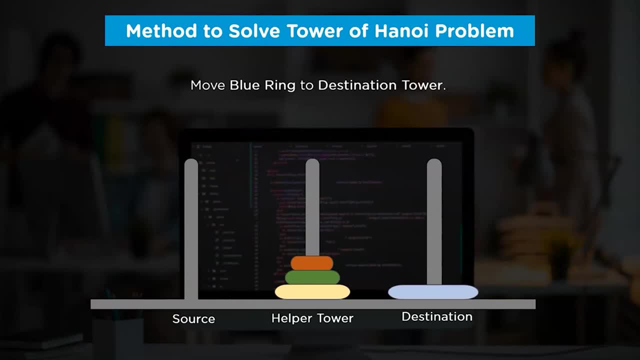 Now We have brought our largest disc To the destination tower. However, we still need to bring Three more discs to our destination tower In order to solve this TOH problem. And to do that Here we will move orange ring To the destination tower And the green ring to the source tower. 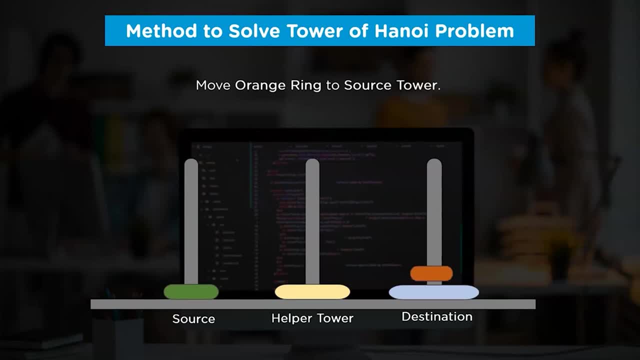 After that, We will move orange ring to the source tower In order to bring the second largest Ring to our destination tower. Here we have successfully placed Two rings at the destination tower. Now we only left with arrangement Of two more rings To attain that. Here we will move orange ring. 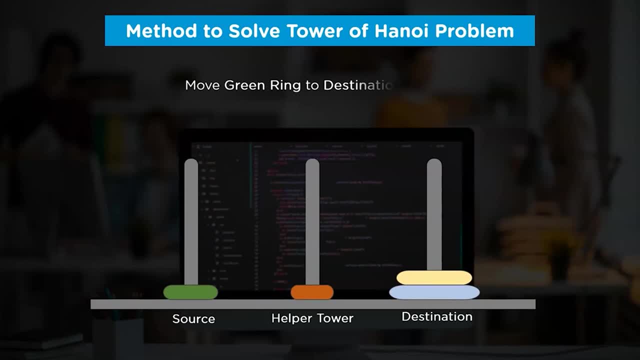 To the helper tower And green ring to the destination tower. Finally, We will move orange ring To the destination tower And this is how we will land That accurate solution to our tower of HANA problem. If you observe this process, You will get that: The process of ring movement. 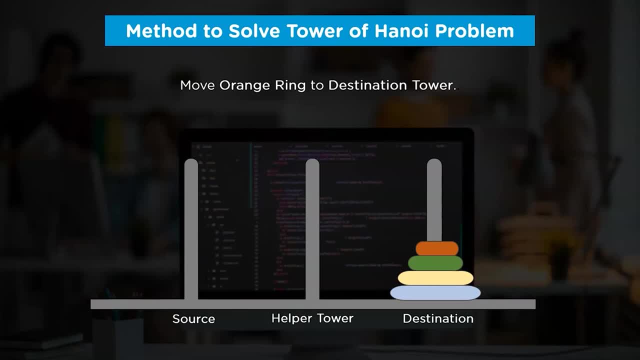 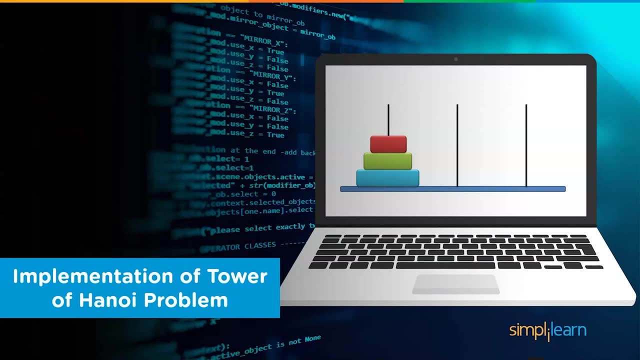 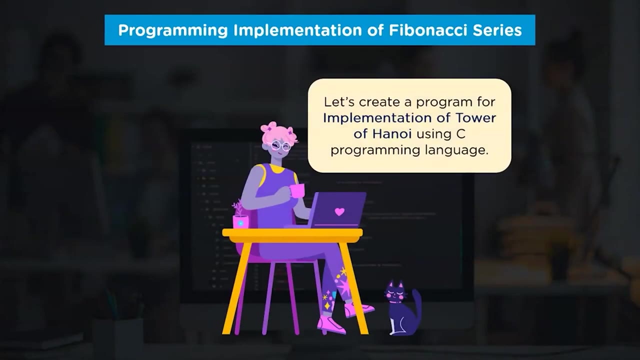 Is of recursive nature And we can develop a solution to this problem Using recursive programming paradigm. So, moving ahead, We will develop a program To implement a solution To this tower of HANA problem. The language that we are going to use For this implementation Is C programming language. 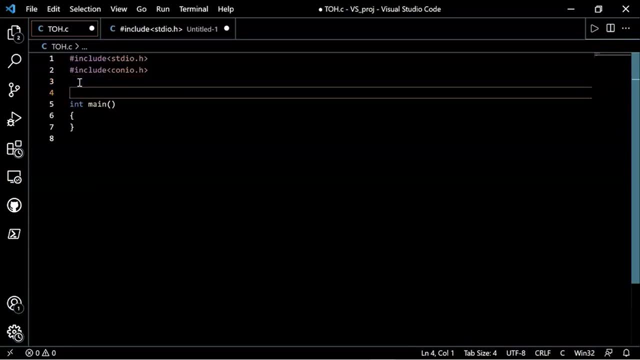 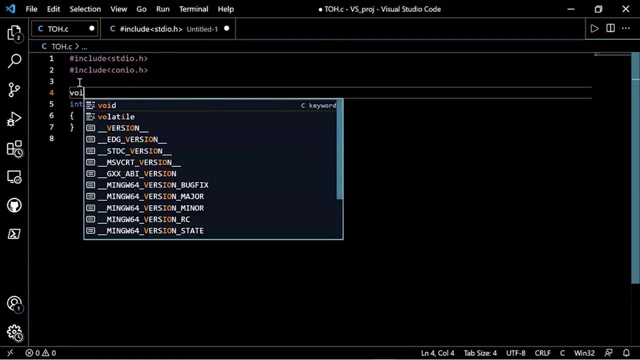 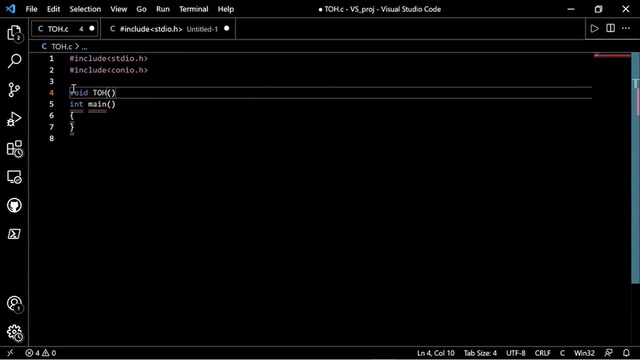 So, without wasting any time, Let's move to the code editor For tower of HANA implementation. Let's first create an utility function Named toh. So we will do that void toh, And inside this function We will pass few arguments. The first argument we will pass: 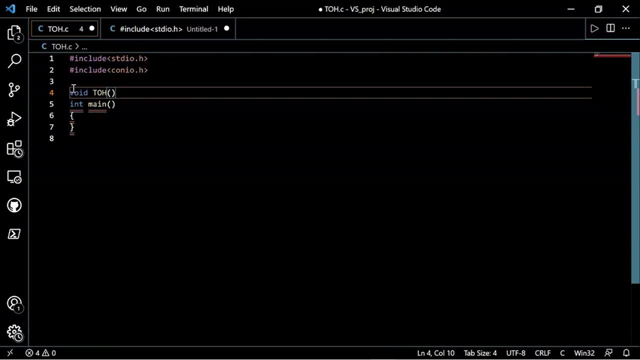 To this function will be The number of rings in our toh problem, So let's call that Variable n And the subsequent Arguments will be the source tower, Destination tower And helper tower. All these three arguments Will be of character data type, As we want to pass the names of towers here. 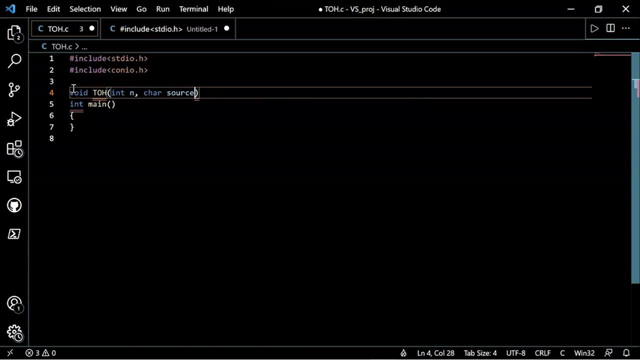 So we will create Car source Next, Car destination And Car Helper Tower Next. We will make recursive call To the same function In order to move the disk Inside. this recursive call Will tell our IDE to move n-1 disk from source tower To the helper tower And to do that. 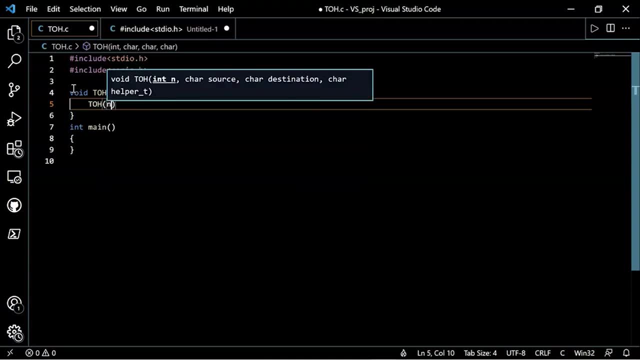 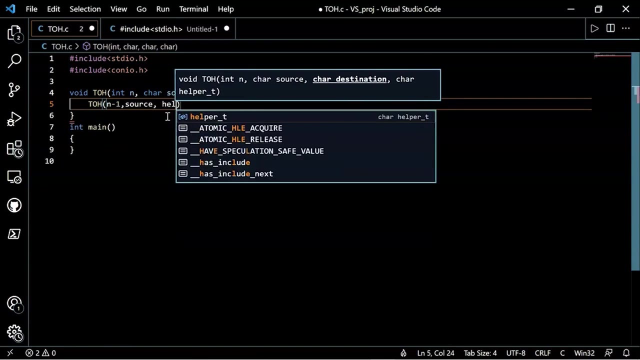 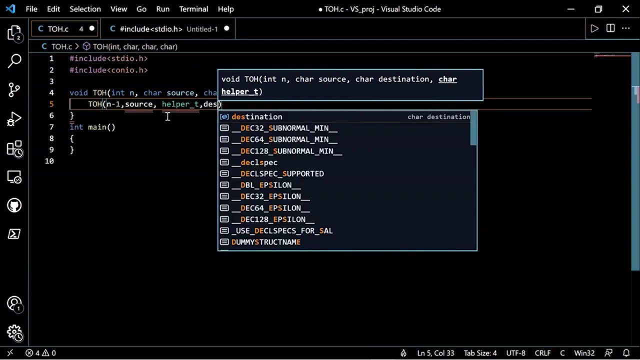 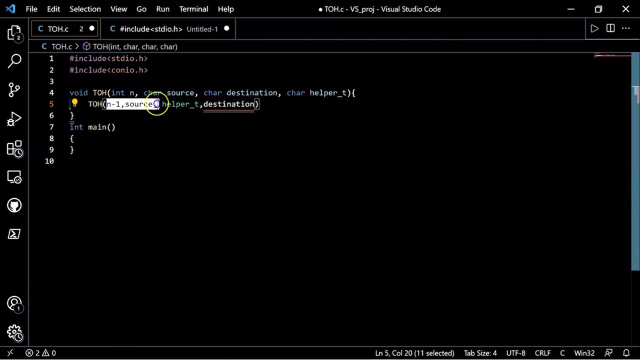 The statement that we will write is: toh, Move n-1 disk, That is this n, Next Will be the source, Then helper Underscore t, Which will act as destination Here, and Destination tower Will act as an Helper tower. So basically, this call Is nothing but these arguments. 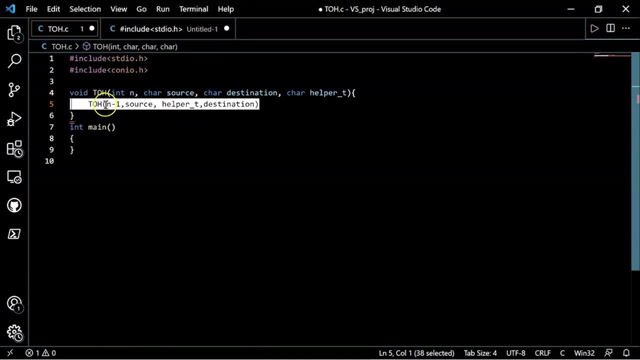 Over here. This recursive call will allow n-1 rings to move from Source tower to the helper tower By taking the help of Destination tower. So by using this statement, We have moved n-1 rings From source to the helper tower. Next, what we will do is: 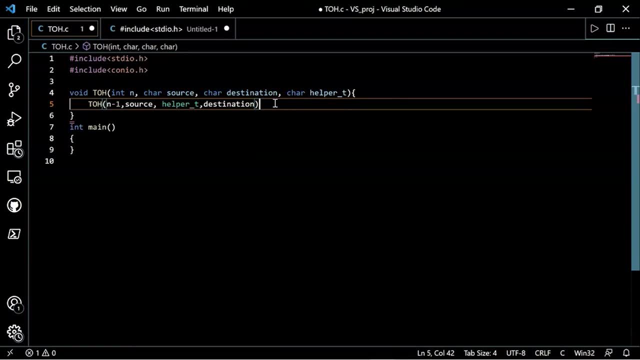 We want to print all these movements Covered by this function. Hence let's create a format For printing the disk movement Using printf function. The format that we will use is: printf- Add, slash, n. Move Disk Modules d From Tower Modules c To Tower Modules c And after this, by taking 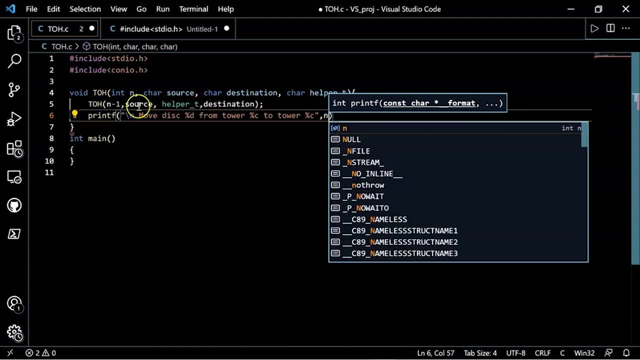 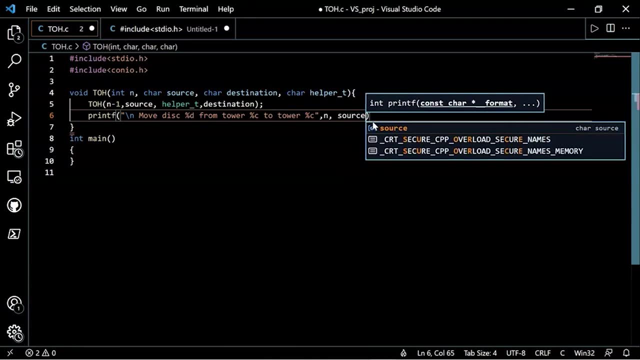 Comma will pass arguments. The first will be Modules d, that is Number of tower. Next will be the source And after that it will be Destination. So by moving n-1 disk to the helper tower We have made space for Moving the largest disk To the destination tower. 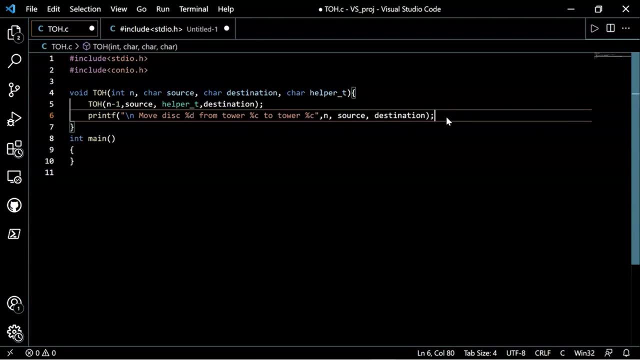 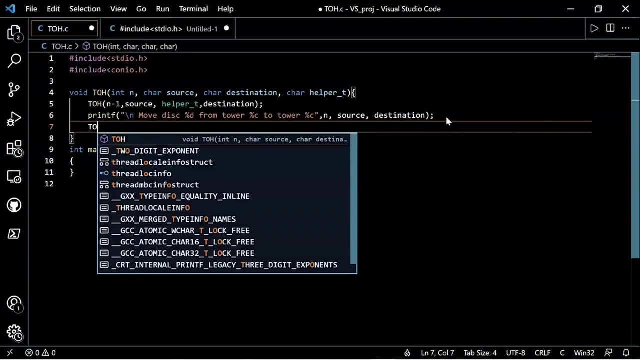 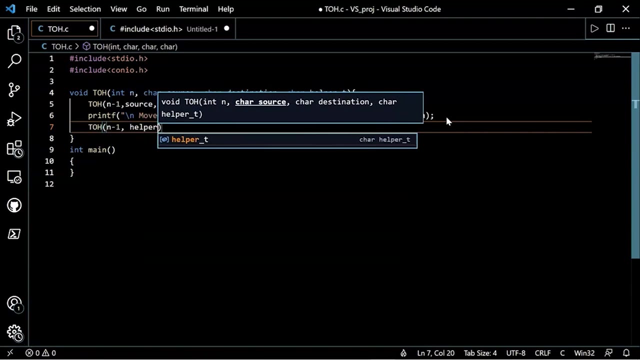 And next we will have to move this n-1 rings to the destination tower From the helper tower by using The source node. So for that we will write another Recursive call toh n-1, Helper. underscore t Will act as source now And destination Will act as destination. 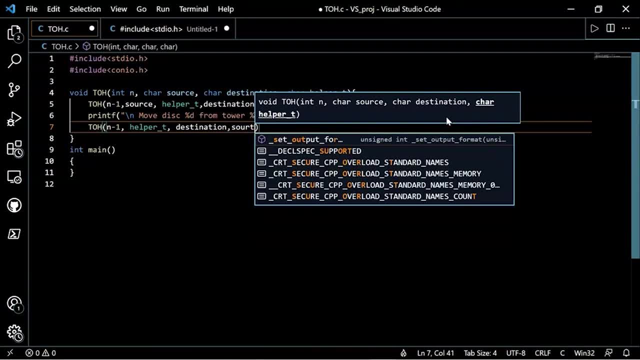 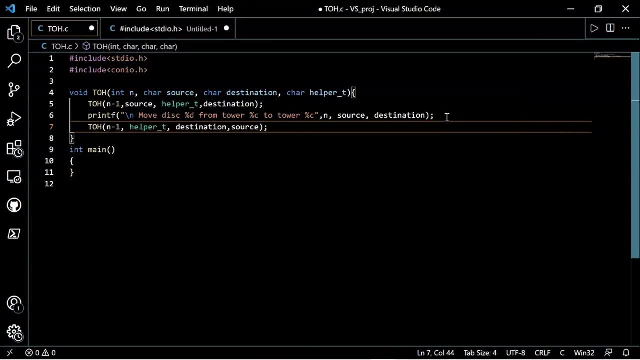 Where as source, Will act as Helper tower. Now, what will be the base Case for this recursive function? Well, it's pretty easy. The recursive call we are making Is actually decreasing the disk number, That is, n-1, And thus, after few iterations, The value of n will become zero. 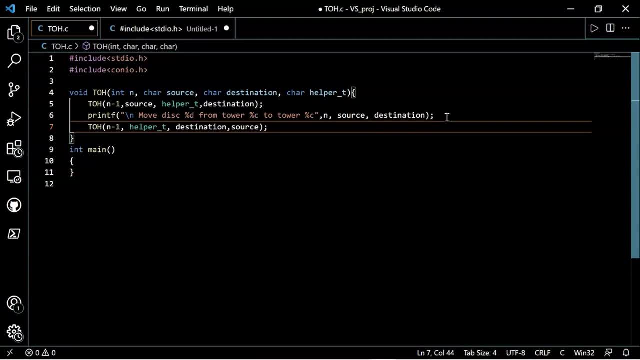 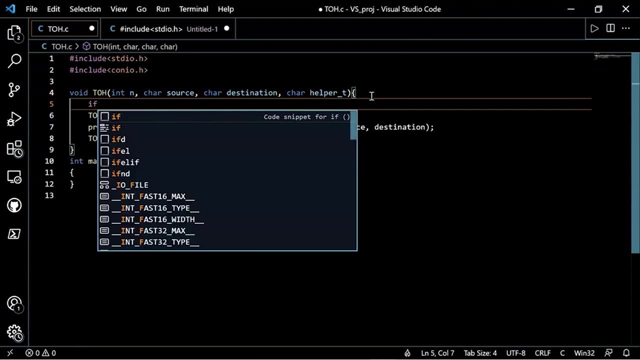 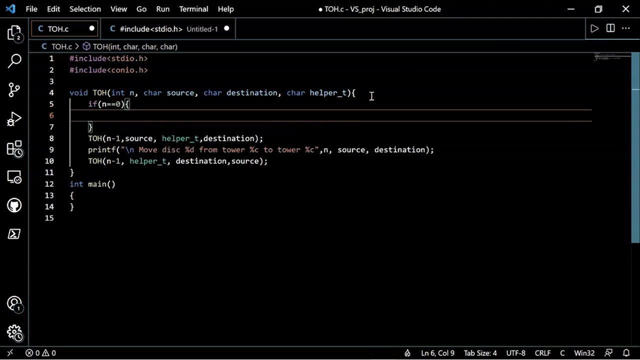 And when it reaches zero We want to stop our recursion. So our base condition Will be: If n Becomes equal to Zero, We will Return the control To the next function. So with this We have successfully created Our tower of n-1 function. Next we will move to our driver. 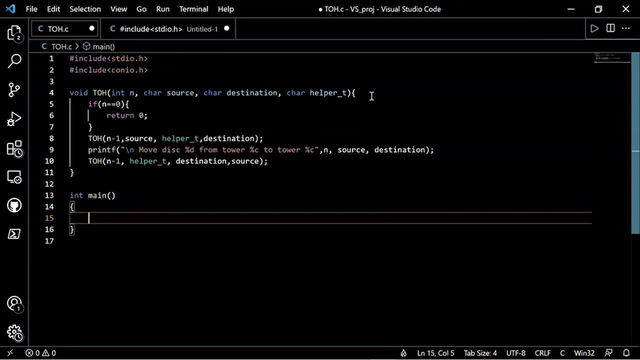 Method, that is, main method, In order to contemplate the toh Function. So what we will do is We will pass arguments to Toh function. The number of rings that we are going to use For this problem will be four, And let's call Our towers as a. 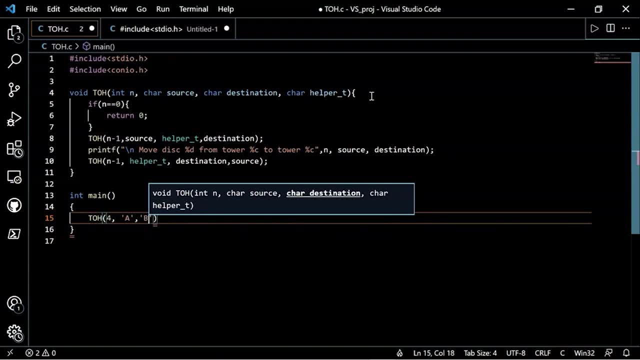 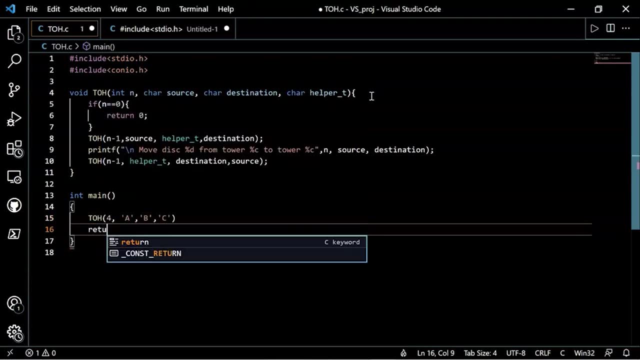 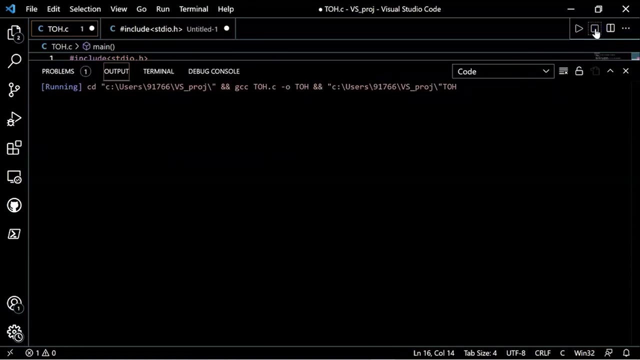 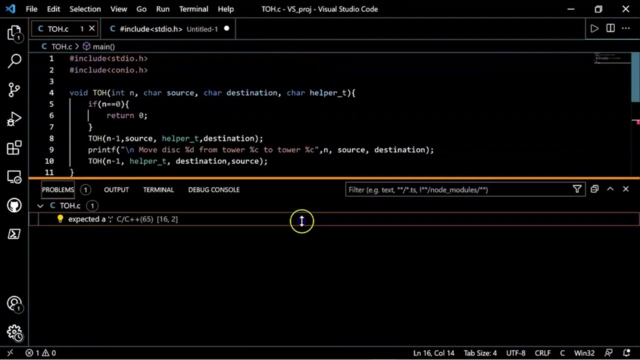 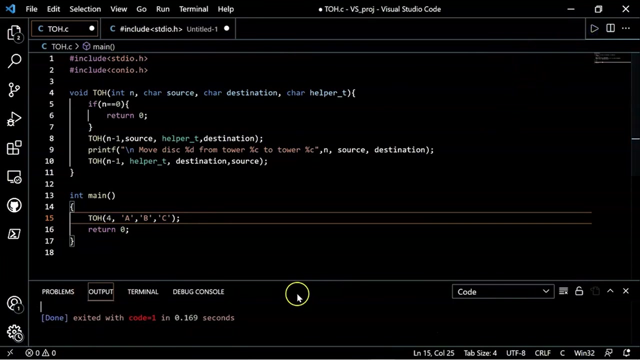 Then b And c And Return Zero. Now let's Check if our code works Fine or not. Okay, so we are getting One error over here, Semicolon missing. Okay, so let's add that semicolon And rerun our code. Okay, so we have received Output here. 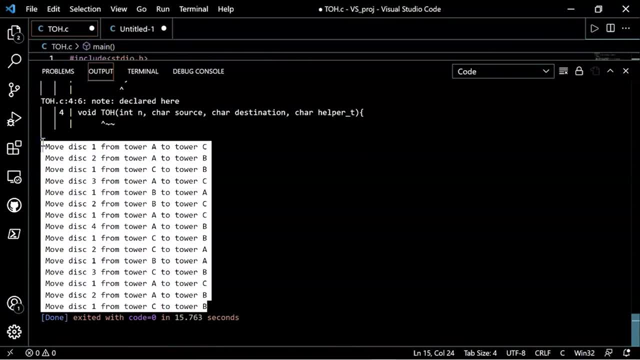 The output is fifteen steps That we have discussed earlier For the four rings toh problem, And that output is What we have received here. That means our program works accurately. You can verify this output By matching these movements With the previous solution That we have discussed earlier. The only thing to note here is: 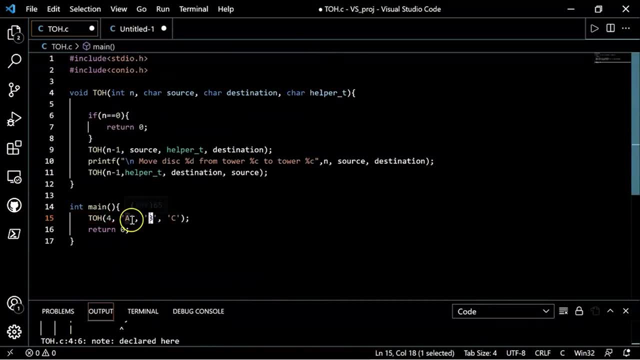 That the tower b is Acting as destination, Tower a is acting as source And tower c is acting as Helper tower. I hope you guys are clear with Tower of Hanoi implementation. now, This is all about Tower of Hanoi implementation using C programming language. With that we have come to an end of this. 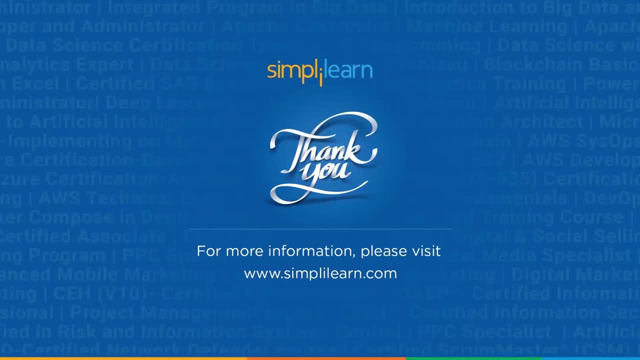 Session on dynamic programming. I hope this session was informative And interesting. if you have any Queries regarding any of the topics covered In this session, or if you need the code Executed in this session, then please Feel free to let us know in the comment section below And our team of experts will be happy.